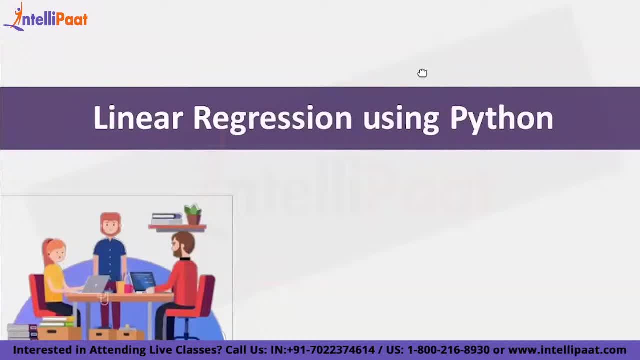 values are related with dependent, which tells the relationship between independent and dependent values. So now, having said all this, we will go ahead and then see how exactly these things are working right. so what is the base and how exactly these things are working? so how do we do this in going forward all these things? so, whatever you said right now, all of them. 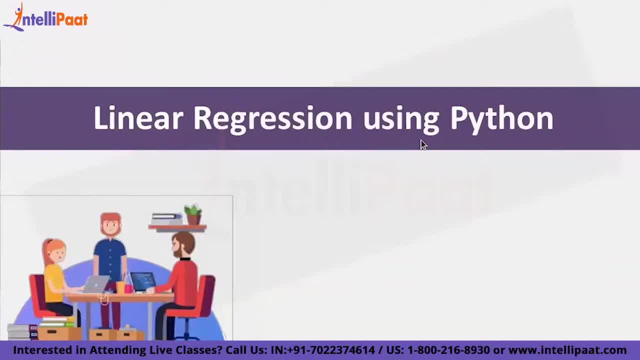 are in a way correct, right. I can't say that is hundred percent correct And at the same time I can't say it is hundred percent not correct also. so in a way, what you are saying is right, but it is not completely right. you're getting my point. what you're? 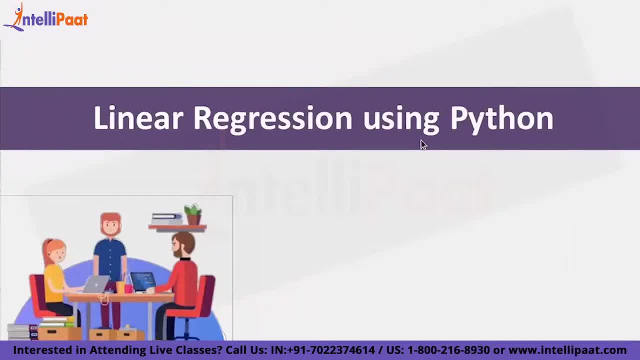 saying is right, but not hundred percent right is what I'm trying to tell you. having said that, now I will tell you what is linear regression. we will understand it from beginning and then how it works. a basic, first level understanding we will get. linear regression is a very, very 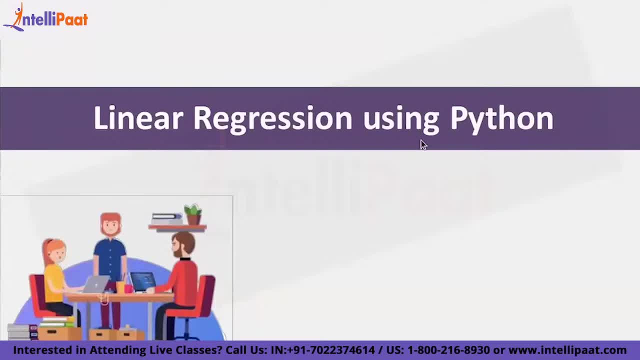 large topic, But I will give you Introduction to linear regression, from where you can pick up and then go deep, dive more deeper to an extent where you find comfortable right. So what is linear regression? how it works? I'm going to tell you right. 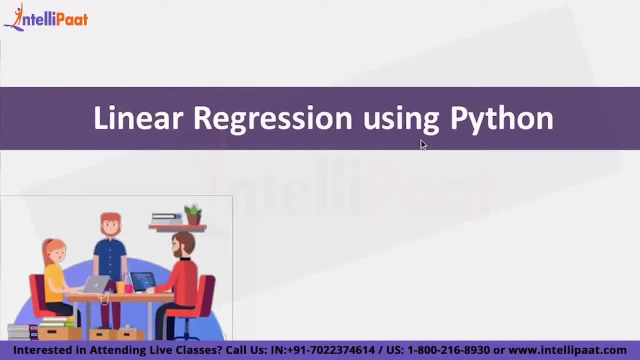 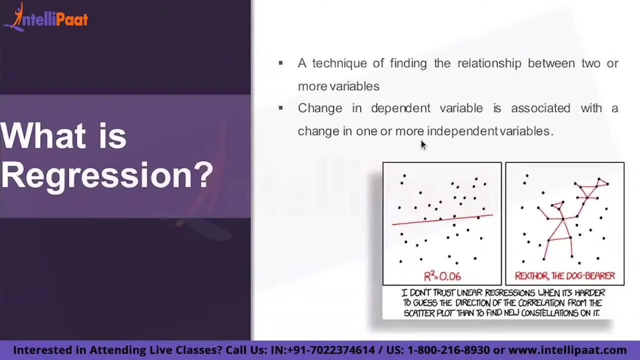 So linear regression using Python. So, basically, what do you mean by regression? right today is completely theory session, so I want you to focus, I want you to understand this theory concepts very well so that it will be useful whenever you're going to check for the further sessions. right, so understanding? 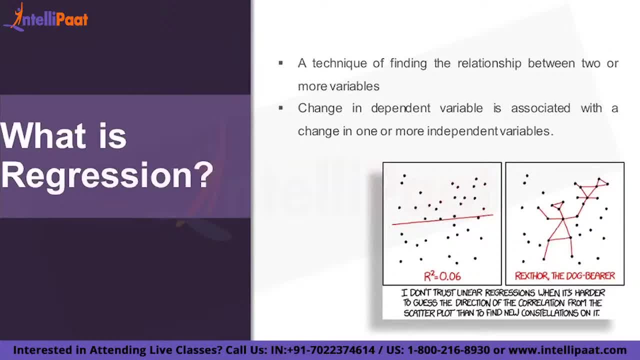 this theory is very important so that all of you will be able to get a very good conceptual understanding and then all of you know code. you can anyway, somehow you, you can practice. so that is the something right. so coming to what is regression. so regression is basically. 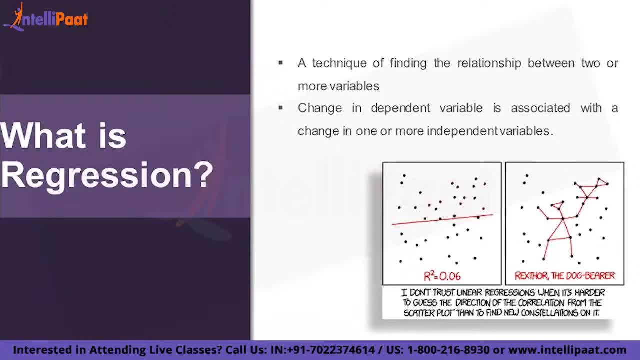 a technique Of Finding A relationship between two or more variables. right, so whenever you try to find a relationship between two or more variables, we call it as a regression. and what is this? linear regression is nothing, but some of you said change. independent variable is associated with the change in. 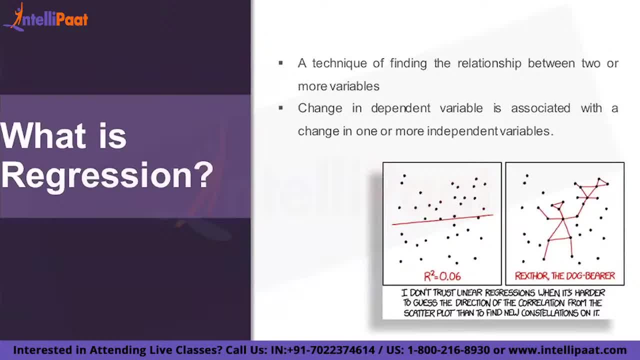 one or more independent variable. so what we are trying to do is, let us say I have multiple. I mean, let us have One independent Variable and one dependent variable. right, we will give examples also, but just now just understand this, so I'll give you some examples also. you have one dependent variable and one. 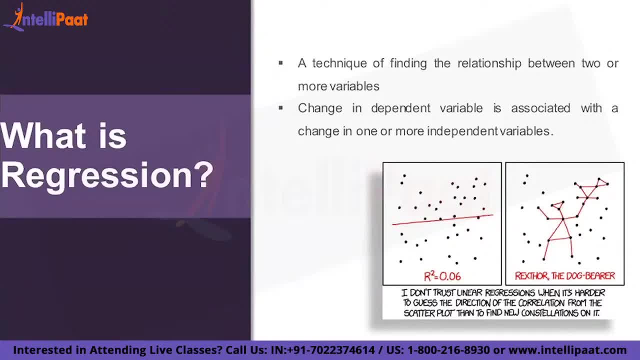 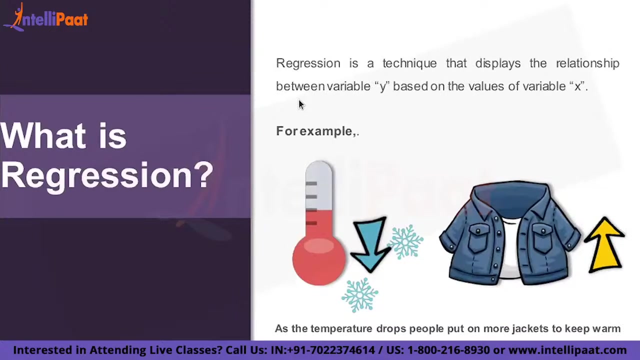 independent variable. now, what this linear regression does is: it will find a relationship between that dependent variable and independent variable, so how both of them are related. so that is something that we are going to check. So let me just Check. Take you to the next slide so you can see here. regression is a technique that displays 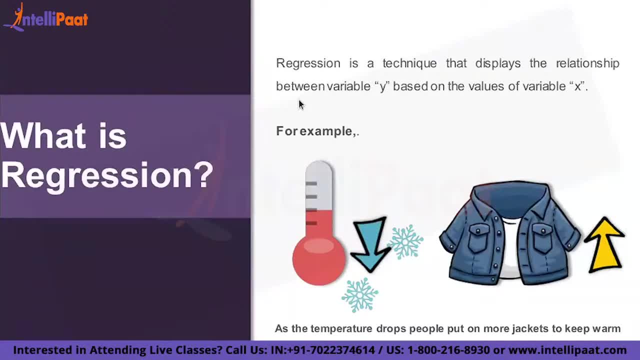 a relationship between X&Y, correct? so what is X, what is Y? based on these, it will give you a relationship. so when, whenever you have a variable X which is increasing or decreasing, you will have a variable Y somewhat related. so, as you can see in this example, as a temperature. 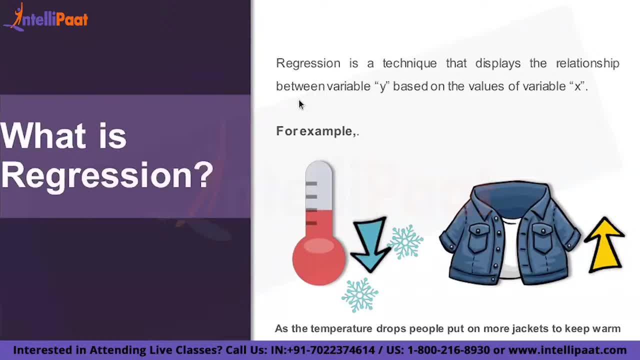 drops, Most people use more sweaters, so, which means this is a negative relationship, correct? when temperature keeps on reducing, the number of sweaters keeps on increasing. and when the number of sweaters keeps on increasing, I mean when the temperature keeps on increasing, the number of sweaters used by people keeps on decreasing. so this is one such example. 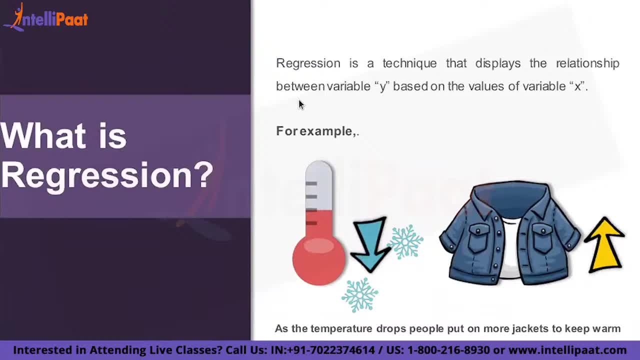 so now I'm just explaining it to you, How exactly Regression is being constructed. so what exactly is regression? so it is a technique to find out. I mean, don't worry about the definition that is written here, what I want to tell us. so linear regression is our technique, which gives you a mathematical relationship between: 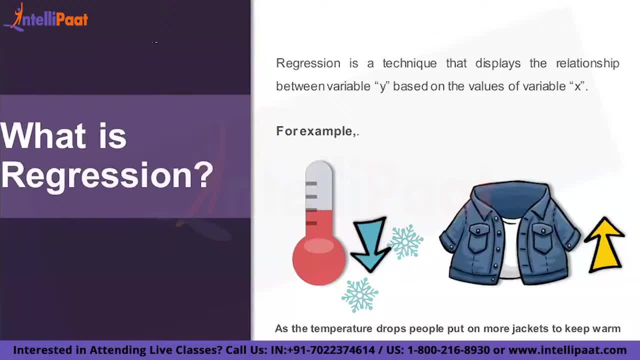 your dependent and independent variable right? so regression is a technique that gives you a mathematical relationship between your dependent and independent variable. is this clear to all of us? just simple basics I'm telling you now. we will go into a little detail. so some of the examples of 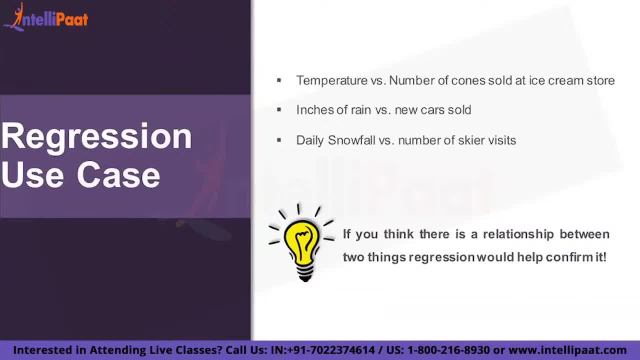 regression. so what are all the examples of regression we have? let us say temperature versus number of ice cream sold in a store. so let us say the temperature keeps on increasing, during summer season, more ice creams will be sold. if the temperature drops, the sales of ice creams will come down right. so that is the important thing. so with temperature, 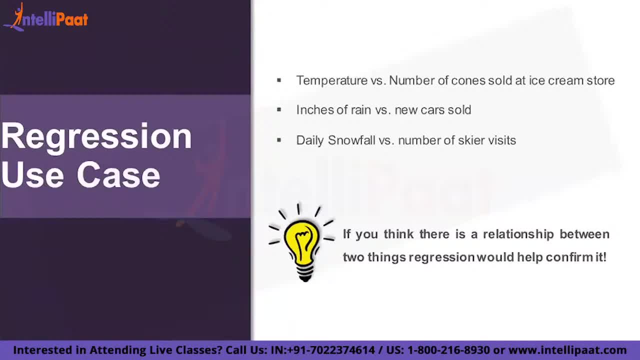 you will be able to see how many ice creams are sold or not. if temperature is increasing, sales will increase. if temperature is decreasing, sales will decrease. so that is a good example of positive relationship Regression. So when temperature increases, sales increases of ice cream. so it is a positive relation. 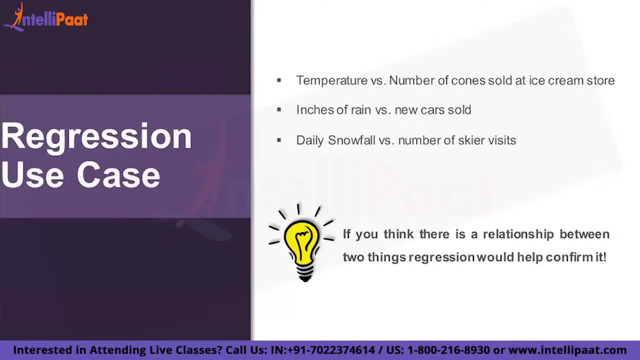 inches of rain versus new cars sold. so I don't know how rain and cars are related, but somehow they could be so. daily snowfall versus number of ski visitors, which means whenever there is more snowfall the people come to ski. ski means like they have this skiing board and 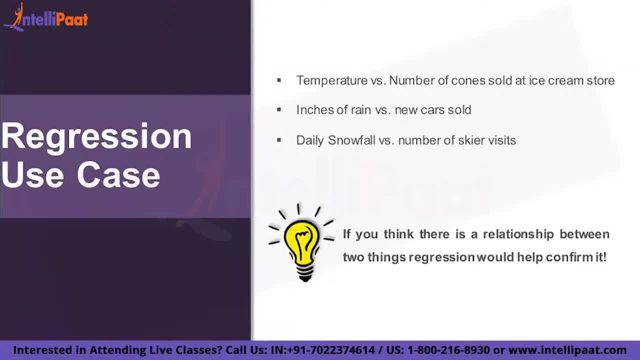 all that And then they use, they, they do the skiing on the snow. so as the snowfall increases, the number of ski visits also increases, correct? so now there is one thing that I will tell you: all of you know what is skiing, right? is there anyone who doesn't know what is skiing? 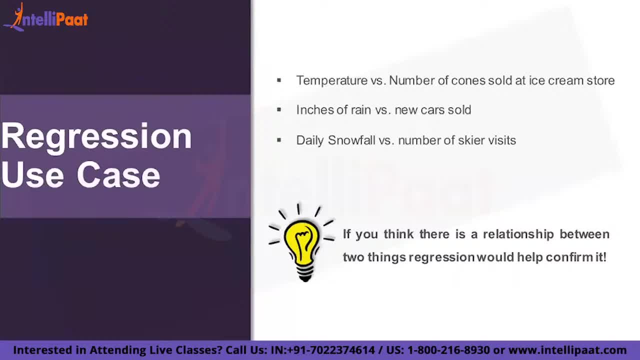 all of you know what is skiing right, yes, no, okay. so now there is one more one thing that you should understand. just keep this skiing example in mind. I will tell you in the future. there are some limitations of linear regression. I will tell you that, but keep this skiing example in mind till then. okay. so these are some of the examples. 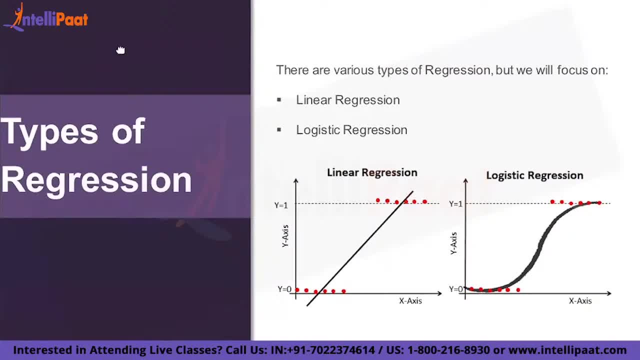 of linear regression. So now, what are all types of regression that we have? there are multiple types. there are so many types, but major ones are linear regression and logistic regression. so, basically, what is linear regression? What is logistic regression? We will see in few minutes. but whatever regression that we use, most of it is linear regression. 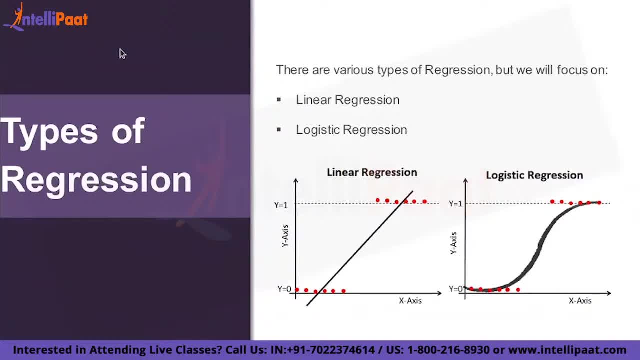 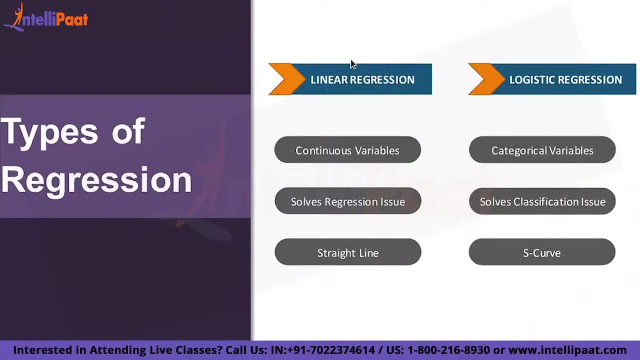 or logistic regression. so why do I need linear regression? why do I need logistic regression? all of that I will tell you now, right, so you can see here the basic difference between a linear regression and logistic regression is: a linear regression helps to solve the continuous variable data. 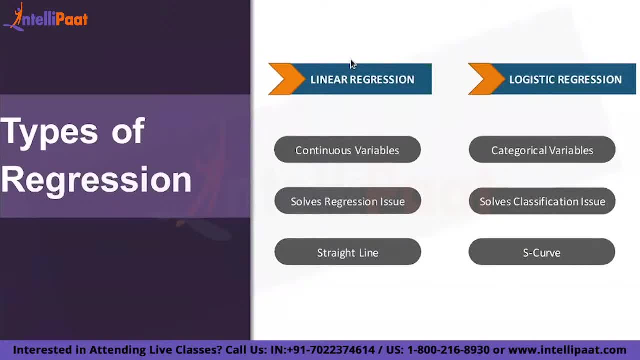 So whenever you have Independent variable and dependent variable, both of them should be continuous, correct? so you need to understand this. both the independent variable and the dependent variable, both of them should be continuous in the linear regression, whereas in logistic regression it can be a categorical variables. so anything, even though your target and other things also can be categorical- 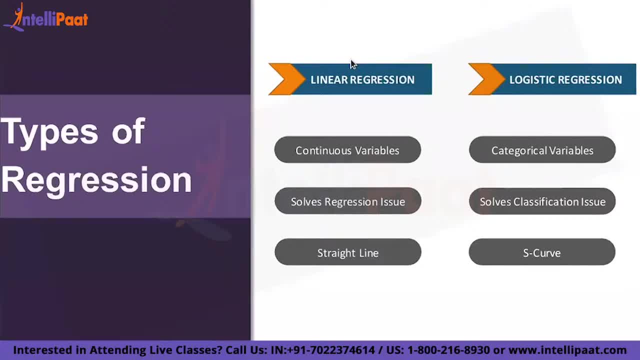 variables right. So basically linear regression. So basically linear regression, Linear regression and logistic regression. that is the first main important thing. next thing: it solves a regression issue. linear regression will solve a regression issue. so what do you mean by regression? I told you, regression is nothing but finding the mathematical. 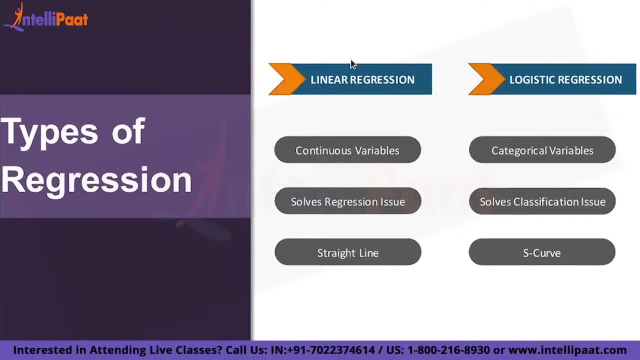 relationship between two variables. so that is regression. so by using linear regression, what you do is You find A Mathematical, Mathematical, Mathematical, Mathematical. What is a linear regression? You find the dynamic relationship between two variables using the linear line like a straight. 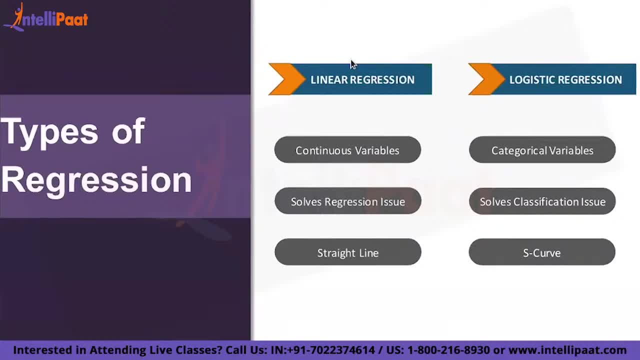 line relationship. so that is, you're linear regression, Logistic regression. what it does? what it does is it try to solve a classification problem. so basically, a classification problem means a zero or one. since it's a categorical variable, it tries to solve a classification issue. so in linear regression you have a straight line. 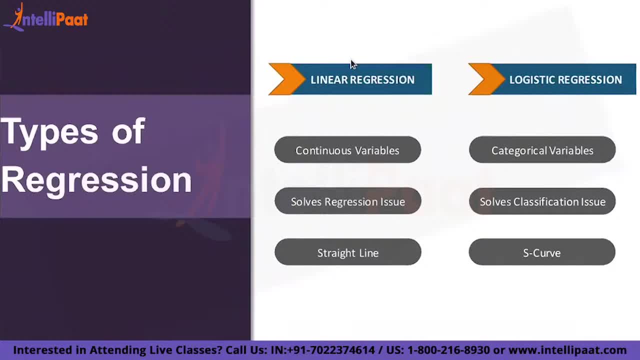 in the logistic regression you have a yes s curve, so we will see what is this s curve in logistic regression when we start with logistic regression. but linear regression is a straight line, so which we are already seeing. so this is the basic difference between linear and logistic regression. okay, fine, so basically, in this particular 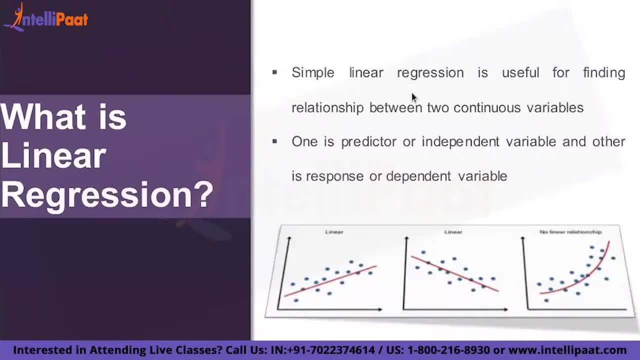 session. what we are talking is linear regression, simple linear regression, where we are trying to find out a mathematical relationship between two continuous variables. so in the two continuous variables, one is an independent variable and another is a dependent variable. so basically we have two types: one is independent and one is a dependent. so let us say, for example, in our 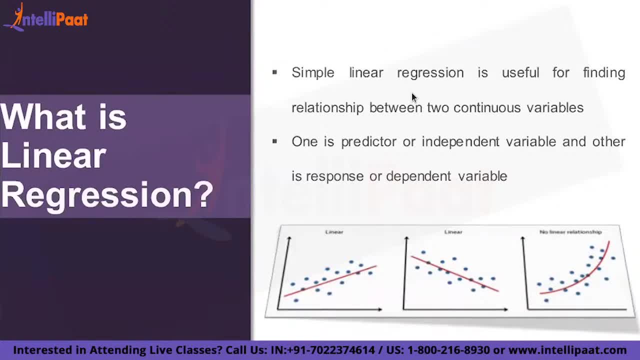 temperature and sales of ice creams which was independent and which was dependent. can you tell me temperature and sales of ice cream, which was independent and which was dependent? can you tell me temperature and sales of ice cream sales is dependent, exactly, temperature is independent, correct, true? so now why? it is because 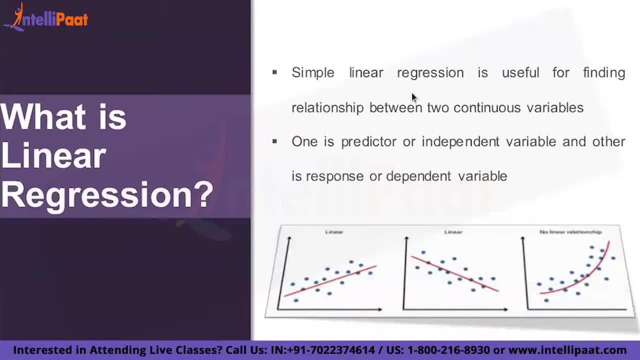 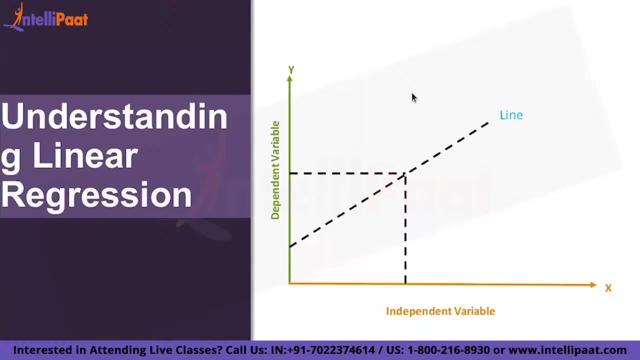 see if you always, if you can remember, sales is dependent on temperature. temperature is not dependent on sales, correct? so sales is a dependent variable, exactly. so what you said is right. so here also in our example, we are going to see this how it works and then we will see. so there are few. 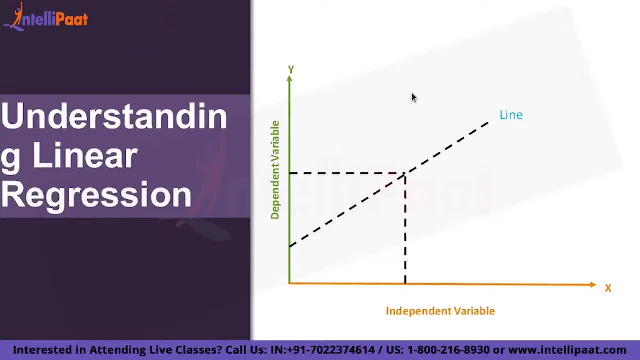 things for you to understand in linear regression before going into the depth of it. so we will, we will. i will also tell you a basic math, not a very high-end math, but a basic mathematics that is required for this thing. right, so you can see. you have a x and you have a y. x is your independent variable, y is: 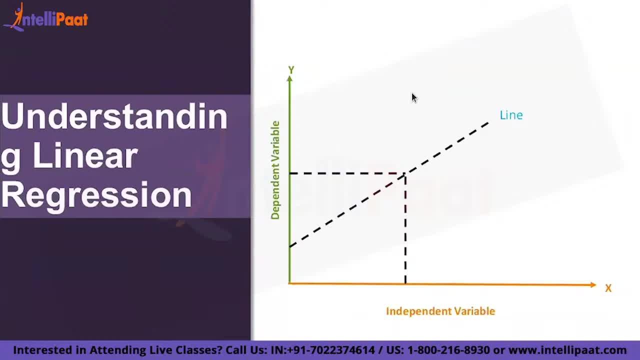 your dependent variable. and then you have drawn a line that looks like that. whatever line you have, that is not a final line, but a some line, so you have to put some line. so when you put one line, wherever the line is there, if you want to measure what is the value of x and y at any given point in time, you can draw a horizontal line and a. 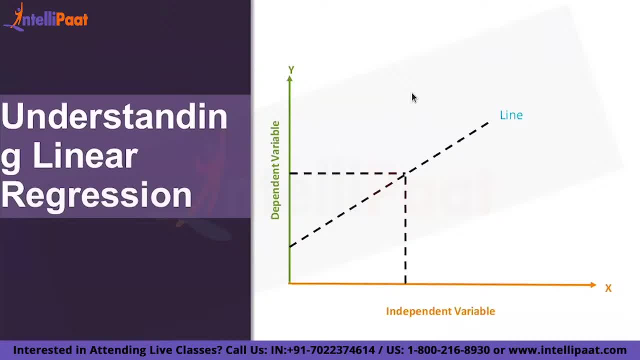 vertical line to find out the values of x and y for a given point in the line. is this clear to all of you? so what i am trying to tell you is: you have x-axis, y-axis, and then you have a line, correct? So if you want to find what is the value of x and y here, how do you find? 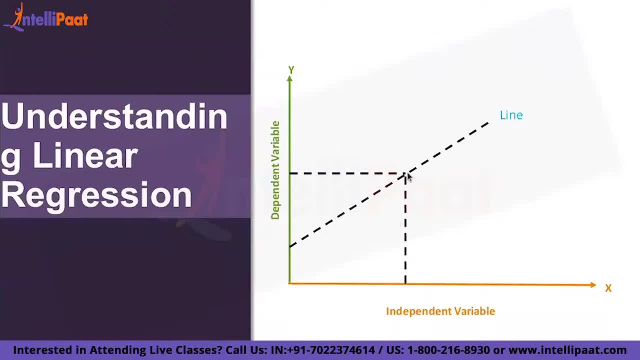 You will draw one line here and you will draw one line here. So this is the value of x here, This is the value of y here. Similarly, if you want the value of x and y here, what you will do? You will draw a line here. find the value of x. 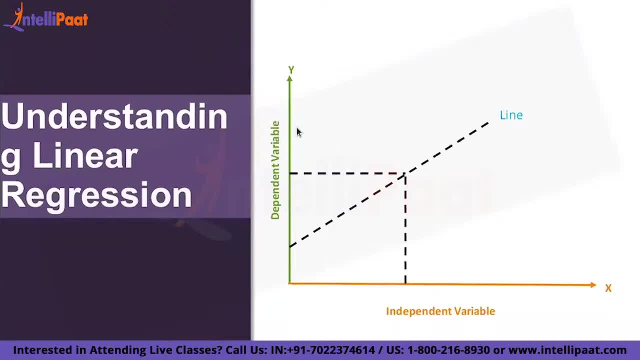 You will draw one more line here and find the value of y Clear. So now we will do one thing You can see. So this is something that I am just trying to tell you. These are the basic understanding of linear regression. So whenever you are going to do this, you can see. a basic linear regression is nothing. 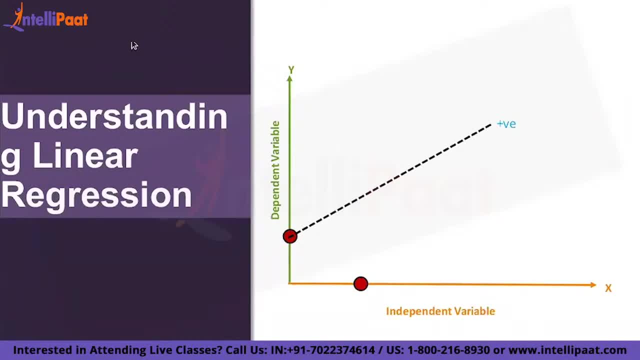 but they have just given you a positive line, So nothing much in this. So you have an independent variable, You have a dependent variable, You have a positive line, which means with increasing independent variable, dependent variable also increases. Clear Now. having said this, let us go to the next one. 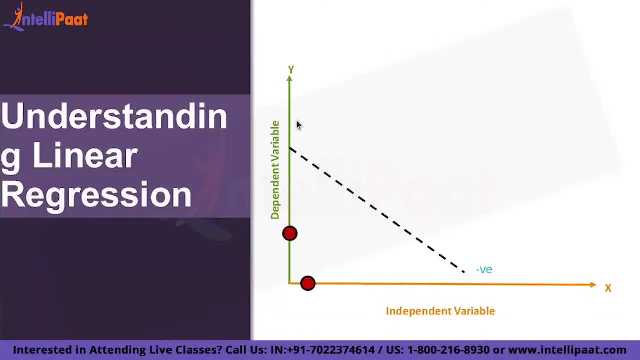 So this is a negative one. So this you saw positive and this is a negative. So when your independent variable increasing the y is decreasing, which means when the temperature is increasing, the number of sweaters will decrease. Correct Agree: Temperature increases means it will become summer. 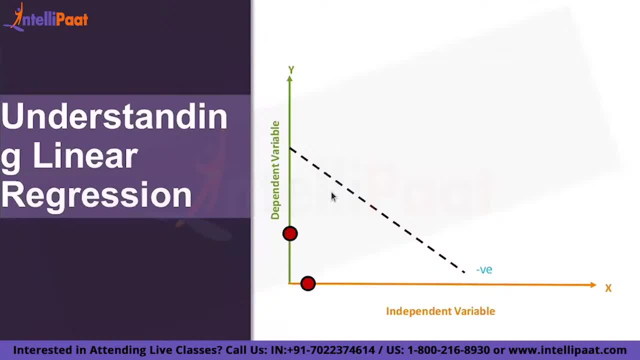 So in summer no one wears sweaters. So that is your negative relationship. So positive relationship, negative relationship. You understood This is just a simple line. Now, whatever line you are seeing, that we can also call it, That's line of linear regression, because linear regression is a straight line. 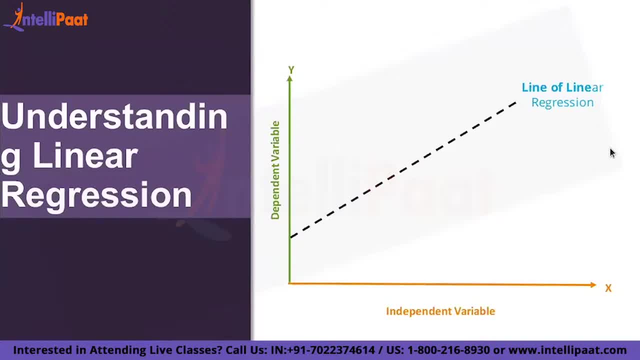 So some of you said y is equal to mx plus c. So y is equal to mx plus c, is the equation of a straight line. So whatever line you are seeing here, we can call it also as a line of regression, line of linear regression. 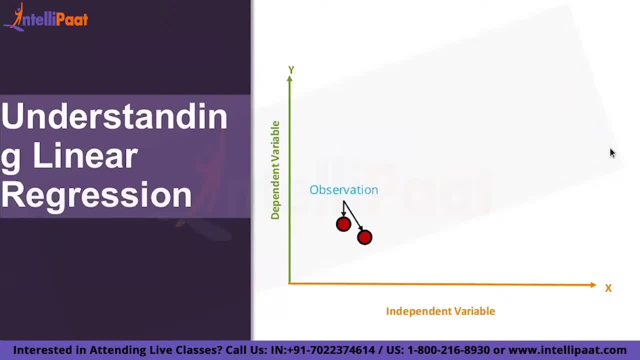 So this is something that we can use. Fine, Now you have data points, So data points are called as observations. Clear, So you understood what is I will. I will, before going to the next steps, we will recap and then we will see. 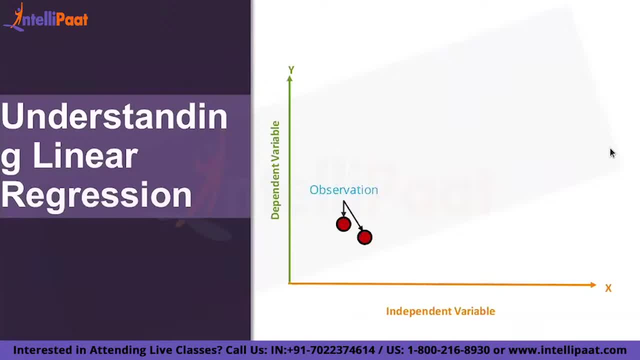 what are all this? Now, before going into the next slide, I will tell you a few slides. Just check this. So what we saw is independent variable, dependent variable and a line. So if you want to find any point in the line, you either draw a horizontal axis or a vertical. 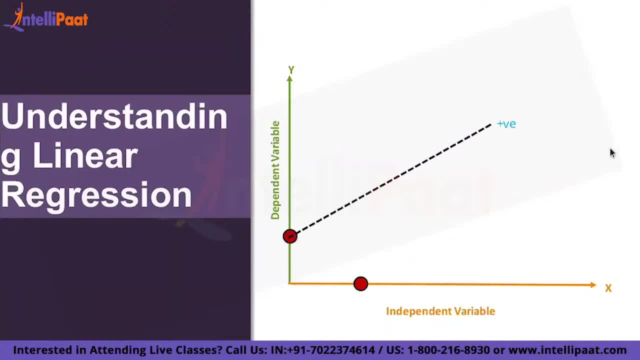 line and then find the value of x and y. So this is line. Then you have a positive relationship line, negative relationship line. This line is also called as a line, Line of linear regression, And then any dots that are there in the graph are called observations. 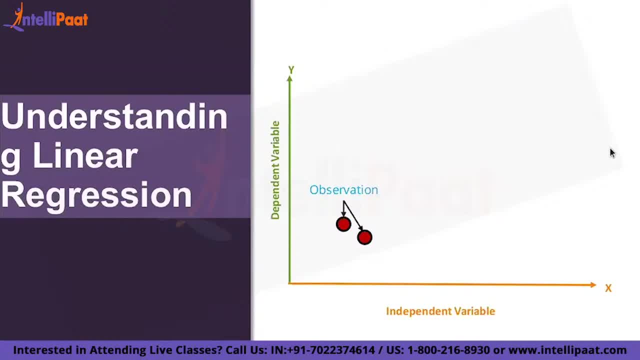 Is it clear to all of you till here. So this is your observation. So these are some of the basic things that you should understand whenever we are going to do a linear regression. So these are just data points to observations. I put just normal data points, nothing much. 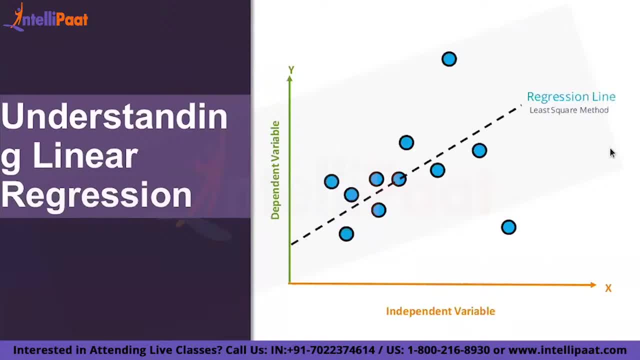 So we call them as observations. Now, whenever you go to a linear regression, You have something called as a least square method. So what do you mean by a least square method? is you're going to reduce your errors? How are we going to do that? 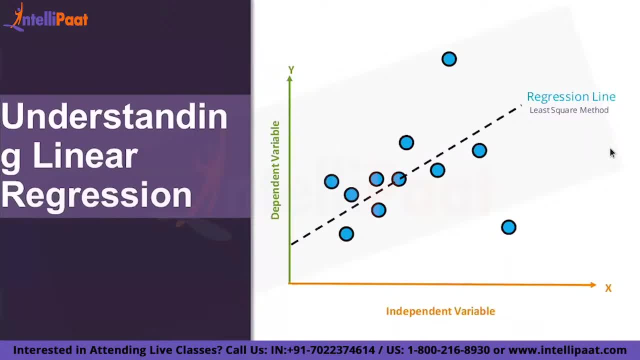 We will check it. And now for our understanding, x is an independent variable, Y is a dependent variable. And then I have multiple dots here, which are the dots that I will be using for my observations. So they are my observations. And then the 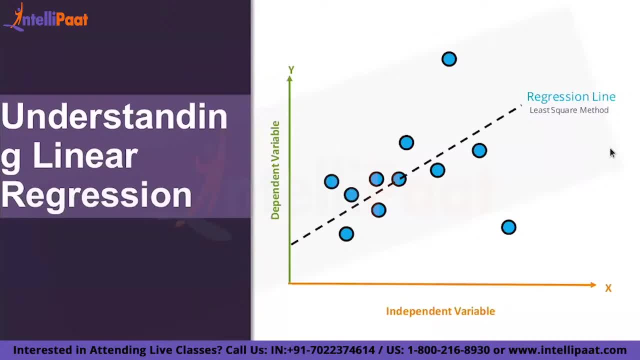 Line of linear regression line is the least square method whatever we have used by reducing errors. That is the line that represents the relationship between x and y. How we are going to do it, all of that we will see. So, basically, this line, all the points will be around this line. 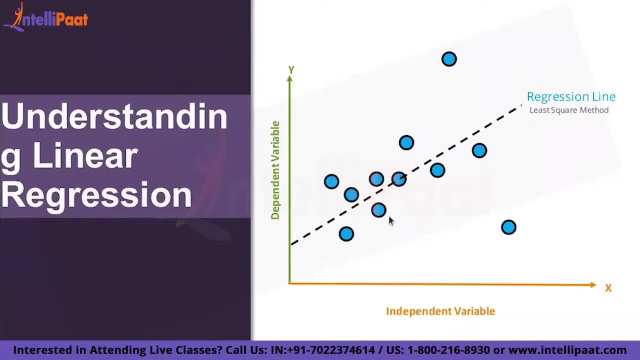 So this gives us a fair, good estimation about the data points. Is this clear? how we are going to get it, We will see, But this is how it looks clear now. What we are going to do is observe this carefully from this line. 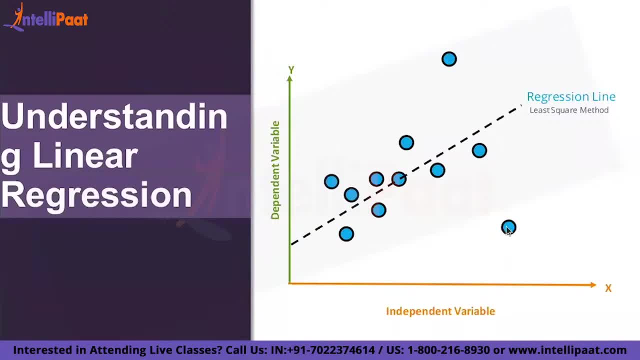 I'm considering two points. One is this point and one is this point. Now, according to your linear regression line, it will not be a straight line. So it will not be a straight line. So that is why we are not connecting the dots. 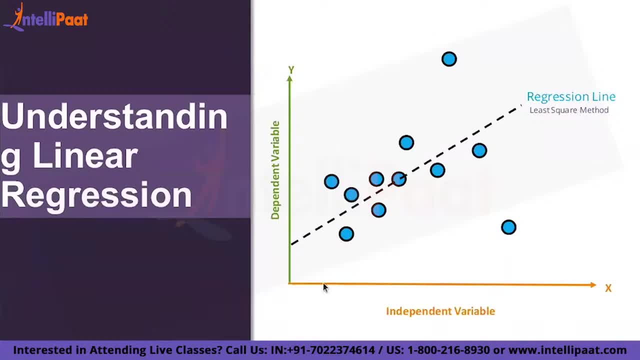 So, according to linear regression, if my x is this, my y should be here, Correct, But my y is here. If my x is this, My y should be here, but my y is here because it is giving you an estimate. 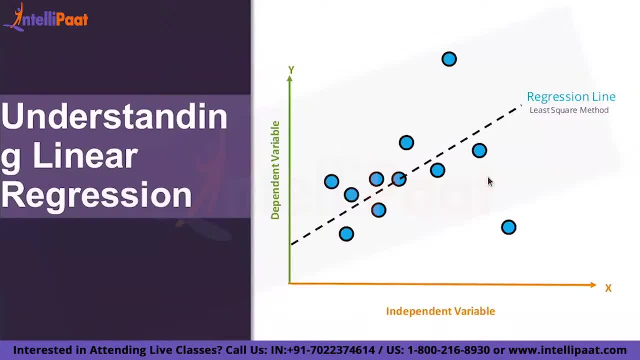 It is not exactly telling you. Similarly, consider this point and this point: If my x is this, according to the linear regression line, the value of y should be this: Same here. If my x was here, the value of y should be here, not here. 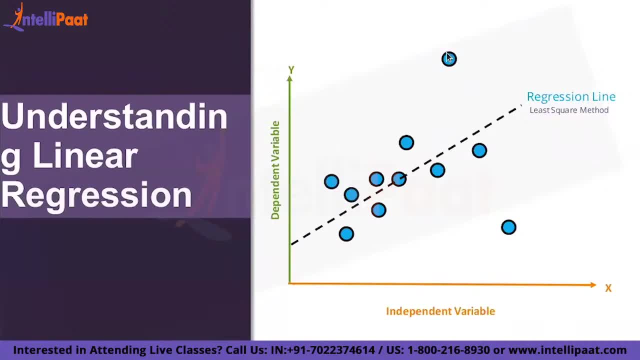 So you're getting these things, What I told you just now, Nice. So now, if you have these things like this, What happens is you can see whenever you have an estimated value, there will be a difference between your estimated value on the linear regression line and also the actual value that you are seeing in the linear regression line. 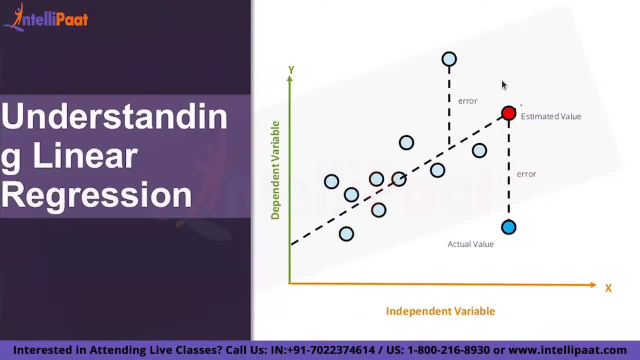 So there will be a slight difference between your estimated value and also the actual value in the linear regression line. So this thing is what We call it as the error: You are estimating something in the linear regression line, but in reality the data point is somewhere else. 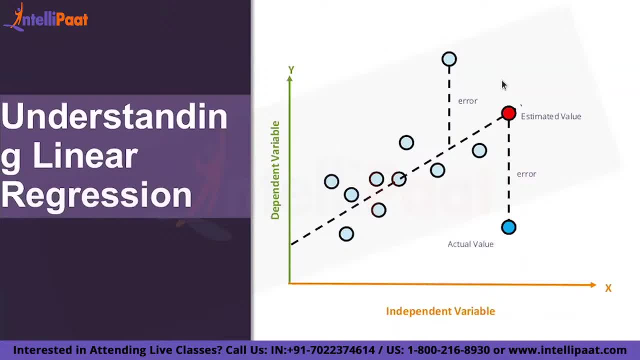 So this is what we call as the error term, Is it fine to all of you? Understood Here? there are no outliers. So what is your estimated value and what is your error? So this is very simple. I'm telling you very, very simple terms. 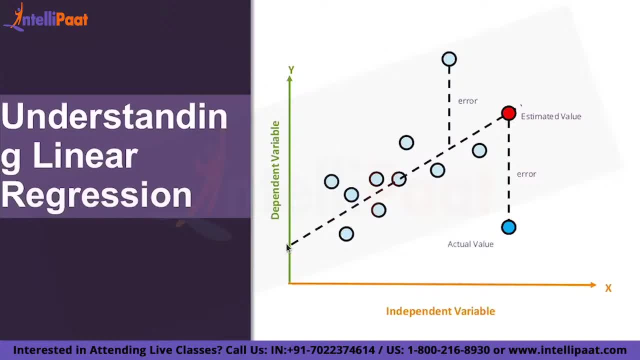 I'm not using any complex words here. Right, So you're having a linear regression line for estimating your data points, But what happens is- this is the one that I'm keeping my mouse pointer. This is a good estimate. where the estimate lies on the line. 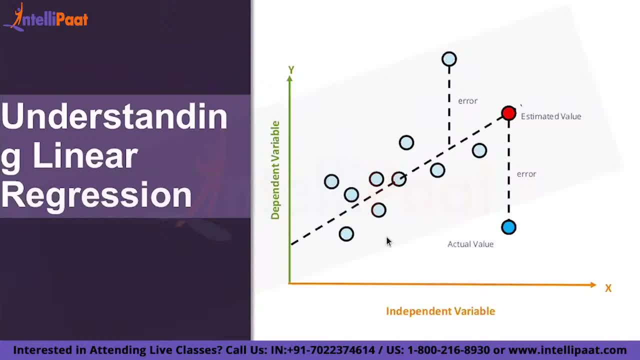 But all others are either a little up or a little down, which means there is a small error between every data point and the line. So this is your estimated value, This is your actual value And this is the error term Correct Understood. 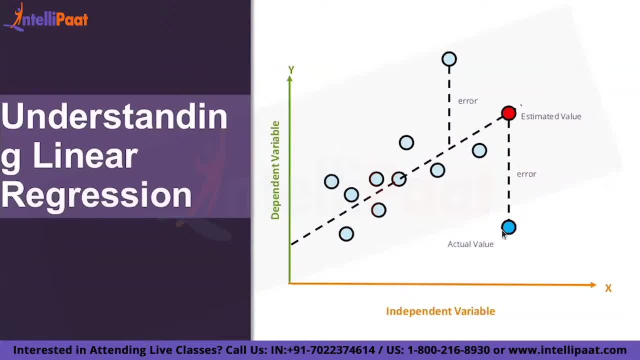 So what? So, whatever is your estimated value, the difference between your estimated value and actual value is the error term, Clear. So these light blue dots are the estimates. actually, I mean not the estimates, but the observations. The blue dots are observations. 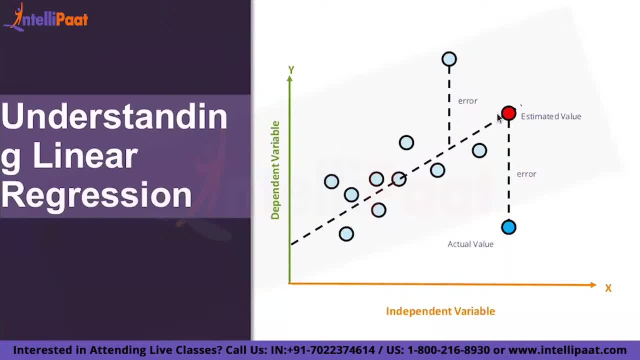 This line is the estimate line. All of you are clear about these things, what we discussed Right Now, let me go to the next. So similarly, just like how we have error For these two, you can have errors for all data points. 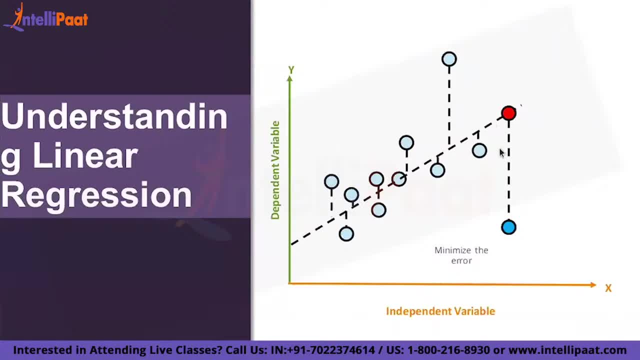 Correct, Agree. So just like how you have estimate, you're finding the difference between your estimated value and the actual value, So you have an error term. Similarly, you can find error for all the observations from your estimated line: Correct, So this is one estimated. 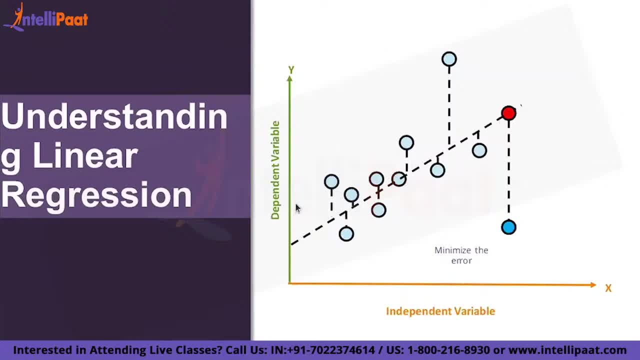 Line that you have given similar to this estimated line. You can draw a few more lines like this, like this, like this: There is no standard rule, right? So this is the estimated line. There's no standard. This is one of the estimated line. 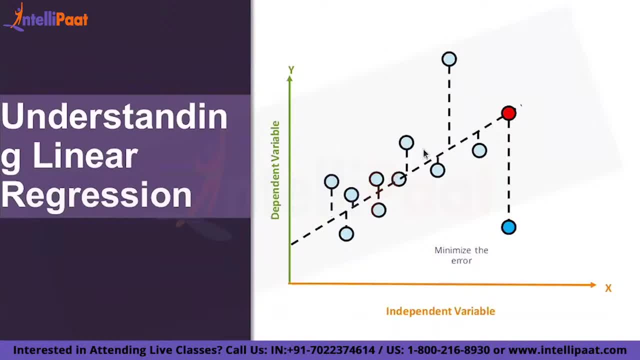 So with every estimated line you can find out the error terms for every observation. Correct, Python. Don't worry Python, We will look at it tomorrow. Now we are talking about linear equation. We should not buy any chance, You do. 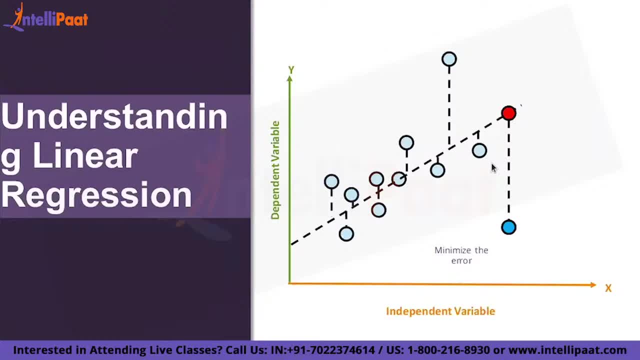 You join late. Okay, That's the reason. So I've explained all of that in the beginning, No issues. So please try to be on time so that it will be helpful, Right? So these are observations. whatever we have, Our objective is to find out an estimator line which is a very fair estimator of all these observations. 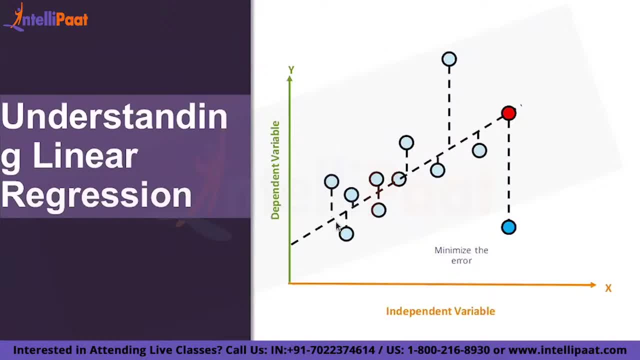 So I can draw multiple lines, I can draw hundreds, I can draw a thousand lines here, a thousand lines here, but my objective is to find out the line that will best fit all these data points. So whatever one line that I have drawn, with that I can get some error terms. 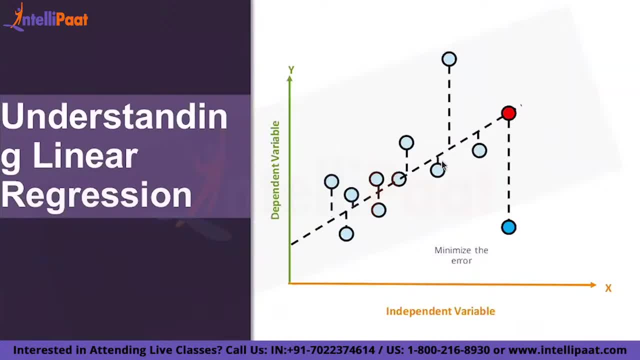 So let us say, I will draw one more line like this, for that line Also I will get some error terms. So let us say, I'll draw one more line like this, for that Also I'll get some error terms. Correct. 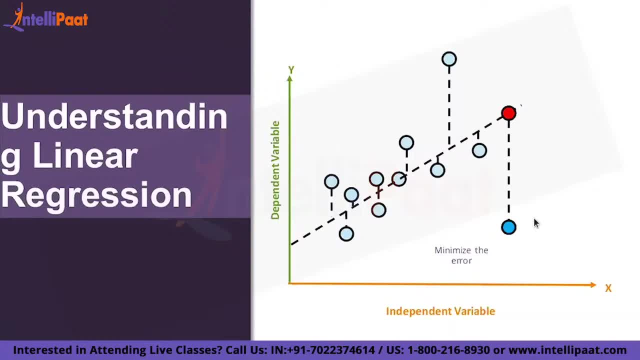 So now the only thing, The only thing that I'm telling you is: for every estimated line, you will get errors from all the data points. Correct, All of you agree. This is one estimator line. You have found out errors for all the terms. 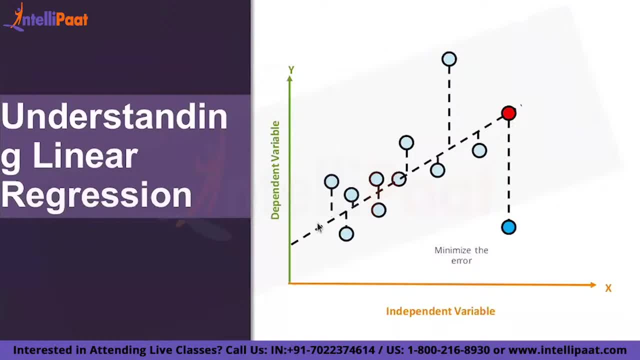 Now, if I have multiple estimator lines, I can have errors for all of them. Correct: Every estimator line will get an error. There is no estimator line that will give you zero error. Correct, All of you agree with me Because it's a straight line. 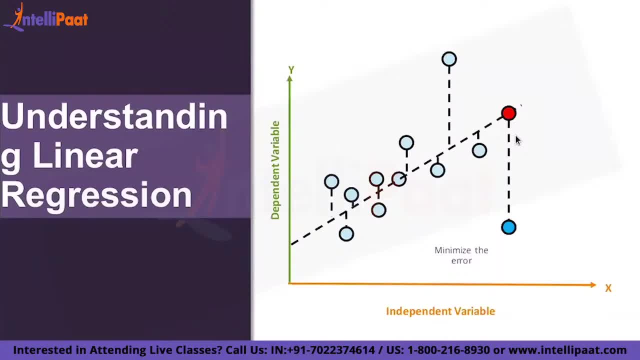 Now, just one line I will tell you, and that is your linear regression. Out of that 100 estimator lines which are giving different types of errors, the linear regression line is one which will give you the least error. Got it? That is as simple as that. 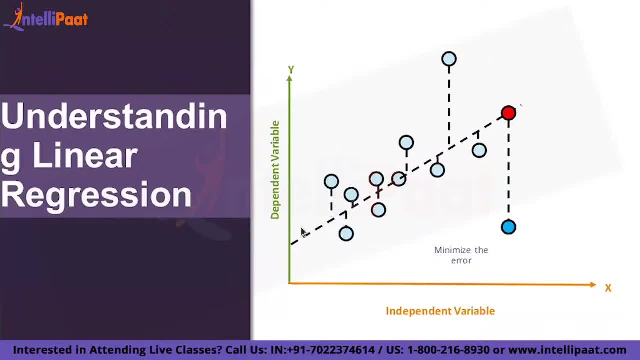 So our objective is to find out a straight line Correct. Linear means it is a straight True Least error for all values Correct. So I have my independent variable and dependent variable Based on the value of independent variable and dependent variable, I have multiple observations. 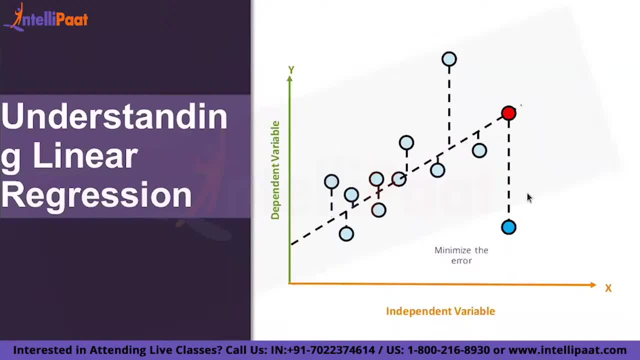 Now my duty is to find out a straight line relationship for all these dots, Because we are doing linear regression. Linear regression means straight line. So how am I going to find out That straight line relationship? by drawing multiple lines, So I don't know which is the correct line. 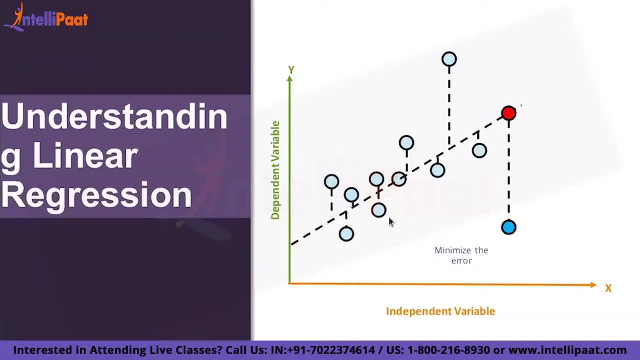 So I will draw 100 lines and I will find out the error for every line. What is my estimated value? What is the actual value? What is my estimated value? What is the actual value? Like that, I will find the error for all the 100 lines. 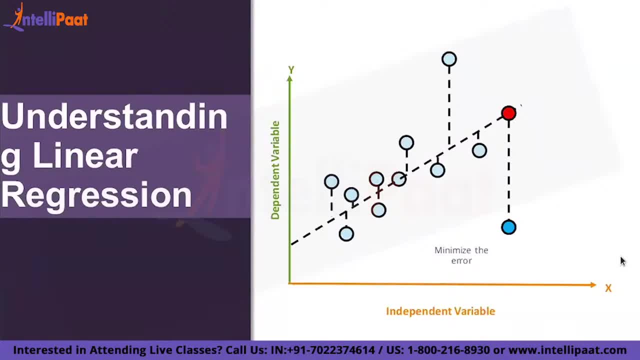 The best line that will fit is that line which gives me least error. That is all. Clear, Agree Clear to all of you. So now, if this concept is clear, the further Gurvinder. no means it is not clear, or no questions. 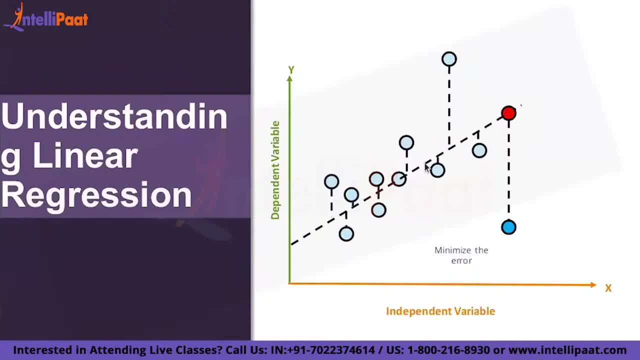 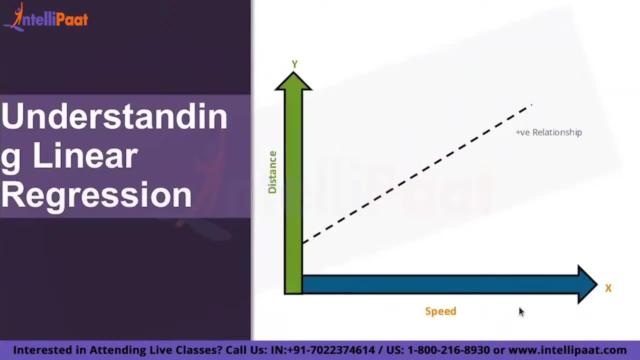 Okay, So this is how you are able to get the best estimate line. So how are we going to do that? I will show you. You can see now you have speed and also the distance, So both of them are having a positive relationship. 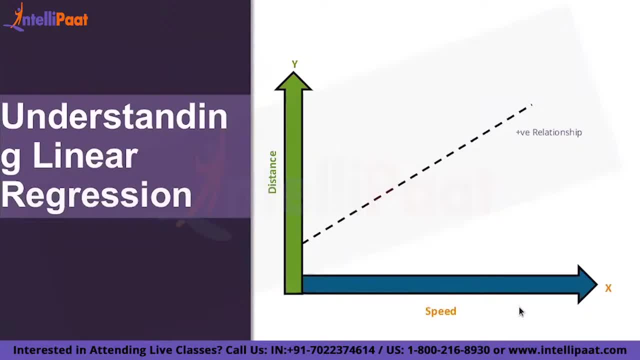 Right. So this is having a positive relationship. So if you go with more speed, you will go longer distance. So that is the general thing all of us know. So if I go faster, I will be able to cover more distance. So that is one thing. 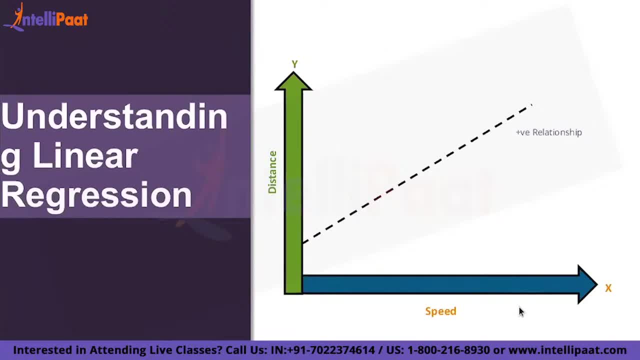 Now let us say I will travel at 1 km per hour. Okay, My speed is 1 km per hour, I will go how much distance in? let's say, 1 hour, So 1 km. If I travel at 5 km per hour speed, I will travel 5 km. 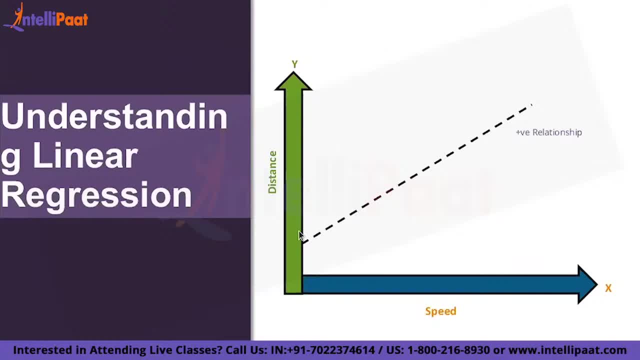 If I travel at 100 km per hour, you will go 100 km. So basically this is a straight line linear relationship: The more speed that you go, the more distance that you travel. There is no issue in this, Correct. 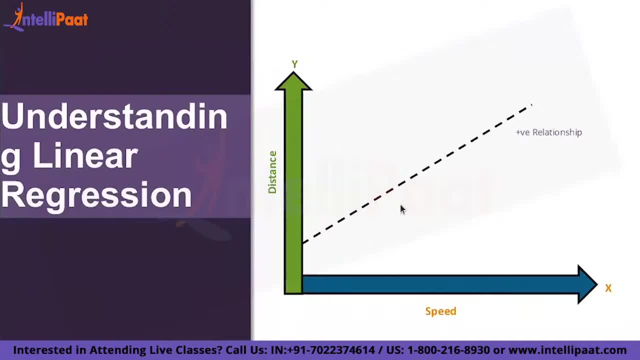 Now what happens is, whenever you have this X and Y, the distance traveled in a duration of time is your Y. Understand these variables. The distance is your dependent variable, because distance depends on speed. Speed is not dependent on distance, Right. 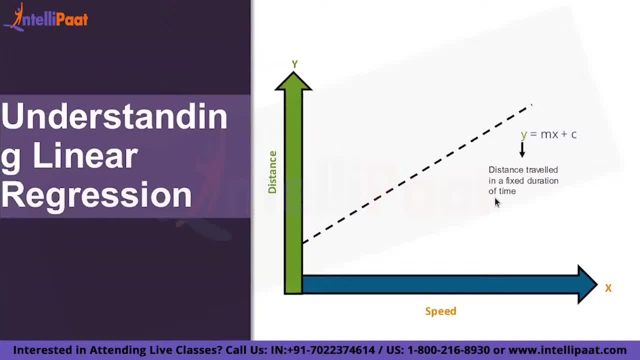 So the distance depends on speed and speed is not dependent on distance. Now, having said this, the straight line relationship, all of you know it is: Y is equal to M, M, X plus C. But what is Y? What is X? 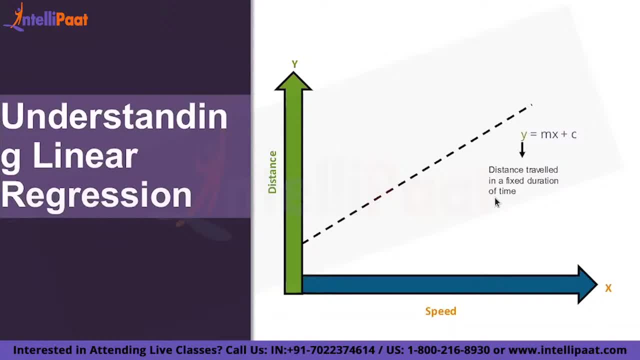 What is C? And all of that we will see. There are two terms here which you already know. One is Y and one is your X. X is speed, Y is distance. Clear Till here To everyone What is M. 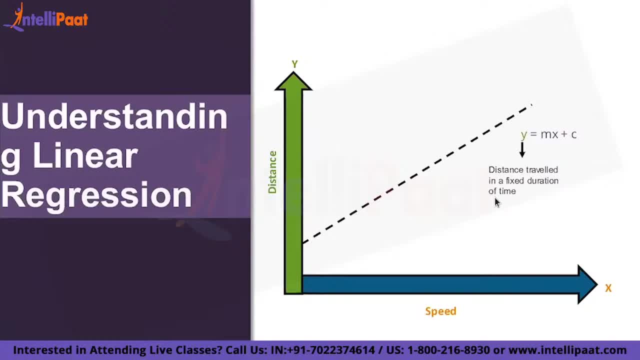 What is C? We will see Now. let us say, for example: X is the speed of vehicle, Y is distance, X is speed. So you saw that Now M is nothing but The slope. So what do you mean by slope? 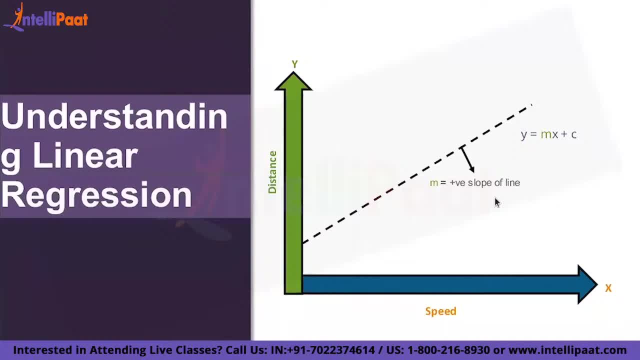 Slope means delta Y by delta X. So that is the formula, Which means you take a small piece. Delta Y by delta X is the formula, But for us, as of now, let us understand whether it is a positive or negative. 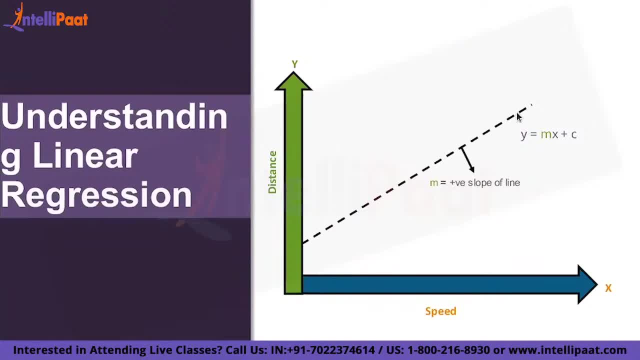 Right, Positive or negative? As of now, the slope is positive, Which means there is a positive relationship, So that one we will keep in mind Next, No, no, no. The slope, how you calculate, is: you take a small piece of X here. 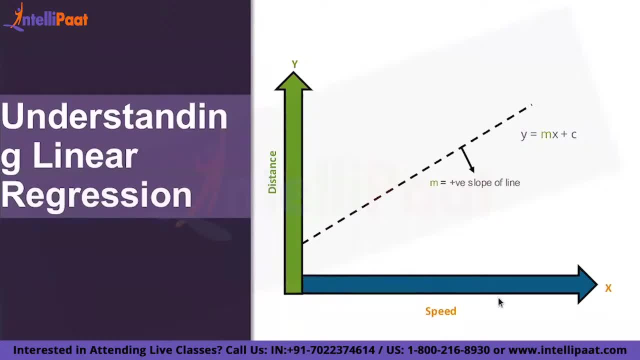 You take a small piece of Y here, You take a small piece of X here. Correspondingly, It comes like a triangle. So this difference of Y and this difference of X is the slope Which we are not using here. Correct DY by DX. 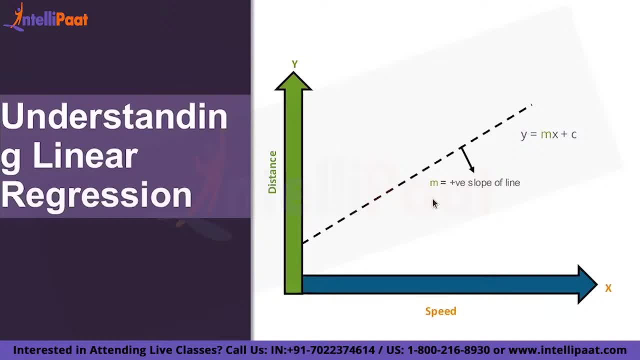 So, which is not required right now, I will tell you. See, assuming that all of us are new, I am just telling you Right now, Right, Right. So we will just go ahead and then see how it works. Now you understood what is Y, what is X, M is the slope. 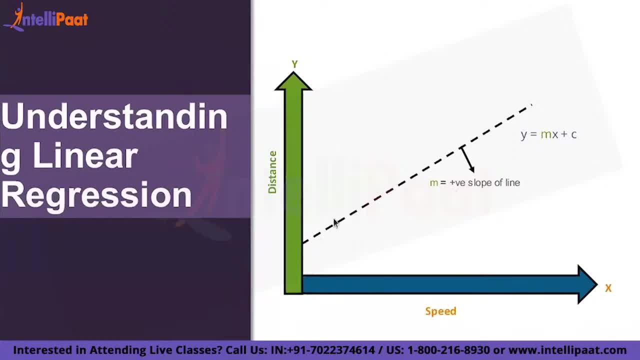 Positive means it is going upwards, Correct. So now M is a positive slope. What is C? So C is nothing but the value of Y when your X is zero. C is the value of Y when your X is zero, which we call it. 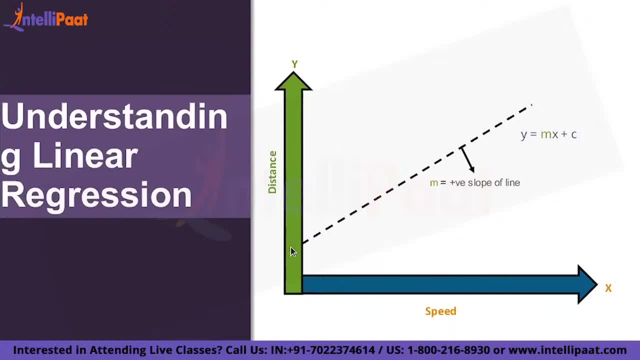 We call it as an intercept, which means, when my X becomes zero, what is the value of Y? So you would have seen right. So whenever there is, let us say, for example, I will give you one example of marketing camp. 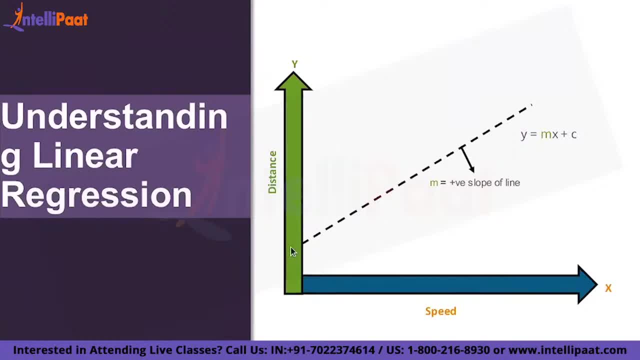 marketing budget and the sales. So if marketing budget is your X and then C is a constant variable, Correct, So it's a constant. So marketing budget is X And sales is Y. Assume that in one particular year the company doesn't give any marketing budget. 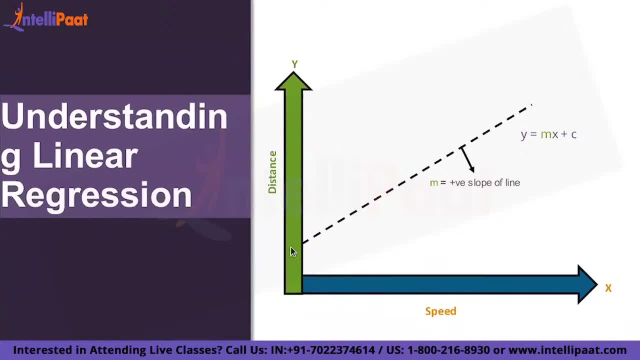 They keep their marketing budget as zero. Do you think there will be no sales at all? if marketing budget is zero, Do you think there will be no sales at all? There will be some sales. I'll tell you, I'll give you some good examples so we can all connect. 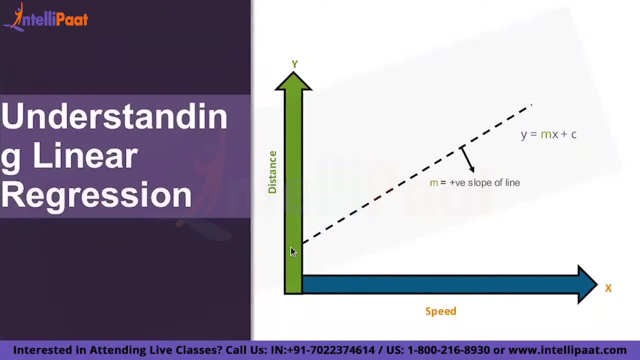 Right, Based on previous marketing spend is one thing, But even though if it's not based Based on previous marketing spend also, there will be some sales. Let us say, for example, there will be. OK, fine, I'll ask you one question. 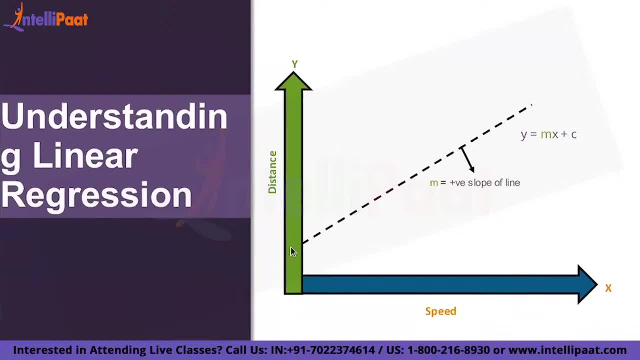 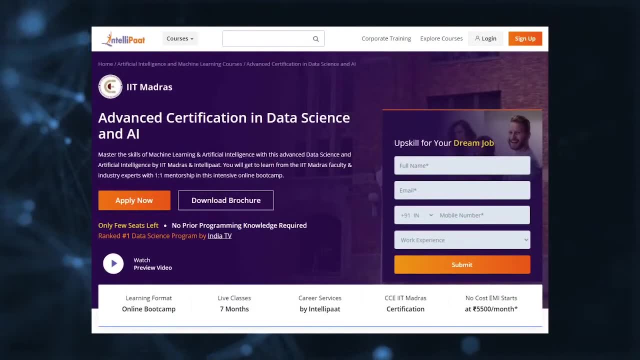 How many of you are seeing petrol advertisements these days? Anyone seeing petrol advertisements? If you want to make a career in data science, then Intellipaat has IIT Madras Advanced Data Science and AI Certification program. This course is of very high quality and cost effective. 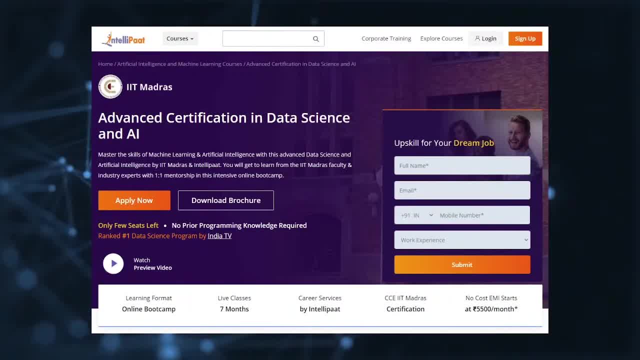 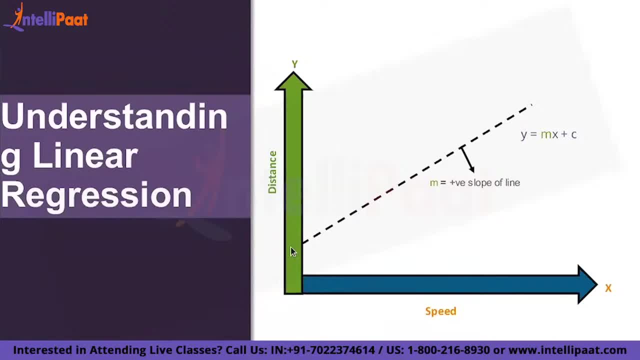 As it is taught. This course is taught by IIT professors and industry experts. Indian oil, HP, Bharat Petroleum. Do you think there are no sales? Every day, everyone will buy petrol. no, That is a necessity, Correct? Forget about that. 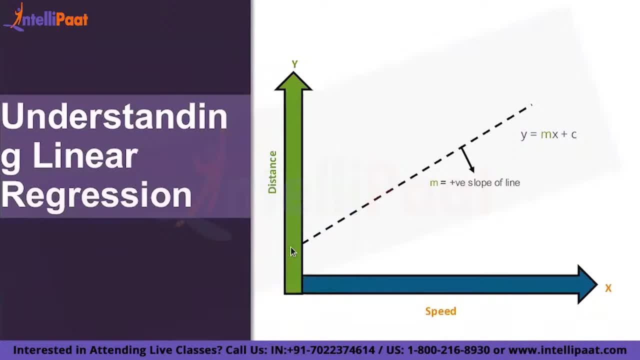 How many of you remember seeing ad of a notebook or a pen or a pencil in the last three months? They used to come Correct. Have you seen any advertisement of a pen Or a pencil in the last three months? No, right. 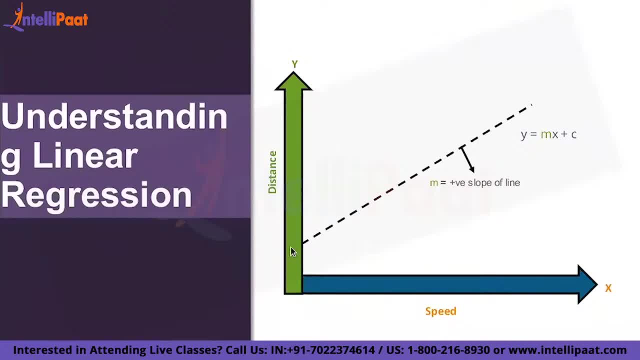 OK, I'll give you one very good example, Very good example of marketing. Have you seen ad of Lux soap in the last three months? Where did it go? Everyone used to come. No, none of you would have seen. But soap sales are there. 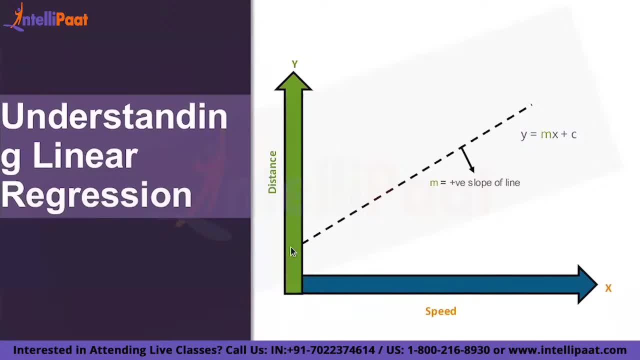 You go and ask in the shop, He will give you Lux soap After COVID coming. only Lifebuoy and DataLads are coming. Correct, Lux soap, Lifebuoy, DataLads, Lysol, Savlon, 4 ads are coming. very much anyway. 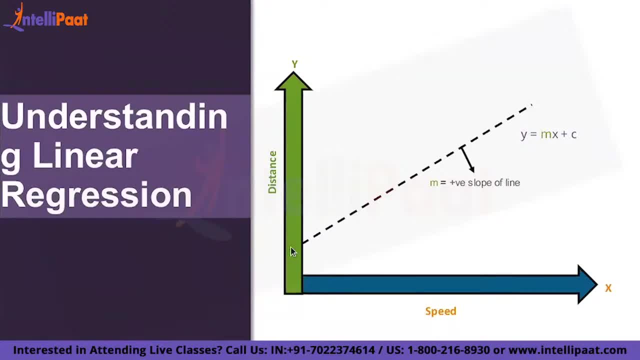 So this is an example of C. Why I am telling you this is remember this properly, right? Yeah, So C is correct: Lux, Lifebuoy, Lysol. so just remember this and you can see, even though there is no marketing. 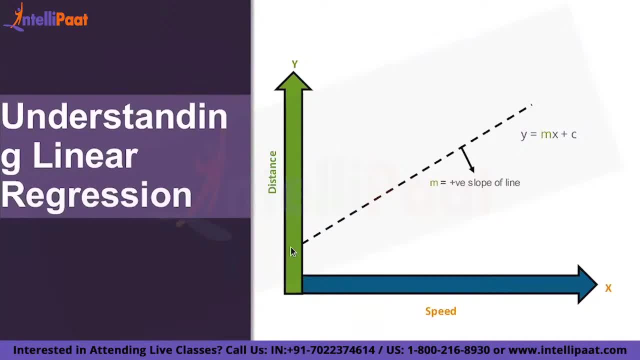 that is happening. there will be some sales. So that is your C, Which is your Y intercept. with zero marketing budget, you will be getting at least some sales. So that is your intercept. Now, here, that thing doesn't work because if you are traveling at zero kilometers per hour, 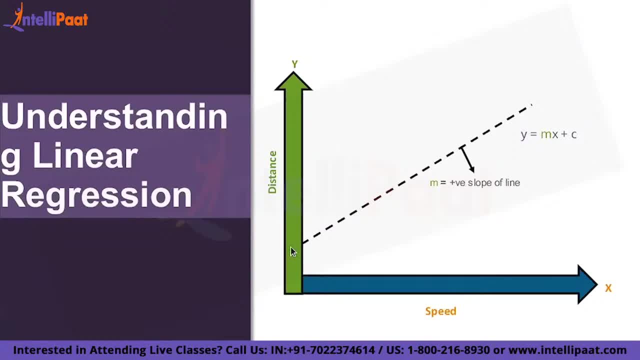 you will be at zero only, So the speed and distance thing doesn't come. So I just took an example of marketing budget. So this is a simple example. Y is equal to MX plus C. So now all the items in Y is equal to MX plus C. are you comfortable? 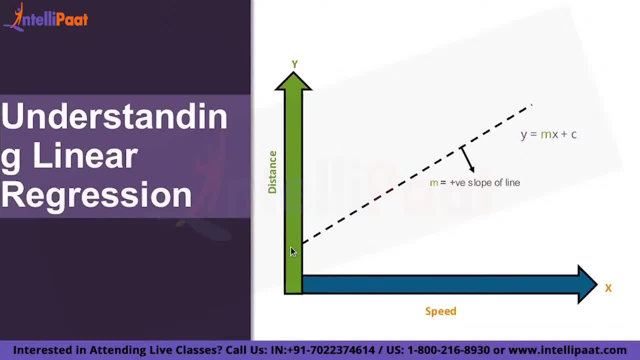 Did you understand This thing? also? I will upload it to your LMS, Just check. and then I will also upload all the codes and all of that so that you can use them. So don't worry, I will give you all the material. 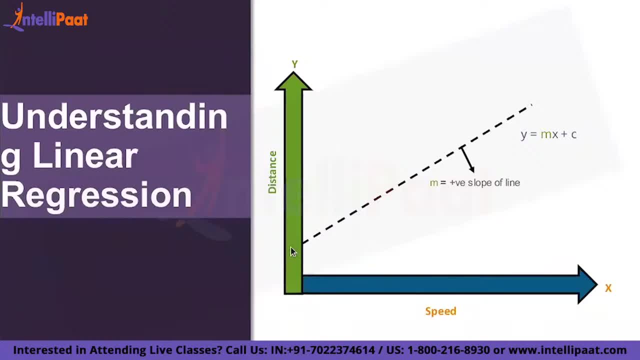 So if the line goes down, it's negative score. Yeah, Sanjay, basically, if the speed increases, the distance traveled by you also increases. Yeah, Yeah, Yeah, Yeah, Yeah. Here it's a positive slope, M is positive. 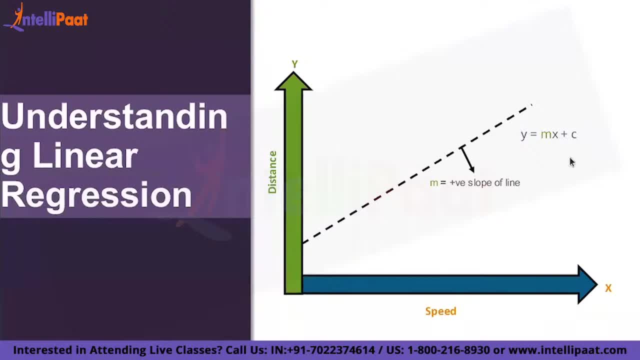 So Y is distance, X is speed, C is nothing. but when your X axis is zero, what is the value of Y axis? So that is why we took example of a marketing method, Right, So this is something that we will go. 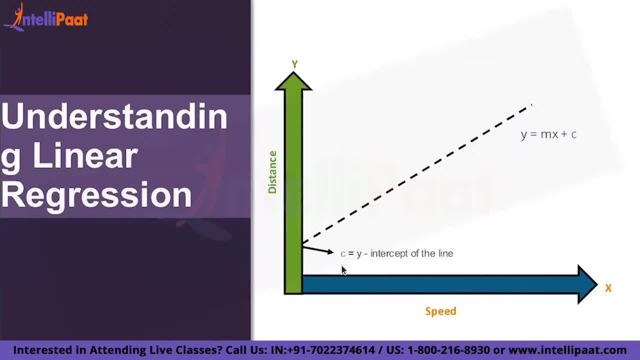 Let us go to the next one. So this I already told you: C is equal to Y intercept line, So C is equal to Y when X is zero. So zero into X is zero, so zero into m is zero, so y will be equal to c. so this is so negative slope is nothing but. 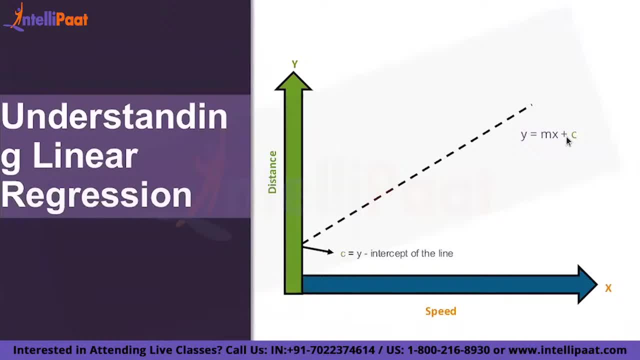 we can just say: yeah, ice cream versus temperature. no, not ice cream versus temperature, sweater versus temperature. so ice cream will increase. so sweater versus temperature, number of sweaters versus temperature, is negative. as temperature increases, the sweater sales will decrease. so that is negative. you can see this is negative. y is equal to minus mx plus c. 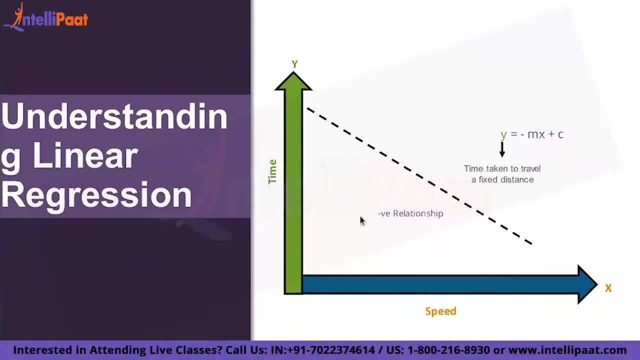 so, which means as, let us say, you want to travel 100 kilometers. as your speed increases, the time required to travel will decrease. so if you go slowly, it will take long time, correct? so this is basically the example of negative one, correct? all of you are clear? so if you go slowly, it will. 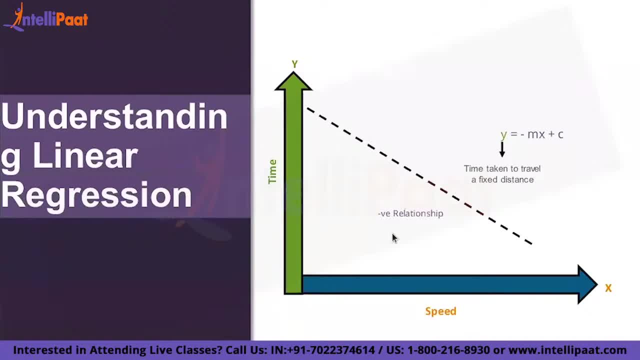 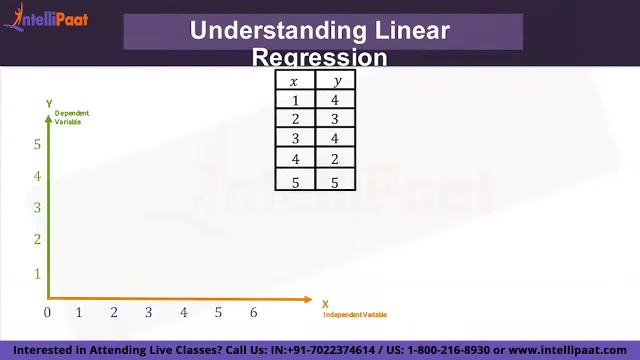 take long time. if you go fast, it will take less time, so this is something which is fine. negative. now, having said this, you can see all these things are: y is equal to mx plus c. dependent variable, independent variable. all these things you already know. now we will understand the concept. 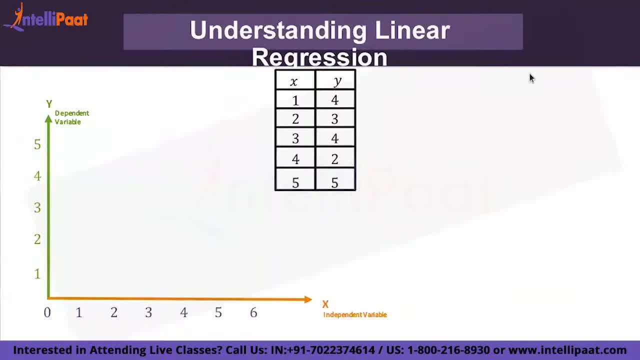 of finding the best fit line. so how are we going to get the best fit line and also how do we measure how good the line is, or how good the linear regression line explains the relationship. that also we will see in this particular mathematical calculations. now i have 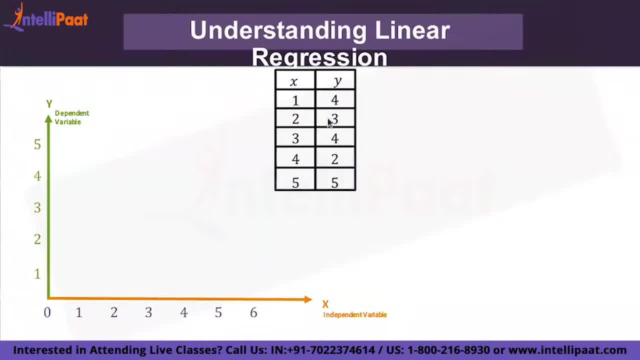 x, i have y. so x is 1, 2, 3, 4, 5, y is this one. now, what i am going to do here is i am just plotting. for every value of x, i am plotting a value of y. so for 1, i am plotting 4. for 2, i am plotting 3. 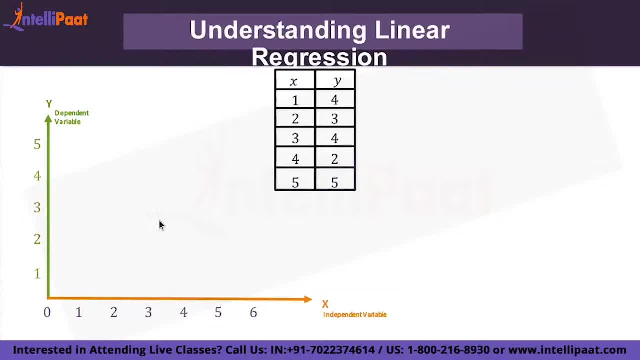 for 3, i am plotting 4. so similarly, whatever value is there here, i am plotting all of them one after the other. so if i do that, like this, for one, i'll plot 4. for this value, for 2, i'll plot 3. so 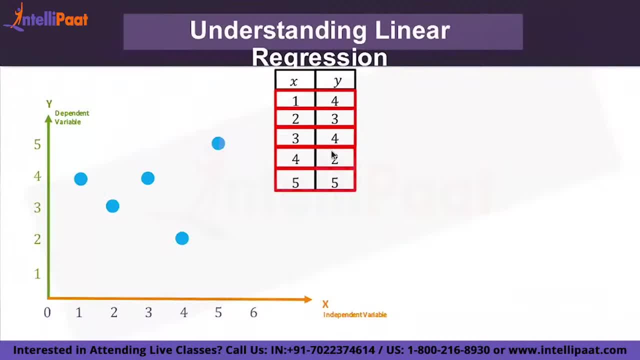 similarly, i'll get a plot like this for a given value of x and y. so this is my independent variable, this is my dependent variable, all of you know. so now i need to find out a line that will be a best fit line. best fit line means that will give me a good estimate of whatever i'm trying to do, so that 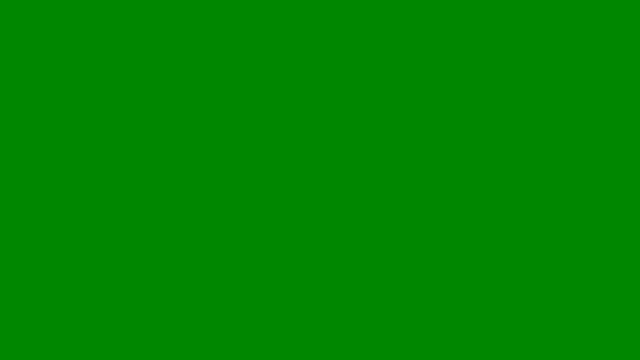 is something which i am supposed to find. so how am i going to find mean of your x and y? so if you find the mean of your x and y, you will get 3 for x bar. this is, i think, 3.6 for y bar. you can see. 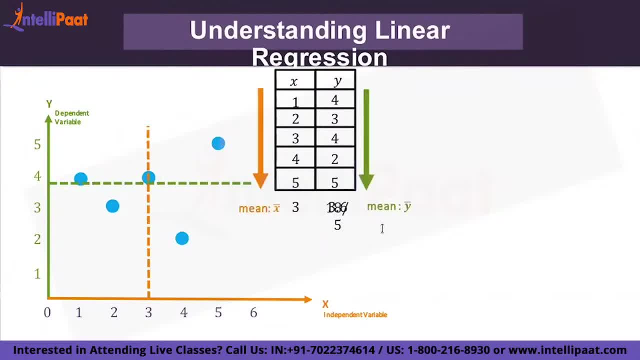 this is 3.6 for y, bar three, comma, three, point six, understood. first step: find the mean. i want you to tell me yes or no for every step, please understood. you plot x and y, find the meaning of x, find the mean of y. so this is step number one, and then you plot this thing here. why am i taking that one is: 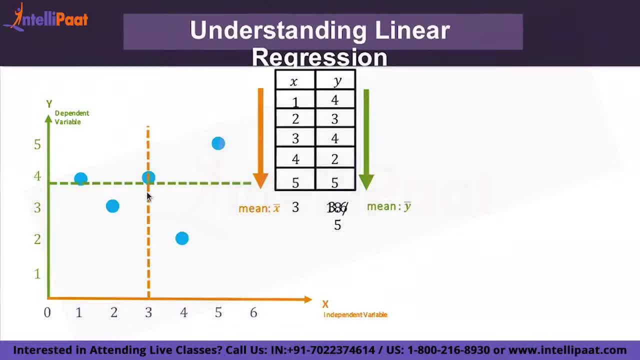 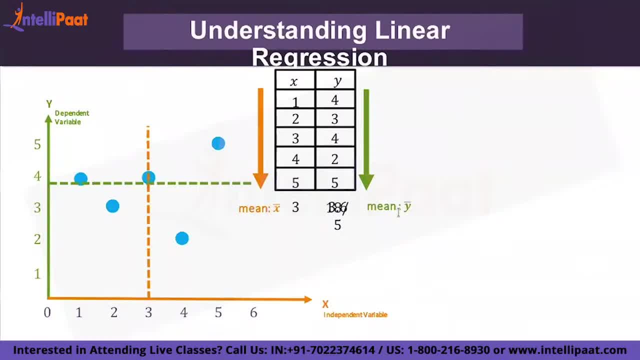 is the objective why we found out this mean. so x bar, y bar. we find a mean and then we plot it here. so this is step number one. step number two is: i have just put the estimate, so y is equal to mx plus c. i have taken a rough estimate line, so this is not the final one, i have just taken one line. 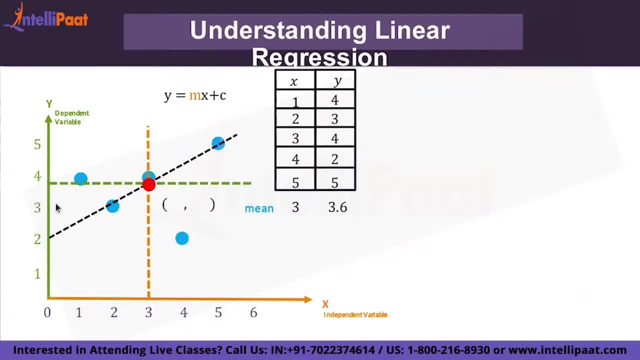 like this i can take. like this also, i can take. like this also, i can take however i want. but that line should pass through, this dot, clear to all of you: till here, nice, now we will see what is this point. so this point, all of you know this is nothing but three comma, three comma 3.6. 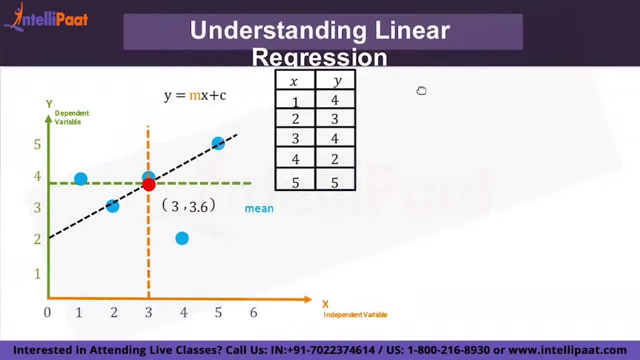 so that's what i took: the straight line drawn connect to the mean of x and y, to x and y y-axis, correct? so the straight line is drawn connecting to the mean of x and y-axis, correct, you're right. true, what you said is true. the straight line is drawn by connecting the mean. 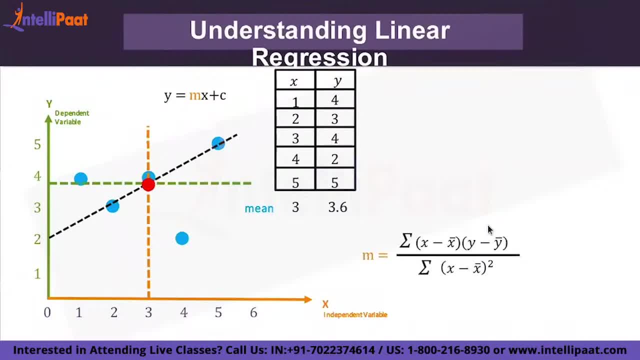 of your x and y. so that is step number one. my next step is finding the value of m. so how am i going to find the value of m? the value of m is nothing but for every value of x. okay, just see the formula. it is summation: x minus x bar into y minus y bar divided by x minus x bar, the whole. 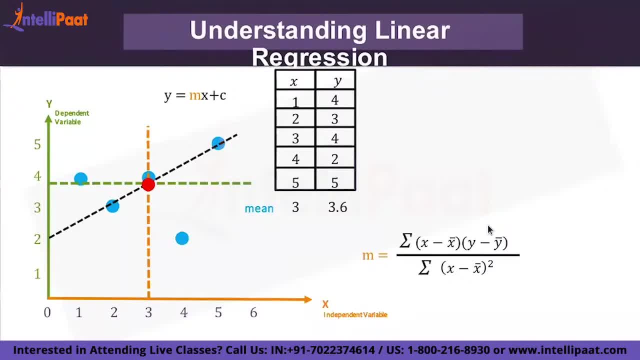 square. so it's a summation. so what you are supposed to do, you're supposed to find x minus x bar, y minus y bar, so to find the value of m. so you know what is y, you know what is x. so only two things that you need is what is m and what is c. so c you will get. 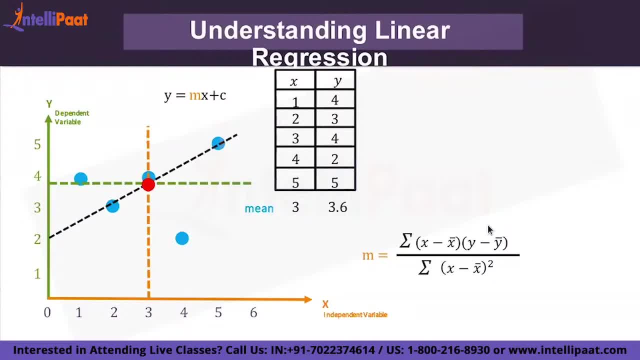 you make, your x is equal to zero, x bar is the mean, x bar means mean right, so x bar is mean. so we have found it out, i'll show you. you can see here you found a mean x bar, mean y bar, so x bar y bar is. 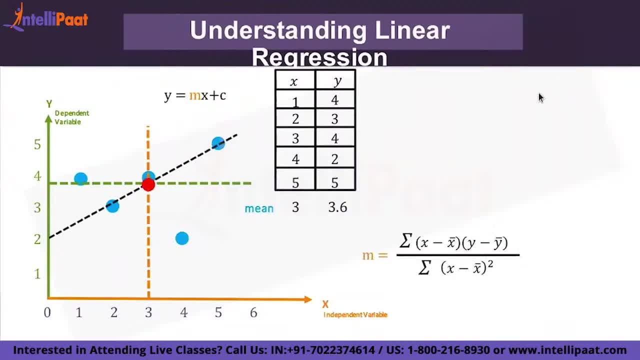 mean now you have x, you have y, you will get the value of c. if you make, x is equal to zero. the only thing that you are missing here is m. so m is your slope, so the value of m. so the value of m can be found by x minus x bar into y minus y bar, divided by x minus x bar, the. 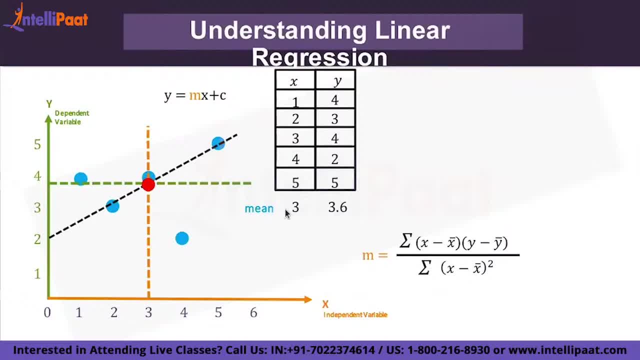 whole square. now what i'm going to do is: i know the x bar value, y bar value. i will find x minus x bar, y minus y bar in two new columns. so 1 minus 3, 2 minus 3, 3 minus 3, 4 minus 3, 5 minus 3, so that. 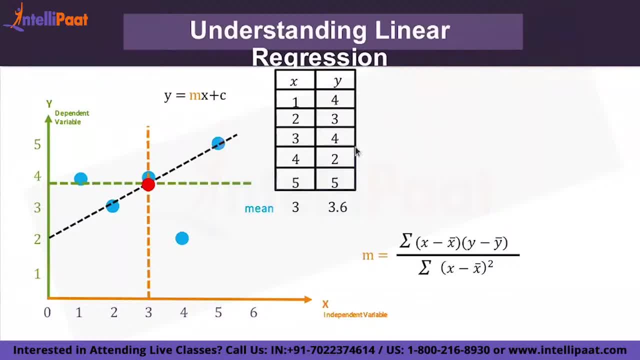 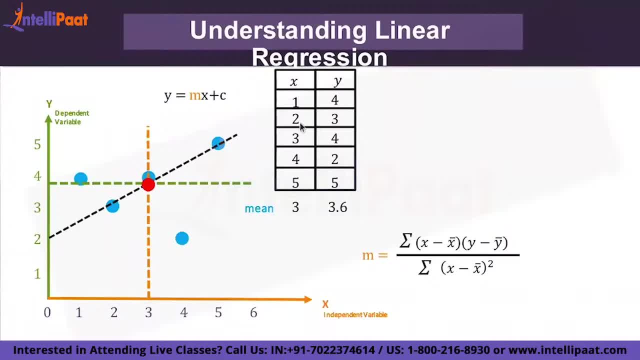 did x bar, but it's the other way around: 1 minus 3, 2 minus 3, 3 minus 3, like that, 4 minus 3.6, 3 minus 3.6, like that. so if you find x bar and y bar in two new columns, it will look like this correct. 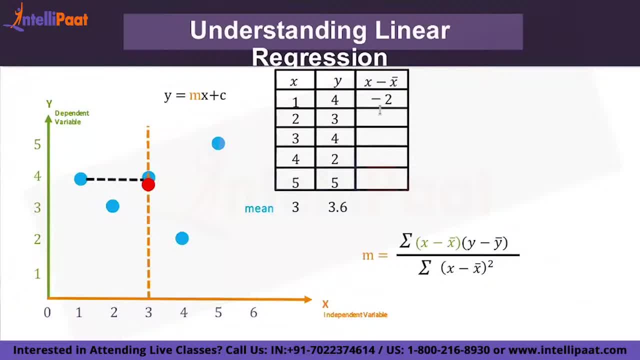 don't worry about the graph, but i'll show you the numbers. just see the numbers. x minus x bar means the difference between your x axis error. so similarly, when you do for all of them, it says this is far away, this much from this. x bar mean y means this is so much distance away. 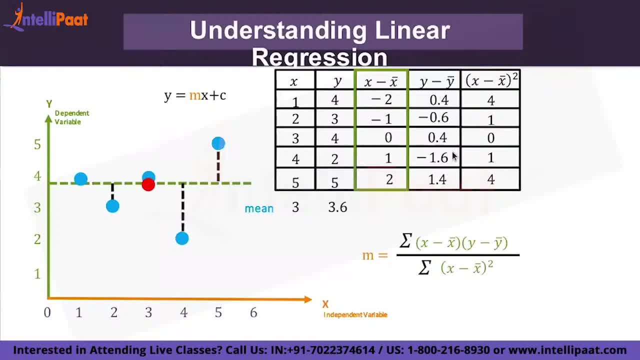 from my mean clear till here. is it clear to all of you? x minus x bar. y minus y bar. x minus x bar, whole square. clear. ok, then, what we are going to do here is we'll be defining these two points now. what you will do is: 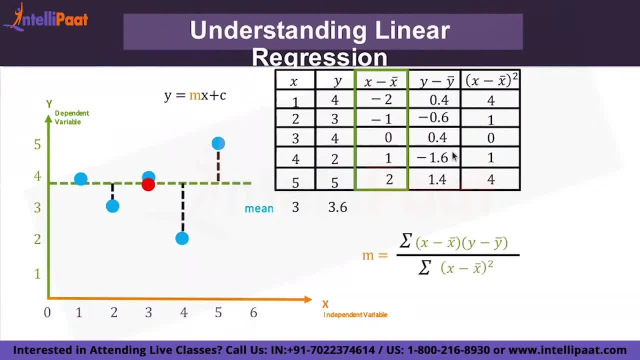 you will find the value of m by dividing. first what you're supposed to do. you're supposed to sum up x minus x bar and y minus y bar and then sum up this. you're supposed to multiply these two, sum them up and divide by this. so if you do that, you can see you'll get one value: x minus x bar, y minus. 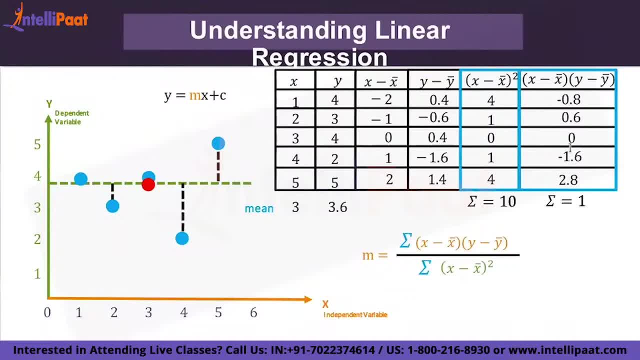 y bar is like this: you will get all these values: sum x bar, y minus y bar is 1. summation of x minus x bar, whole square is 10, so basically 1 by 10. so 1 by 10 is what? 0.1. so that is the value of your m, correct? got it? no issues still here? 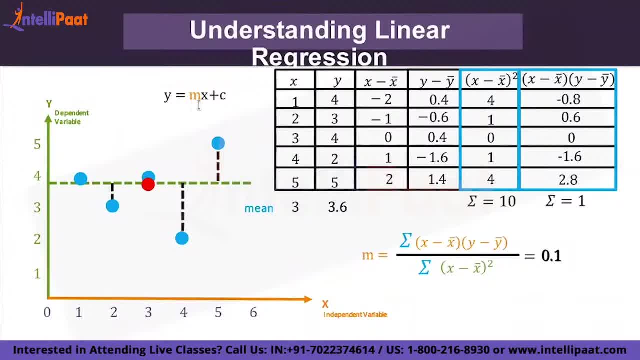 now you can replace: y is equal to 0.1, x plus c. that is your linear regression equation. clear: see 3.6. see y is 3.6 here because y average is 3.6, x, m is 0.1. you don't, you got it. no, c also. 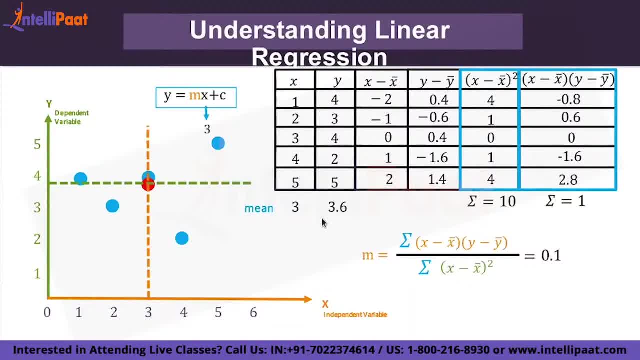 will get it. and then x is 3 average now 3.6 is equal to 0.3 plus c. you are getting how we are getting this equation. now tell me what is value of c: 3.3. now you got it. now, once you get your c value, now tell me what is your linear regression equation. 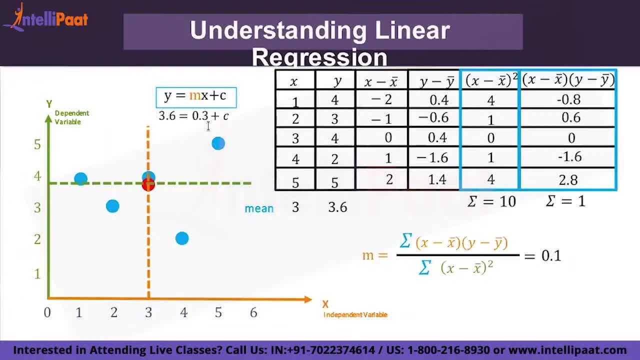 y is equal to mx plus c. with what all values you found out. what is the linear regression equation? y is equal to. y is equal to 0.1 x plus c value. you got it. no, just know exactly. y is equal to 0.1 x plus 3.3. so that is my. 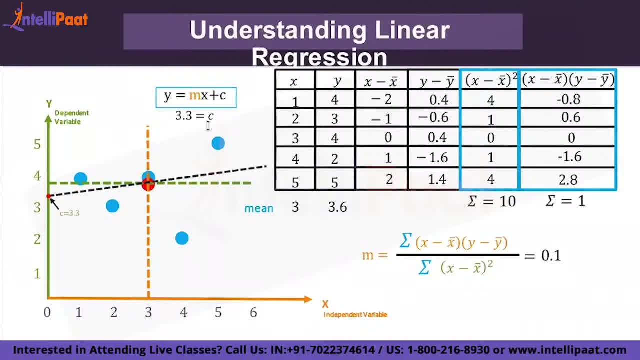 solution: linear regression equation. you can see that is what you will get. c is 3.3. now plot the c here. any line, i mean see all of you know to draw a straight line minimum, how many points are needed? two points. to draw a straight line minimum, two points are needed. so one point. you got it by. 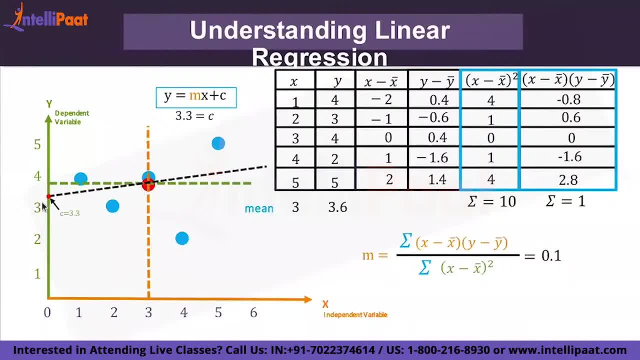 using the mean of x and y. one more point: you got it by c, so now you can draw the straight line. you have two points. no one. you got it by using x bar and y bar. one more point: you got it using c. with these two points, don't you think you can draw a straight line? all of you got it. now this: 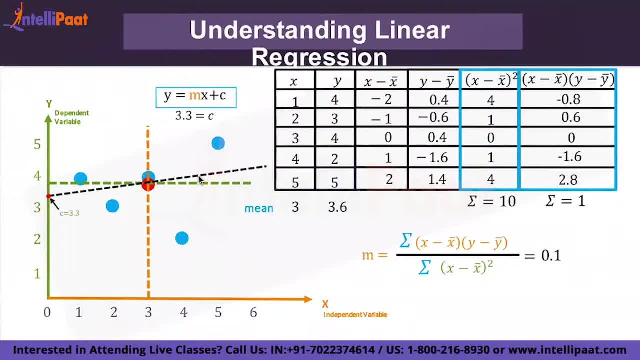 is the line that you will be considering for your linear regression. very simple, step by step. i will tell you and then we will see. you can see. equation is same what you said: regression equation y is equal to plus 3.3. now, by this you can estimate. 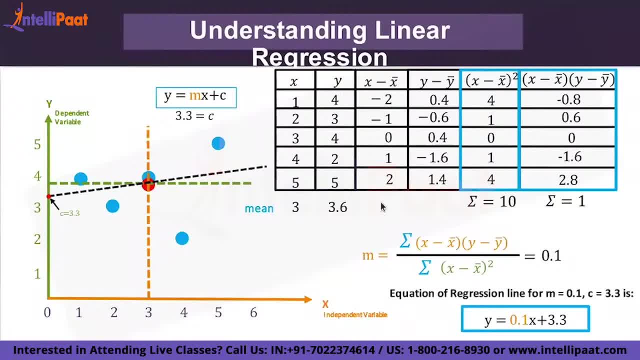 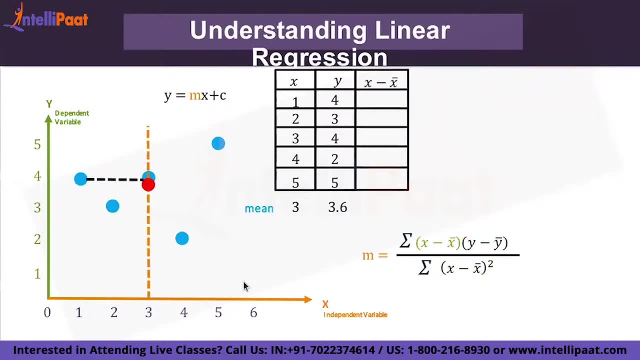 i will just repeat the complete process once again. this is the line of best fit, correct, this is the best fit line. i will tell you the step by step approach once again, just see if you are able to understand or not. so i will just run it once fastly so that you can just observe. 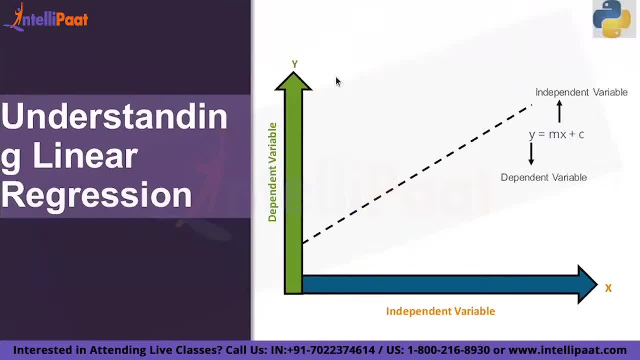 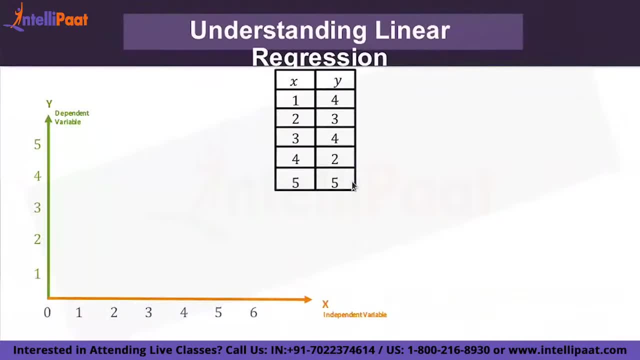 and then tell me- so this is a quick, quick round, okay, understand this carefully- to find out a linear regression equation. what are we going to do? we are independent variables and dependent variables. we plot them like this, all of them: first step, find out x bar, y bar, which is mean of x and mean of y, and then plot a dot using these two values. you got one. 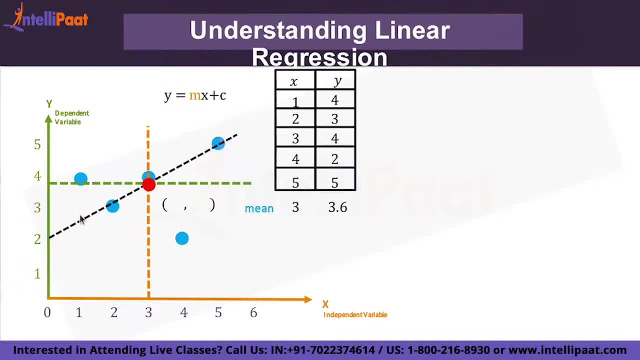 point to draw a line. you need another point to draw a line. so what is the equation of your straight line? y is equal to mx plus c. c is your y intercept. y is dependent variable, x is independent variable, m is a slope. now what we are going to do is: 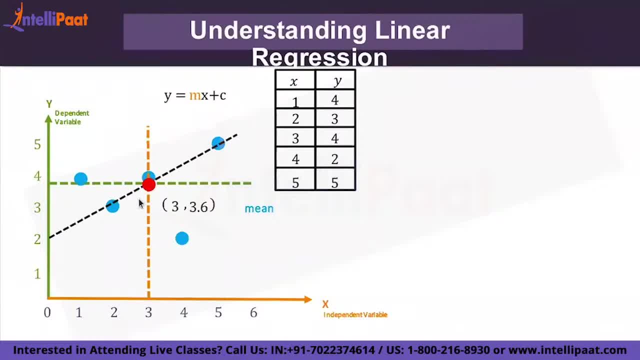 by using these values we are going to. you plotted a dot then to find out my value of m. m is nothing but x minus x. summation of x minus x bar into y minus y bar. x minus x bar, whole square summation. so this is the formula. so, anyway, you have x, you have x bar. you have y, you have y bar. 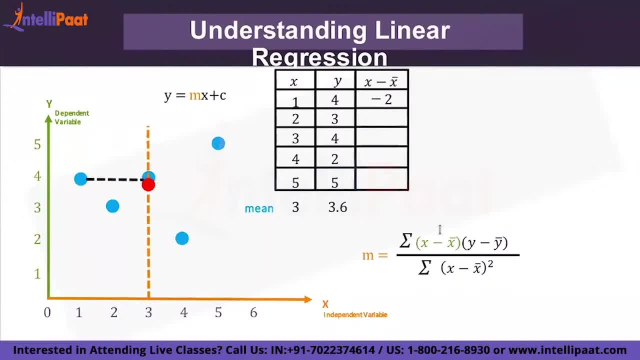 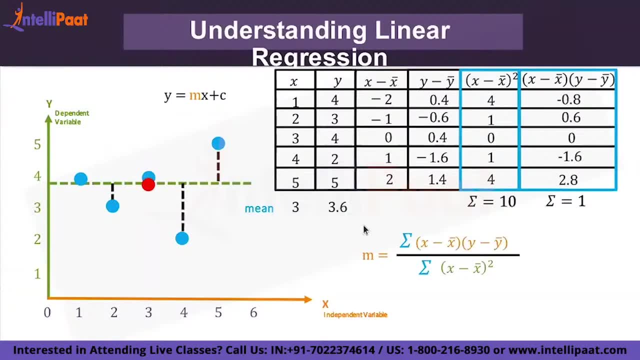 so you find out m. so you basically find x minus x bar and then y minus y bar and then x minus x bar, whole square. then do a summation of these two. then you will get 0.1 as your m. now you have your value of m. so y, you know, x, you know m, you know c, you need to find out. so what you will do, you will. 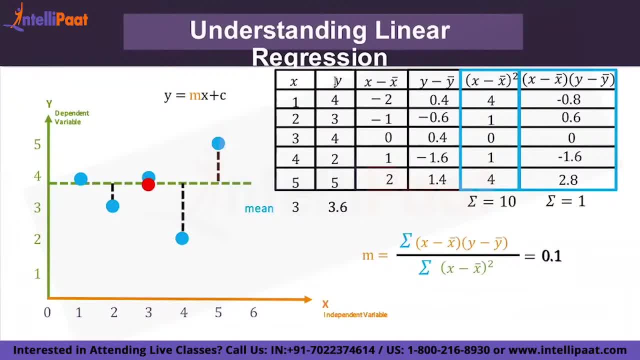 replace them. for x, you will put it as 3. for y, you will put it as 3.6. for m, you will put it as 0.1. so if you replace these values, then what you will get is c is equal to 3.3, so you already got 3.. now a. 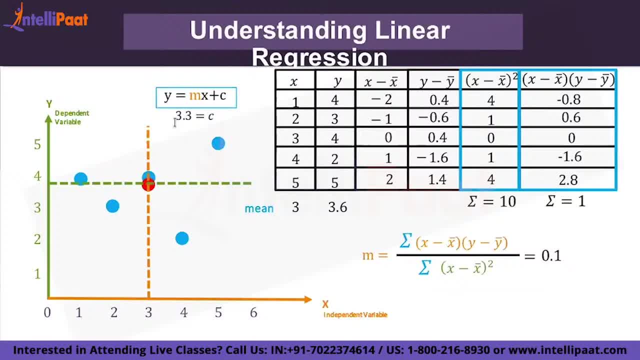 value, which means c is nothing but y intercept, which is 3.3, which means you'll, as you'll, put a point here, this point is 3.3. now you have two points. you draw a best fit line, so now this is the particular linear regression line that you're having. now. if you want to construct a linear 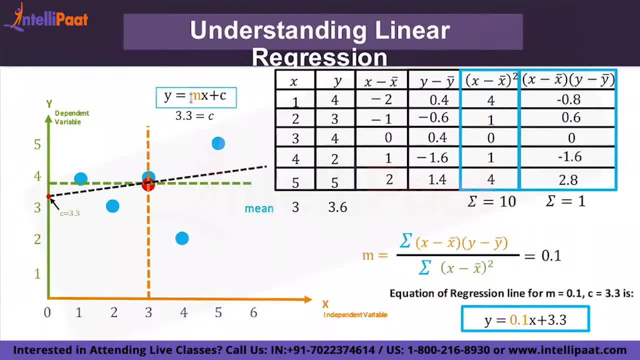 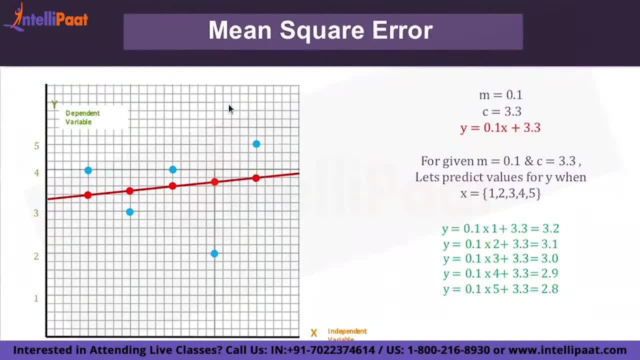 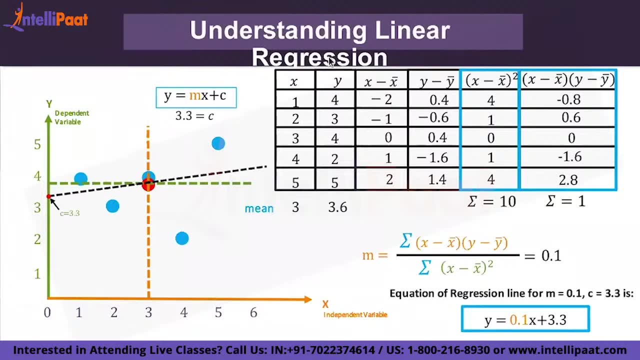 regression equation: y is equal to m is what m is 0.1, c is what 3.3. y is equal to 0.1 x plus 3.3. so that is your linear regression equation, step by step approach. clear. we are not going to run all these things in code sanjay. so what we are going to do is we are 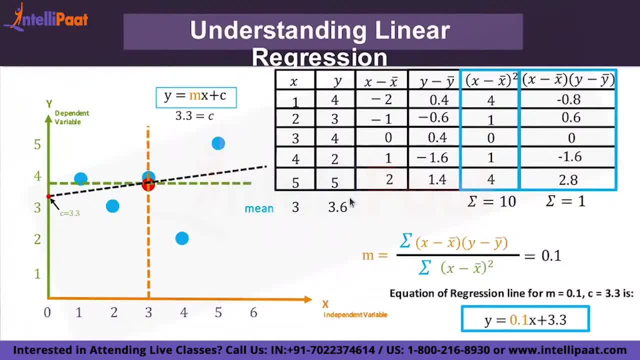 just going to see few things. i mean how to build a linear regression model. so these things you're not running in code. these things will be used to learn. so in python it is only one or two lines of code to draw a machine learning model. but you should know how it works now. so that is the reason. 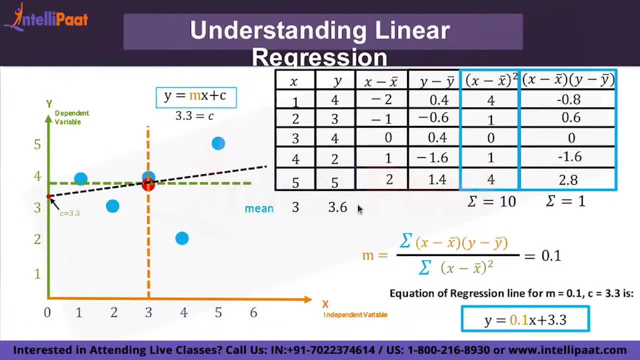 now you understood that you can use this particular uh equation which will give you a fairly good estimate of the data, which means it will tell you, like okay, how your data is there, just like how we have accuracy and other things right. so we also should have a matrix which will tell us how good or how. 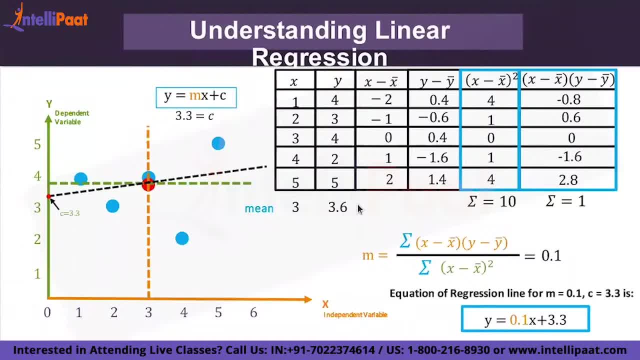 well, this particular line is explaining my data right, because it is not 100 good model, i mean 100 best hit line, because you have some error here, some error here, some error here and here. this is the line that will give you the least error, right? there are multi, multiple ways of finding that least error. one is called as ordinary square one. 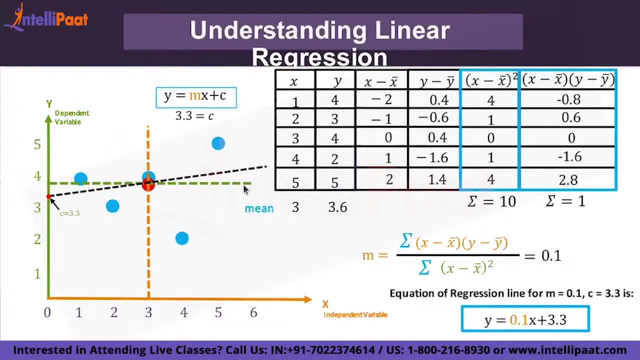 is called as gradient design. so multiple types are there. this is one of the type. now, having said this, so you can see your m values are the same, as you know, right, and then you can see that the m value is large or zero. so the new match or the new number here is 1 in the number. 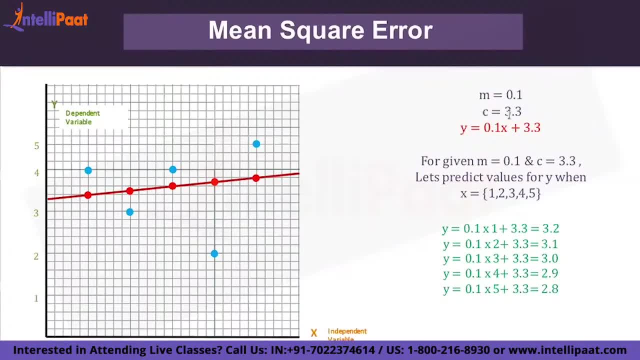 It is not 100 good model. so if it is 100 good model, value: 0.1 c value is 3.3. y is equal to 0.1 x plus 3.3. now what you will do is for a given value of 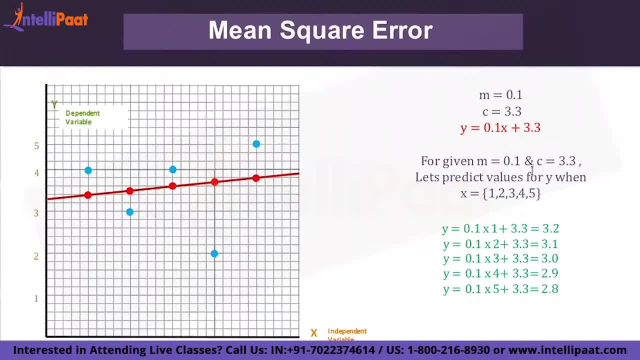 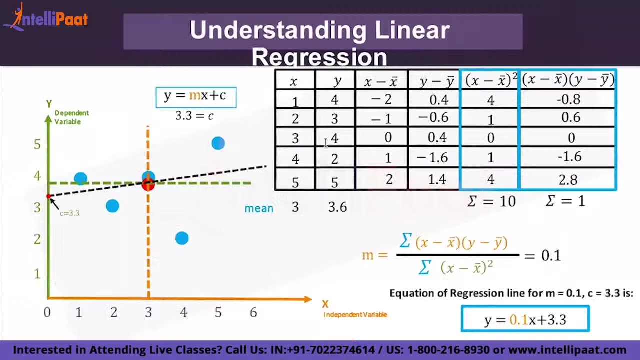 m. understand this carefully, for given m is equal to 0.1, c, c is equal to 3.3. let us predict values for y when x is equal to 1, 2, 3, 4, 5. here, if you can see, the value of x is 1, 2, 3, 4, 5. so these are. 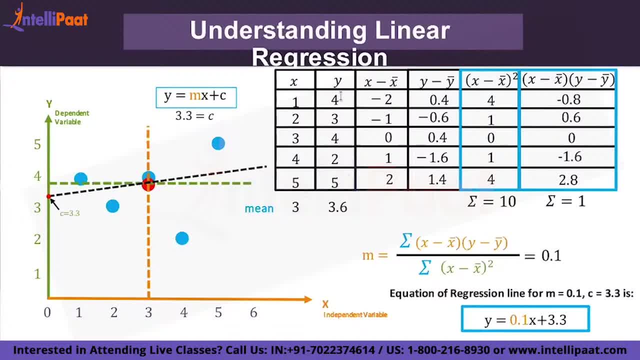 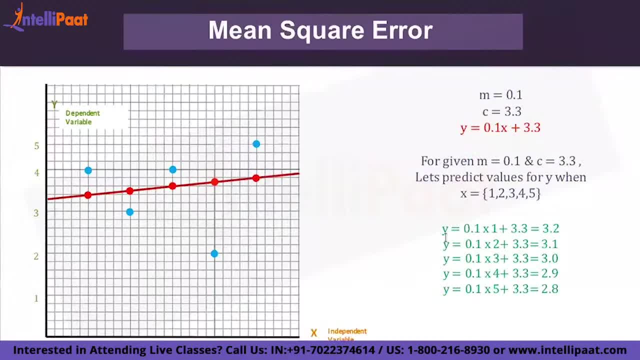 actual values. y is equal to 4, 3, 4, 2, 5. these are actual values you have brought. you have got the line. now you will predict the values. so if you predict the values, it will become 3.2, 3.1. 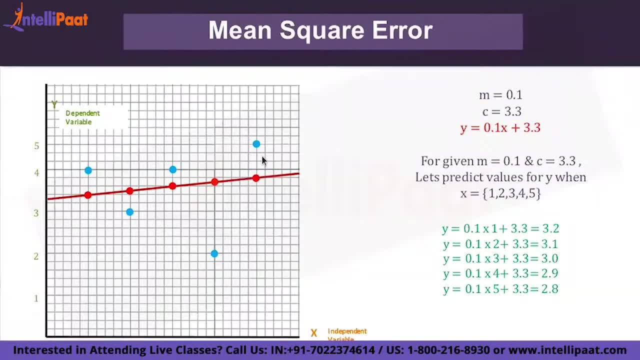 something, something you will get, so predicted values. so blue is your actual value, red is your predicted value. clear by using the linear regression equation. clear to all of you now, once you do this particular prediction, just replace your value of x with 1, 2, 3, 4, 5, and then you will get the value of y. so this is your. 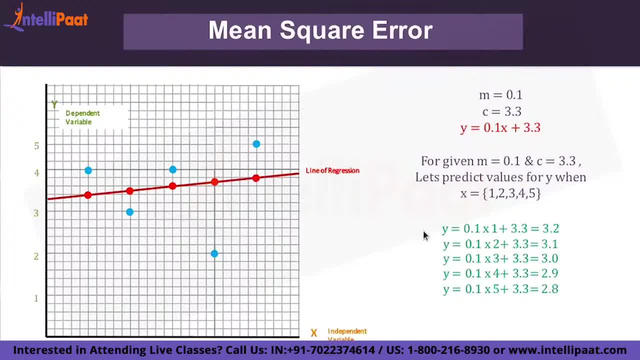 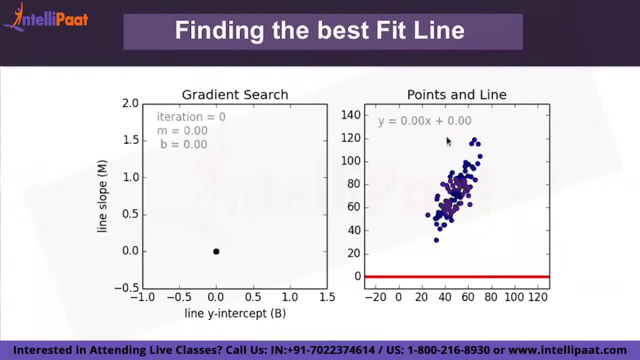 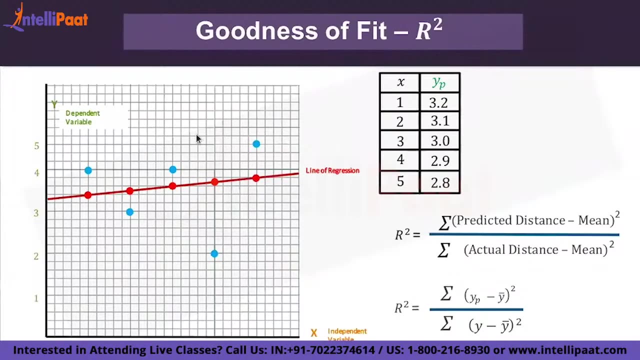 predicted values. so you have actual values and predicted values. now the next step is- this is, as i told you know, by finding the best fit line, gradient search, and then you have ols, multiple methods. what we are trying to do is, you are just trying to see what is the goodness of it of this. 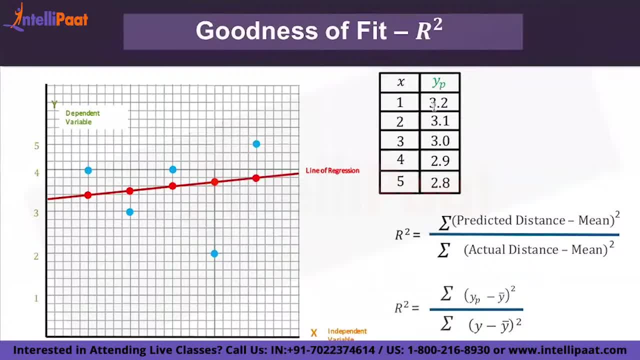 particular line. so this is my x, this is my yp means y predicted. i have something called as r square. r square is a measure of goodness of fit. you can consider r square as an analogous to your accuracy, which means you can. you can probably understand r square is similar to your accuracy, which means how well my model is able to explain. 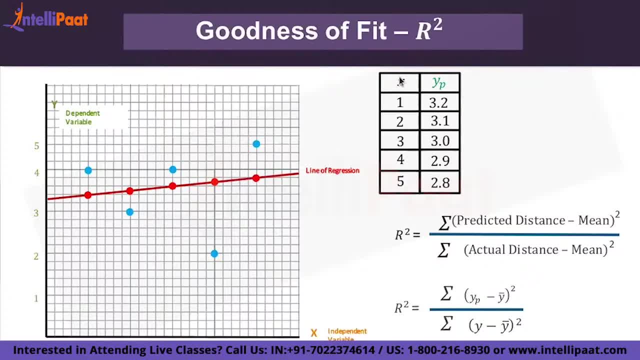 my objectives or observations. we are actual, red is estimated. blue are actual, red is estimated. values on the line: estimated values. all of them are there on the line. how do i find r square? r square is an error at all. okay, r square is nothing but predicted distance minus mean divided by actual distance minus mean the whole. 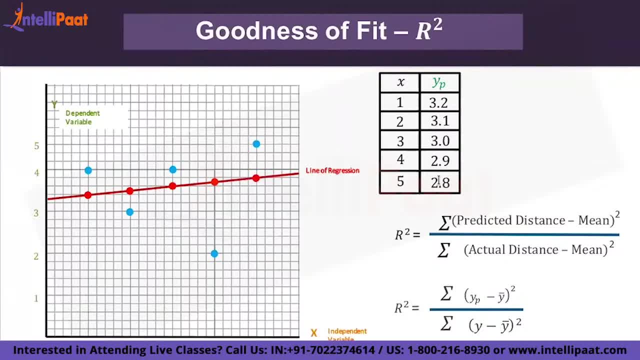 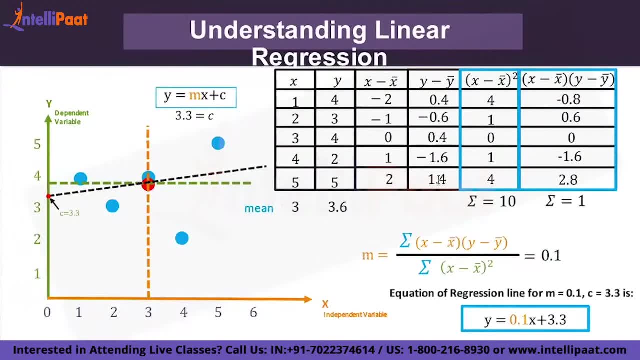 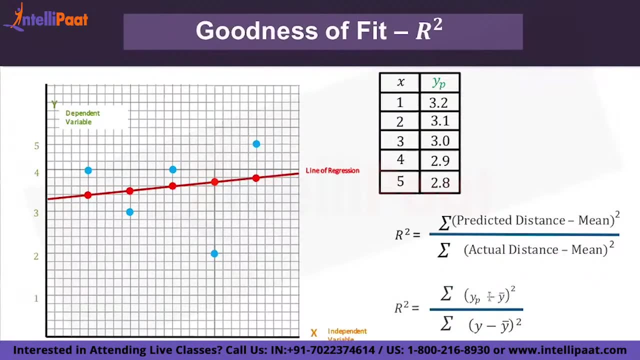 square predicted distance minus mean. what is my y bar? all of you know y bar is three times the three point six you saw on the top. correct y bar was three point six. you can see y bar is three point six. now, predicted minus mean, actual minus mean. so yp y bar, y y bar. so if you sum them and then keep it, 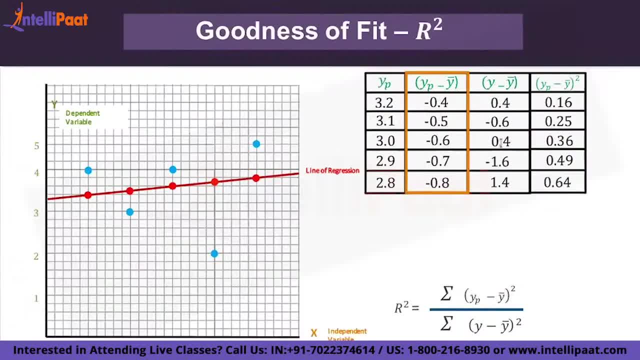 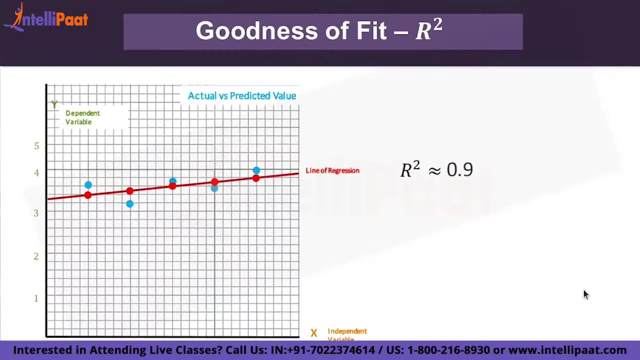 you can see. you can do this: yp minus y bar, y minus y bar, so summation, and then this also you have. so when you sum this, you will get one point nine and five point two. right, so one point nine by point two. this is your r square. so you get 0.36. r square is 0.36, r square is 0.36. you can see this. 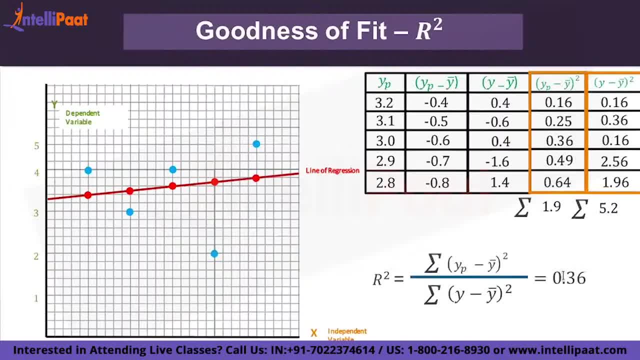 there are some different lines. i am trying to show you r square for our particular line is 0.36, which means my model is around 36 percent. it is explaining- it is not explaining me the complete observations. so it is not explaining complete observations, it is only explaining around 36. 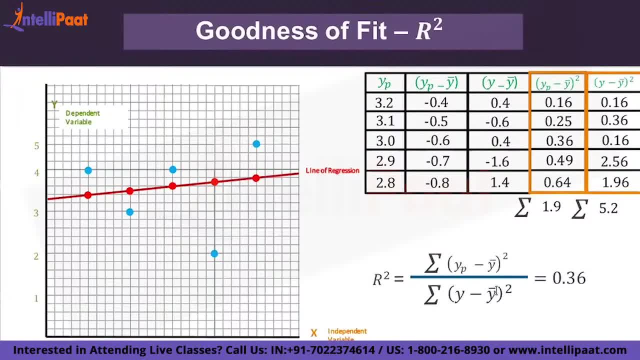 percent. so when i, when i just say my line, i'm only around 36 percent confident that i'm able to get a correct estimate, so that is a goodness of it. or r square. now if i want to show you a few more lines. so let us say, for example, when r square is 0.6, which means your dots will be good. 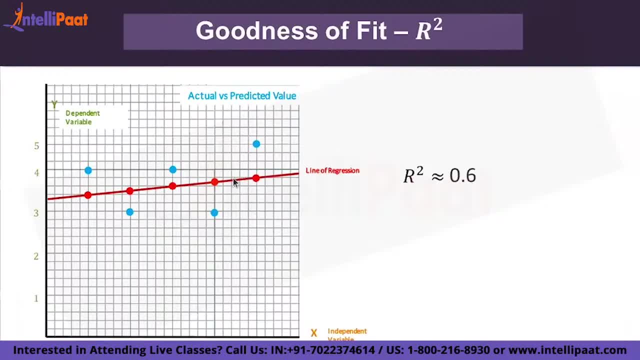 so this is for a different values. i'm just telling example how it varies. 3.6. it looked like this: all the dots were far away. 0.6- all dots are little nearby, so if you bring them little more closer your r square will increase. 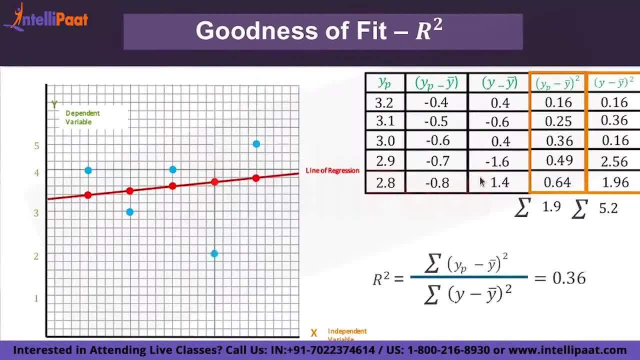 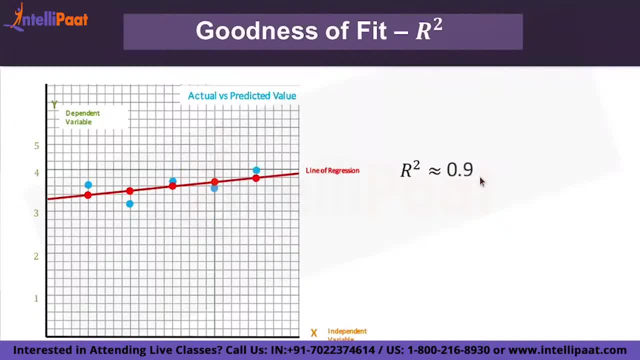 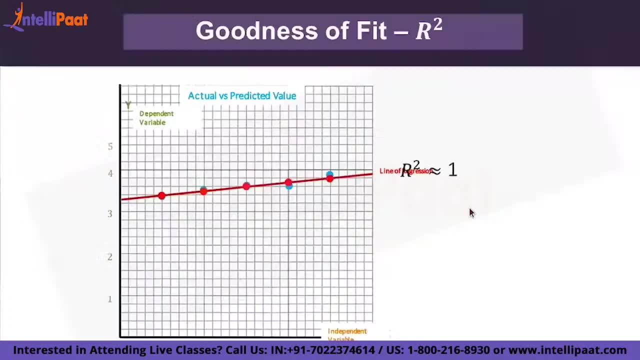 so, basically, your r square will reduce if your data points are far away from the line. r square will increase if your data points are near to the line. so if your actual versus predicted both are same, then r square is one. so this is something that i wanted to tell you. 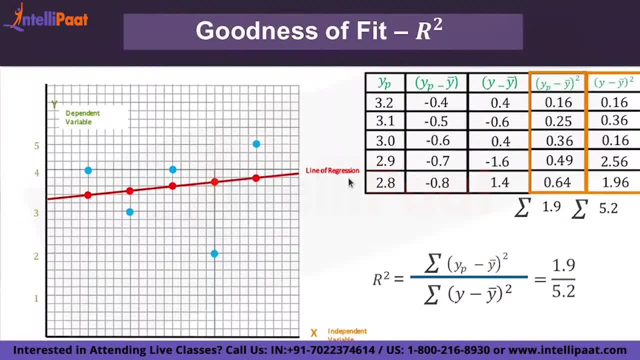 r square. is this clear about r square? goodness of fit. clear to all of you. so r2 is r2 is r square. it's not r2, it's r square. r square is a goodness of fit, which means how well my line is able to explain the observations, which means how nearly. let us say, for example, how near. 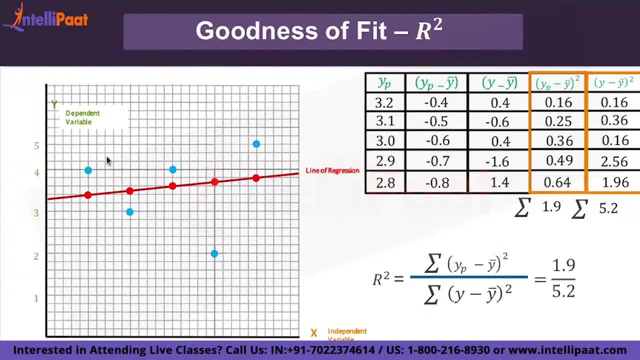 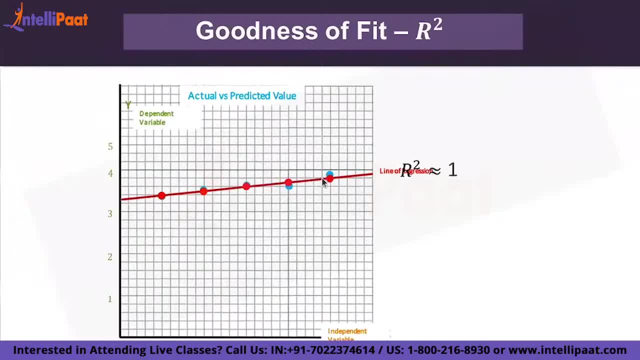 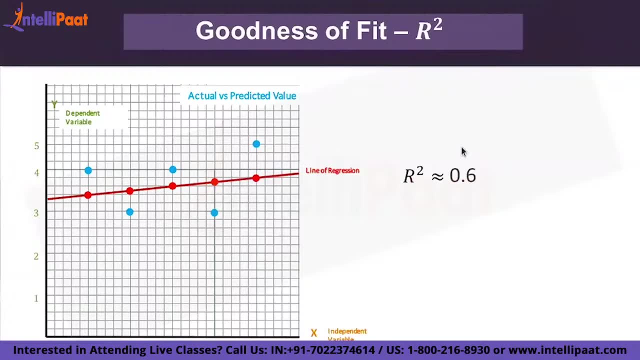 nearly nearly the data points are near to my line, so it's a degree. so when i say 100, all data points are near to my line. i have a very good estimate, very linear, very good. if this increases, which means the data points are far away, which means only 60 correctly, my line is able to explain the dots. 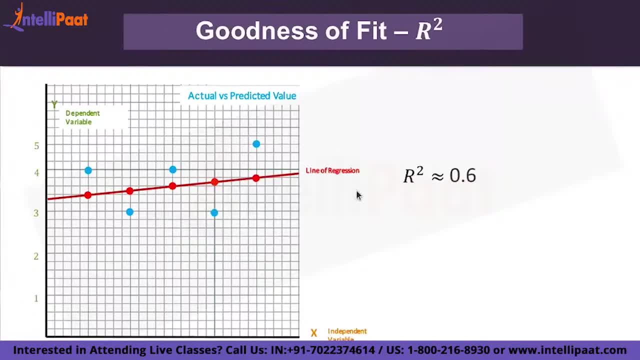 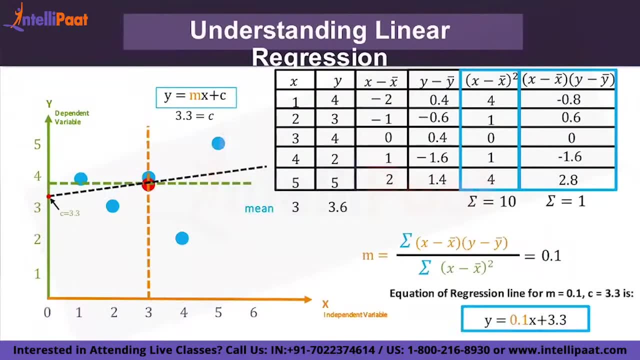 correct. so that is your r square. i'll explain r square again. just see and then understand this. okay, so all of you know how to find this particular linear regression equation correct, how frequently. but you call it, you don't call it as how frequently my actual and this will sink. it is nothing but. 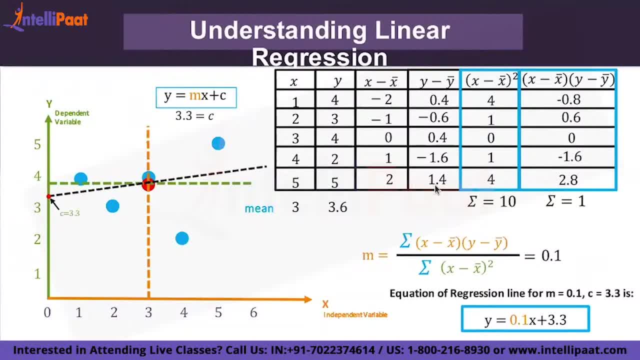 how to what extent you are able to explain your y and x. are you able to explain it 100 percent, or are you able to explain only 30 percent of the times? so that is r square. so now it's a goodness of fit of a linear regression line. now let us say: 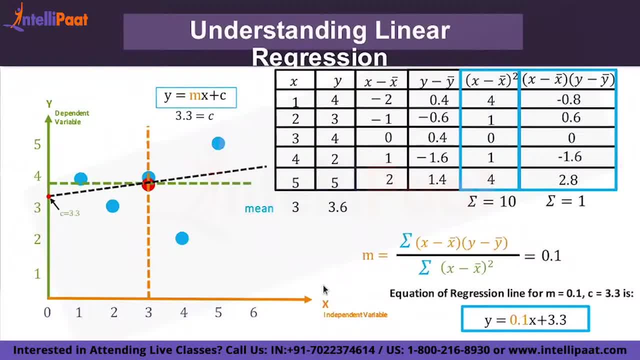 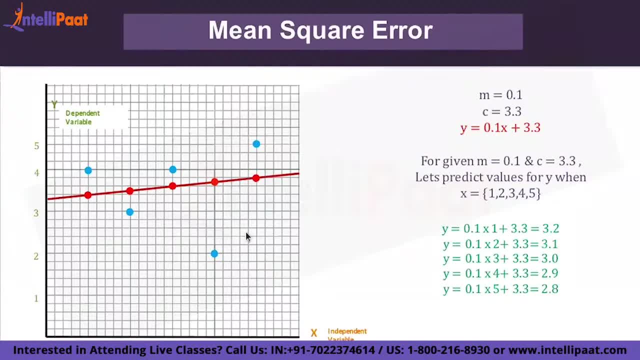 r square is a goodness of fit. this line you found out. what you will do is by using this linear regression line. you will find the estimated values. so you have a set of actual values for every value of one, two, three, four, five. for every value of one, two, three, four, five, you have a set of observations. listen to me carefully. 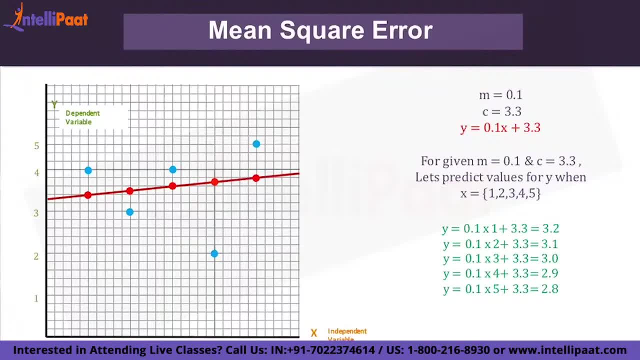 and later we can have a q, a session concept. you understand it, then you will be able to understand it, and then you will be able to understand it, and then you will be able to understand all the questions, also for a given set of independent variables: one, two, three, four, five. 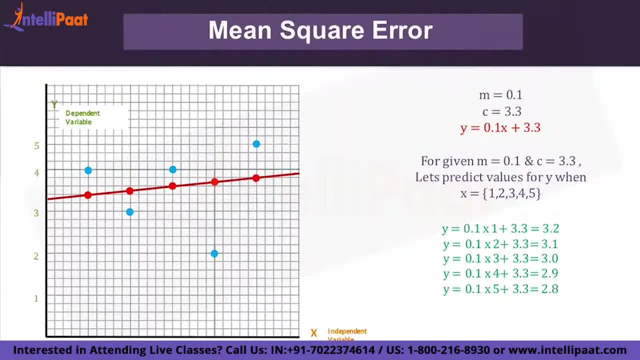 i have some observations which are plotted in blue. by using the linear regression line, i am predicting values for every independent variable, which are plotted in red, so i have actual values in blue, predicted values in red. y is blue and i have actual values in blue, so i have actual values. 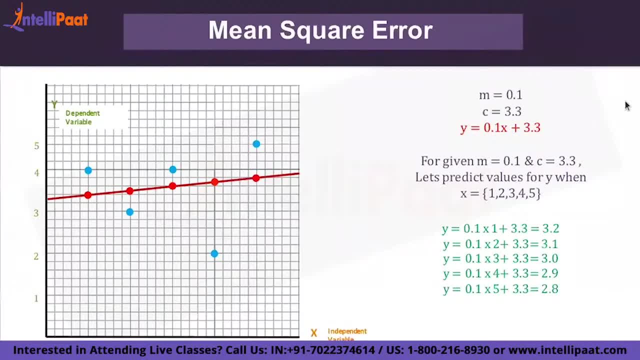 in red. so i have actual values in blue. so i have actual values in blue. so i have actual values in blue. yp is red, okay, y is blue, yp is red, right, so y is blue, yp is red. so you are estimating: y is equal to all this value. so these are your actual values and these are your estimated values, now our 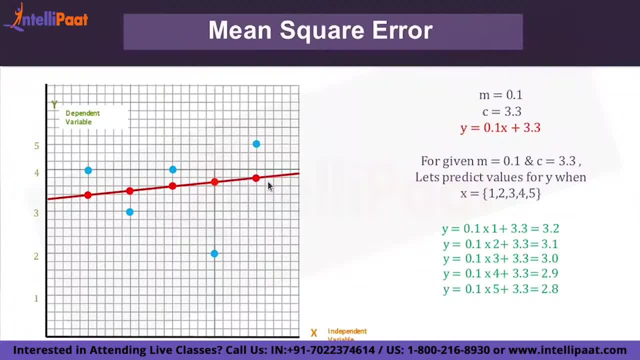 objective is to find something called as mean squared error. mean squared error is something called as r square. so how are we find out that r square is? by using these particular calculations, which i'm going to explain you now. right, r square is nothing but mean square error. 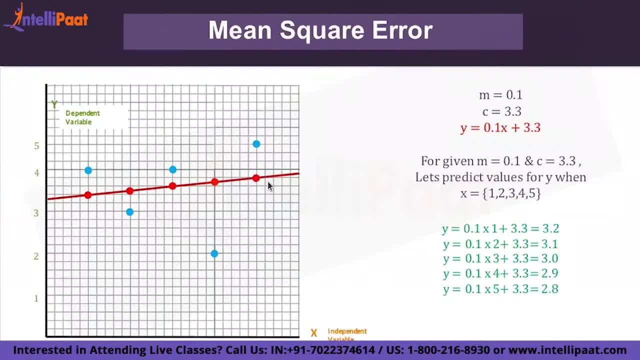 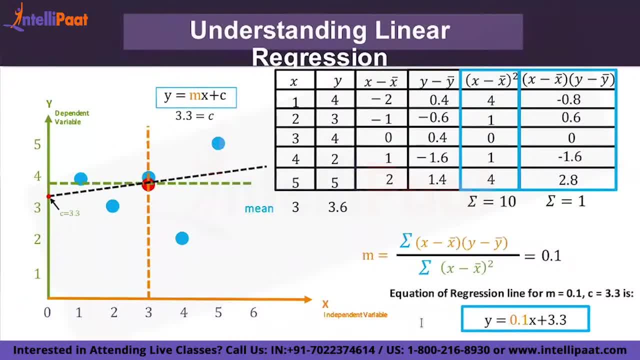 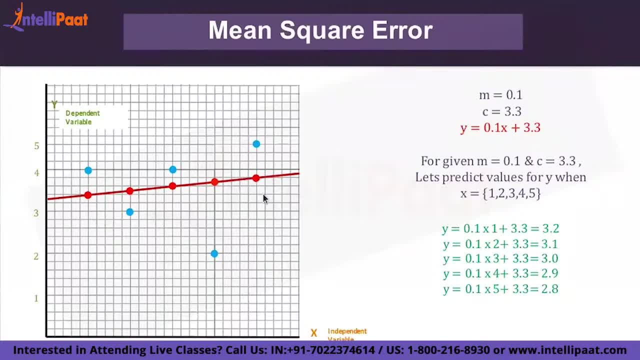 0.1 x plus 3.3. so this is a linear regression equation. by using this, we identified this actual values and the estimated values. now, to see how exactly i'm going to find my mean square error- which will give me a goodness of fit- which is r square, i am going to find out the predicted values. 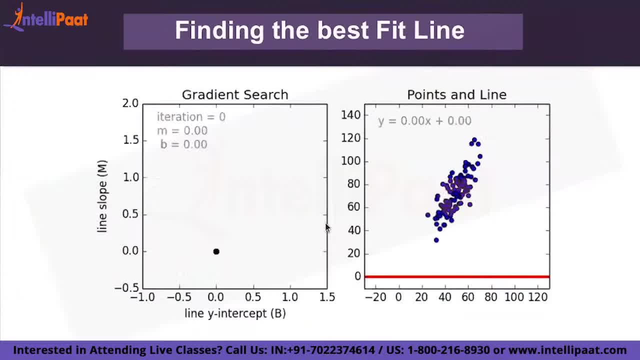 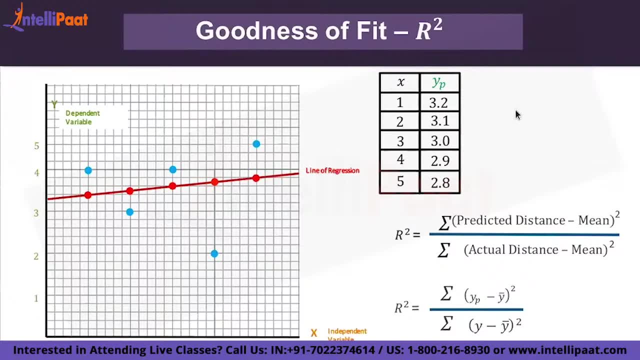 you can see here the regression line and also you are finding your r square. the formula of r square is nothing but predicted distance by mean divided by actual distance by mean, so predicted distance by mean and actual distance by mean, so mean you know how to find. so y bar 3.6, so predicted. 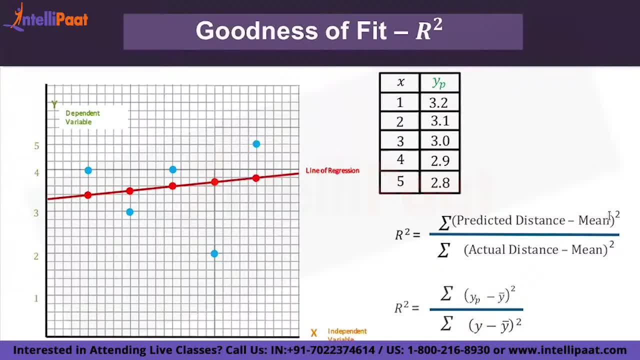 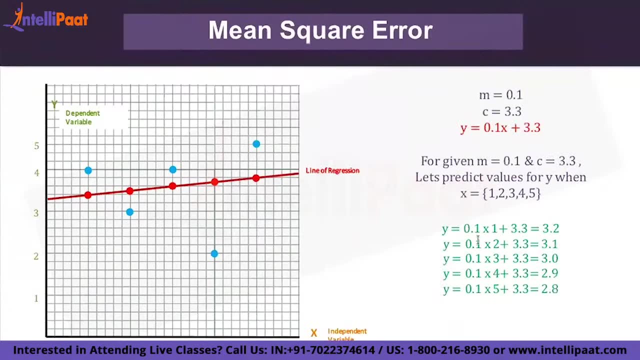 distance minus mean, which means yp minus mean. actual distance minus mean means this value minus mean. so these things that we are supposed to do, so we are supposed to do this, so we are supposed to do this. you know y, you know yp, yp. you identified like this right. so all these values that you are. 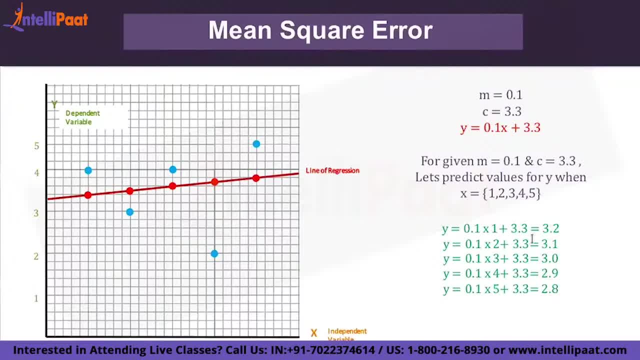 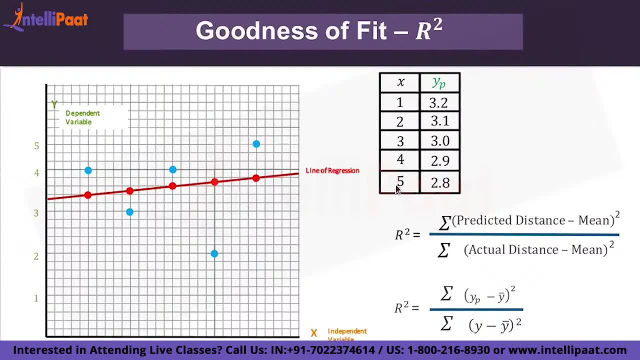 getting are y predicted 3.2, 3.1. so calculation mistake is there, but this is the values of yp, so you are getting. for every value of x, you are identifying yp. you also have y for every value of x. so you have, you have y for every value of x, which is actual value. yp is the predicted. 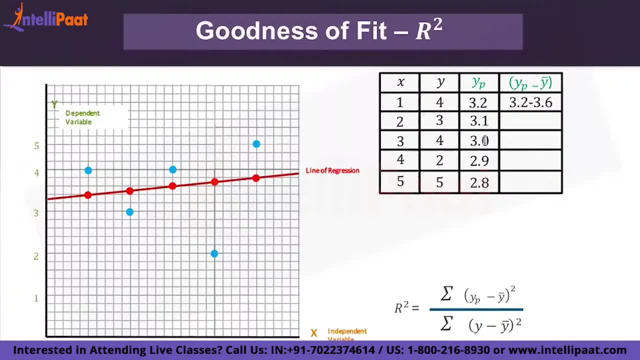 using the linear regression line. so you have y and yp. now to find out your r square, you know the formula: yp minus y bar whole square by y minus y bar whole square. you sum them and take a ratio. so you find yp minus y bar. so you have y and yp. so you find yp minus y bar, then you have y, so you. 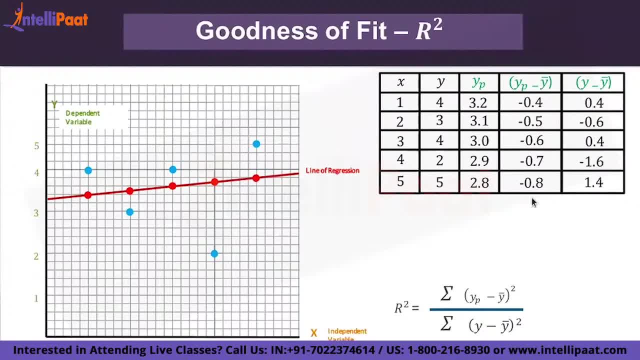 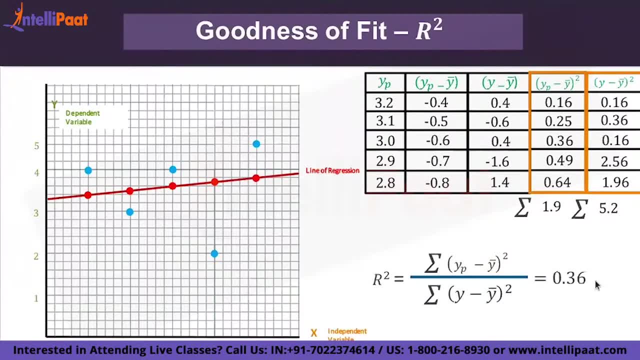 find difference: y minus y bar. so these thing, these thing you find, take a summation of both, you will get 1.9 by 5 point. 1.9 by 5.2 is 0.36, which means your r square is 0.36 around 36. 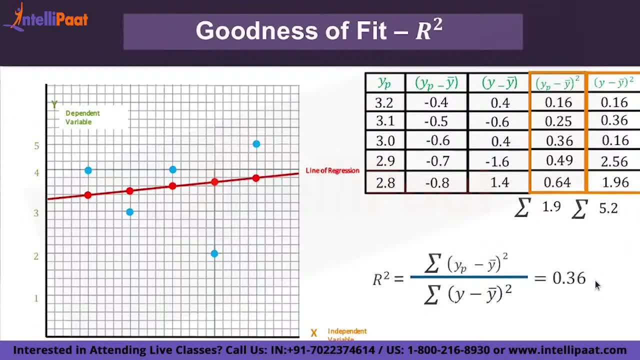 percent your line is able to explain the dots, which means 36 percent of the line is able to explain the dots. and that is how, your goodness of fit, your line is good enough, 36 percent of the times to identify the values. or you can indirectly say that your model is around 36 percent able to give a good estimate of your basic y when, for every 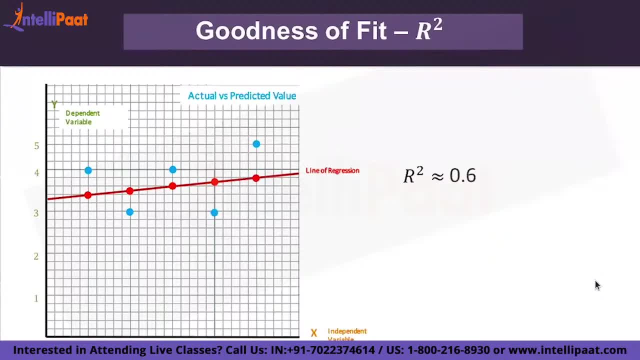 given value of x. so now how r square varies is when your r square increases, all your observed values will be the same, so you can say that your line is good enough, 36 percent of the times, to be equal to your estimated value. so you can see, r square is one means. it will be like this: 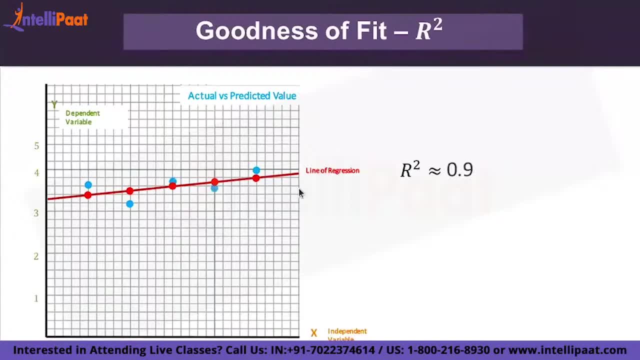 r square varies between 0 and 1.. r square is 0 means a very bad model. r square 1 also very bad model. r square 0 means a underfit model. r square 1 is a overfit model. overfitting is also not good. 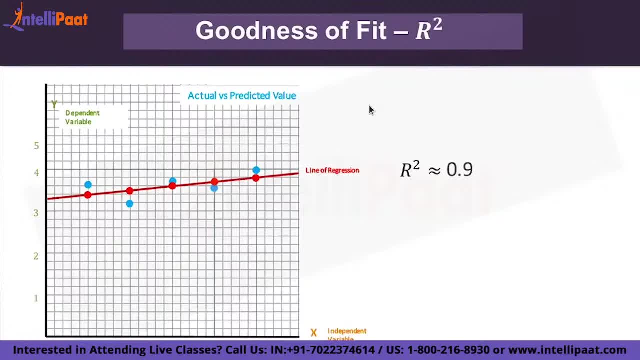 underfitting is also not good. a good estimate of r square is somewhere approximately 0.7, 0.6 to 0.85 or 0.9. so that is the good estimate of a good r square. so this is how you find out your r square. is this concepts clear to all of you? yeah, the idea behind giving negative. 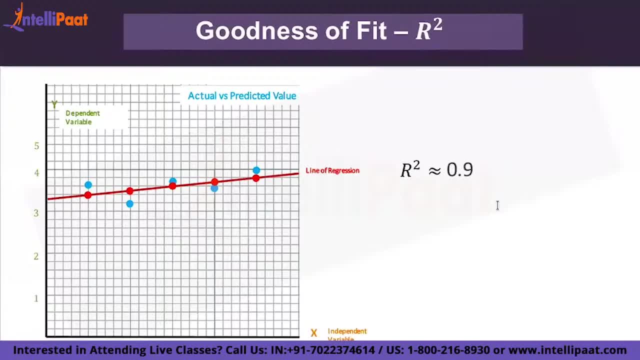 i mean, squaring is nothing, but error can be positive or negative. so let us say you have 10 data points. five values have negative error, five values have positive error. if you just sum them, it will become zero. to avoid that, to get a very good estimate of error or to get the true value of error, you square them and you will take it. 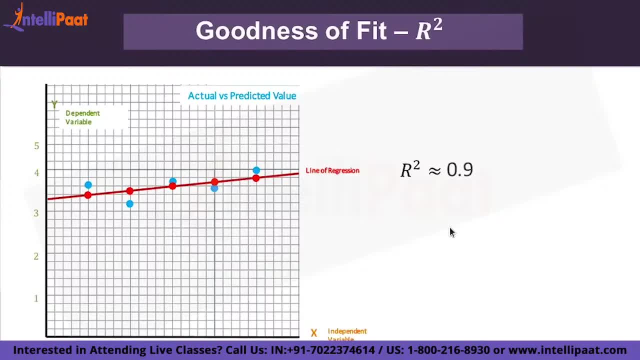 overfitting. i have not told you, i've just, i'm just told you that term. i will explain it in detail, don't worry so, but as of now it's not necessary. i just told you because, since you asked me what is the range, so zero means 100 and one means overfit. right, fine, so all of you are able to. 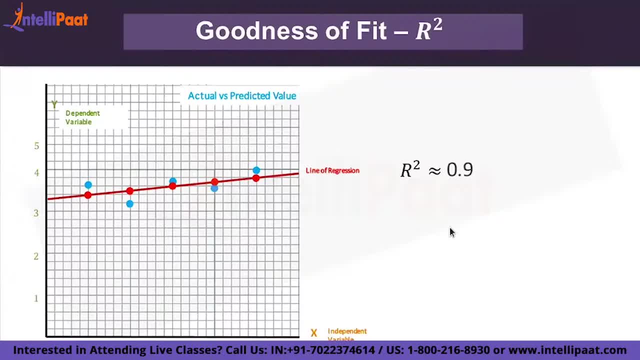 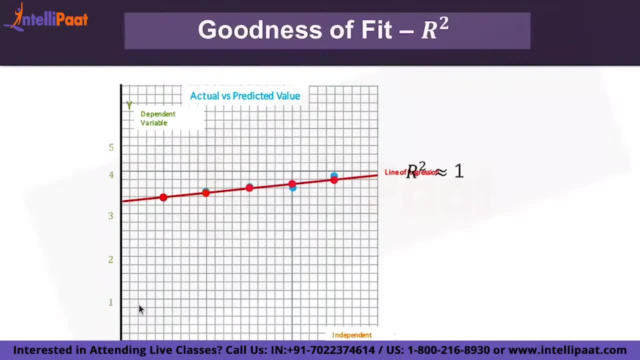 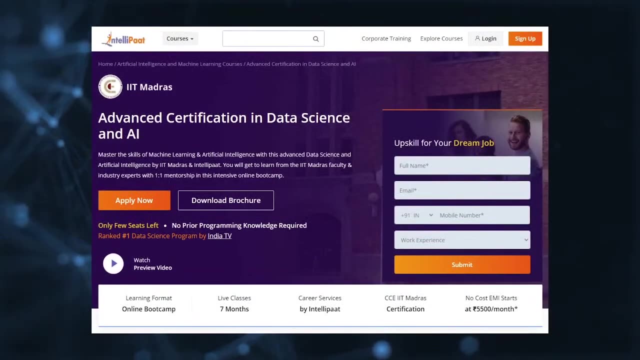 understand this concept, how exactly this is going to work. so let us say that you have a. this thing is working, okay. so i request all of you to open your jupyter notebook. we will start building the regression now. if you want to make a career in data science, then intellipaat has. 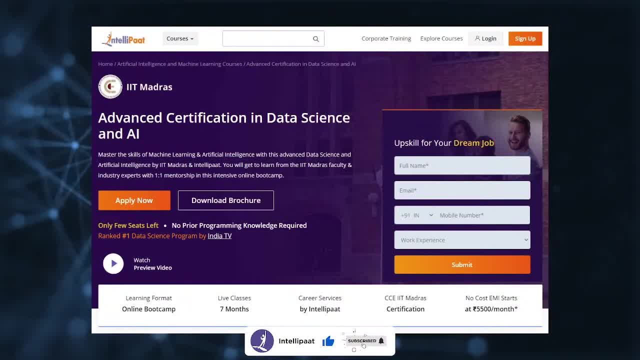 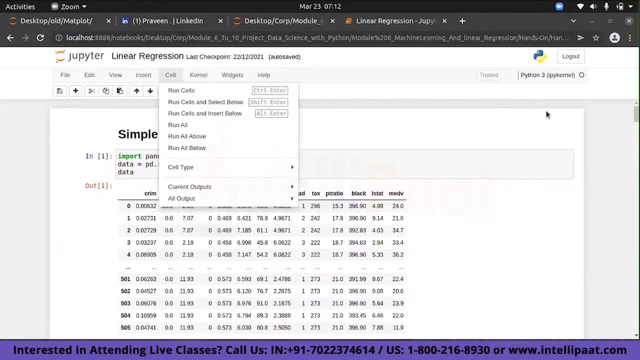 iit midras advanced data science and ai certification program. this course is of very high quality and cost effective, as it is taught by iit professors and industry experts. fine, have較a. let's check this out now. let's say that you will get a bit of a. 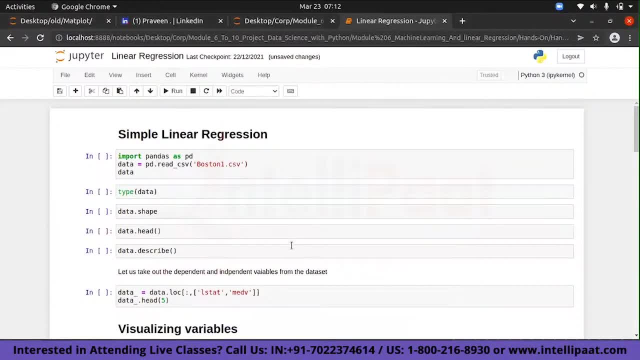 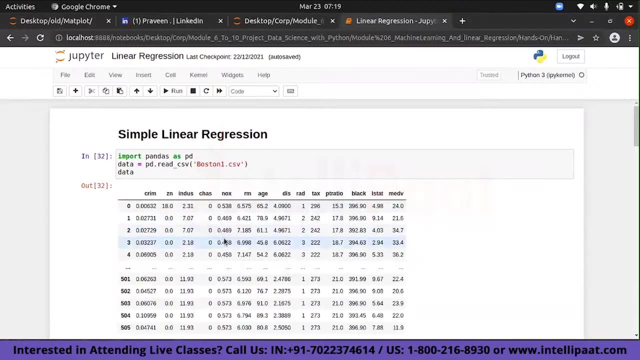 problem and then, step by step, like how we used to build, we'll try to build the linear regression. i'll explain what is the data set and we will see. we will use this data for our analysis today. done, very nice, fine, so everyone, all of you, are able to. 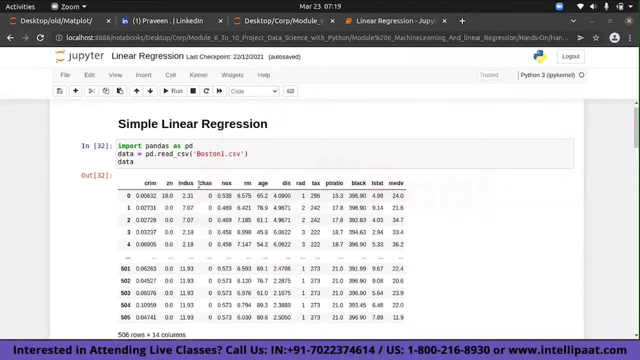 read this and see this. we'll go into the data now so you're able to read it, no issues. so now, uh, this is just for you to uh understand. i'm just giving you. so you have something called as a washten data set, right? so this is nothing but, uh data set. 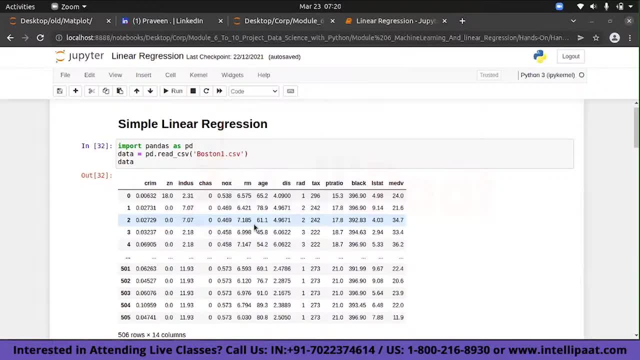 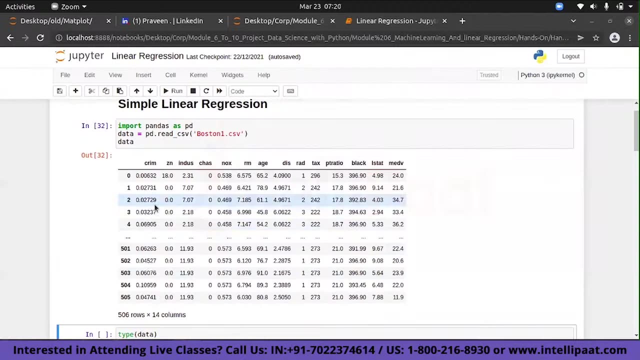 contain information collected by a us body about the house and everything. so it has like around 14 attributes. so you are seeing this here: 14 columns. so what are these columns? so, basically, whenever you take a data right, you will not understand all these details, okay, so 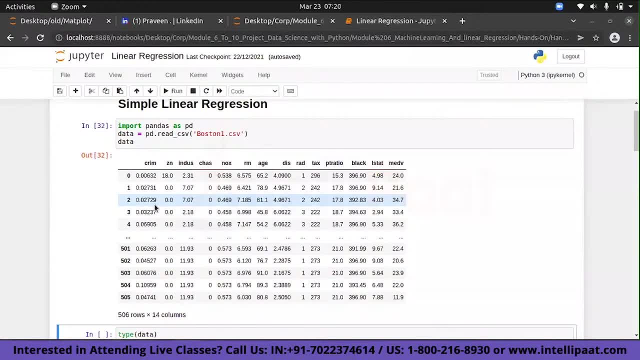 basically what it contains is like some of the information about the housing data, right? so your jupiter location you can find here. so if you open here, this is your jupiter location. so where your jupiter location is. so this is your jupiter location. so this is your jupiter location, so 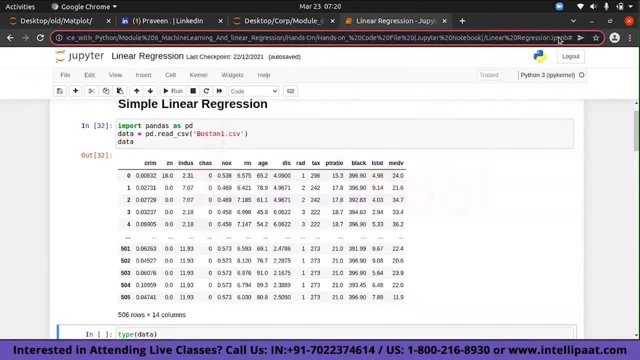 jupiter is. so try to keep it in this folder. you can see, mine is machine learning, linear regression, hands-on hands-on code, linear regression. so in this folder you have to keep it, so wherever your current file is there. there it's just the this thing in a browser. just click that and then you'll. 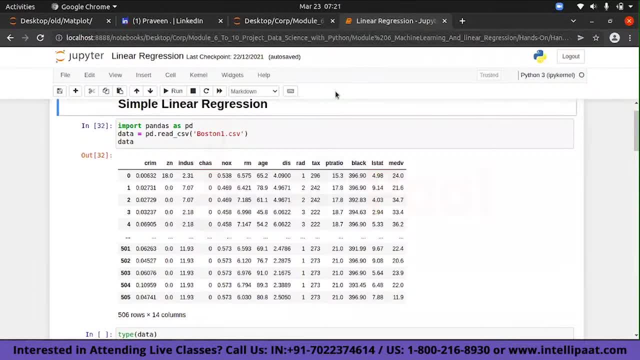 be able to get it right. so it's in the browser. it will show in the top now. so i will go ahead and then i will tell you slowly. david, try uh in case, if you're not getting no worries, so you can follow this and later you can uh read it from the recording. 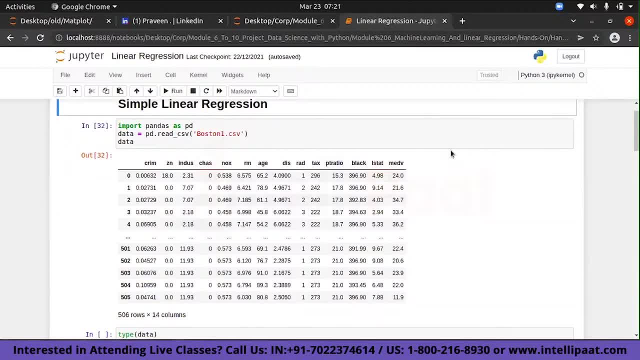 whatever. we have showed how to read the document and all and practice, so don't worry. so we'll help you. no issues, right so, but please try right now. if you can read, it will be great. so now, what i am trying to tell you is there are 14 variables. i will explain each one of them, right so, whenever. 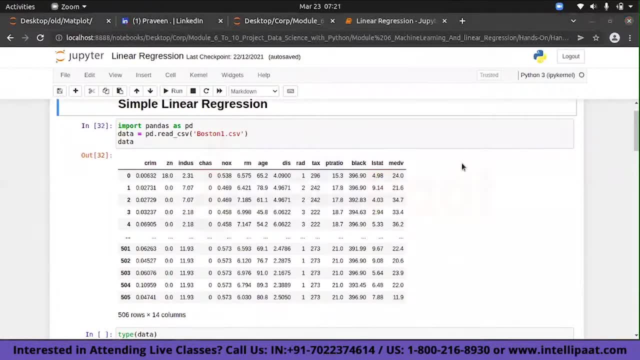 you get a data, what happens is you may not know all the variables. so understanding the variables is very important, right? so you have something called a scrim, you have something called a zn, you have something called as index, you have something called as- like indus, cas, nox, rm. so what are these we need to understand so that we get a idea like: 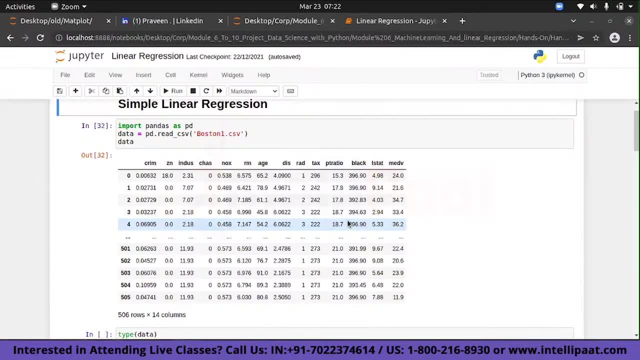 what is the main thing that is driving what we want to find right. so now the first one: crim means per capita crime rate. so crim means per capita crime rate. so what is the crime rate? so obviously, if crime rate is high, then the price of the house in that locality. 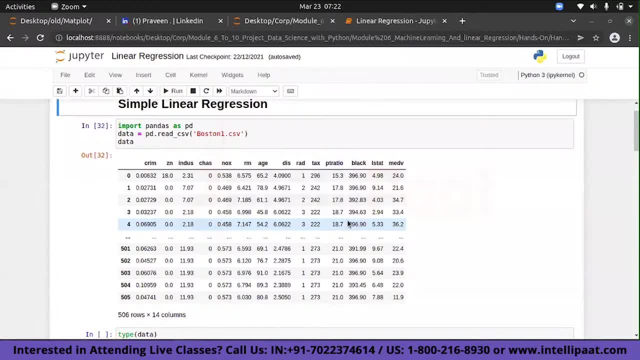 is less correct. no one wants to be in a place where crime rate is high, agree, all of you so, which means it's like a negative correlated variable. so you will. you'll get an understanding that, okay, one variable and then another variable, and then another variable and then another variable. 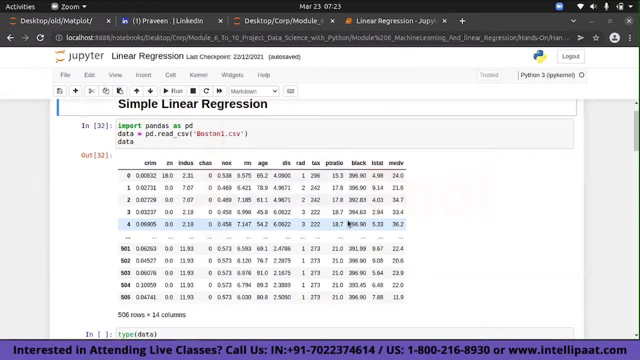 you understood. now you have zn. so zn is nothing but proportion of the residential land zoned for lots over 25 000 square feet approximately. that is the zone, which means in that zone what is the land for lots so? which means government is doing some kind of activity there. 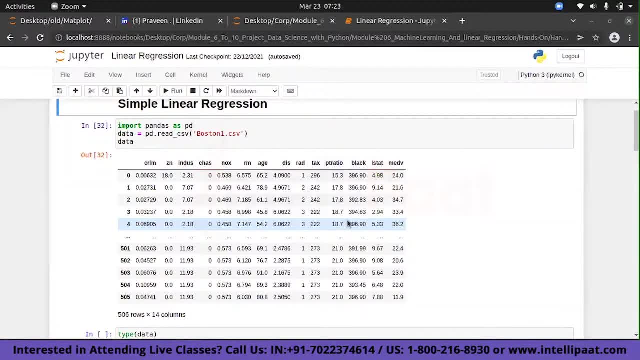 so that is also one variable, that is there: zn so, which means zoned right for some zone. they are taking some thing, let's say. let's say for example, for an it park or maybe for some bus station or maybe for some college or something: government is zoned right for some. 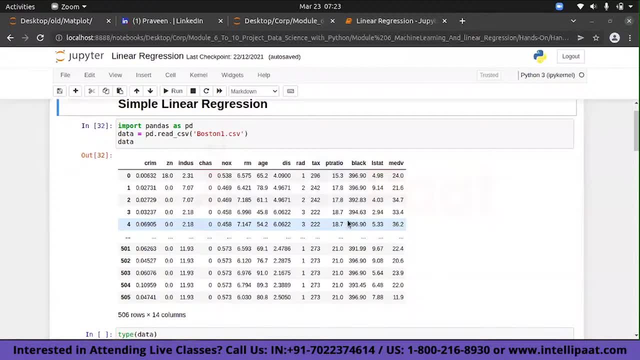 purpose. that is zn. how much, how many? uh, what is the area that is zoned? that is something. now you have something called as indus. so indus is nothing but proportion of non-retail business acres per town, which means, let us say, if you take a town, how many acres is non-retail business? 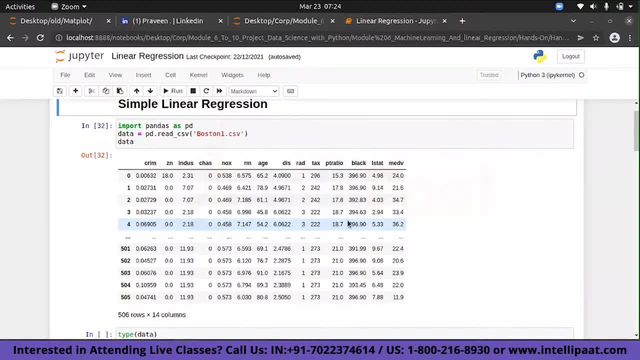 area, which means more the business area, better will be the price. so that is variable. some people don't want to stay in business area, some people want to stay outside. so that is also depending. so what is it? so, indus is some one variable. now you have chas, so what is chas? 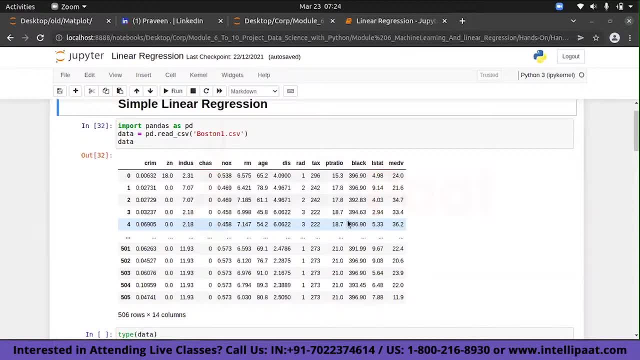 chas is nothing. but there is a river which is called charles river. so charles river one. if river is bound, which means if the river is passing near your house, if you have a good view, if it's zero, which means river is not passing by your house, so that is chas, then i have nox. 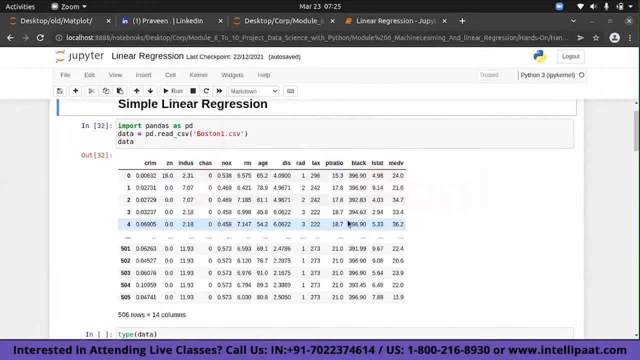 nox is nothing but nitric oxide concentration, right? so parts per 10 million. now tell me nitric oxide concentration, nox, is it a positive one or a negative one? so when nitric oxide is more, your price of house will be more or it will be less. 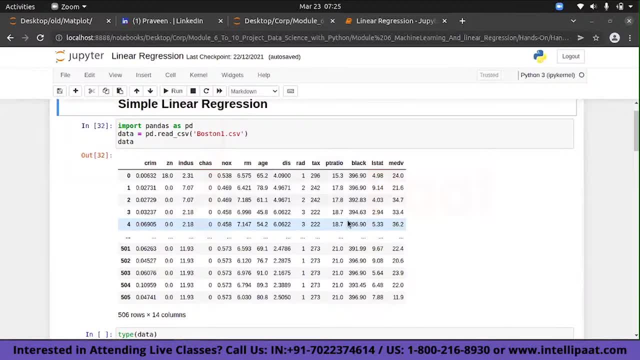 price will be less. no one wants to stay in nitric oxide location, correct, cool. so now rm. so rm is nothing. but yeah, river view depends on flooding, so there are so many things that are influencing, as you rightly say. now rm is nothing but average room, average number of rooms per dwelling. so what is average number? 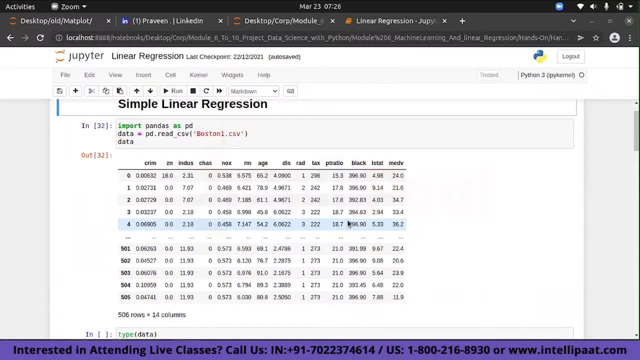 of rooms per dwelling, which means, let us say, let us say you have a location in that, what are the average number of rooms that are there for every house? so that is rm. then age is nothing but proportion of. uh, there are two things. okay, age, if you can see, 65, 78, all these things are there. 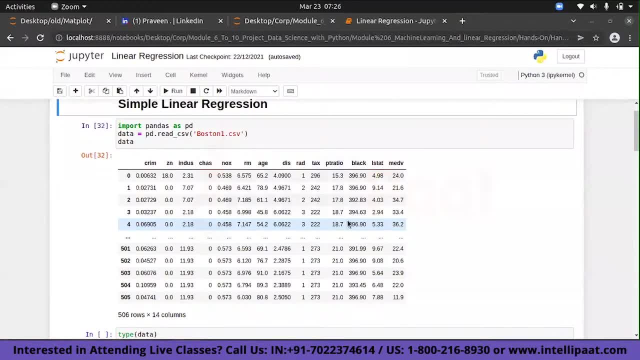 so what is the age of the building? so that is your age. so basically, more the age, let's say the price. this means weighted distance to the employment centers. so this means how, how far is it from a tech park? so to be simple, so that is your, how far is it from tech park? and then rad means 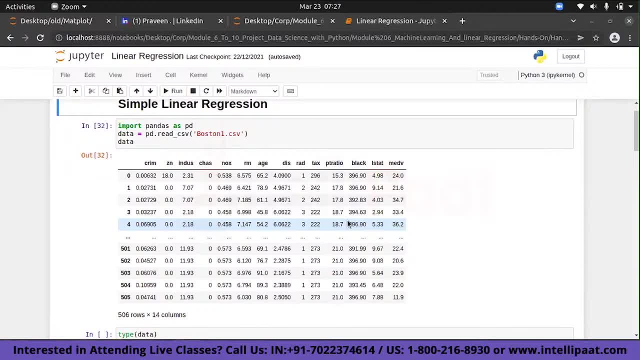 accessibility to highways. how many highways are there? so this is the age of the building, so that is how many highways are near to that location? one, two, three, so nothing like that, right? so that is. these are some things that you need to know now. tax is nothing but the property tax. what is the 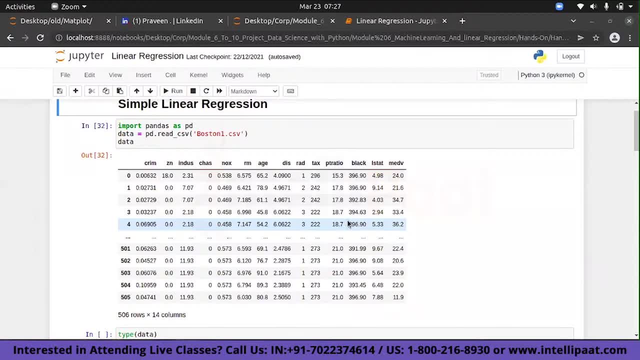 value of property tax. uh, that is in thousands. so that is something they have given and later i have pt ratio. what is pt ratio? pt ratio is nothing but nearby my house. how many schools? what is the uh pupil and teacher ratio by town? right? so there are five, five, not five towns, and you have what is. 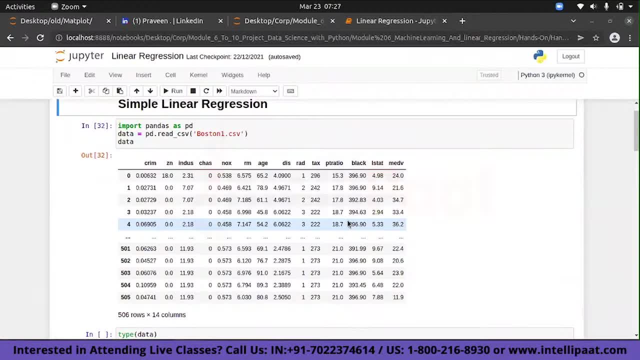 the people, pupil and teacher ratio. so if someone wants to go to school, so that is something, and i have something called as a black right. so black is nothing but the proportion of people from african origin. what is the percentage? so what is the number of people? so what is the? uh? what do you? 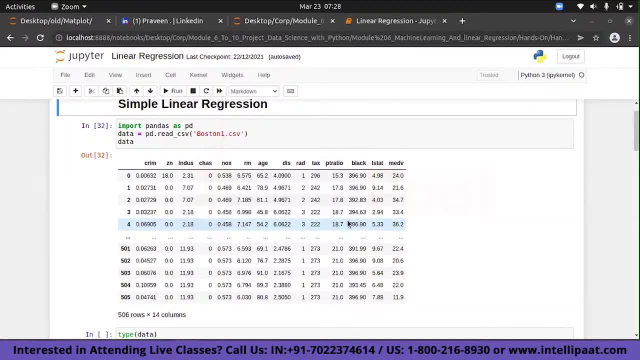 like proportion of the place owned by african origin people. so that is black ls stat percentage, which means what is the percentage of lower status people. so in the complete community, last but not the least, you have m e d v. so m e d v is nothing but the value of the property. 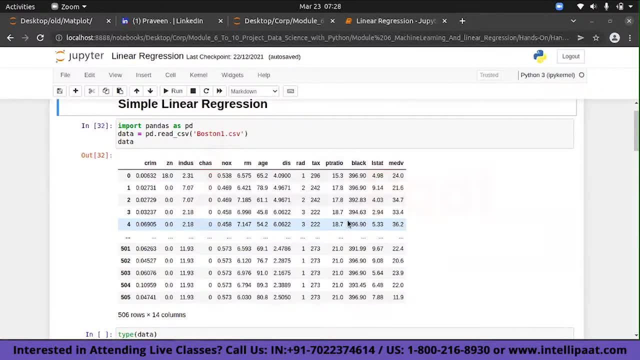 in thousands. so the value of property in thousands. so this is the data in this. if you want to predict the price, which is your dependent variable, can someone tell me which is the which is the dependent variable? i mean, what is your target, what you are trying to find? i told every variable: no, m, e, d, v, which is the 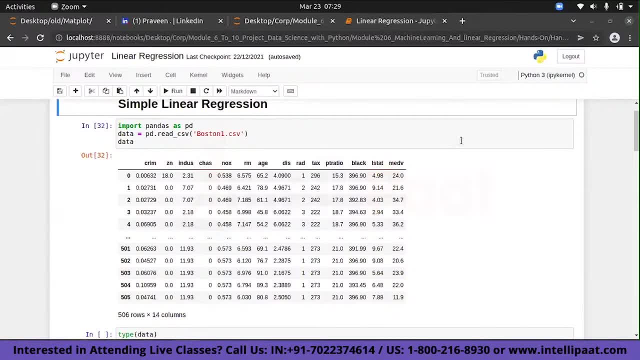 median value. some other, all other than median, are independent variables. m e d v is dependent variable. i think just the confusion you got right. so dependent variable is dependent on all others, so price is dependent on all others. so that is something that you need to remember. so m e d v is something which we are going ahead and then 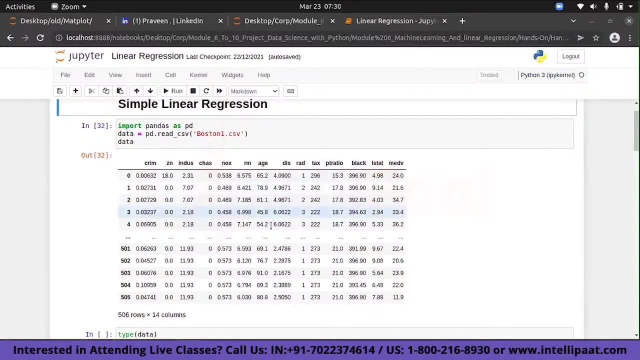 finding our problem right now. we understood the data, so this is a preliminary step that you are supposed to do: read and then see the data. then you will get a fairly good idea about how exactly you are going to deal with it, right? so this is something that we saw. now, once we are completed with this, i just want you to 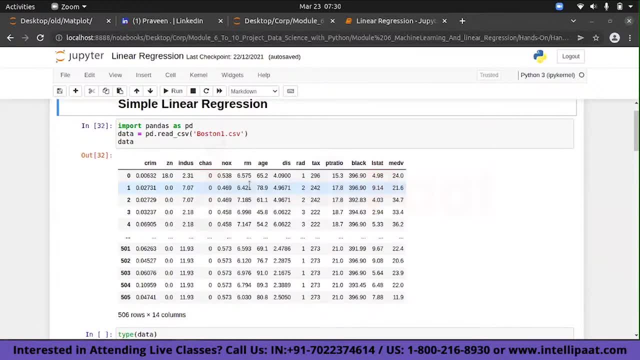 basically understand the data. so data understanding creates a very good. uh, what do you say? if you understand the data well, then model creation will be easy. without understanding the data, creating a model will be a little challenging. but if you understand the data well, then you will be challenging. right? so you don't know what are all your variables, how they are functioning. 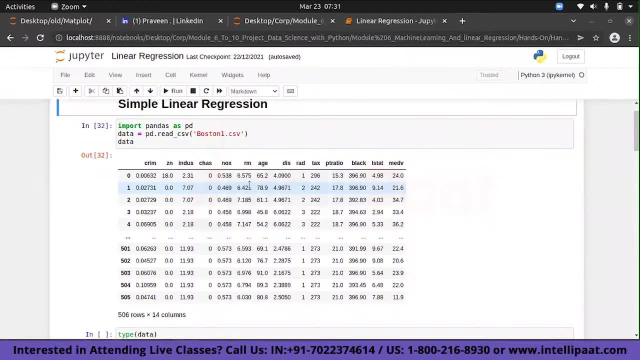 and all that, but this is how you get started. now, once you understand all these variables, what are you going to do next? so the next step that we are going to do is: we will see, explore the data. so all of you know, right. so how are we going to explore the data? 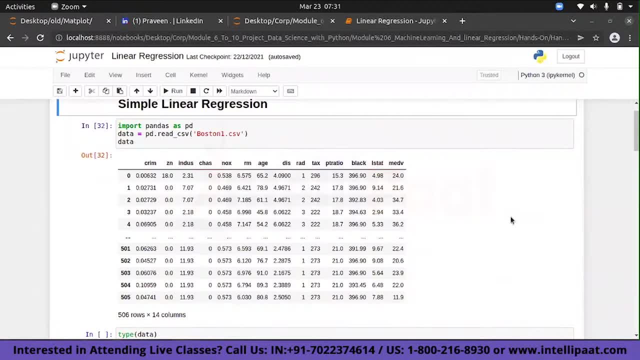 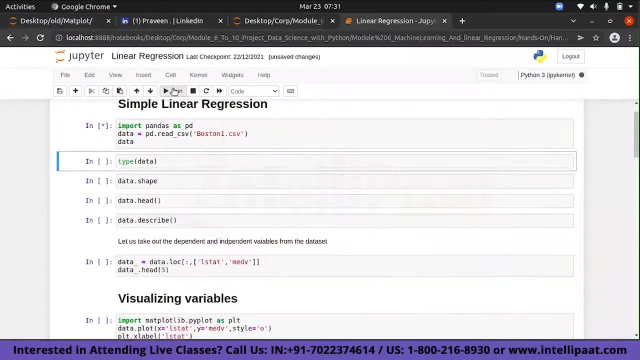 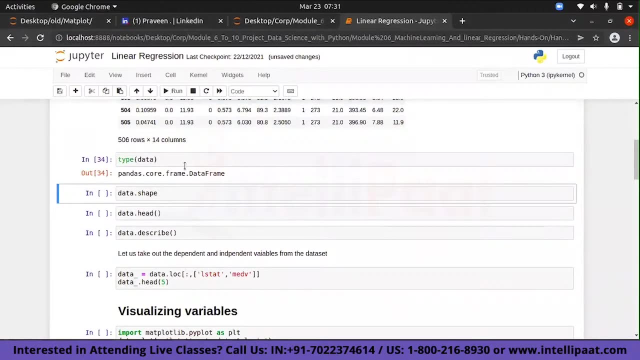 so basically we do all our describe info and all of that right. so you saw this correct. so we will go ahead and then do the describe info and all other things. so you can see, i'm just checking the data type. so this is data frame, so shape will give me what. so, basically, 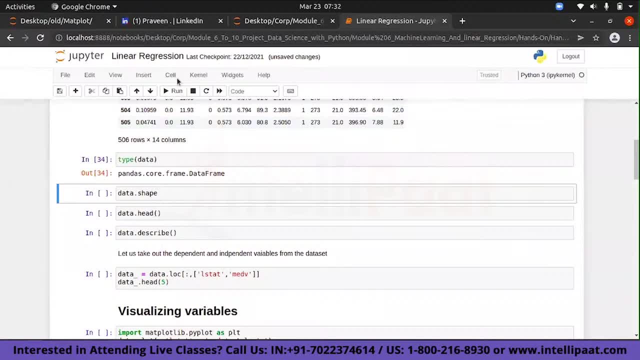 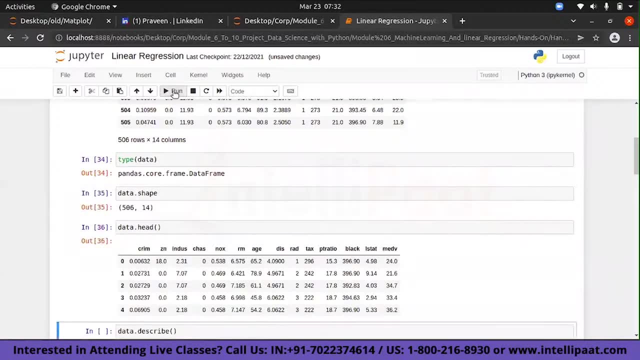 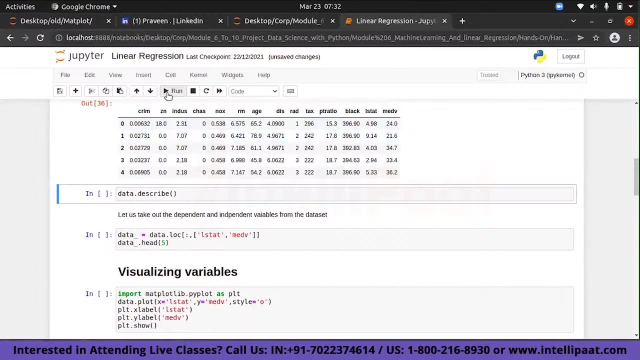 506 into 14. so rows and columns correct. so just understanding how many rows, how many columns are there, i got it. so data that head, all of you know. now i'm just taking to data dot describe. so this describe will give you a basic statistical summary. so, main thing, what you're supposed to look. 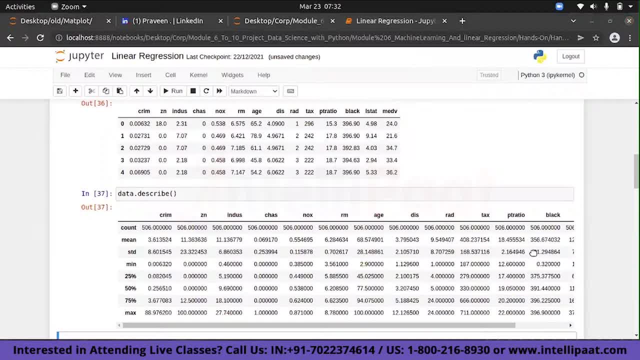 here in describe one important thing. you should look what is it first thing. when you do a describe, no before mean also no. so whenever you do a, describe, your first thing first check is the first line. see, all the columns are having five, not six, exactly. so now what is the conclusion? 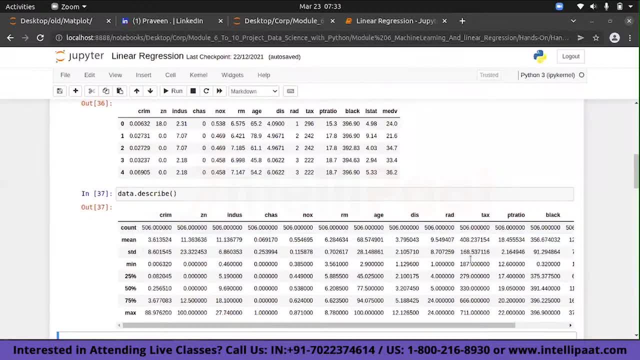 our end describe. so what is the conclusion? so, which means no null values. there is no need for you to replace any null values, correct, exactly. so this is something that you need to understand right now. so this is this is the first step. once you understand this data dot describe. 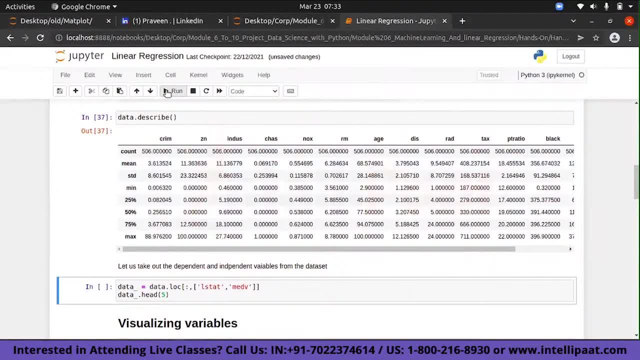 what we are going to do is we will take two data points, so one is my l stat. so what is l stat? i told you. if you can recall what is l stat means, what that means. right, we also give the yes to function. do at least in g as well. 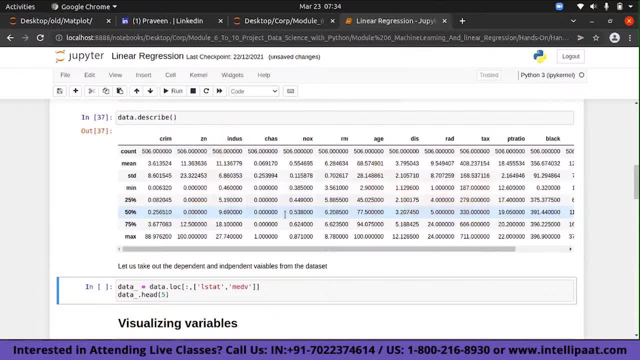 so here, the logic was that for it to create these columns- and you need one of these columns- you need a type. so typically, in that case, a little bit of it is inside c is actually there, c indeed you need one, two c which is internationally closed. you need some analytic. 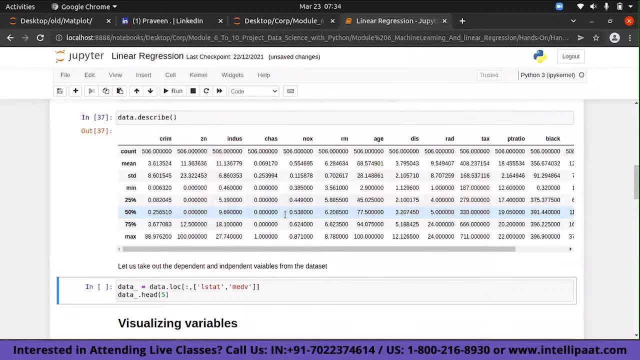 tubularvé, because this is bicycle and this would put a text- and if you just want to put it as something門 equal to 20, that would be good- theふé down a little bit. this means that at the origin of the variable j, ether- this is the operating method you can kind of 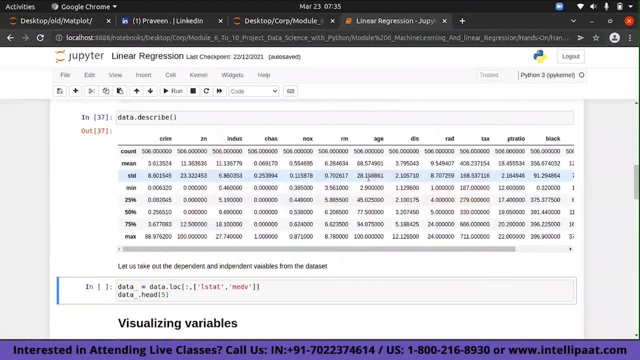 make this. so if we were keep numbers for minus r three, this would be like a correct statement, like all right. so now here enter the section queen of those people in g: the value of value of madmu. the 14 variables: i am selecting one independent and one dependent variable, correct? so i'm just. 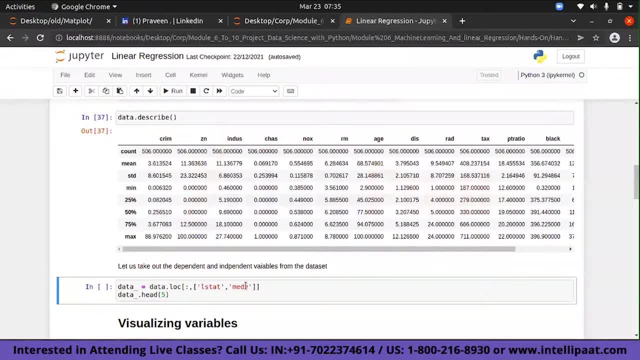 taking one independent and one dependent variable, so which was like an example that we have right. so whenever you have such single independent variable and single dependent variable, it is a simple linear regression. so this is something that we are supposed to do. so what we understood from data 37 is right, so we are supposed to check this count. 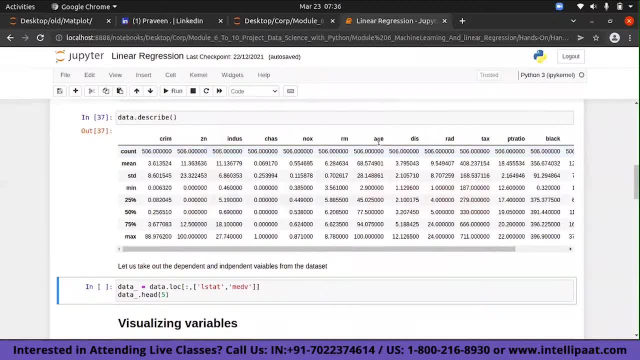 so if the count is same, which means we don't have any missing values, so that is the easiest way to find the missing values using describe. so that is the outcome that we are supposed to see, right, just observe here. so the data has multiple columns, but we are just selecting two here to start with. 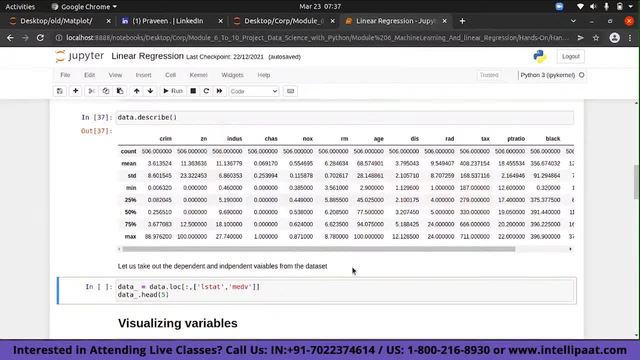 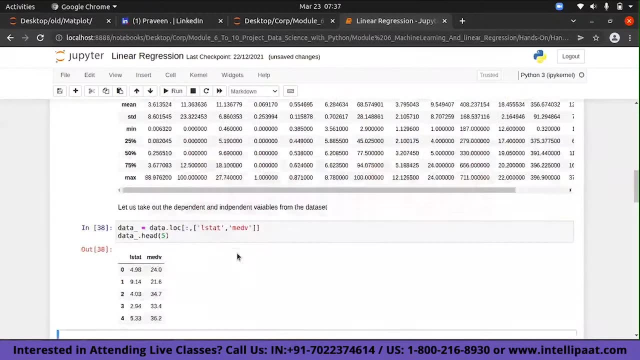 so that is why i am telling it is simple, linear, to start. you can see we are just taking two of them to start with, so let us see how it works. so that is the objective. we are not taking all of them, we are just taking one and checking it starting. so this is a simple linear regression. so you have it. 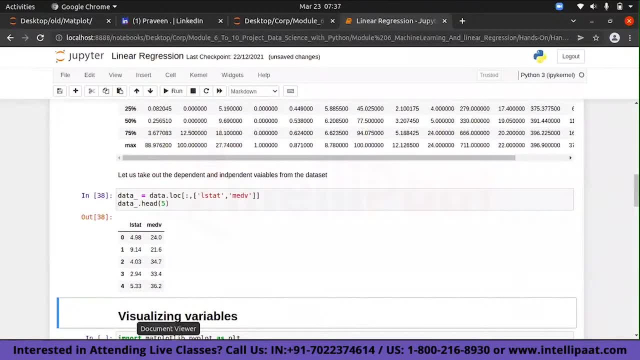 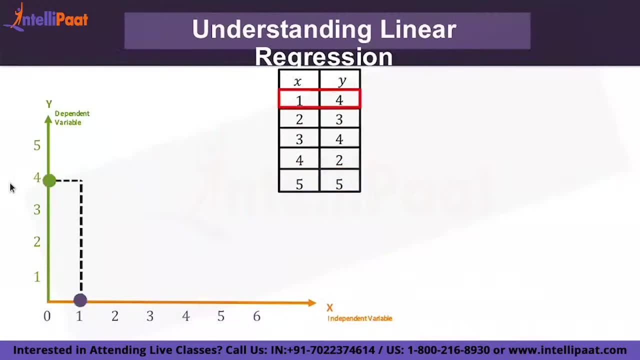 now all of you know right. so in the ppt also you had a similar data. so if you can observe, okay, you also you had the same kind of data. you can see you started with two variables like this: x and y, one, two, three, four, five and here. but 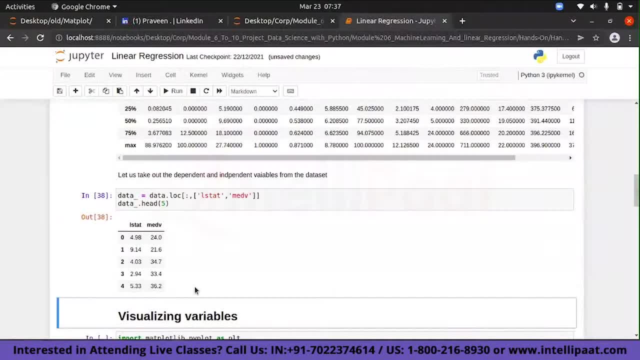 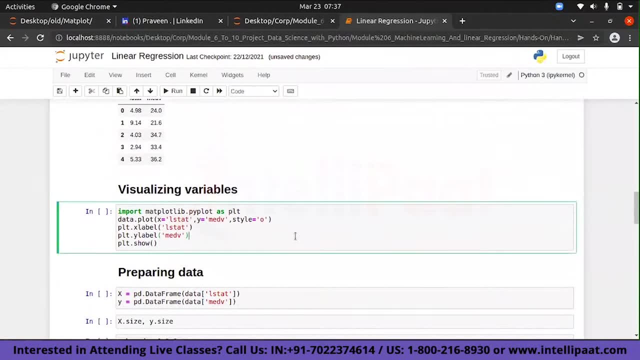 the only difference here is, instead of five variables, you are having around 500 variables. that's all now. first thing, what we did, we supported to plot. now i'll ask you one question here. this is all you know, so you're already done. data, dot, plot, x, y style, all these things is there now. 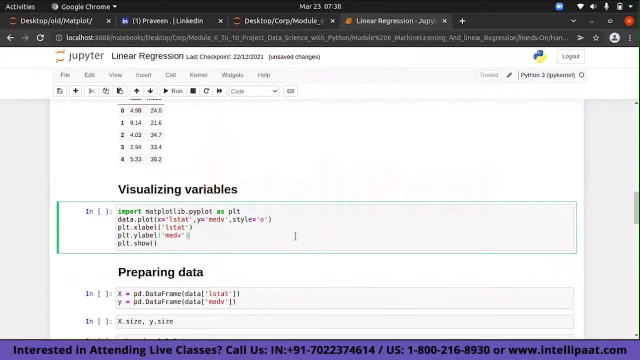 what kind of plot will come? bar graph- scatter, plot area graph. what will come of? you have done it already in matplotlib. i think i only have taught you. tell me what plot will come in this. are you sure i have not mentioned bar anyway, for bar we need to give bar or bar h. 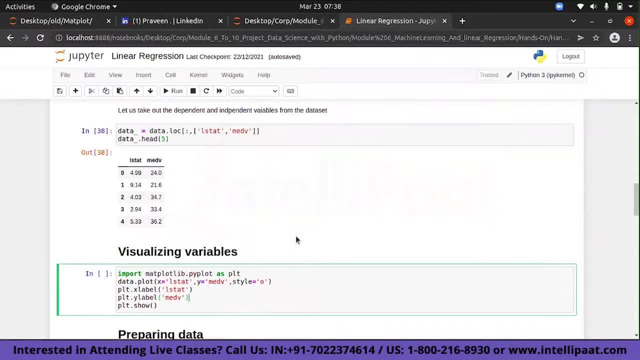 so line also. i have not given. so line means okay, fine, uh, okay, you may think it's line, okay fine, i agree. okay, few people think it's line, few people think it's scatter, okay, fine. so why am i not telling you that you can plot a line graph? because you can see both of them are continuous. so if both the 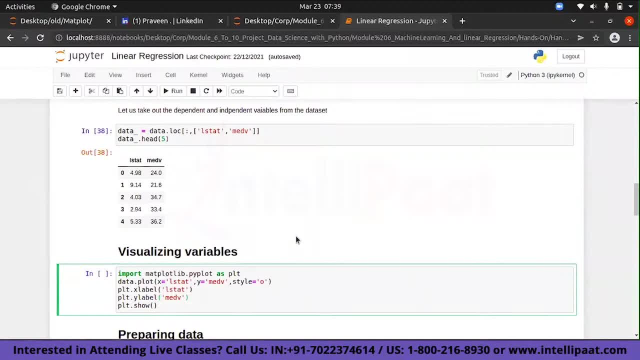 x and y are continuous. do you think you can plot a line graph? at least x should be discrete. no, for one. what is the value of y? for two, what is the value of y? so if you have like that, at least you can plot a line. but both of them are continuous. you don't know what point comes where. so do you? 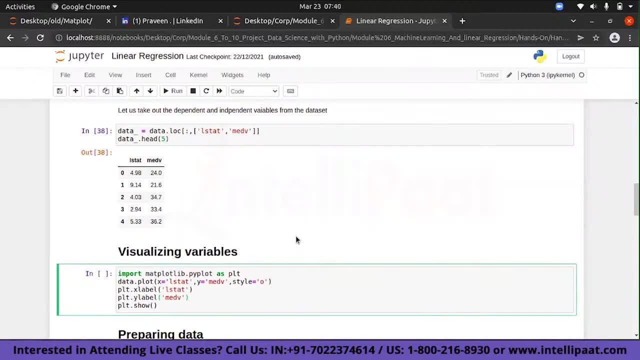 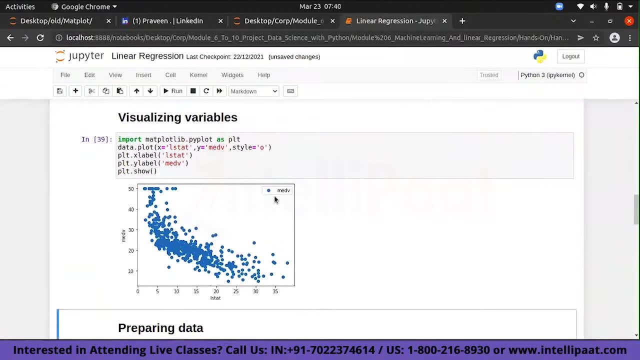 think line graph is possible. think and tell me, is it line or scatter? again, scatter, correct. so once you run this, you can see you will get a scatter plot. all of you are able to understand this. it has a legend, it has l stat, it has mdev. so all these things cool, are we fine? okay, yes, so you. 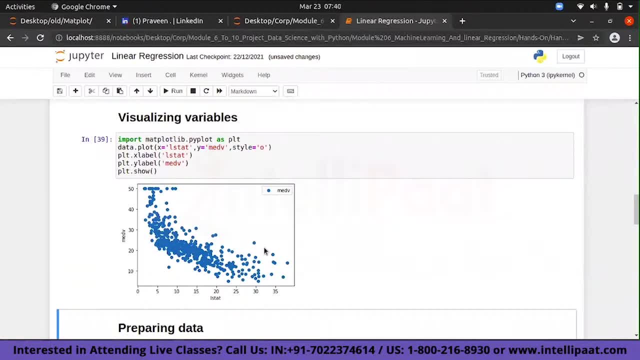 people are understanding. so what is the line? right, how it goes? is it positive or negative? you take some time try to type it, so we need to type the code as right. so slowly you type, no issues, i mean, if you're not typing. also, typing is only for practice, right, so it is negative. 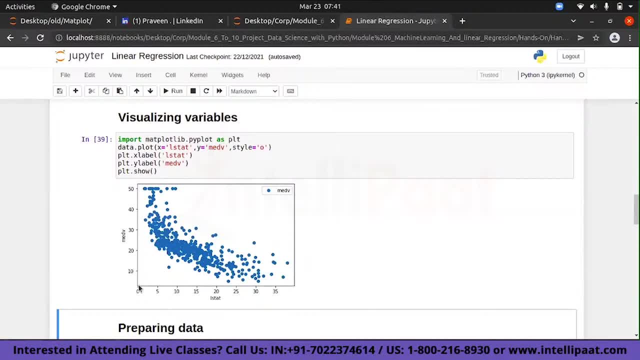 correlation correct. fine, so there is no reason. see, your x value is continuous, y value is also continuous. so if you want a line graph, you should get. for 5 it should be 30, for 10 it should be 40, for 15 it should be 20.. so some kind of variable should be there so that you can connect them and 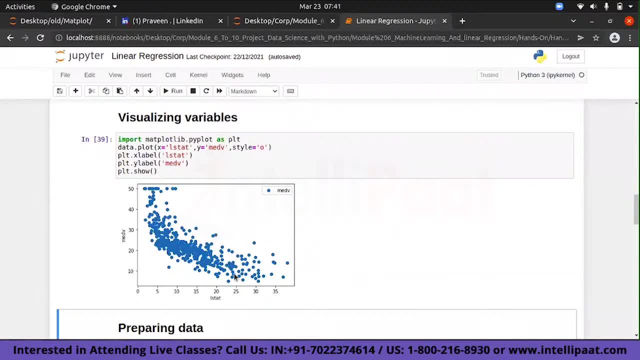 make a line graph. you can also make a line graph here like this bar plot, but that doesn't look good, so that is why it is a scatter cool, so all of you are able to understand this. so let's go ahead and see if you are able to type till here and then get it. anyone having any issues? so this graph is. 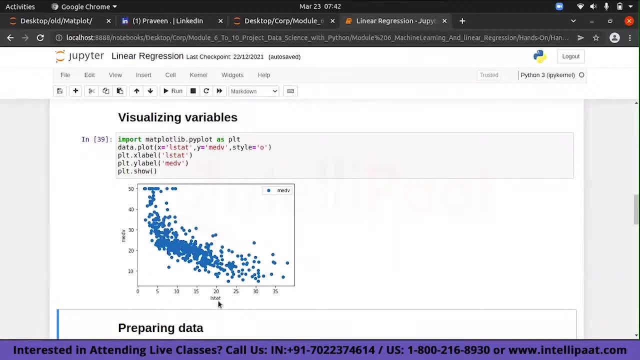 nothing but a comparison of your. the people who are having it will run without subplot. also, you're just plotting something, that's it so. data plot labels. i'm using three components, that's it right. so i have lstat and emdev. so what happens? the number of people, uh, which means in a given 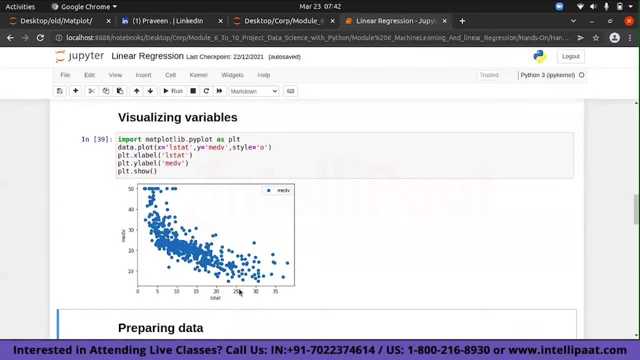 location. more the number of people, lower financial stability or probably lower financial status, lesser will be the price. as the number of people with lower financial stability increases, the price will come down of the house. understood by default. it is correct, no issues. you can. you can watch and then you can. 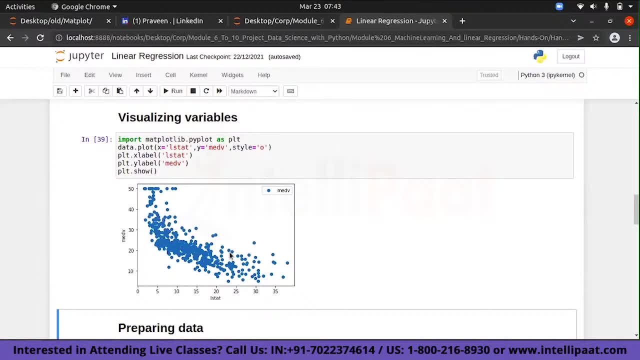 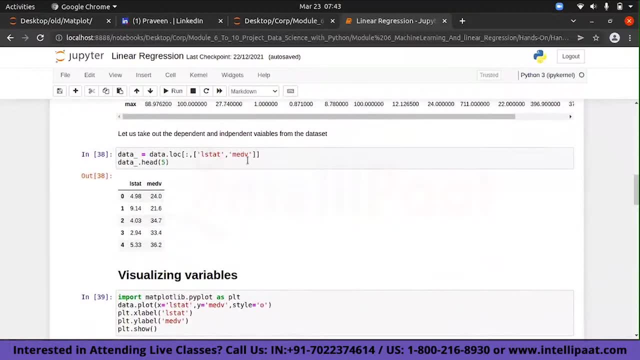 practice later. anyway, this is, this is something, uh, that we are going to so, basically, the comparison between two variables. you took two variables for a initial linear regression, correct? so you know what is lstat- the number of people with lower financial status- and you know what is the price of the house. so, if the colony or if the location, 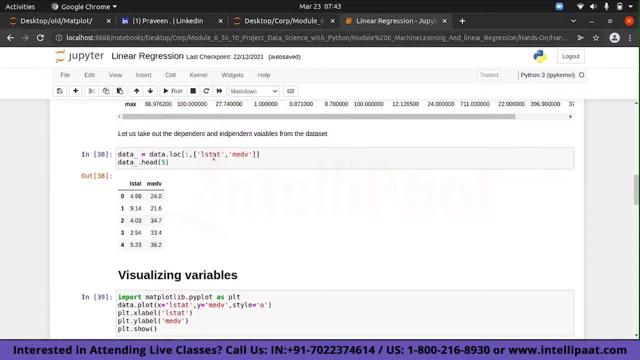 has more people whose financial status is less, the house price also will be less correct. it is not a very fast area or a rich area. it's a low financial status area. so that is what we are seeing here. so you can see lstat whenever you have. 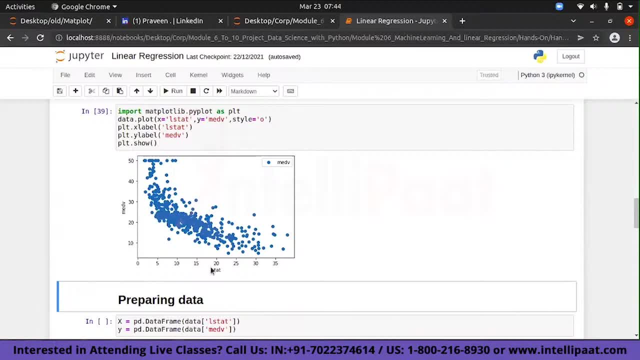 the number of people with lesser financial status increasing, then the mean value of the house price also increases. lesser the low financial status people, more will be the house which price, which means it's a rich location. so if the number of people are more or locations are more, then the 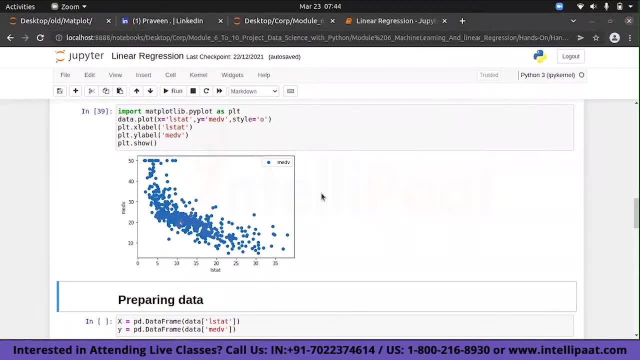 house price will drop. is this clear to all of you? cool. so till here it is. now there are some assumptions in linear regression- linear regression which i have not covered, but i'm just stating it to you. so those assumptions correct: if the lower status people are high, then price is less. no, where price is high, l stat is. 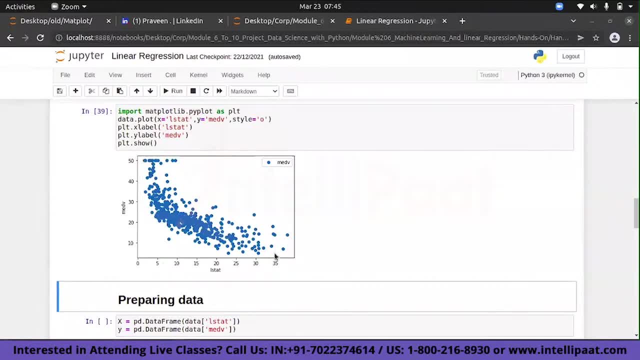 less, which means less people, then price is high here. more people, then price is less. people with low financial status will not take the house price higher. that will become a medium society. it's not a rich society. for the price to become high right now, don't you think you can get a linear 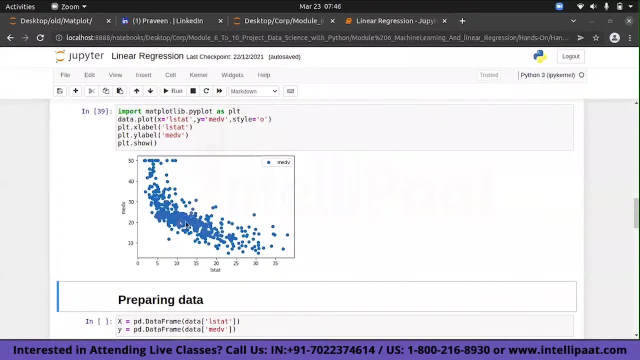 relationship between l stat and m correct, so you can get a linear relationship. if 35 people are there, then you will get house at 10 million dollars. if five people are there with less financial status, then your house is 50 million dollars, which means you are in a rich location. 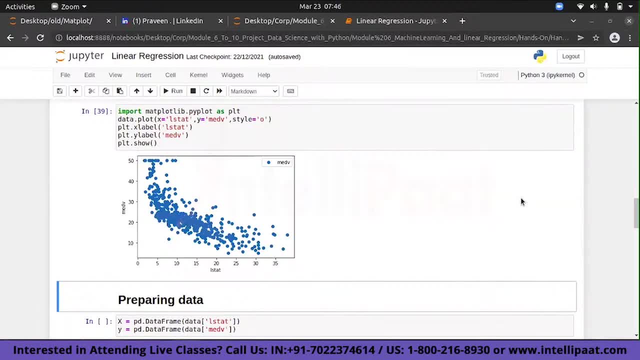 if more low finance people, then you are in a moderate location, right, thanks. so now you're going to, you're going to plot a line or whatever it is, so you are going to find a linear relationship between this right. so this is a percentage, krishna. so now what we are going to do here is we will just go. 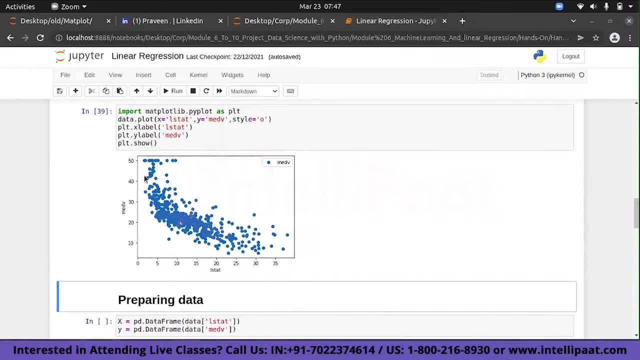 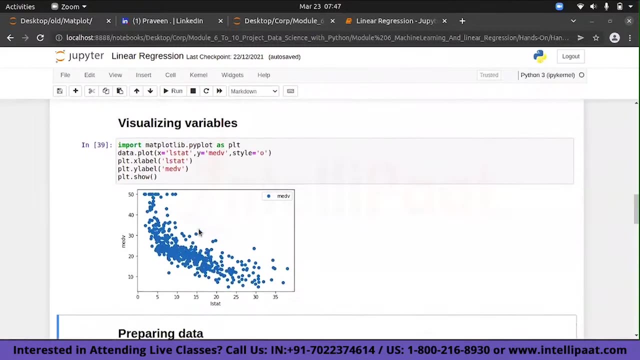 ahead and then see how we are going to get a relationship between this, how our relationship comes right. so, if you can see this, there is a line that comes right. so there's a line that comes. how to find that line, all of that we will see. now what is the next step once you do this? here you have x and y. so what is the next step? can someone guess and tell me? 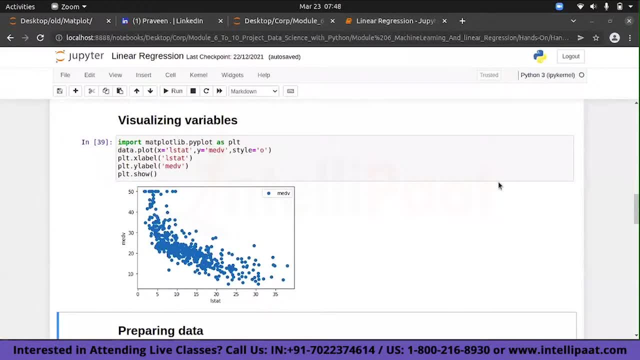 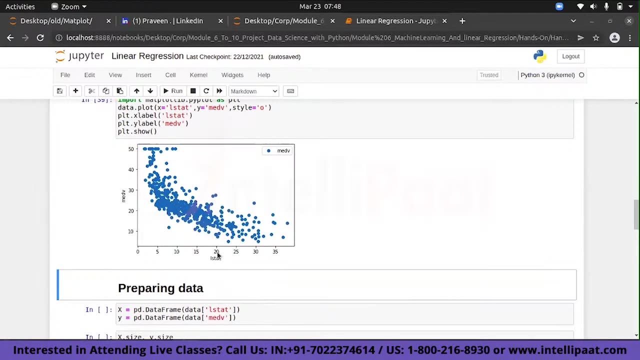 find mean. okay, before that, before finding mean and all that, what we are supposed to do. so, like I will go step by step. okay, we'll go step by step and then we will see right. so the first step is you need to identify what is your x and y correct out of these two? x is l stat, y is m dev, because 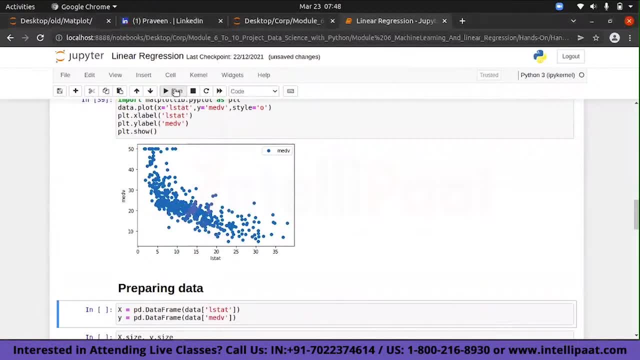 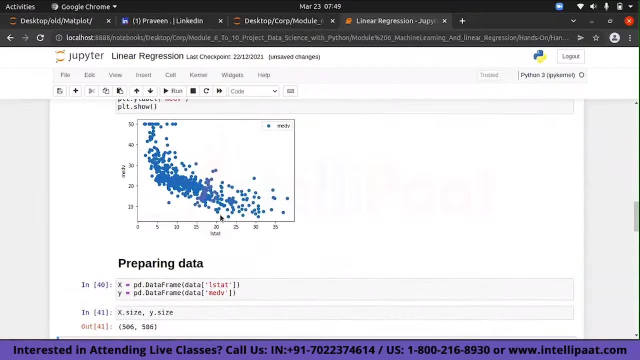 is dependent on l stand. so i'm just preparing my data accordingly. i'm taking x and y, i'm just checking, so try to do it till here. all of you are done. just check right. so some assumptions are there in linear regression, so which means the data should be linearly related. so if it is like 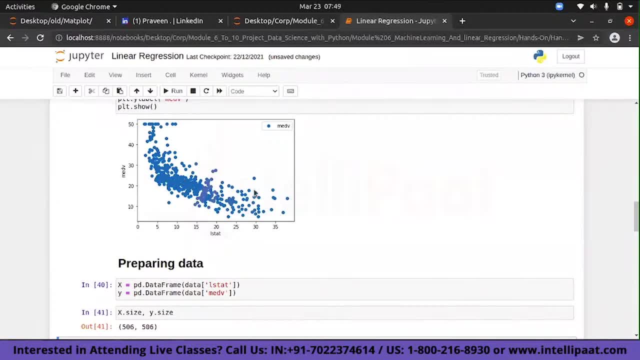 scattered all around, then you can't do a linear regression. the first assumption is the dependent variables, and independent variables should have a linear relationship, which means you should be able to fit a line. that is one assumption. so there are two, three assumptions: more multicollinearity. 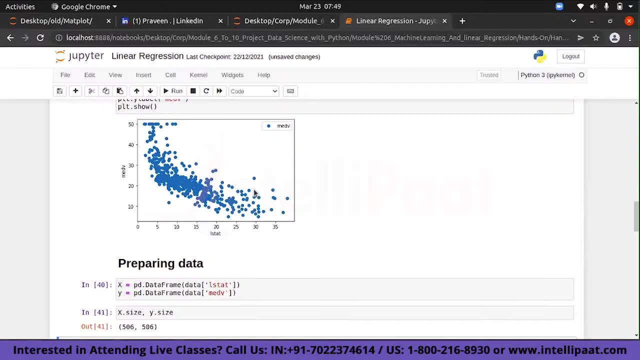 and also you have something called as constant error variance, which is called homoscedasticity, and all which not going to cover right now. it's not part of the course that is there, but i'm just, i'm just telling you these things are also there, so you have some assumptions, which needs to be. 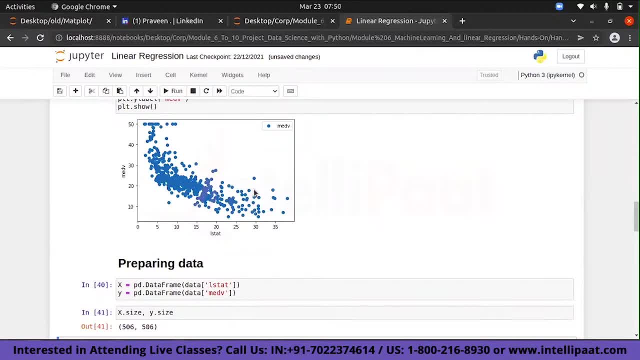 taken care, but for initial version and initial learning, this is sufficient so you can go to the next level and then you'll be able to understand them in detail. so that is something that i can probably tell you. so i'm just giving you a precursor. so i'm just giving you a precursor and then i'm just uh. 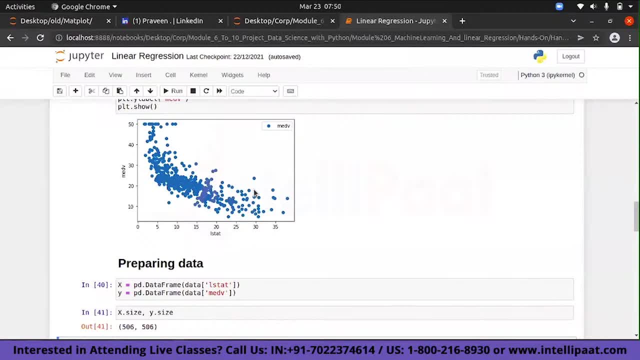 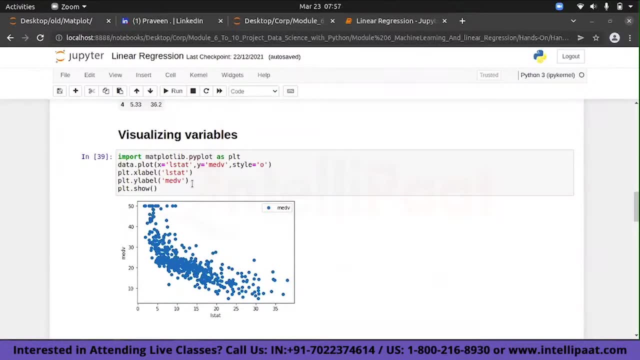 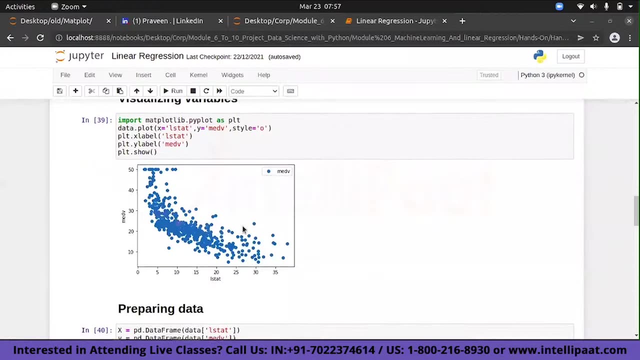 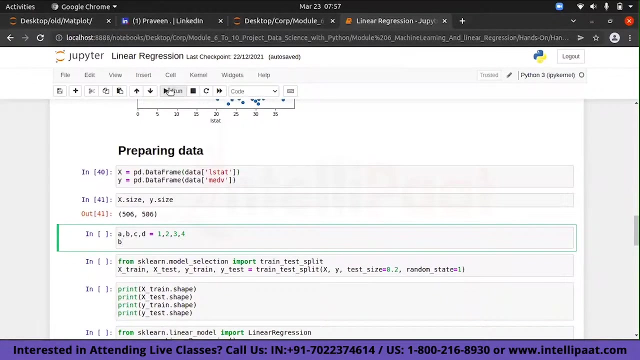 telling you about this, right? so this is something that i'm going to tell you, all right. so this is basically our dished plot. now, having said this, what we are going to do is this: is o, not zero. once you complete the visualization, we are preparing the data. you took what is x, y, and then you did it, and don't worry about this abc, this one, just i've. 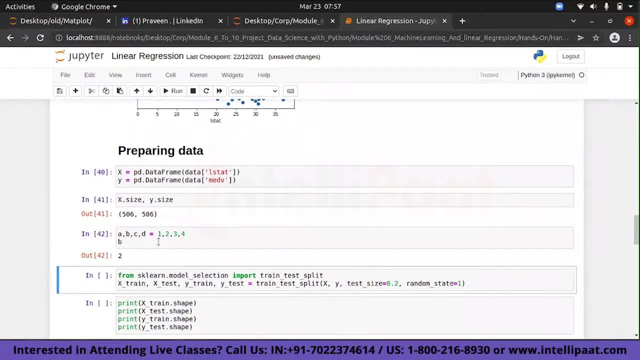 just done assignment. just to explain, if you do any assignment like this, a will get one, b will get two, c will get three, d will get four. correct, so this is how assignment happens. order. why i'm trying to tell you this is because whenever you do a, 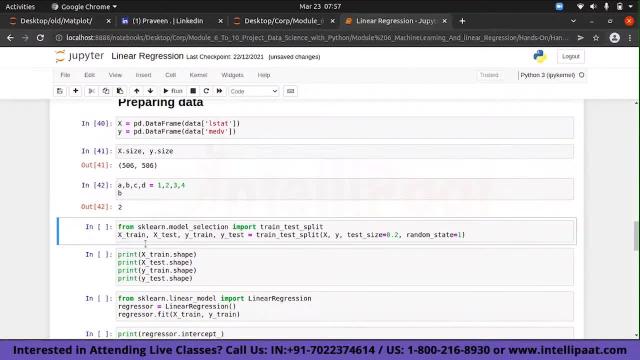 skill and model selection. import: train test split. here you give x train, x test, y train, y test. so this order should be maintained. if you miss this order your variables would get jumbled. the output of train test split will come in this order only. first will be x train, then will be x test, then 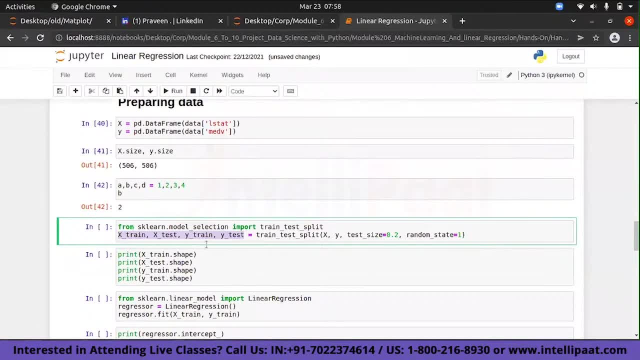 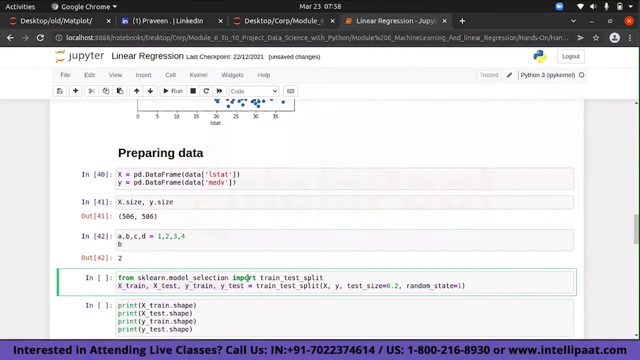 will be y train, then will be y test. so this is the order in which your output will come. so please ensure that this order is maintained. so to explain that, i have given you abcd example, so i want you to just go ahead and then complete till here. so once you are done, just let me know and then we will see how it works, right. 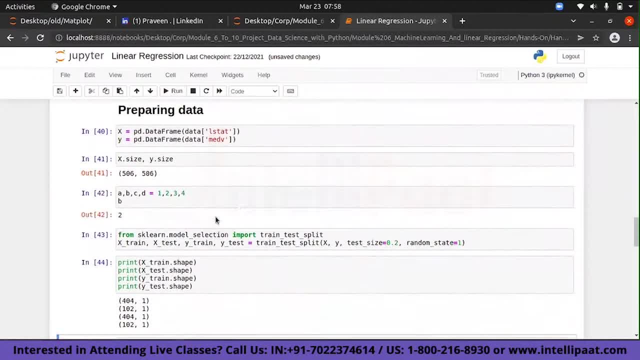 so i just want to see it how you are going to do it. so split this and then we will see simple linear regression. we will practice, and multiple linear regression also. i will explain it to you. so it is: it is similar to multiple, but usually what happens? you will always not have a. 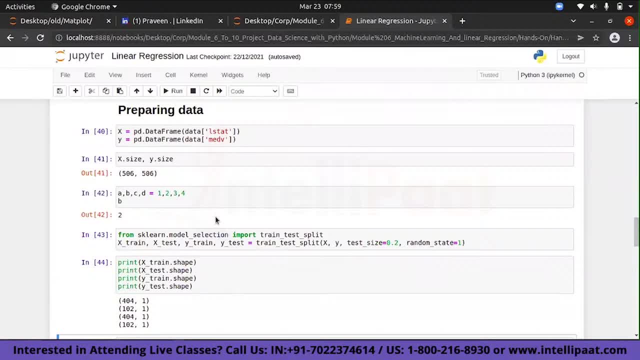 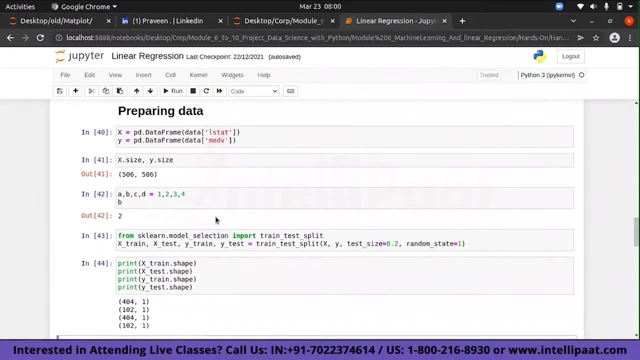 simple linear regression, so you may have multiple linear regression also. so that is the reason i'll explain you multiple linear regression as well. we will work on. so all of you done till here, done. okay enough, just see how exactly it works. is you can just see this? okay, i have something. 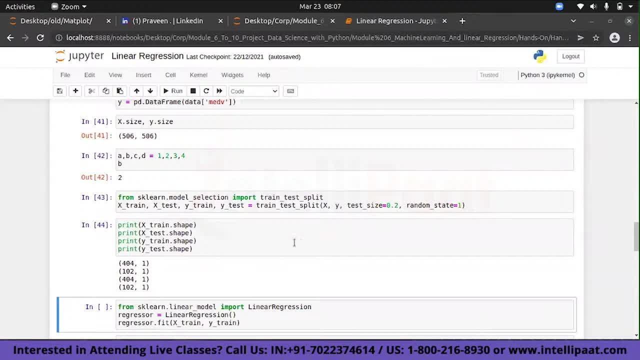 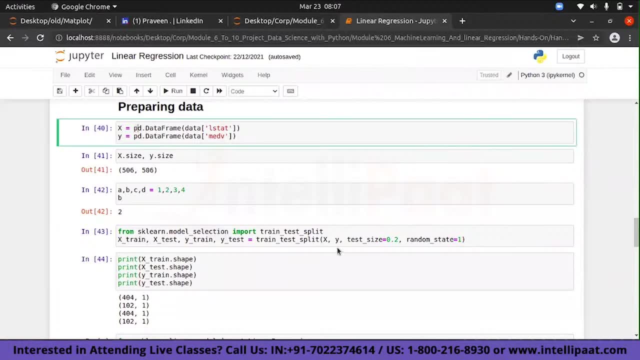 called a strain test split. so how this function works is: you're having your x value, so what is the x value else time? so you took your x value. here you have y value, so y value is now the y value is but m dev. so basically you have a x value and also y value. so x and y is there now what you? 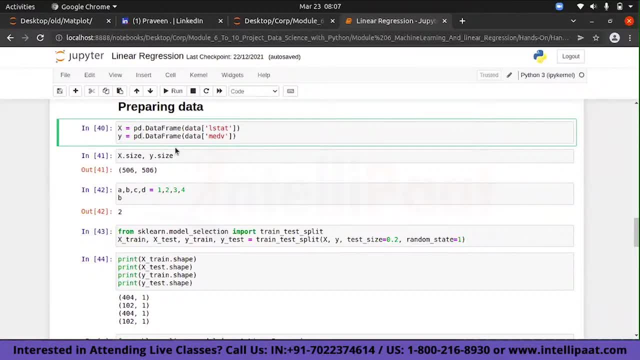 are trying to do is you are splitting your x into x train and x test. you are splitting your y into y train and y test. so what is the proportion that you are splitting? so the first two arguments in train test split the first two arguments is your x and y. so the order you need to follow x train. 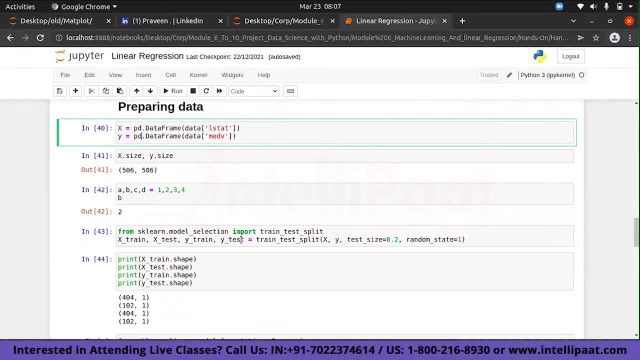 x test, y, train y test. so this is the order you need to follow. then train test split: the first one is x, second one is y, x and y, and later you need to define either a train size or a test size. so here i'm defining the test size. so what does test size mean? test size? i am telling that the 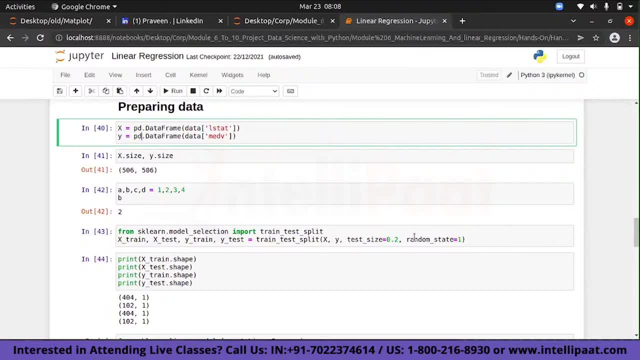 size of my test data set should be 20 percent, which means the train data is 80 percent random state. one means you: whenever i give one, generate the same kind of random variables. if i give 20, it will generate a different kind of random variables. it's like a key. does that answer the question? muna, understood. 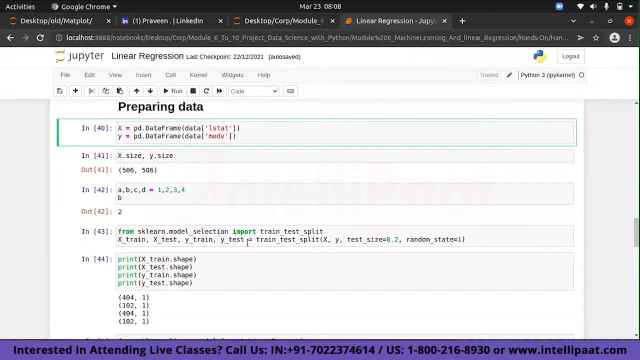 but this order you should be careful: x train, x test, y train, y test. fine, muna, getting the issues. train means you're you're training the model, no, so you'll be training the model, right model, you'll be training. that's why it is trained. it is not the railway train. 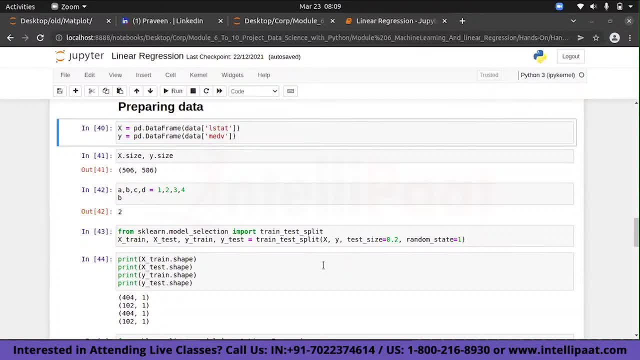 it's a training model, training train instead. i also in the beginning understood, like why are you training, so anyway. so one two, three is like a key, right? so one two, three is like a key. you can give any number you want. when i give one, it will generate one set of random numbers, understand? 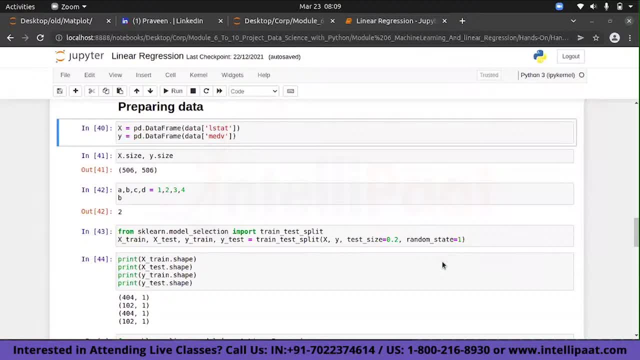 when i give 40, it will generate one more set of random numbers. it is like a key. next time when you use one, it will generate the same number of same set of random numbers which was generated in the beginning. so this is something like this. assume that you have 10. 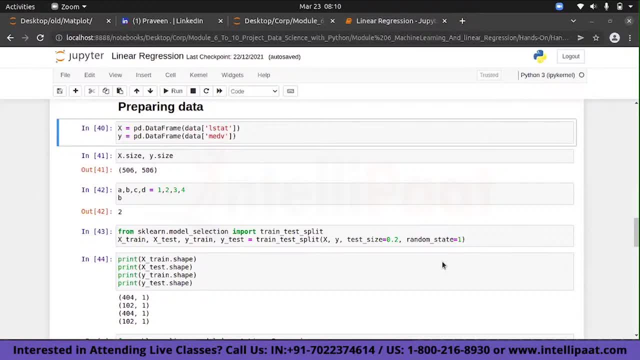 containers. every container's title is random state 1, random state 40, random state 62- something. something is there. it is a key now. in random state 1 you have set of random variables. whenever you take random state 1, you will use that random variable set only if you use random set 42, then 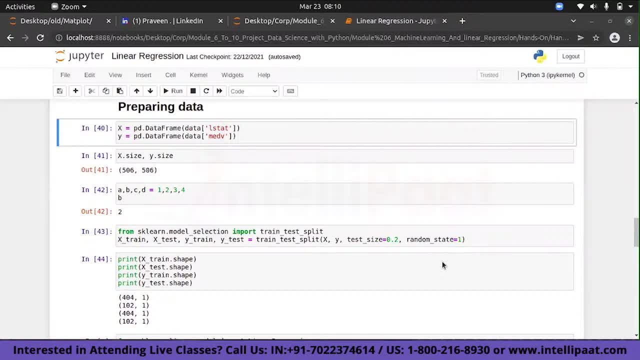 you will have a different set of random variables, random numbers, so those things you will see in the video select. is this understood? what happens otherwise? it will generate different set of random numbers every time, without random state, right. so it will generate different set of random numbers every. 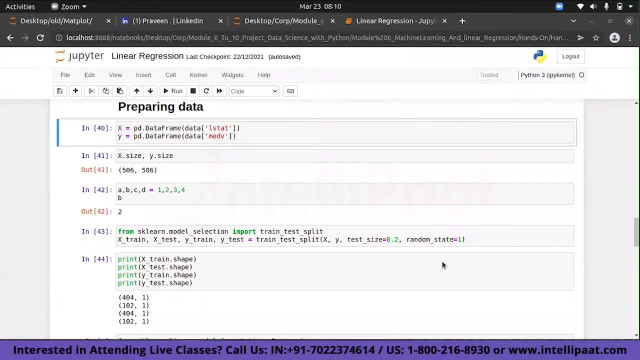 time if you don't give random state, just to have a consistency in the random numbers you will use. random state is equal to one, two, three or something. got it clear? cool, test size is nothing, but you need to split your train and test data. no, so you need to split your train and test. 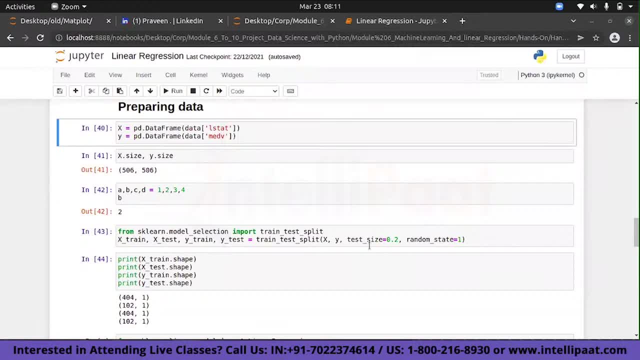 data. train size is the percentage of your train data out of the 506 that you are having. test size is the percentage of the test data out of the 500 that you have. if you change random state, then the random variables will change as per the random state, but if you come back to one, it will generate. 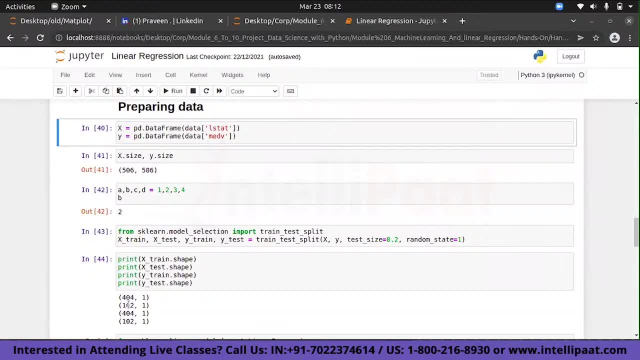 the same random variables that were generated when you used one. that's it cool, are we okay? understood all of you why we have four variables here: x train, x test, y train, y test. so training means you need to train your data, right? so first thing, you have to train, so for that you have two variables for testing. also you have to test for. 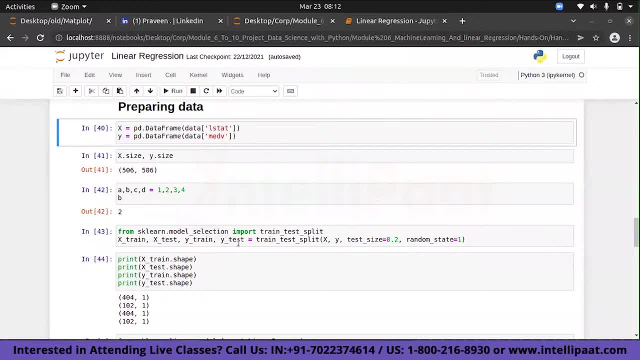 that also, you will have two variables. so basically, training and testing. both are there because you have to train your model and then test the model. so that's why so x train, y train will be used to train the model, x train, x test, y test will be used to test and validate the model. so that is why you have multiple things. 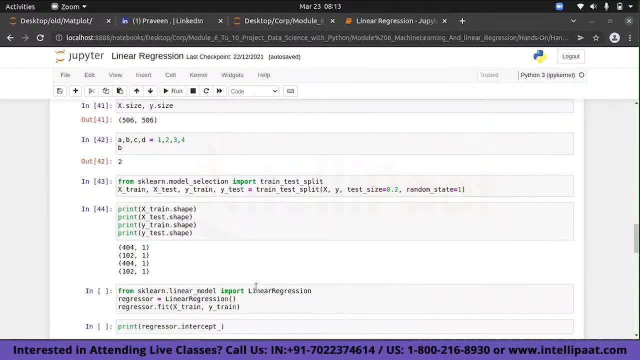 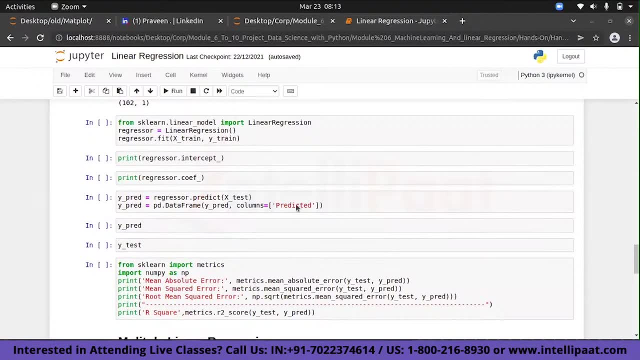 here. so what we'll do is next: there is one small thing that i want you to do, right? yes, it should be both same, for example. correct. so now to build the model. so, whatever you are seeing, this is the three lines that you will read. nothing else apart from these three lines. yes, samir, you are right. 404 and 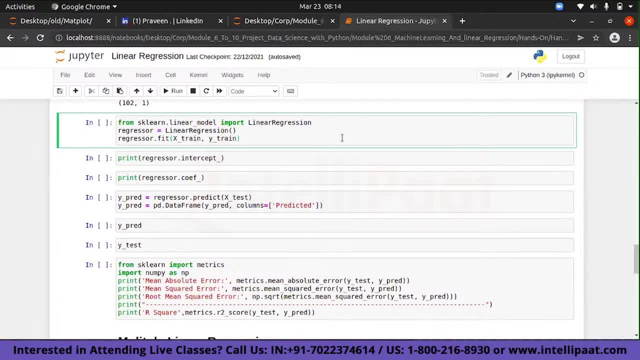 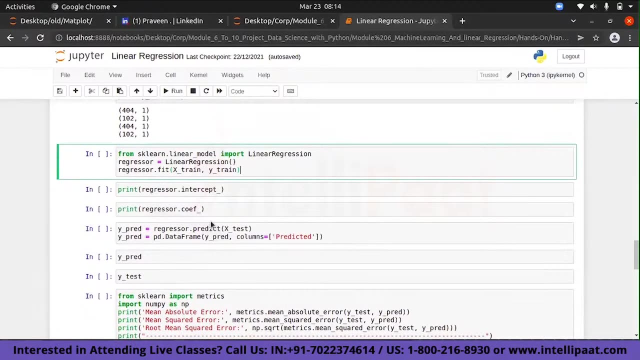 104.. so you can see here here. next, one more library. i am using it, which is nothing but my sk learn. so sk learn is a scikit learn library, so that i'm using from here. so by using sk learn library, what we are trying to do is. 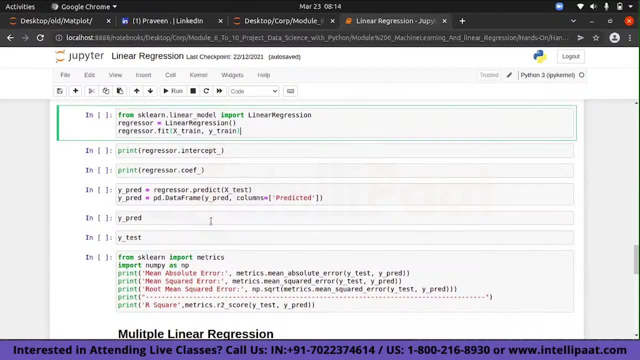 we are importing something called as a linear regression right from sk learn linear model. import linear regression. so scikit learn has multiple models, so one is a linear regression that we are taking, so nothing else apart from that. so basically, you are importing this linear regression function, storing it into a regressor, then you are fitting. 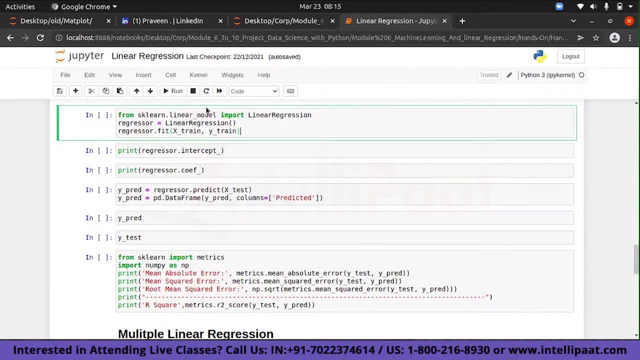 it. so these is the three lines that will help you build the models right. first thing, importing linear regression, storing it into a variable and then fitting it for x train and y train. so when you fit it for x train and y train, what happens is it will construct. it will basically construct a model and train it will. 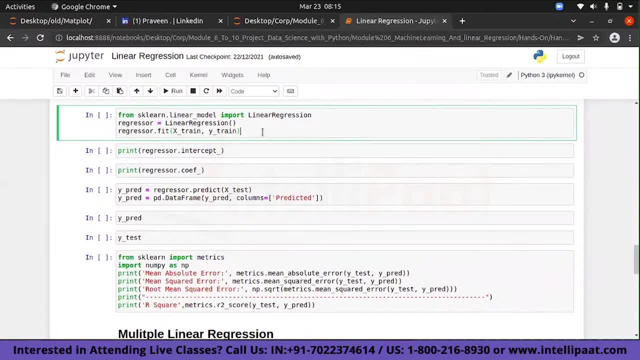 construct a linear model and train it on x train and y train. so just like how we did the complete math process, you remember, yesterday we tried to solve y, m, x, c, we tried to find r square, we tried to find all of that. so this is something that it will do. 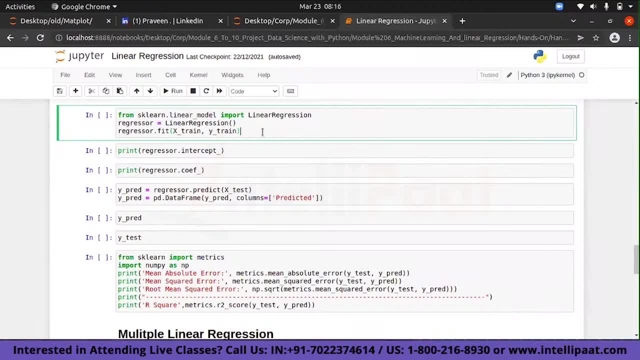 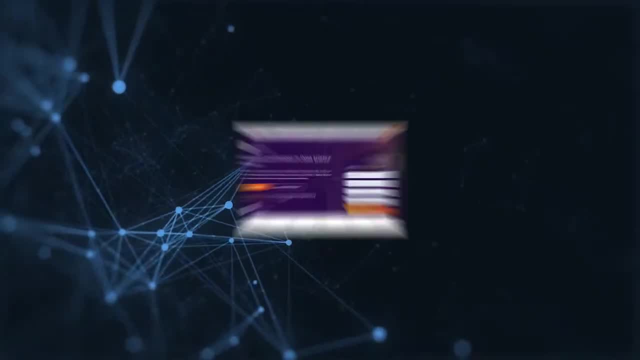 whenever you try to fit the model. intercept means c, coefficient means m, correct, clear. so the three lines that will come and then that will save. if you want to make a career in data science, then intellipaat has iit, madras, advanced data science and ai certification program. 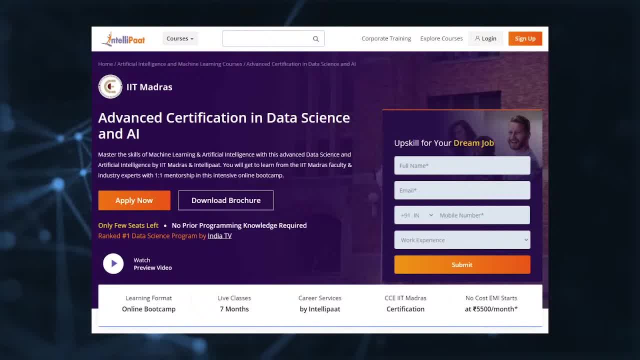 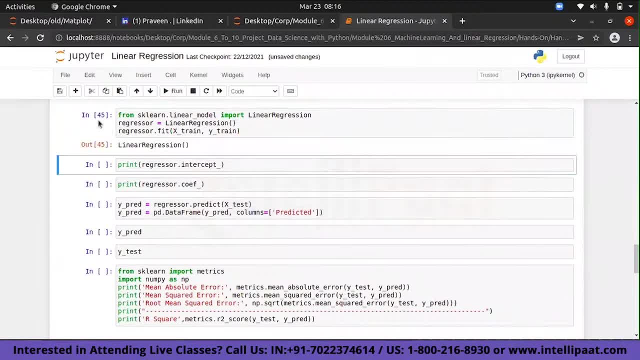 this course is of very high quality and cost effective, as it is taught by iit professors and industry experts. for building a model, it will take some time. if it is complex, it will take some time. if it is simple, it will run very good. now you all know what is intercept and what. 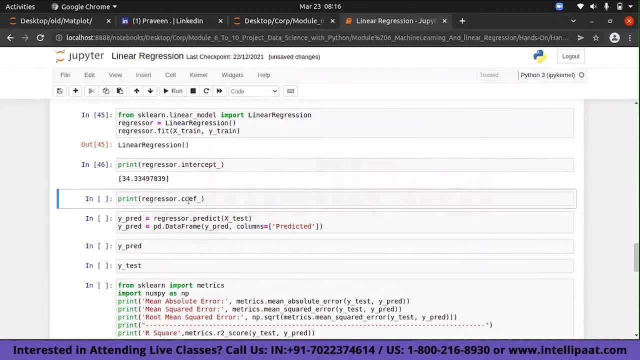 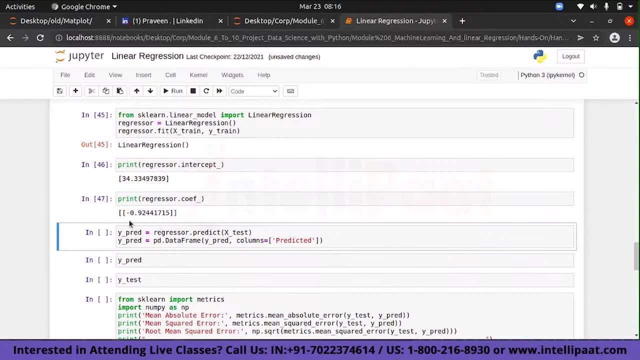 is coefficient, right, you can see: when you put an intercept, you are getting 34. when you put a coefficient, you are getting 0.92, right, so you are getting a minus 0.92. what does this minus mean? can someone answer? correct, exactly, right, so you can see whenever you have minus 0.92. 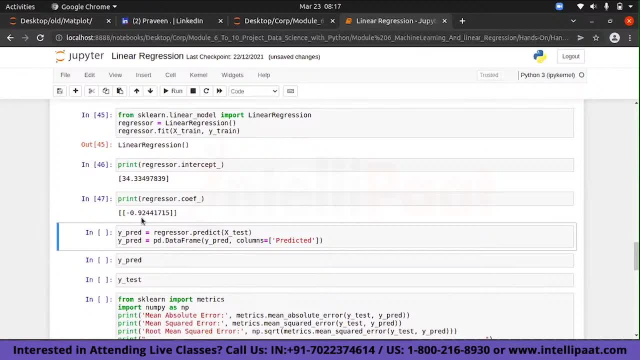 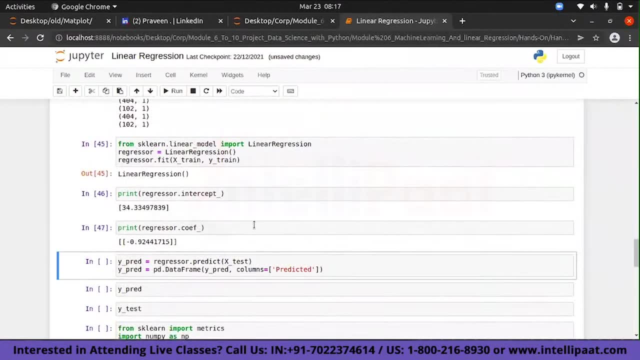 which means i have a negative relation. so obviously right. so you can see by visualization also, all of you saw it is going to be a negative line. your coefficient and these things are also telling that it's a negative one. so is this justified? now can someone type what is the linear regression equation? y is equal to. 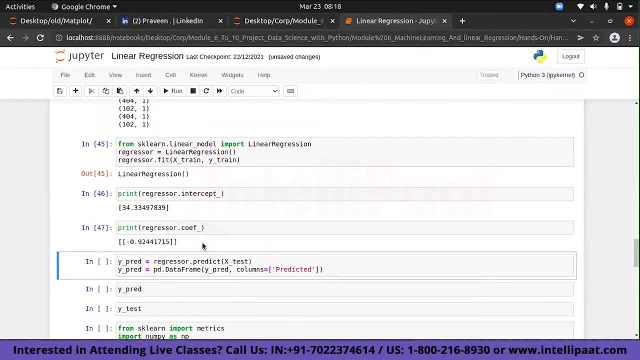 can someone type the final regression equation, a mathematical relationship between your l stat and your m dev. so m dev is y, m dev is equal to what m dev is equal to use m dev and l stat. l stat is equal to minus 0.29 m dev plus 34.33. cool, now i have one question for all of you. 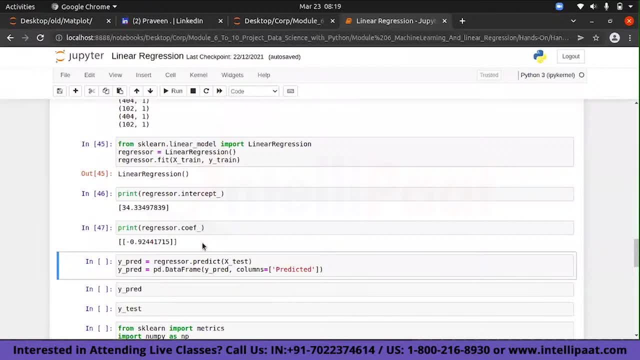 what is the minimum value or the minimum price of a house if i have zero l stat people? what is the minimum value of a house if i have zero l stat people? understood now the concept. now you are able to understand how linear regression works to get starting and so on. you are doing it all by yourself. whatever concepts you learn, you are. 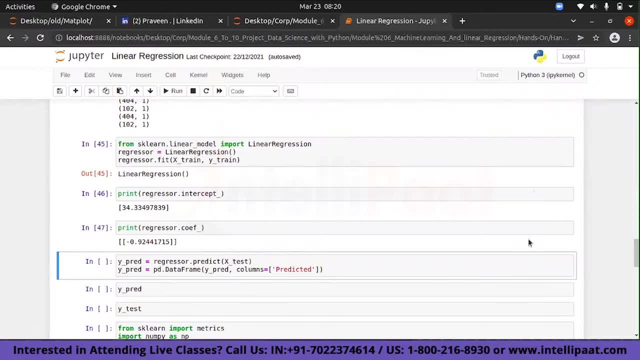 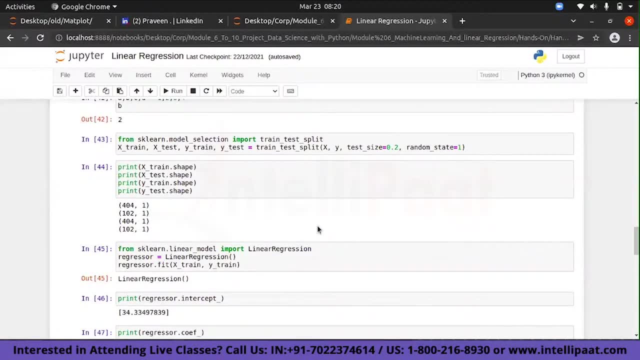 using them and then you are doing okay. a is negative means l stat goes up. price will come correct. tell me what is the question correct. we have two test and two train variables. why we have it? because x train and y train. now you know why i have x train and y train: to train the model, correct. 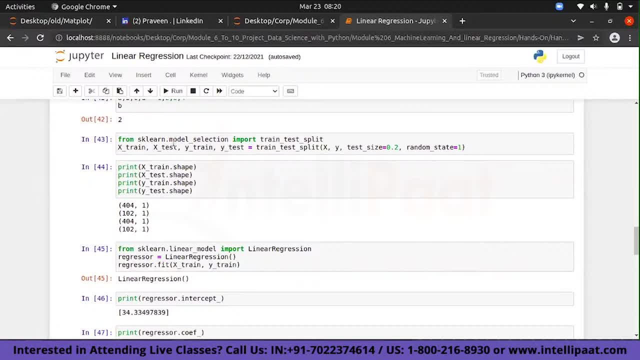 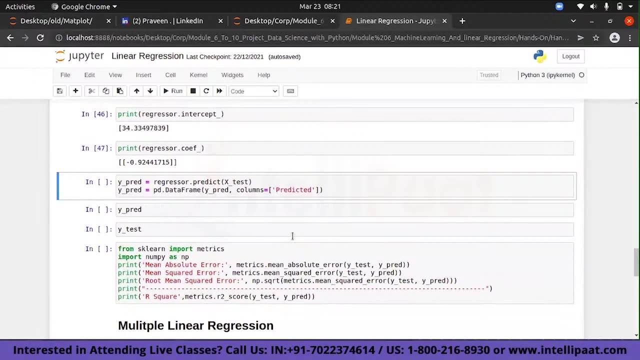 i have x test and y test to test my model. i will use x test. i will get a prediction. to compare my prediction with actual, i have y test: m dev is y, l stat is x. so all of you are able to understand it. till here, no issues, no problem. yeah, train test split is assigning four values. yes, in this order, train. 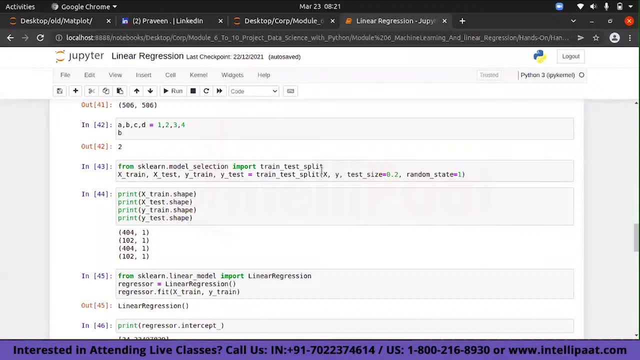 test, train test. whatever you give, so you can see here: x will be split into two pieces, x train and x test. test size will be 20. train size will be 80. y will be split into y train and y test. test size will be 20. train size will be 8. it will. 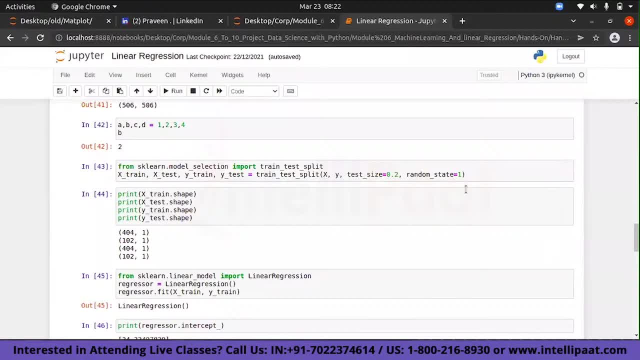 not take decimals, it will take only integers. just remove decimal. it will be 404, correct? x train and x test. we can't correlate. so x train, x and y are the variables that you need to understand. x train and x test, y train and y test are the variables. it's not the variables, they are the. 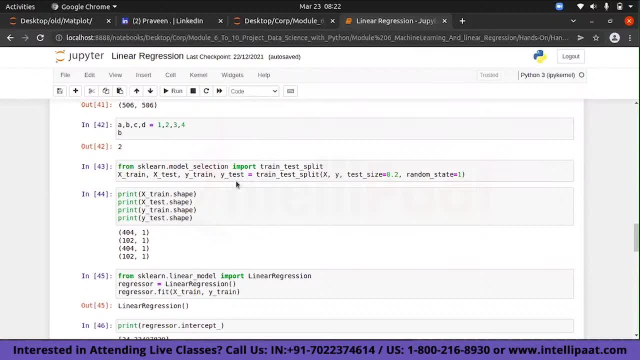 data, small subsets that you are using to find out the model. so 404 is 80 percent of 506, 102 is 20 percent of 506, so that is the test size. if you give test size 0.2, then train size is 0.8. so 80 percent of 506 is 404, 20 percent is 102 train and. 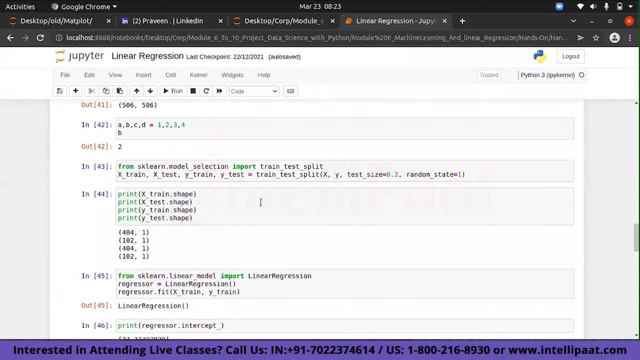 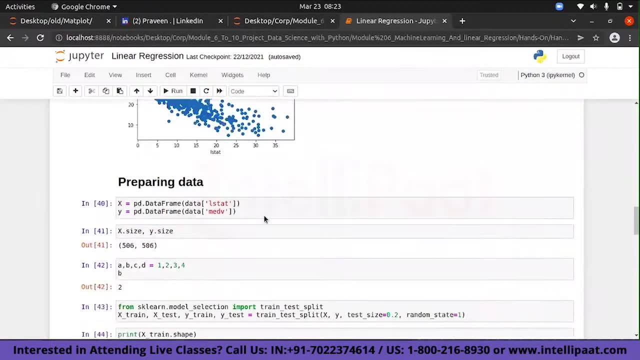 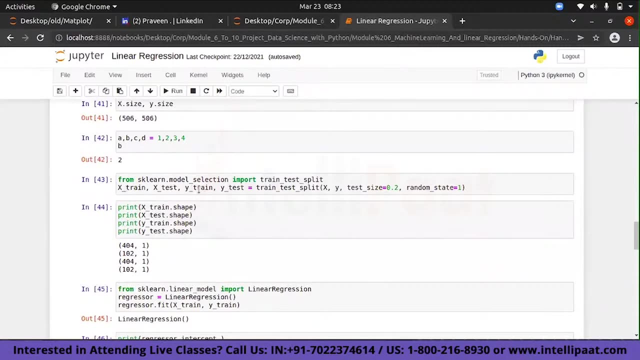 test. both are different. x and y are different. so x and y is what you saw here. now x and y is used and we built a model statistically. but for machine to learn i need to teach it. no, so teach it. i am using x train and y train, so to train the model. so this is the model. 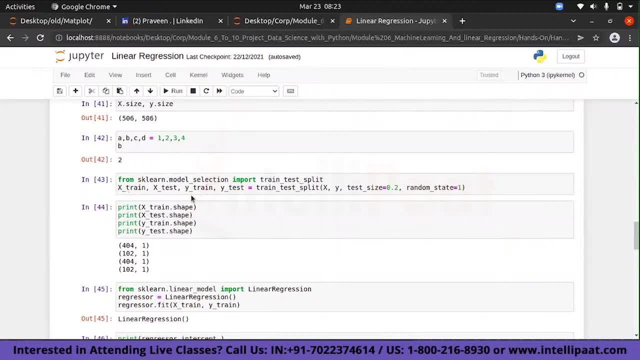 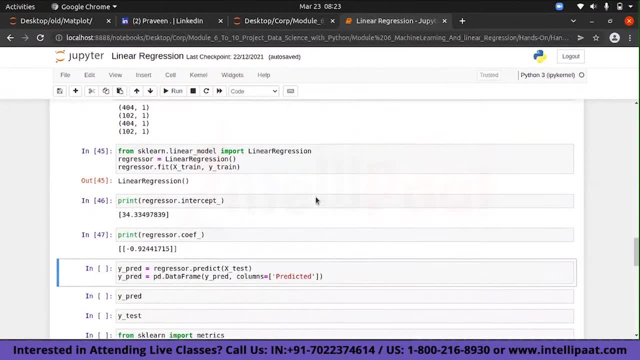 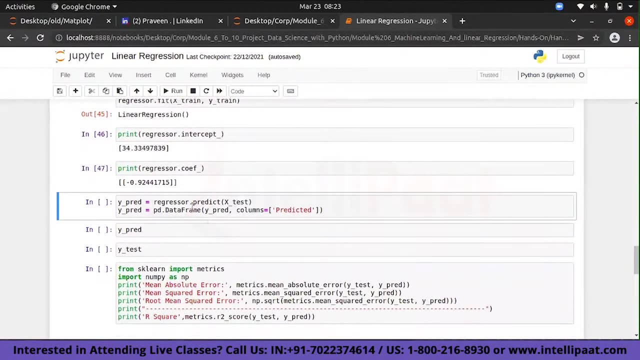 you learn. then, based on this learning, whatever it has done on x train and y train, it will test for x test and y test. clear, all of you. so now what i am going to do is: all of you got the equation. so this is how you build a linear regression: simple linear regression. so now you do a predictor. so 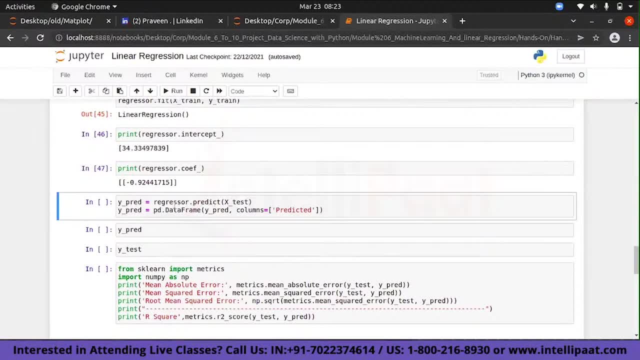 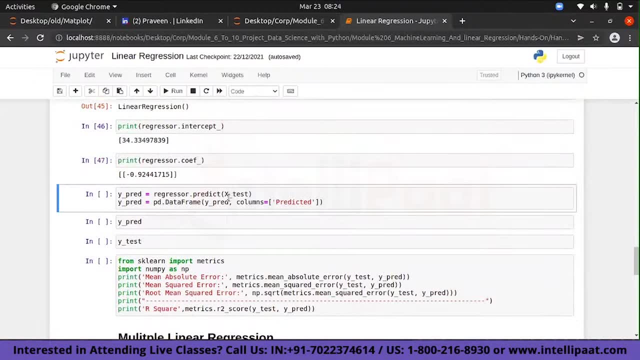 y pred is equal to a regressor dot predict. so what is there in my regressor regressor is linear regression, so y predict is equal to regressor dot predict of x test td dot data frame. y predict columns is equal to columns. so you're just trying to type this and then predict it. 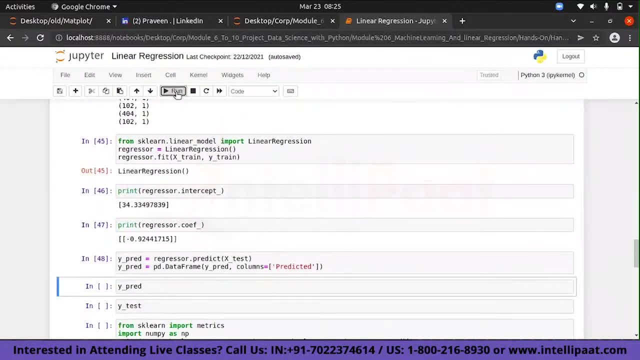 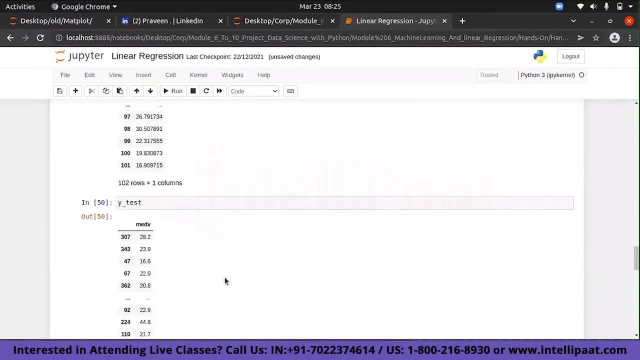 apart from that, now, once i do my prediction, i'm just comparing my y pred with y test. so y pred and then y test, y pred and y test. if i do a comparison, which is my actual and which is my predicted, can someone tell me test is actual? because 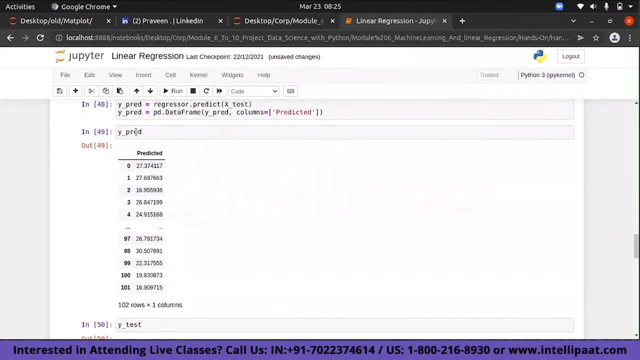 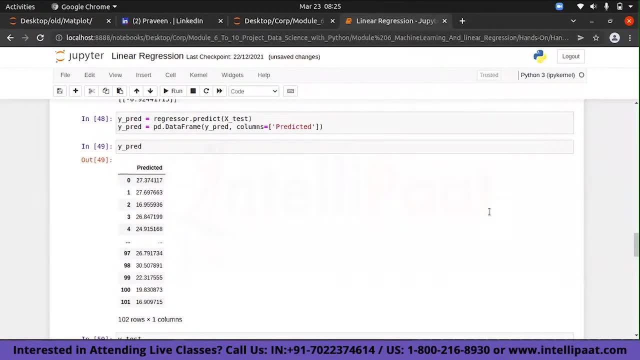 test is what the data has in reality. correct y pred is the predicted. so this is the things that we have right. so this is the same something. we can't take the entire data set, because if you take the entire data set, you will not have a data set for you to test it if you take 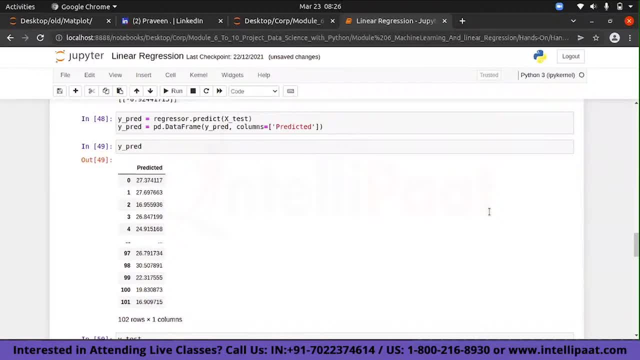 entire data and train. your data will be over for training only exactly. you're getting the point. so now you have predicted an actual value. by comparing these two, you will get your r square. so we have to train and test every time we build a model. no, so first time you build it, there is a. 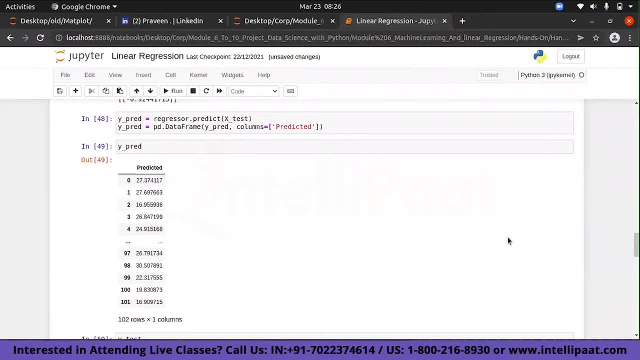 process of deploying models. so if you're using it, then no need to use the basic things that we are trying to do, whatever we are trying. but right now, yes, for building, training, testing- you have to do no other option. now you have a predictor. so if you have the model, you are creating and your model will. be higher than the standard model, then, like, finish after two days. that is why, when you're breaking it, the model will burn. will burn because it's loss, but now you have a predictor that will burn, because then you have the model, you have to build one architecture and you have the price oneient. 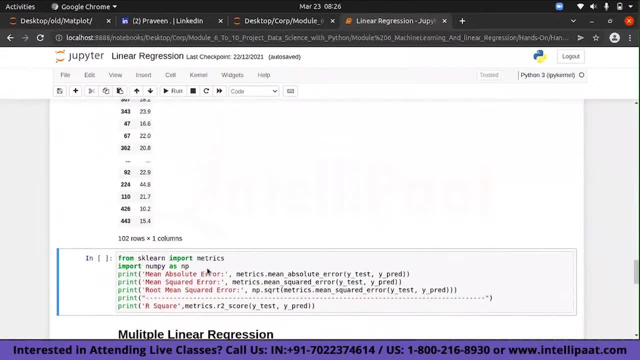 architect that will burn because of you building a model. you don't take a model. you have to predicted and actual. so now you are able to get your r square. so now there is no need for you to write the formula. also, there are metrics available. i have printed all of them so you can just take. 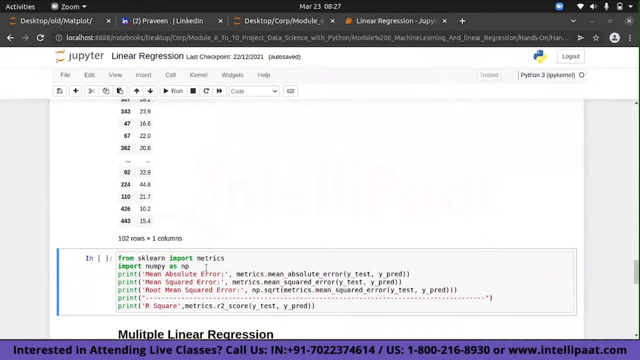 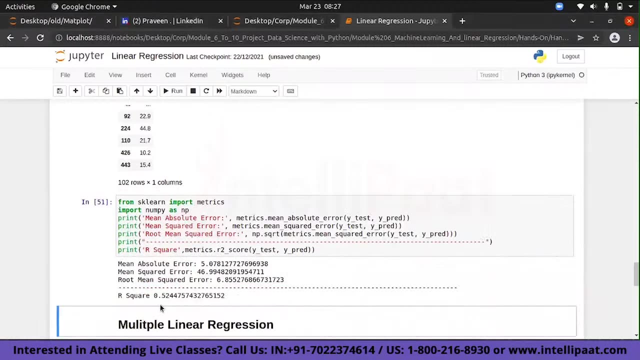 it later and then print it. i'm just showing it to you how it is done. mean absolute error is mae you get. mean squared error is metric, rmsc, r square. so these three things are some kinds of errors. don't worry about this. right now our focus is on r square. so you can see you have 52, which means 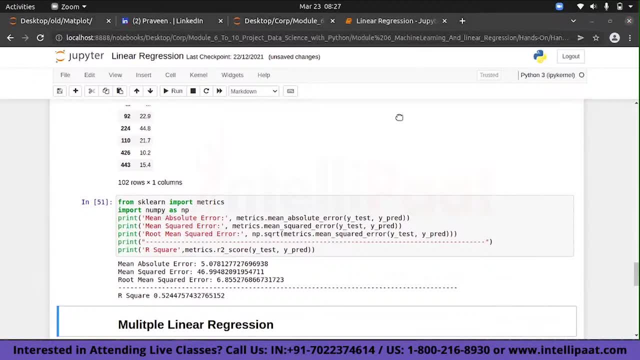 what can someone tell me? scipy and scikit-learn? both are different. no, no comparison. goodness of the model. it's not like 52 percent accurate, but it is able to explain around 52 percent of the variance that is there in the model. so that is what r square means. you can say it as an analogous. 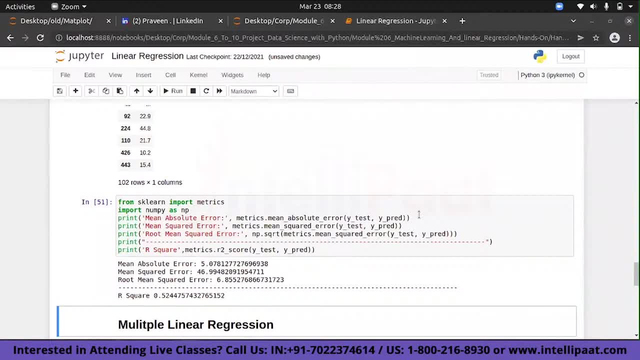 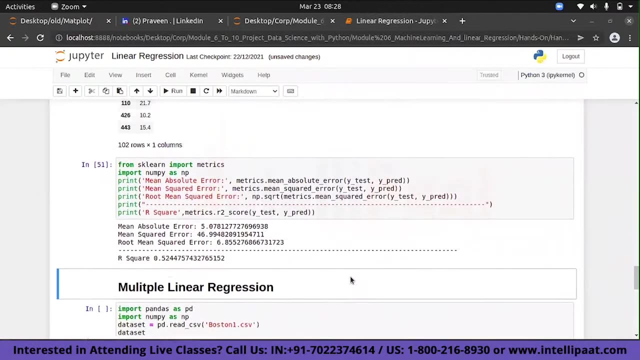 to accuracy, but it is not accuracy. but you have an idea, right? so 52 means a moderately like, not so good, so that is something that you need to understand. fine, now i'm just showing you briefly about multiple regression, which is not there in the coverage, but, keeping learning interest in mind, i'm just showing it to you. so, using one variable, 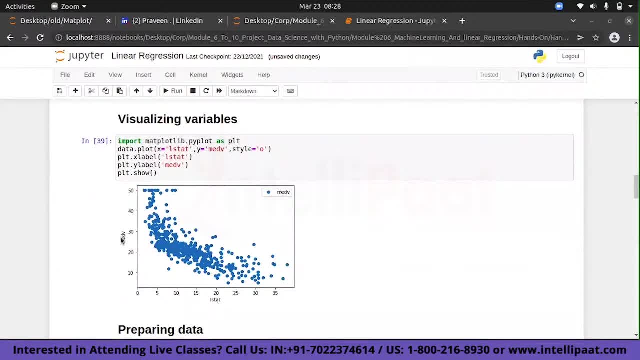 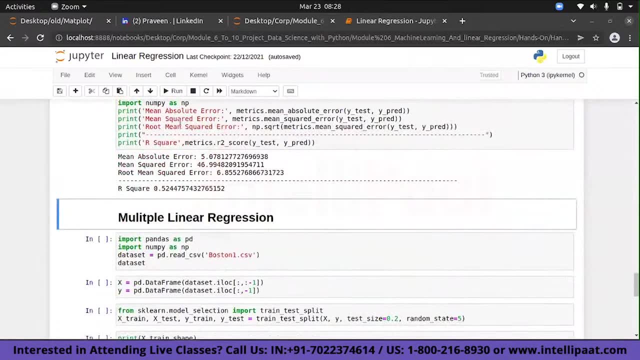 you can't do regression right, so you can't do a l stat and m dev. only one variable will not influence. now we have multiple variables. you can see the process is same. you have multiple linear regression. you import pandas, read the data, so don't type this. 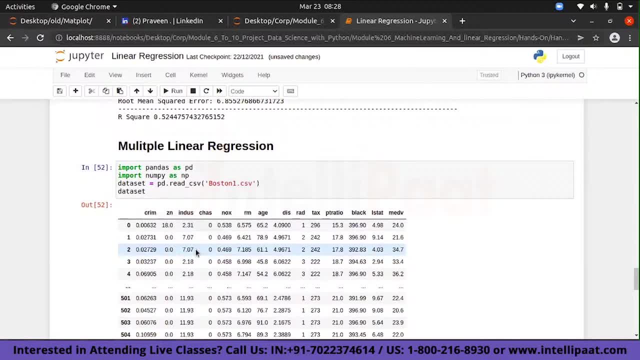 no worries, just understand this, but understand the concept of multiple linear regression. but before going to that, i just want to confirm: simple linear regression is okay, right, you type, you understood the flow, you understood the concept, how from data to get a model, coefficient, intercept and also the r square, thanks. so this is, this is a getting starting point for you. so 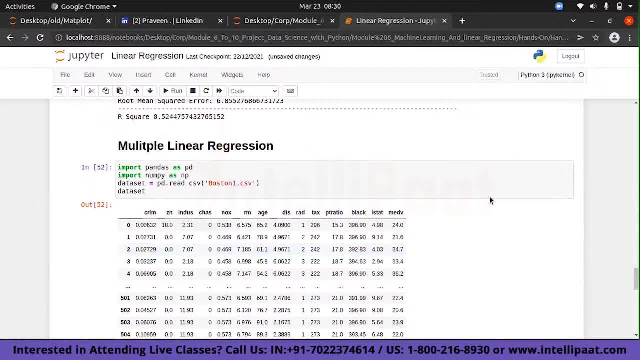 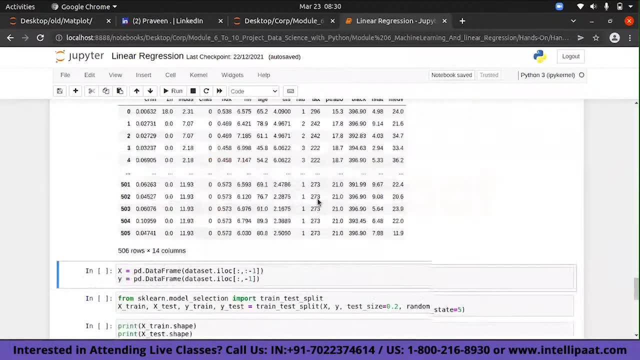 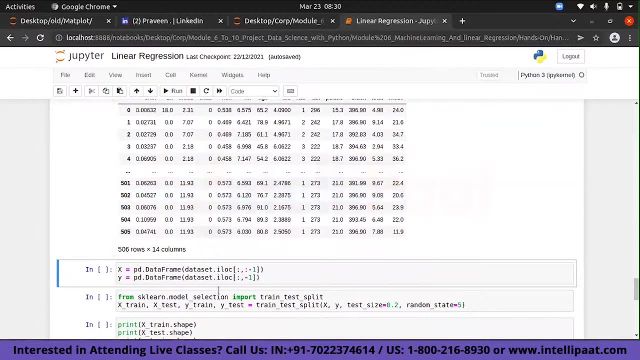 on top of it. you you have to explore. you can't get correlation using describe, right, so now we'll go to multiple linear regression. how it works. so basically, you read the same data set, no change here. what we are trying to do is, you can see i log minus one, which you are all aware. so what i'm trying to do here, x, i am assigning all. 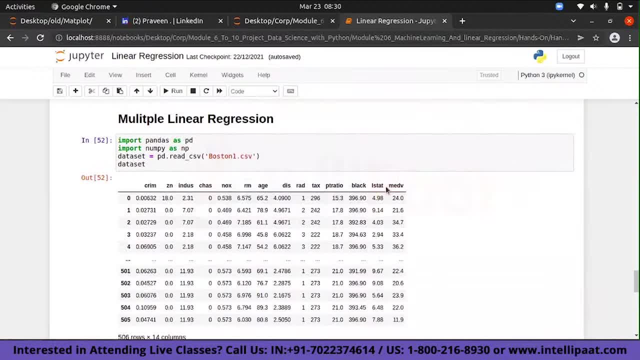 the values, except the last column, which means m dev. all of you agree, all these things are my x, only this is my y. so i'm assigning all the values, except the last column, which means m dev. all of you agree, all these things are my x, only this is my y. so i'm assigning all these things to one variable. 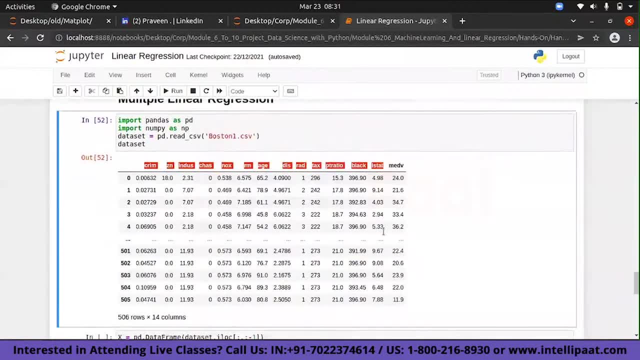 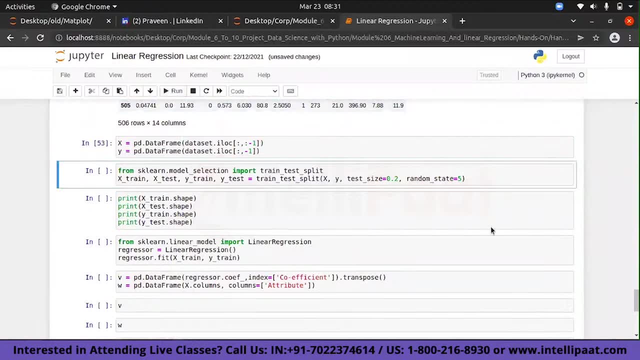 which is called as x, and i'm assigning only m dev to one variable which is called as y. so basically, i have split my x and y right. so once i split my x and y, i'm just splitting the data: x train, x test, y train, y test and all these things. so this is also done: split there's no. there's no nothing. 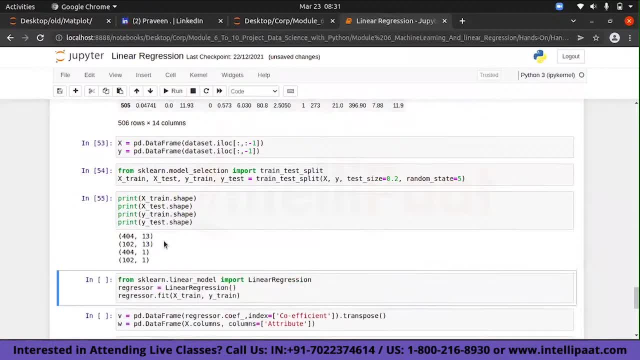 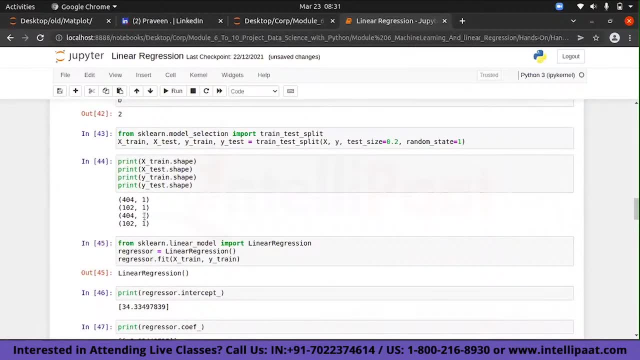 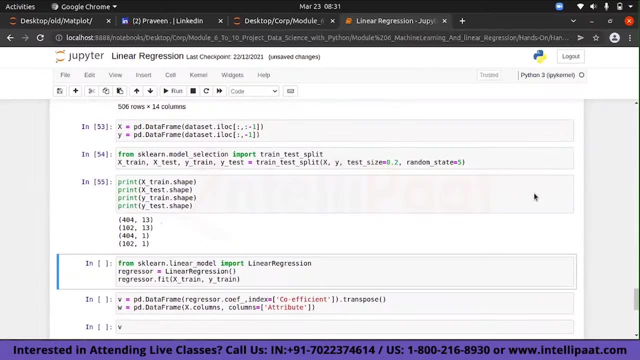 great here. i'm just telling you one thing that you need to note here is: you can see, here you had one column, one column x and one column y, simple linear regression. here you have 13 comma 1, which means x is 13, which means multiple variables. are there multiple linear? that's it. so only this is. 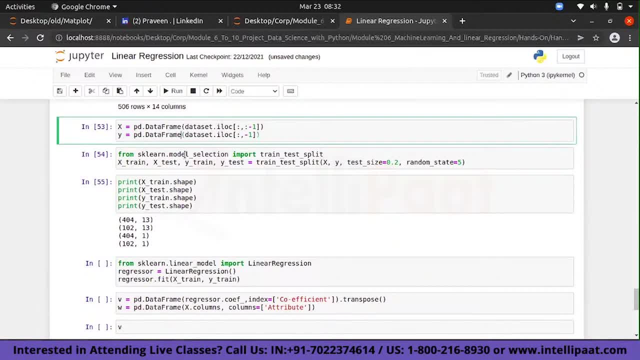 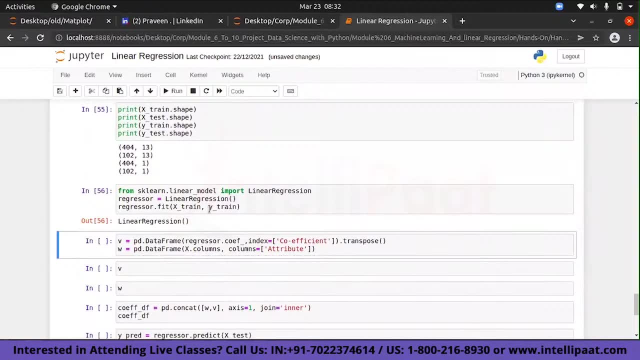 the changes that you have to do whenever you're assigning your x and y rest. all is the same. i'm just fitting a line here. you can't visualize because two variables- 2d, 14, 13 variables, multiple dimension- you can't visualize it. y is only one value, because y is m dev. the target variable is one, so that's why you have only one. 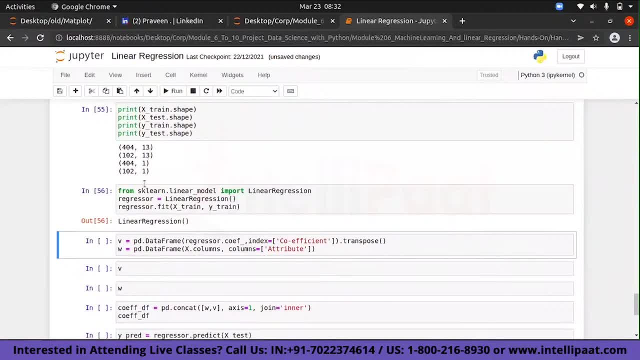 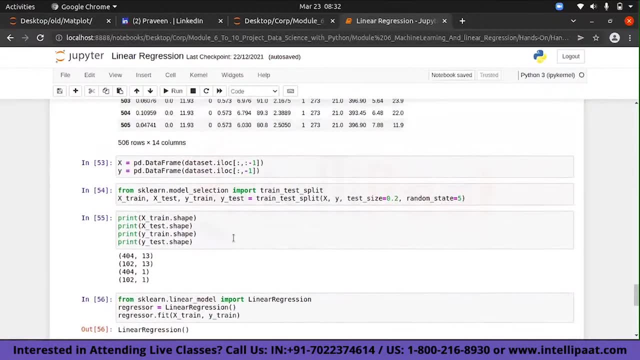 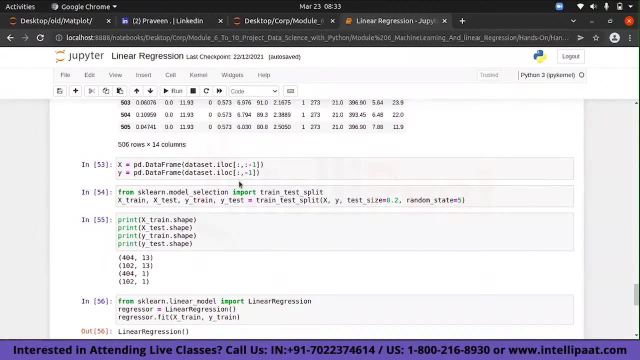 value. there are 13 x values and one y value, so that's why it is multiple linear regression. now the same thing that you are trying to do. okay, let me just wait till here. is it clear to all of you? no issues if things are clear till here. okay, ilo see what we are doing. the last column except last. 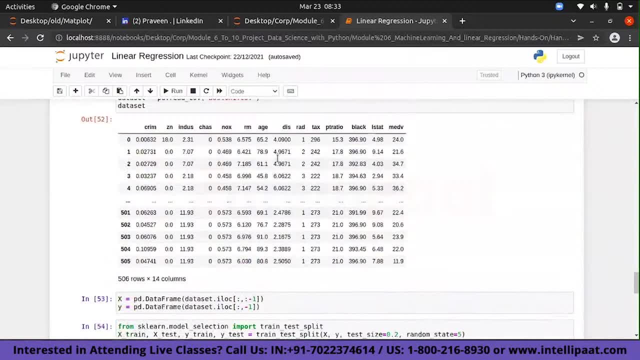 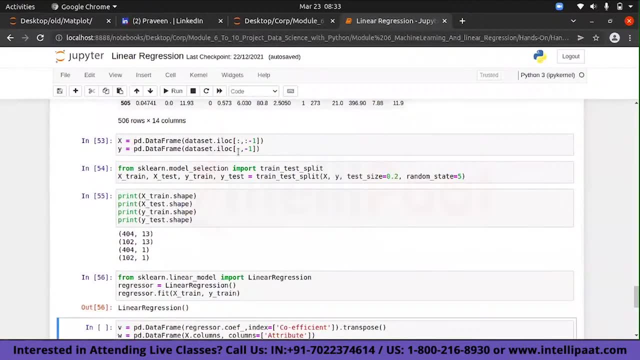 column. all other columns we are putting in the last column. we are putting in the last column into x. so here all other columns are putting it into x, only the last column we are putting it into y. so that is what this iloc is doing now. you don't code it right now. so this is i'm explaining. 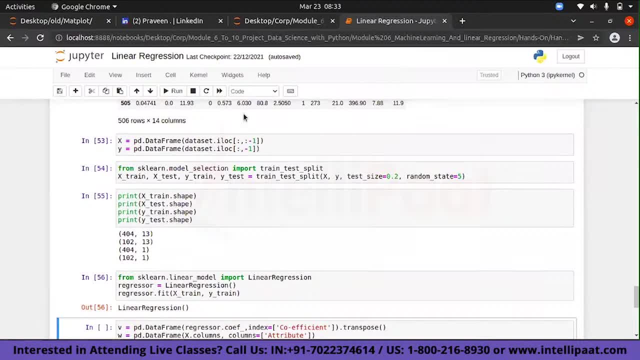 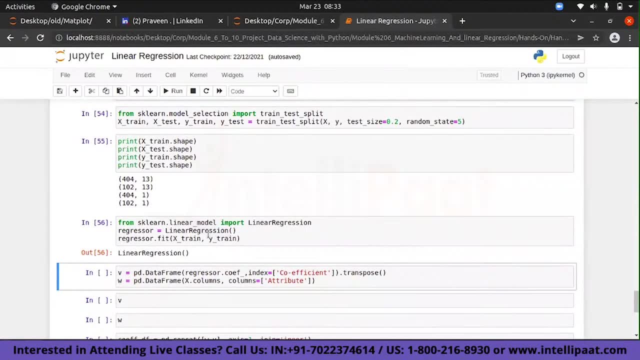 so this you understand, then you can code it later. no problem, right? so you have these things. now what we are trying to do is, from sk, learn import linear regression and then you build a model. once you build this model, next thing is finding out the coefficients and the c. now tell me how. 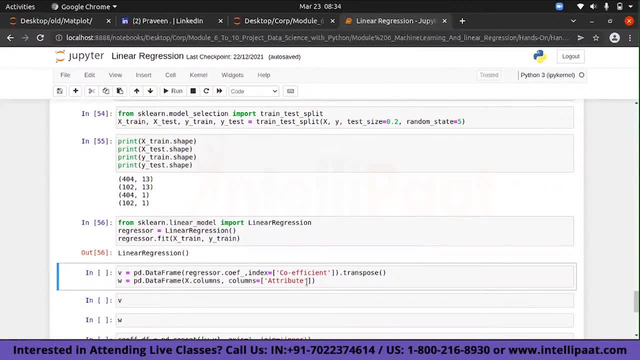 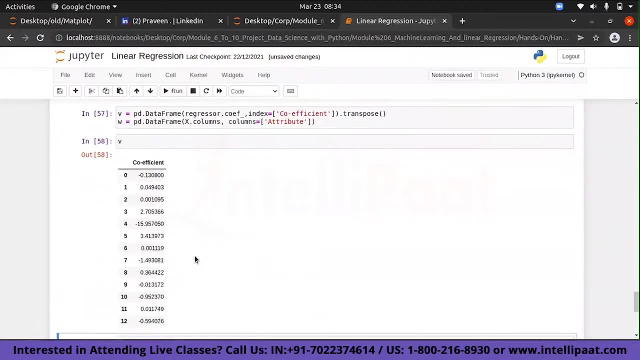 many values of c will come and how many values of x will come. c will be 1- correct. x value will be 13- correct, exactly. so basically, for every independent variable, you will have a coefficient. so that is what you will get here. you can see here: this is my coefficients. 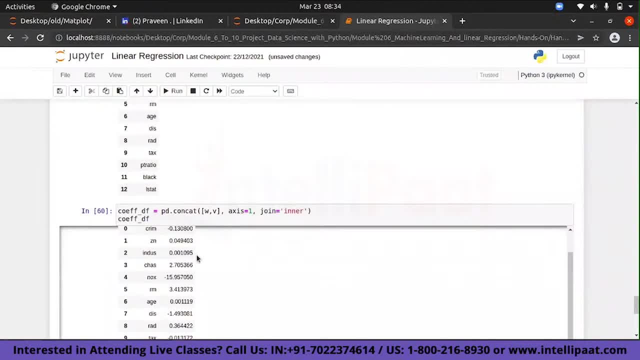 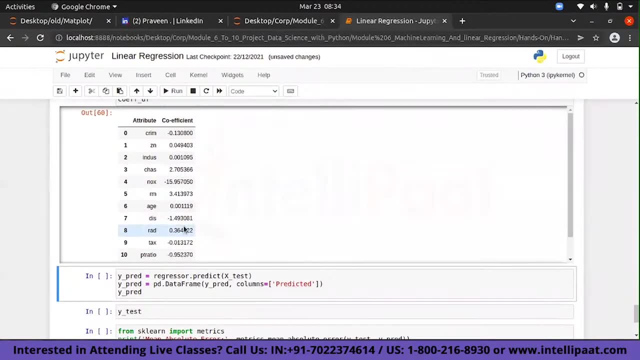 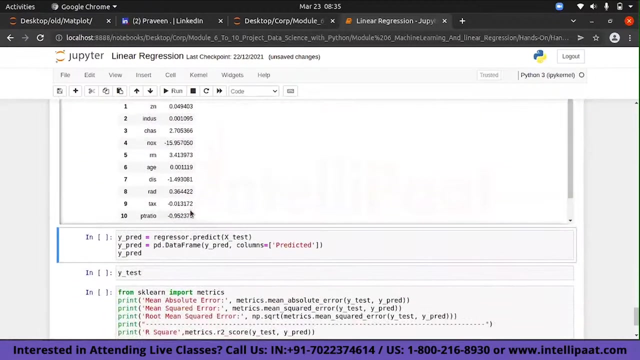 this is my attribute, which means when you combine both of them, you will get something like this: this is the equation. now, if you want to make a multiple linear regression equation, how? because you have 13 independent variables. so for every 13, every independent variable, you will get a coefficient. now for us to get a equation right now. so i did not get. 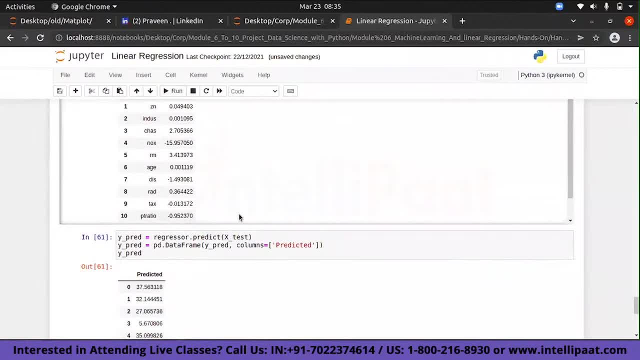 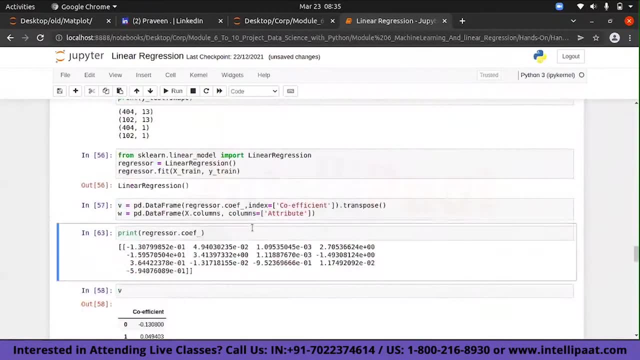 the value of c. so let me just put the value of c. also, this is a predicted y test. let me just get the value of c as well. coefficient is printed intercept- right, is it intercept? let me just take the code. you can see 37. right. 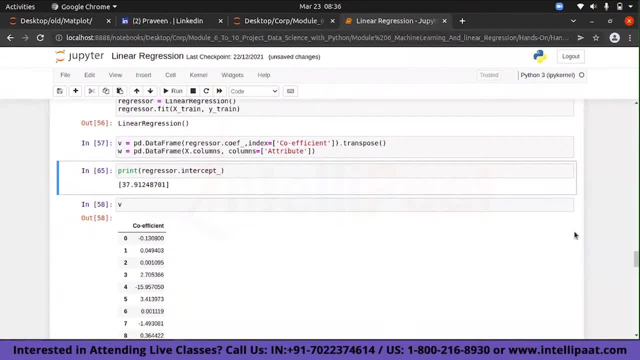 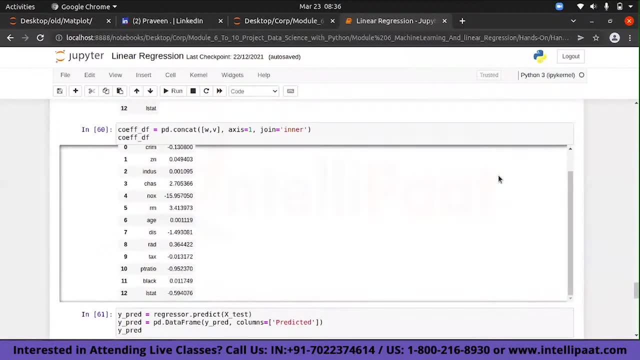 with these values. don't you think you can find the multiple regression equation? no, c will change. c will change if you change the variables correct. i mean see, c will change not for every value of x, but for every set of x. if you take one x and one y, it will be different if you take three x's and 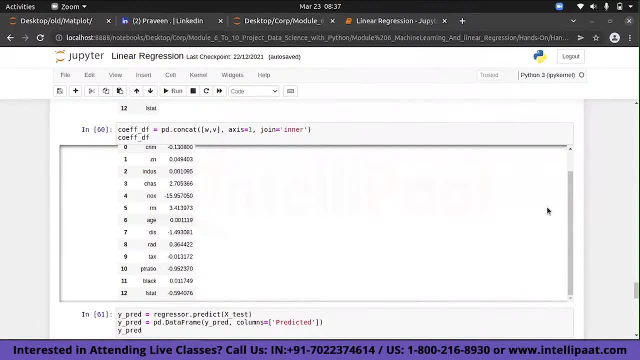 one y, it will be different. if you take four x and one y, it will be different. if you take nine x's and one y, it will be different, because you're changing the variables every time. so that is the 13 different c. no, 13 different x, 13 different m. you will get, sorry, 13 different values of m. you. 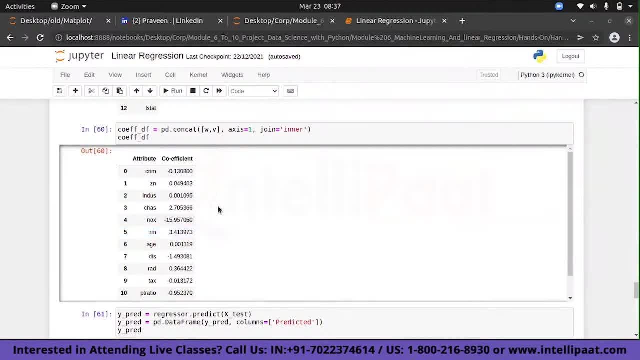 will get, not the c values. so now the regression equation is nothing. but m dev is equal to minus 0.13 crm plus 0.04 zn, plus 0.01 indus plus 2.7 chas. so like that, like that, like that. 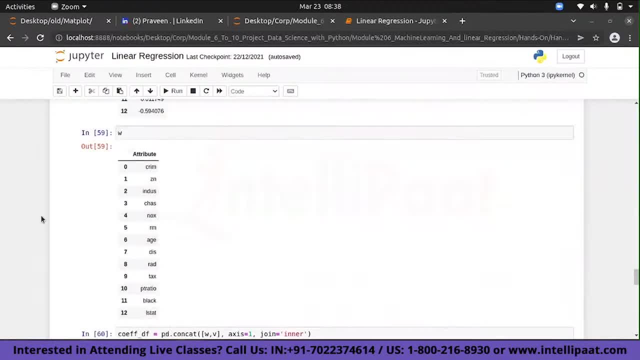 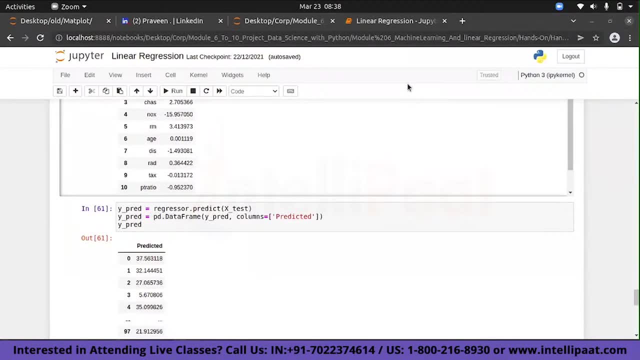 last plus what is the value of c around 37? that is my multiple regression equation. clear to all of you. any questions? we can't display the equation, we have to, uh, write it. there's no library, so separately they will have different m and c together. different. yes, separately they'll have. 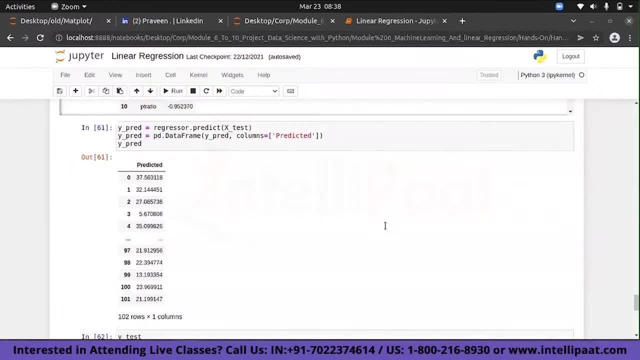 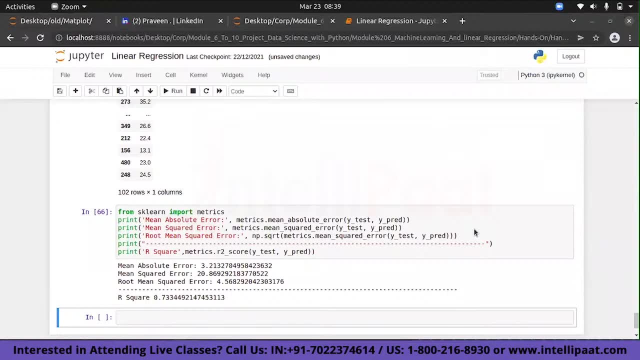 different together, different, correct- understood this concept of multiple linear regression. all of you- and this is nothing but our normal one- our wipe rate is computed using both coefficients. now it is actually doing the same. now, if you can see, if you include multiple variables, your r square has increased to 73. all of you saw that. fine, all of you getting 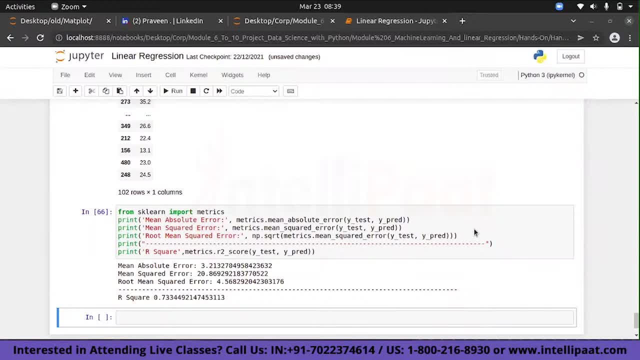 this point, how exactly we are seeing it? is this concept clear to all of you? more number of variables, you will get good accuracy, but there is something called as dimensionality reduction. you remember i taught you dimensionality reduction. it's not more number, it is quality, quality of variable. yes, jerry, you can go ahead and answer your questions. you got it. 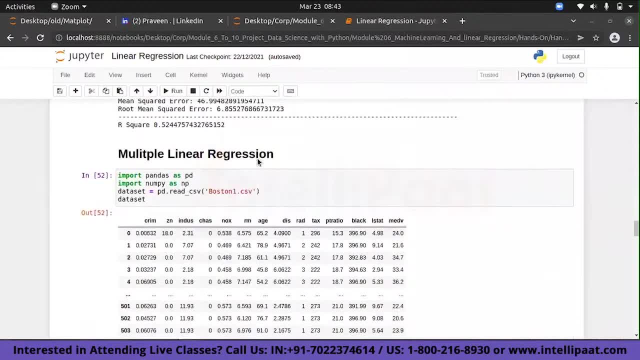 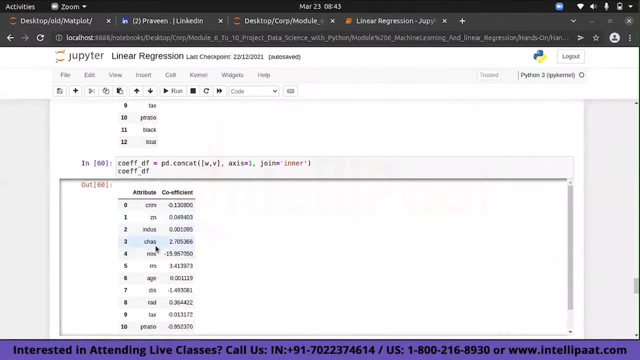 okay. so whatever negative numbers you are seeing here, which means when these things increase, your house price will decrease when positive number increase, let's say charles river. so who doesn't want a river view behind their house? so then its price is increasing. so who doesn't want something? 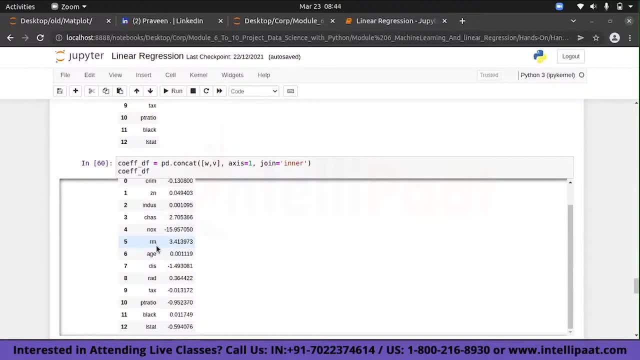 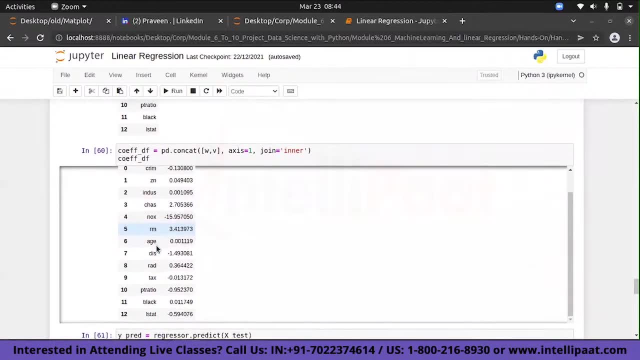 called as, like rmi, for example. so if you have a river view and you have a house price increase, you have to go ahead and convert what was rm. so i think it was- uh, i don't know, i'm not even looking for it, but let me just see. and then you also have, let us say, for example, rooms per dwelling, correct? 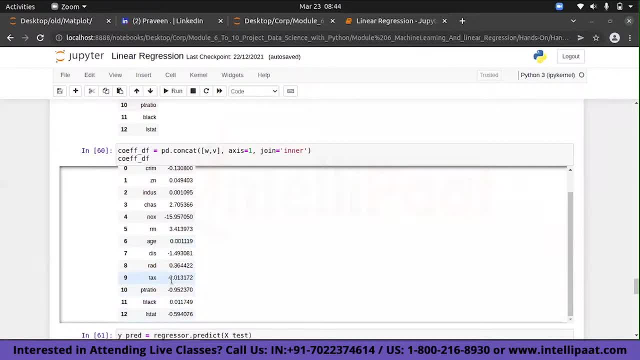 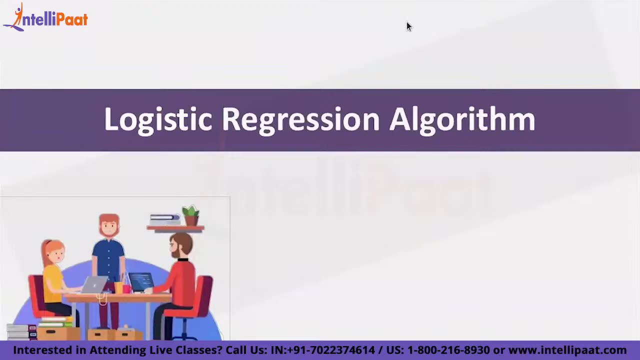 so rooms per dwelling is rm, so something like that, right, so you can just go ahead and then see this and then, based on this, you'll be able to do an analysis. you got it. okay. let us start with something called as logistic regression today. so what do you mean by logistic regression? so there are two things here. 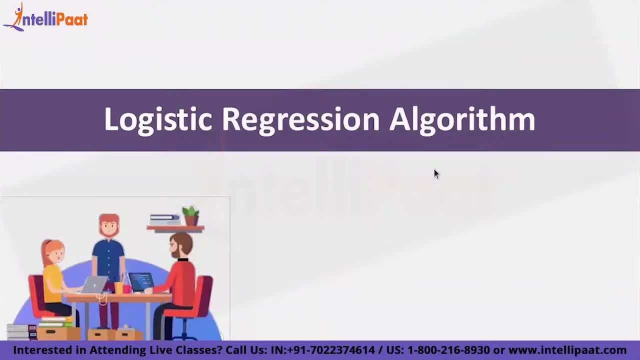 one is logistic and another is a regression. so what do you understand by logistic? so anything related to logic or any, any, any idea. what do you mean by logistic regression? anyone have heard about it before. okay, so basically, class of regression techniques can be used in multiple places so you can use it for doing regression problems. so regression, as in finding a straight. 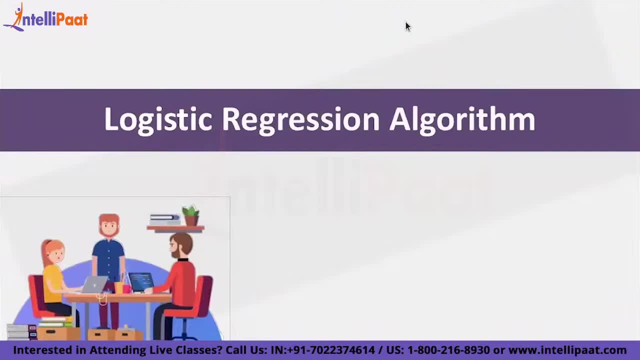 line relation. you can also use it for doing a classification problem. so in this case, classification is nothing, but you're classifying things into yes or no, one or two pass or fail type, understanding it right? so basically, logistic regression is nothing, but you are using our algorithm to do. 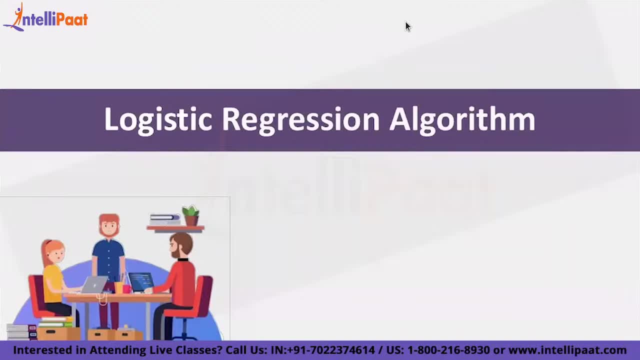 some kind of problem? classification. logistic regression is a classification algorithm. yes, it is basically for binary results. as of now, it is for binary results. we are doing a classification now. once you understand how exactly you do the classification, you will see an example of how it is done. was for: 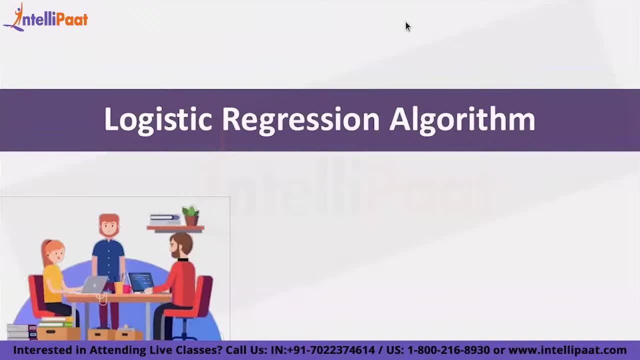 regression. so regression here means you are trying to get a straight line relationship, so that is now. we are doing something called as classification, right? so classification is nothing. but you're trying to classify things into multiple pieces, right? so yes or no, pass or fail types, so that is your. 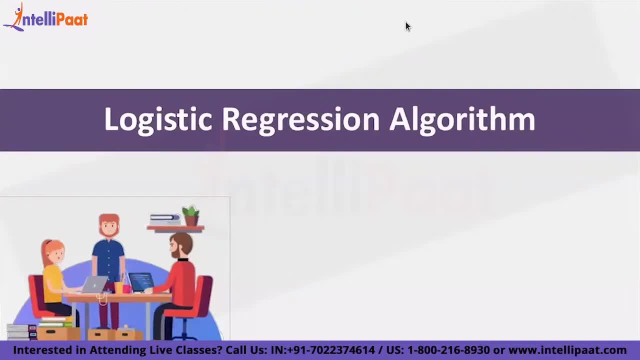 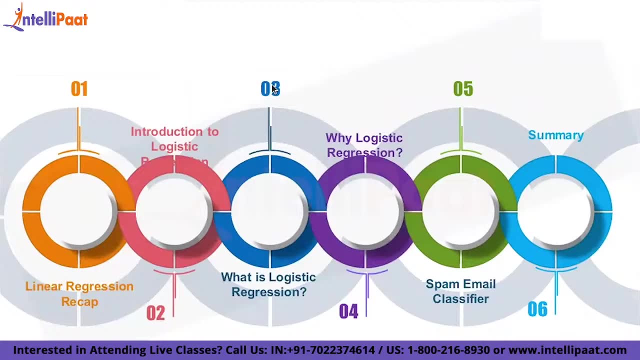 classification. now, having said all that, we'll go and then we will see how it works. so you can see what we are trying to do is we will see how we did linear regression and then we will do introduction to logistic regression. what is logistic regression? why do i need logistic? 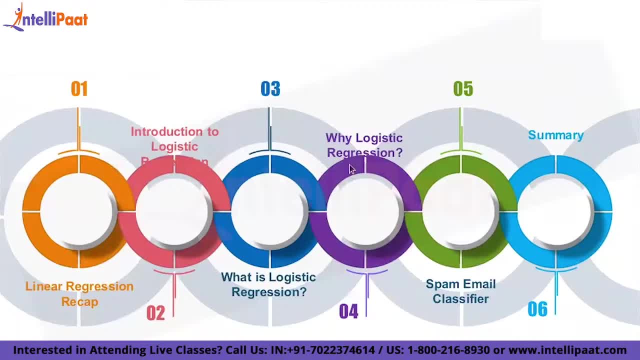 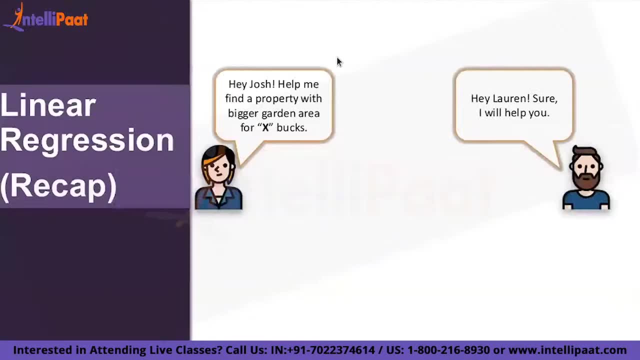 regression. i have a spam email classifier and a summary. so, looking back at linear regression, what, what all do you think that are there in linear regression? i will tell you so you can see. this is just a conversation that is going on right. so if you can see here what all the things 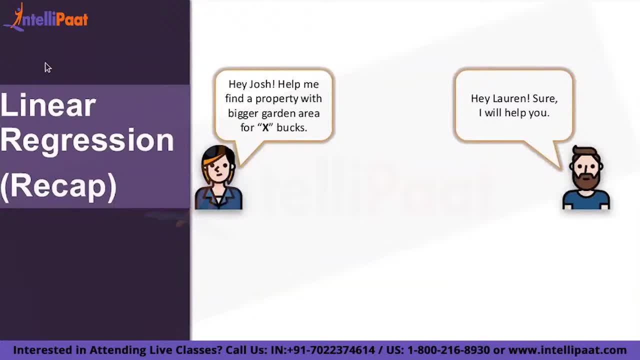 that you saw in linear regression. you saw house price. so one guy is asking: help me find a property with bigger garden area for these many rupees. so other guy is saying: sure, i will help you. so what are the things that we can do? so x and y so you can see here: x is the amount where we'll get a. 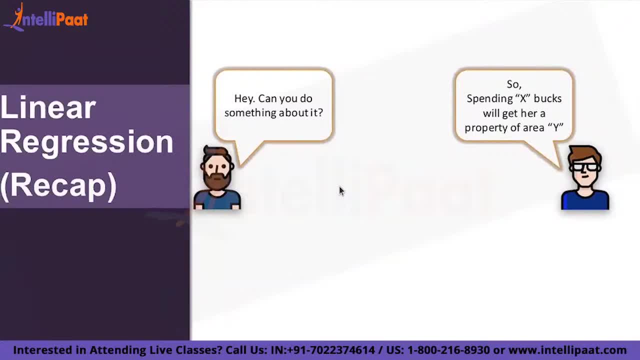 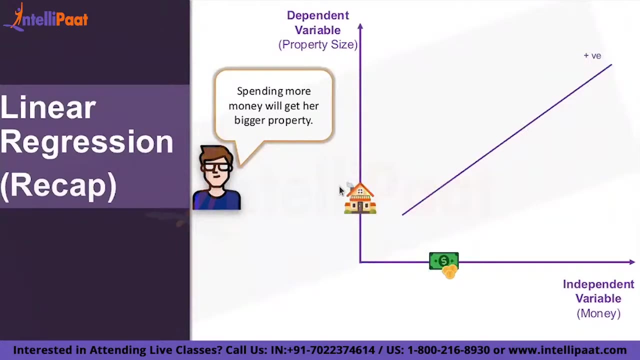 property of area y. so one guy is defining his x and y parameters. now how do you find it out? so what is the area that we get? that is by simple linear regression. so we can see how. so you can see here. this is a example that we saw. independent variable is revenue, dependent variable is property. 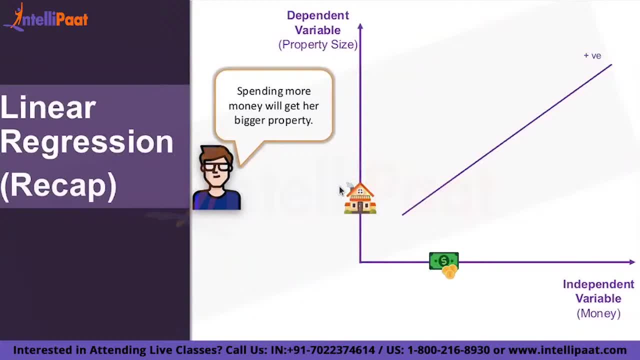 size here, which means you can see here this is a property of area y, so one guy is defining his x and y parameters. so more money you give, bigger property you get. so basically this is something right. garden independent, independent variable is garden area right and then house area. so if your garden area 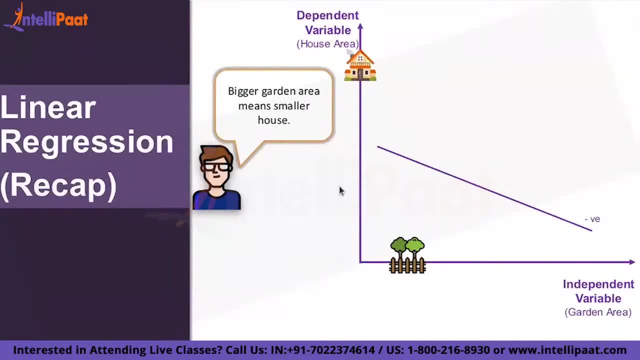 is increasing, house area means it will become small, because if the plot size is limited, if garden area is increasing, house area will become small. so these are some of the examples of linear regression. now, by using these things, what these people are trying to do is they are finding they 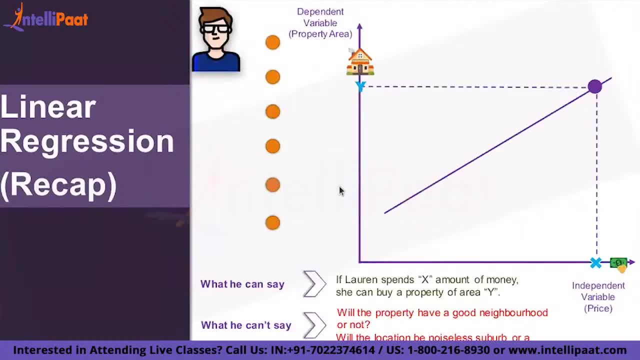 are trying to find a house area and they are trying to find a house area and they are trying to find a house for their budget. so if lawrence spends x amount of money he can buy a property of so and so area. so he can tell that one because he knows the linear regression curve. now, what is not? 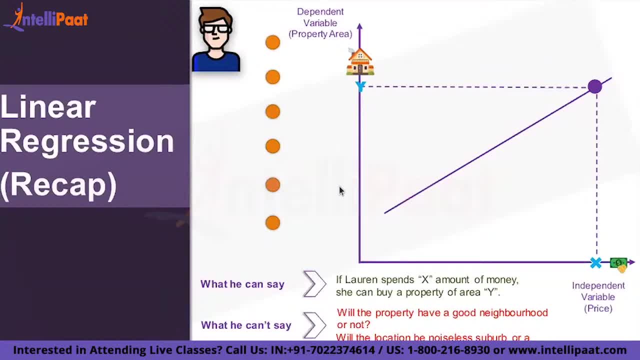 assured here is: will the neighbors be good or not? that you don't know right. will the location be noiseless or not? that also you don't know. those things you can't say because you, you have to go to the property, check all that and then, only then, you will understand. so this is point number one. 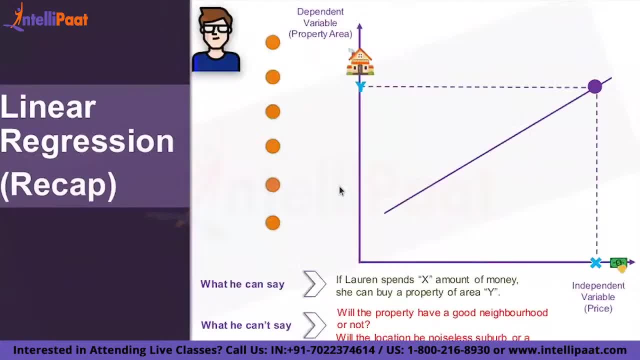 point number two is now you can see here you have multiple things or multiple aspects that you are considering. will the property have good neighborhood or not? that is a yes or no kind of a problem. will the location be noiseless or noisy? that is also yes or no problem. so basically, if you can observe, 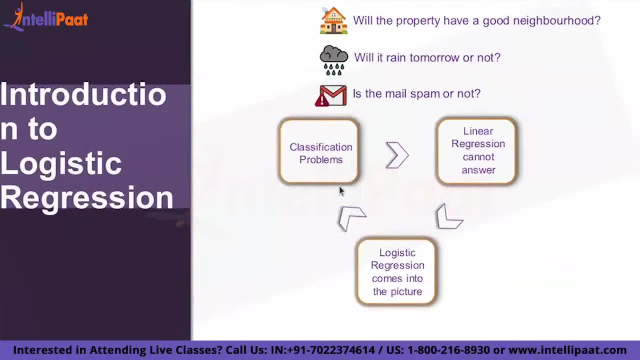 this is like a classification. so, as i told you, will it be noiseless or not? will it be noiseless or not? so those classifications, and along with that, you also have one more example that we are sharing here: whenever you get a email, a email can be a spam email or not correct. it can. 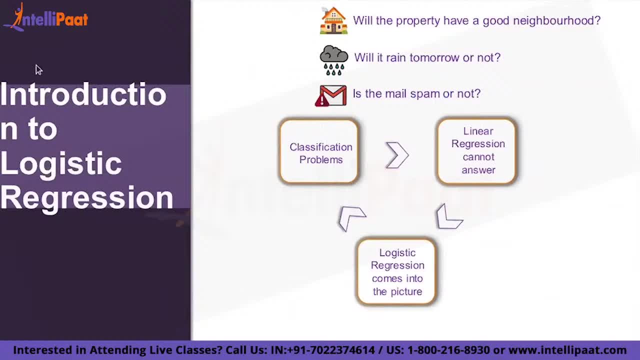 be a spam email or not. so this is something that we are doing right now. you can see here there are some problems that a linear regression cannot answer. so those things, logistic regression will answer. so this is the main objective, correct? whatever linear regression cannot answer, logistic regression will answer it. so this is something that 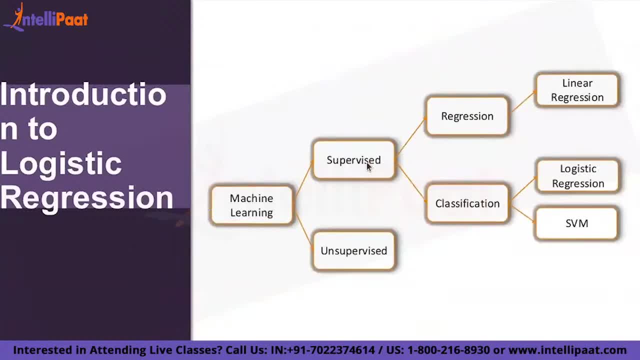 i wanted to tell you now you can see here, machine learning is basically classified into supervised, unsupervised. supervised, you know, is regression and classification. regression: you have linear regression, classification, you have logistic regression, less vm. so today we are learning about logistic regression, right? any confusion still here? what all? whatever i told you there, 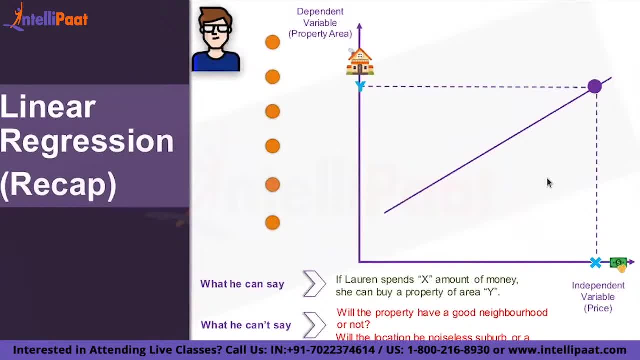 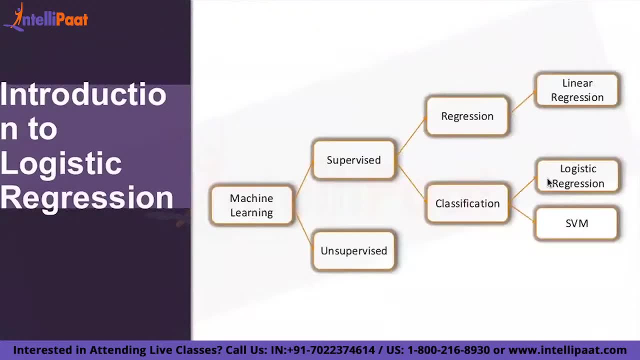 are some things which linear regression cannot solve. for that we are using linear regression, logistic regression, clear no issues, fair enough. so now what we will do is we will go to one step ahead and then see how it is done. right, so, if you can see, statistically speaking, so whatever that. 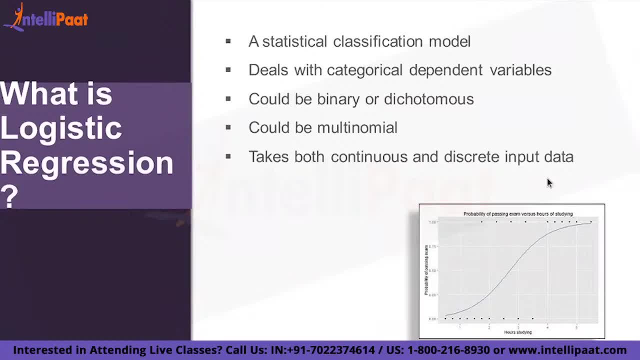 you are trying to do here, if you can observe, whenever you try to do a classification model. so, to start with, you will be using two things, which means binomial, like a yes or no, just to keep the things a little simple. having said that, we are going to do a classification model. 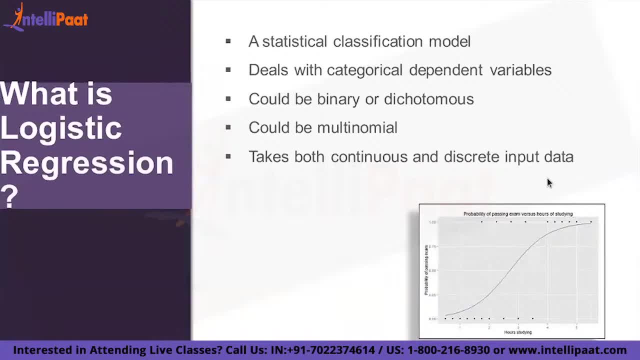 for that. i will see how to do it, but do let me see if it works. drum p. it is great, simple and convenient to develop at home as well. so after OSU starts we will, as it will be possible. but primarily it has to recognize that it is a well set up on. having said that, 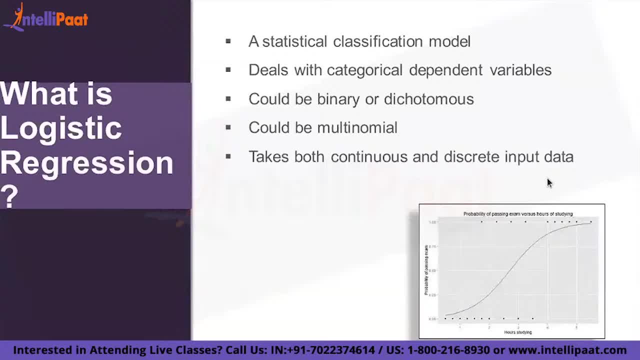 binomial things is what? something that we are trying to do. so whenever i say a binomial or whenever i say it is like two outputs you get, you will be able to understand or probably get to see two places where you get out, if you can observe linear regression. in linear regression we had a 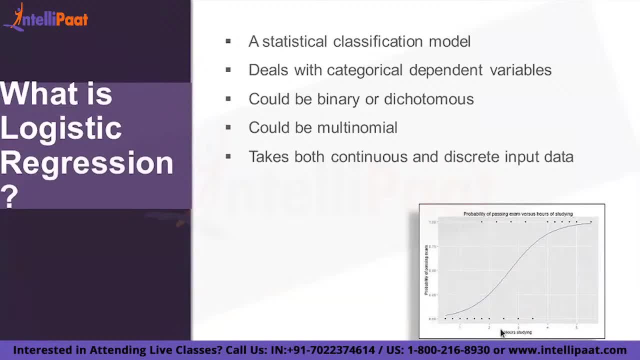 scatter plot, but in logistic regression we are having a plot, even though it is scattered. you are having data at two levels: one is at zero and one is at one. is it clear? are you understanding it? so, basically, what we are seeing here, if you can observe this image, just i am just showing you an 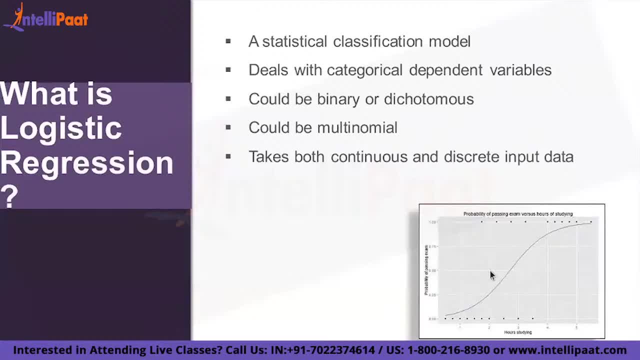 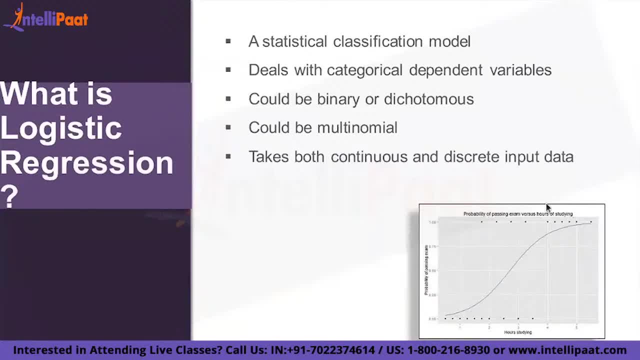 one is at this level, so this is not a normal one. i think i'll show you a bigger, bigger image. but as of now, in a binomial logistic regression, you will have outputs which are two, which means you will have the data which is available in two levels: one is at zero and one is at one. so this 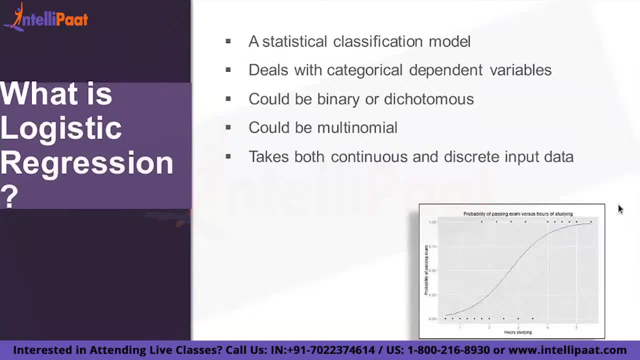 is something which is point number one. now, having said this, you can see it could be binomial, or it takes both continuous and discrete input data right. so i mean, just ignore this. but just the objective is understand that there will be two levels. that is what i wanted to tell you, right. 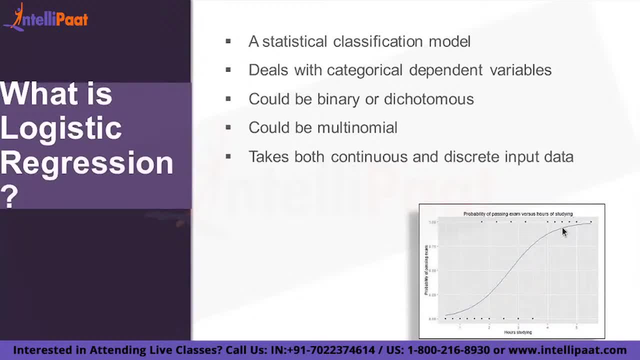 now nothing much apart from that. fine, so don't worry about the details of it. what i wanted to tell you is only this: one, right? so one and zero. dichotomous means two outputs. multinomial means multiple outputs. dichotomous means two outputs- multinomial. 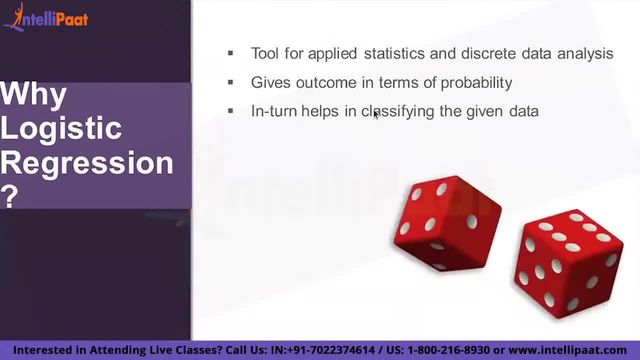 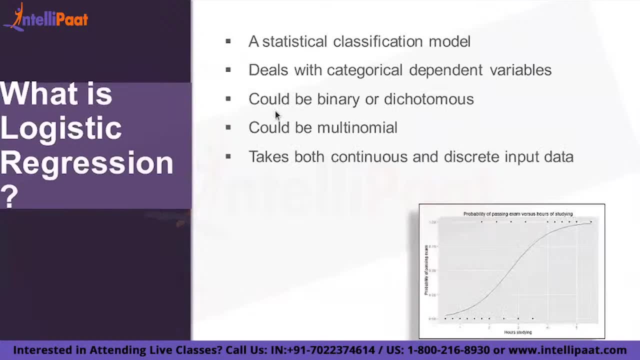 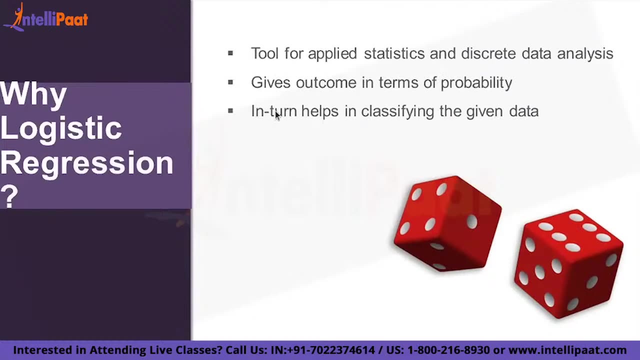 means multiple outputs. that's all now. we will go to the next one. now let us say, for example, you have multiple outcomes here. what you saw here was like a single outcome. now you have something called as a multiple outcome, right, so one is a single outcome and one more is a multiple outcome. 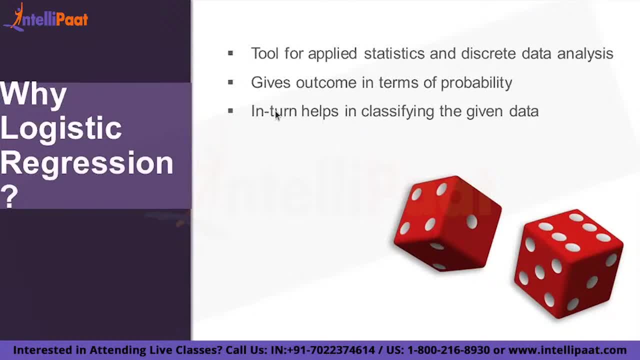 single outcome and multiple outcome. so whenever you have a multiple outcome, your probability things would come into picture, right? so whenever you have a multiple outcome, you will have a multiple outcome, probability will come into picture and then by using that probability, you will be able to define or probably do your analysis. so this is few steps that it will come. 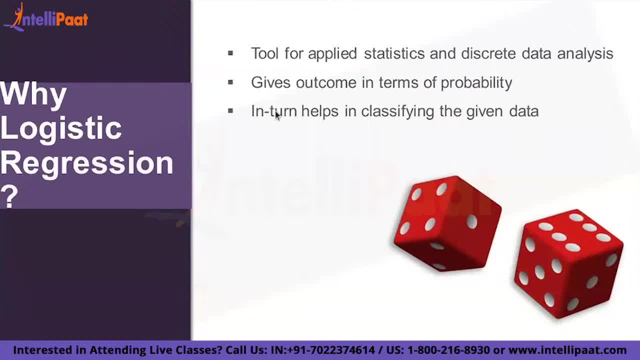 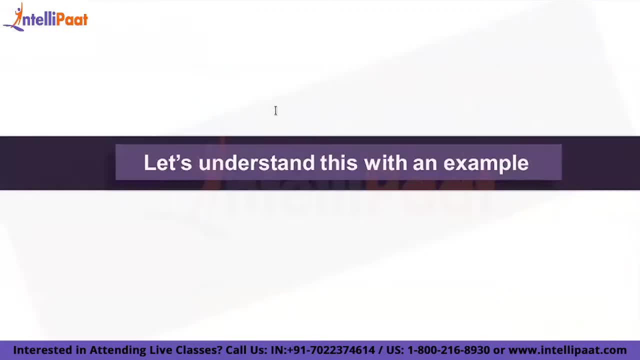 right slowly, we will see how exactly we are trying to do. it will help us to classify the data. so these are some things that we are working on right now. having said all this, we will try to understand this with an example. so what exactly is the example that we are? 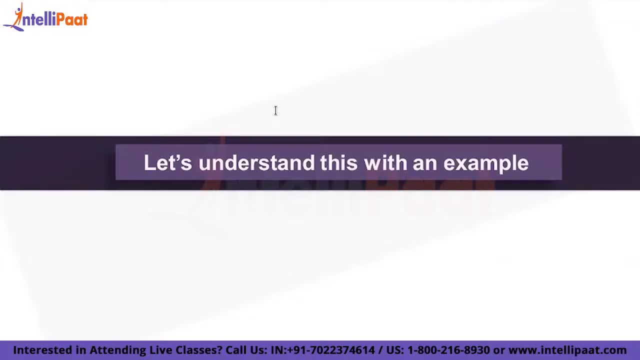 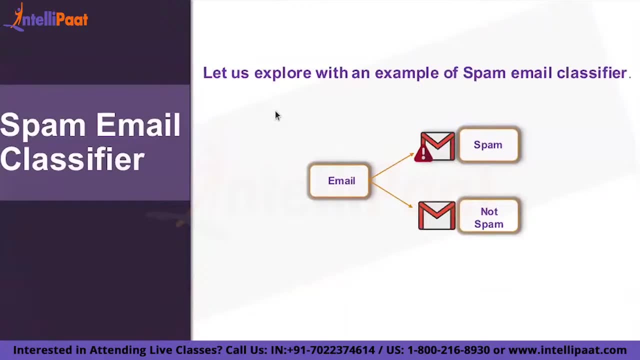 looking at. so we are looking at example of a spam classifier. so you can see, all of you agree that whatever we are seeing, yes or no, is an example of a classification problem. so all of you agree that it's a classification problem, right. so now, since it's a classification problem, so what we are going? 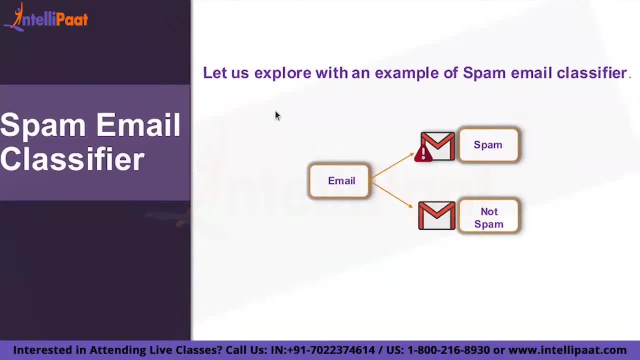 to do is we will see how exactly things would work out here. right, so we will see how exactly we are using it for our analysis. so now, if you are checking this one, we will be having some some kind of keywords, or we'll have some kind of methodology to classify it into a spam or no spam. can someone tell me one or two? 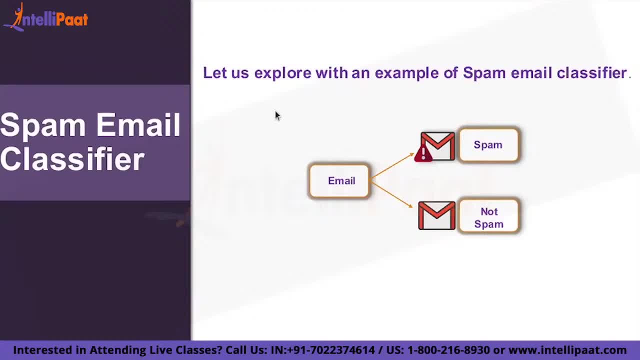 methods how you can classify it into a spam or no spam. just simple methods. so, in case, if you remember or if you know what, how it is done, correct? so there will be some keywords, as you are rightly saying. there will be some keywords which are going to be classified into a spam or no spam. 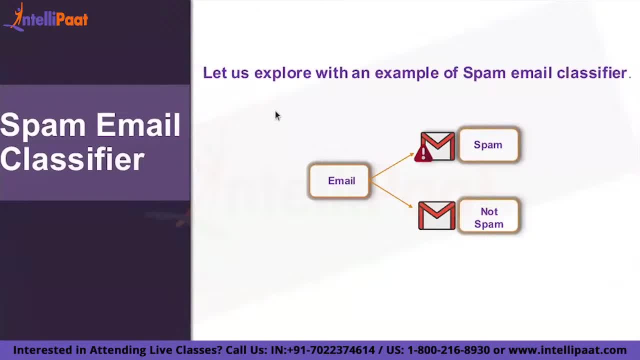 can be used to classify them. so, based on those keywords, we will classify them into spam or no spam, kind of things. so that is how it will work: 100 true, right? so you have a spam, no spam, and how it works we will see in some time, based on some keywords you said here, keywords will play a major. 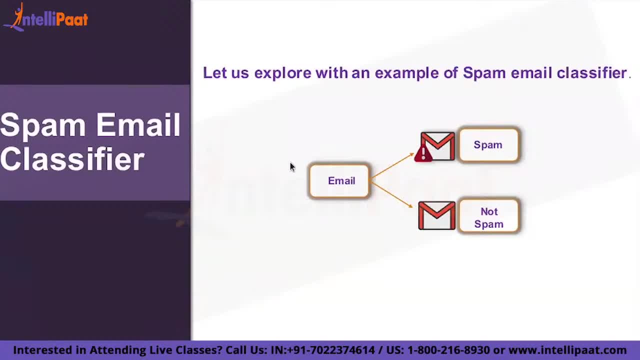 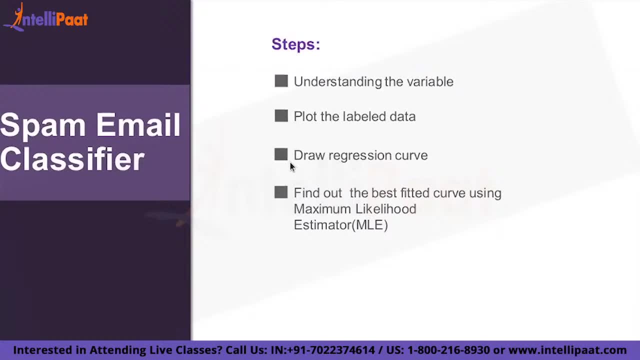 role in classifying it into a spam or no spam. now let me take you through the example in detail, and then we will see how exactly we are classifying it into a spam or no spam. and then we will see how exactly we are going to identify whether an email is a spam or no spam is by using few steps as all. 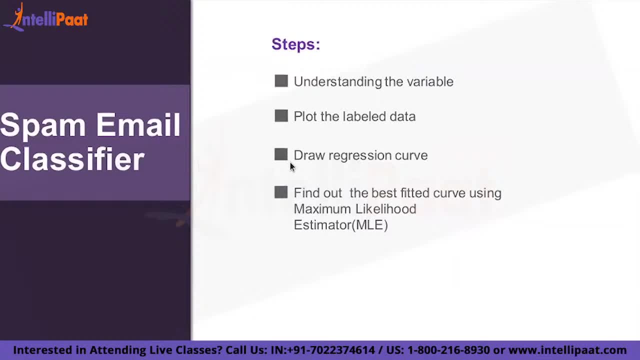 of us know. the first step is understanding the variable. means what all variables are there? how am i going to use them? so understanding that variable. second step is plotting the labeled data. so basically, you will plot the data. third step is drawing a regression curve and and the 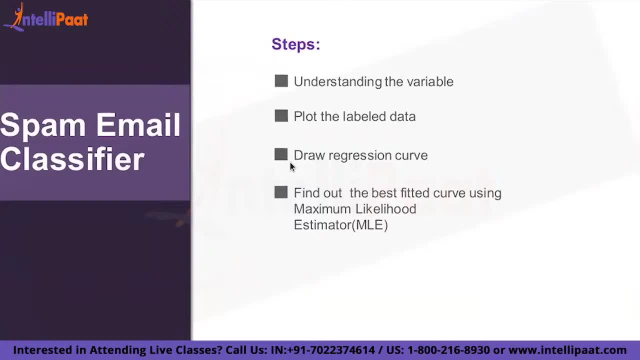 last step is find out the best fitting curve using mle. so mle is maximum likelihood estimate, the estimate which is highly likely. so this is something. this is the steps that you will follow: uh, understand the variable, plot the labels, draw the curve and find out the maximum likelihood estimate. so this is. 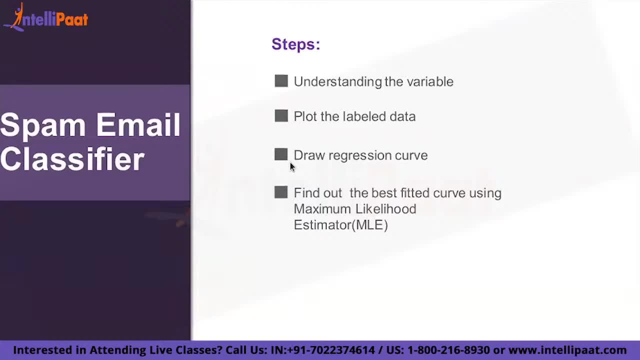 something that you need to be aware of see. logistic regression at the back end is linear regression only. why we call it as logistic regression is because you are using a regression or regression method to solve a classification problem. so logistic regression is also regression. linear regression is also regression, but linear regression solves a continuous kind of a problem. 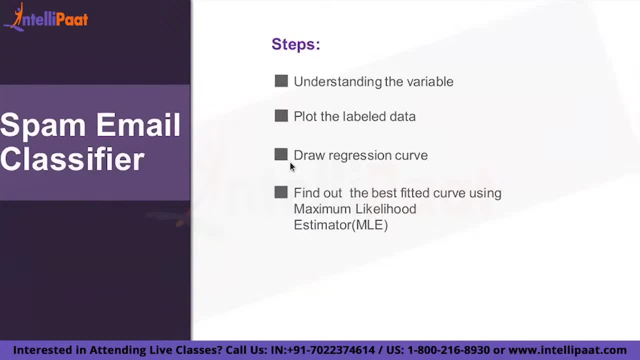 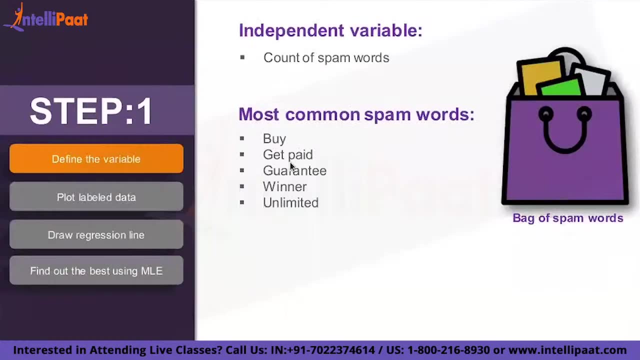 this one solves a categorical kind of a problem. so that is the difference. so we are. we are using this mle to find out. so how we are going to do it step by step, we will see. now, having said this, you can see here independent variable. so these things you need to understand a little slowly. 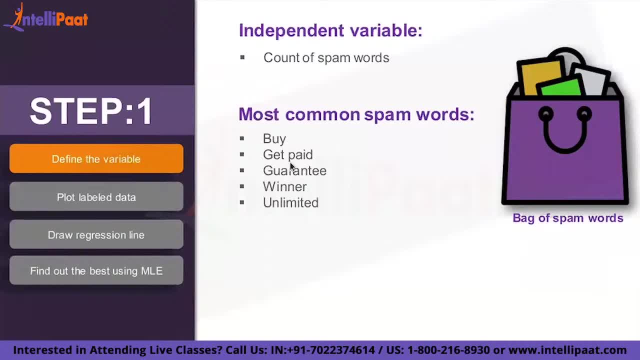 independent variable is count of spam words, correct. so independent variable means: how many spam words do i have? so that is your independent variable. here, the most common spam words are like: buy, get paid, guarantee winner, lottery, credit card. you know, you remember all these things, all of you. 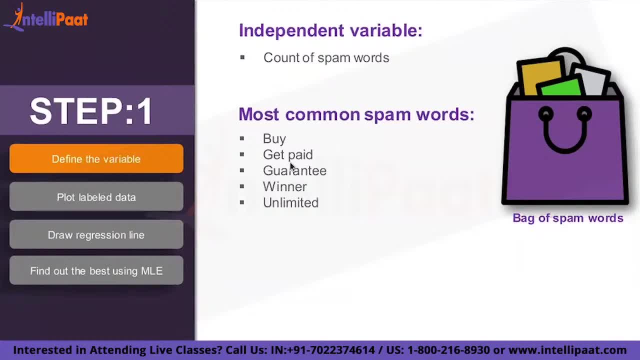 know what all words will be there in the spam mails, right? so these are all some kind of spam mails. so you can see here, independent variable is count of spam words, correct? so independent variable means that we have count of spam words now, exactly. so we have all these things, what we are. 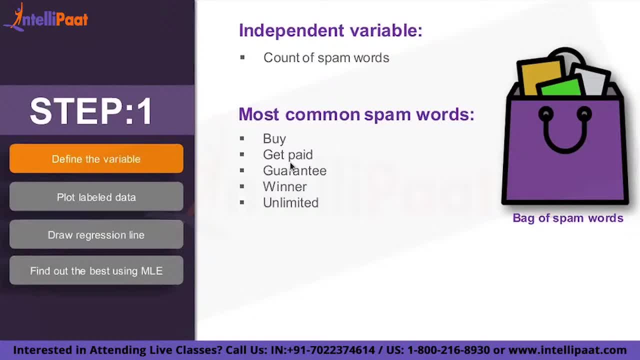 assuming is: all these things will come under something called as bag of spam words. so this is a hypothetical or probably a illusion. okay, whenever i get all the spam words, i'll put them into a bag. just assume that you're putting them into a bag. it is called bag of spam words. so now, 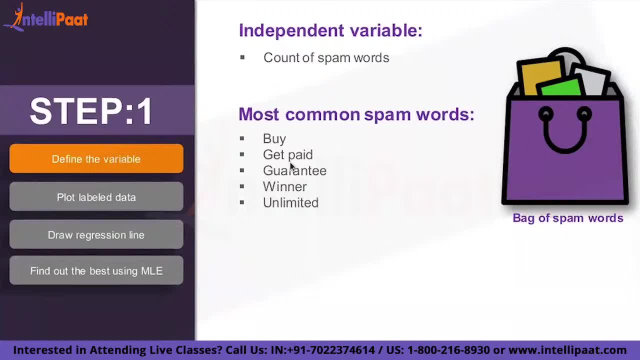 once you understand that this is a bag of spam words, how we are going to use it for our analysis is something that we are going to see now. once you have this bag of spam words, how do we do it so you can see here, this is the spam words. 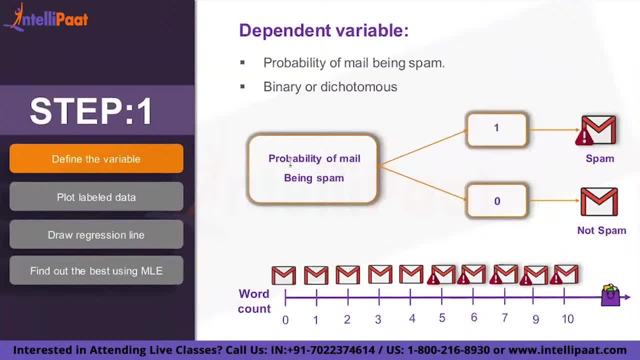 now, the dependent variable is a probability of an email being a spam, which means yes or no, correct, zero and one. my question, simple, is: your independent variables are spam words? dependent variable is a yes or no, spam or not kind of a thing. so now, when you have this independent and dependent, 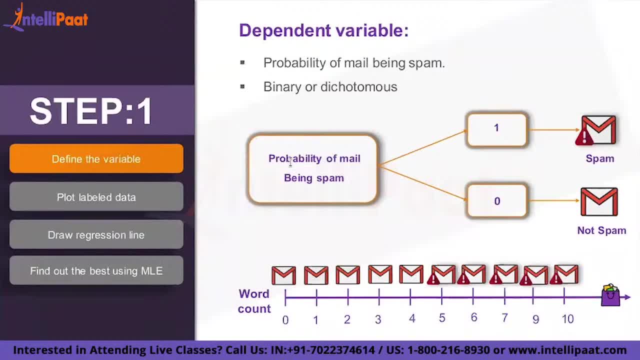 variables like this, how are we going to use it for our analysis and how are we going to do a classification problem? so if you were to see this image which is down word count, the spam word count is there. let us say, for example, you have zero spam words in the mail, is it not spam? 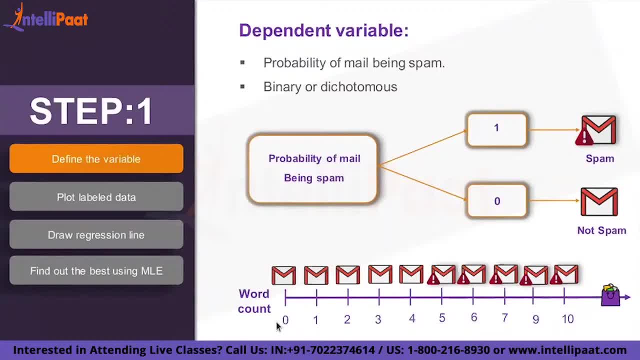 or spam normal mail or spam mail. if there are zero spam word, not spam one spam word. one spam word maybe may not be, no, can be right. so one spam word maybe may not be, but likelihood is very less so some friend might have sent you congratulations on your promotion, so congratulations could be a. 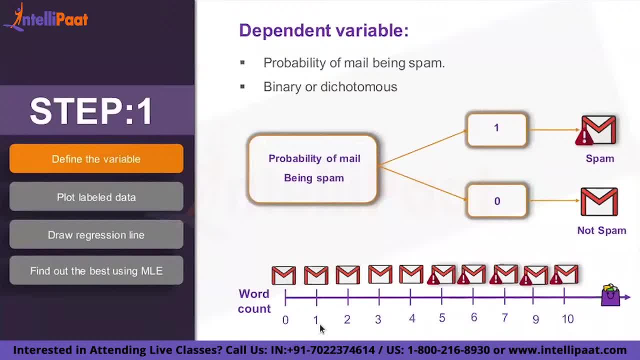 spam word. so usually you would have gone to some place, you would have purchased something, they would have sent you some reward points. or if you use amazon, you will get reward points every day, so that reward point mail also will have rewards. all that, but it's. it may not be a spam. it could be a spam. very less probability of being a spam. 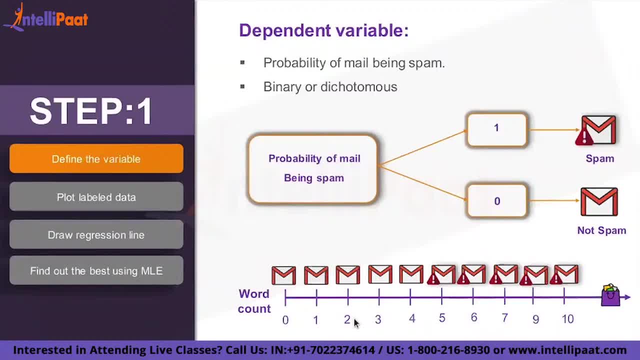 similarly, if you have two words, then the probability of being spam increases. if you have three words, then it is more like a spam mail. if you have four words- doubtful, you have to check whether it's a spam mail or not. but you have five and above, let us say. i mean, i'm just giving you a. 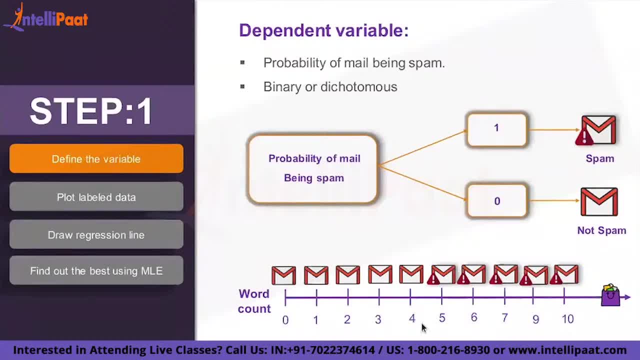 little example. don't go with this number, but just to understand. i'm telling you in case, if you have, if your mail has five spam words, then you classify it into a spam. probability of that mail being a spam is very high, so you put it into spam. so similarly, you have six, seven, eight, nine and all. 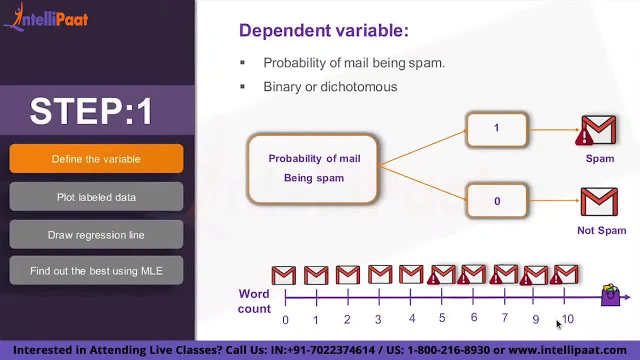 that. so basically, if you have 10 spam words, then obviously it is a hundred percent spamming, correct. so this concept you are getting- don't worry how many numbers to consider, we will see, no, we don't specify it, we will see all that, but understand these concepts first. correct so my 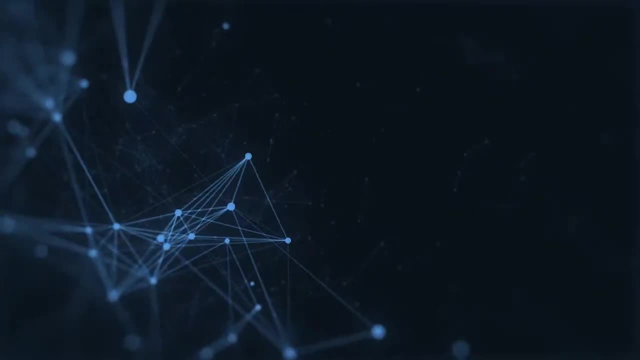 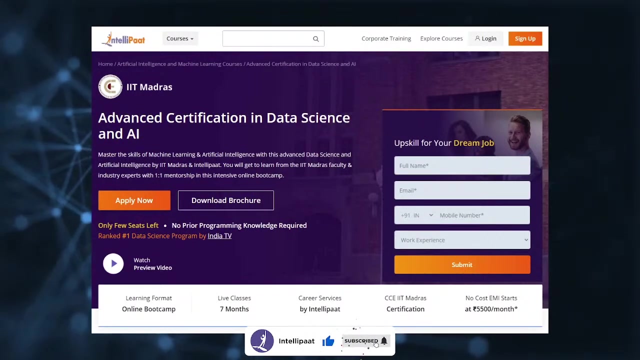 independent variables are spam words. if you want to make a career in data science, then intellipaat has iit, madras, advanced data science and ai certification program. this course is of very high quality and cost effective as it is taught by iit professors and industry experts dependent. 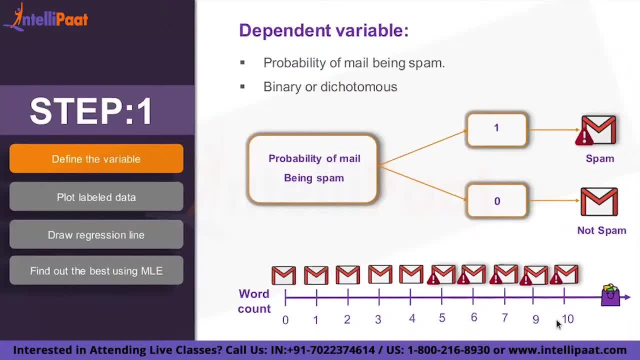 variables are the classified thing, whether it's a spam or not. what i'm trying to do now is i am just counting my spam words: one, two, three, four, five, and all that based on spam words. i'm just classifying into a spam or not spam if the spam words are less. it may not be a spam mail if spam words are high. 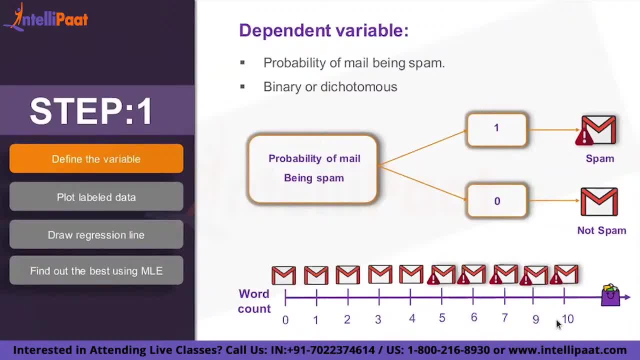 it could be a spam mail. so that is the object. so basically, count of different spam words in a single word. does i mean this is clear to all of you? how do you identify how many spam words, those things and all we will see in the next things, mle? i have not explained it yet, so once we come to mle i will. 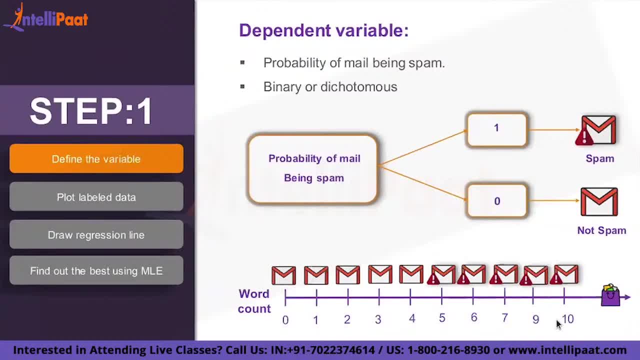 tell you how we are going to do it. we are not doing this using mle, but this is a concept. how we are going to do it is using regression. that i will tell you three points that you should know. here is: independent variables: are spam words. dependent variable: is a mail is spam or not. 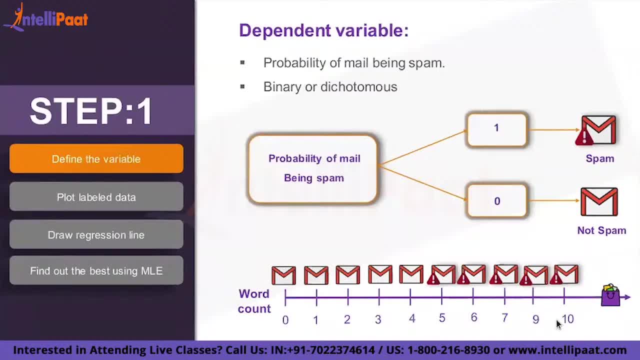 more the spam words, probability of a mail being a spam is high. less the spam words, probability of mail being spam is less. that is what you are supposed to understand. is it clear to all of you? spam word means so whenever you get an email, it can be classified into multiple types. one is a. 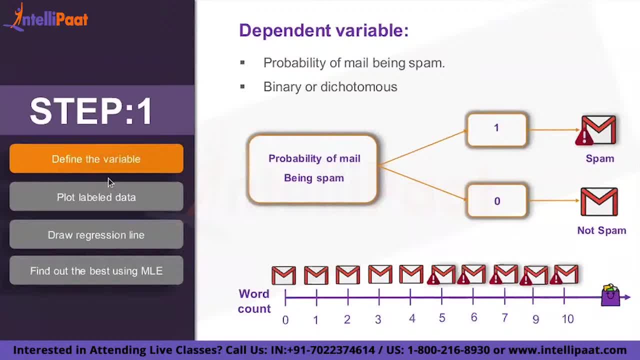 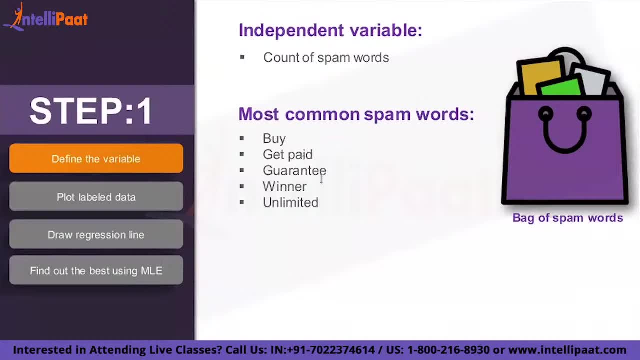 junk mail and one is a normal mail. so junk mail, we call it as spam. so here spam words is: if your get paid, guarantee lottery rewards winner. so all these things are some kind of a junk mails that we will get. yes, so whatever mail it is unnecessary, that one, we will call it as spam. 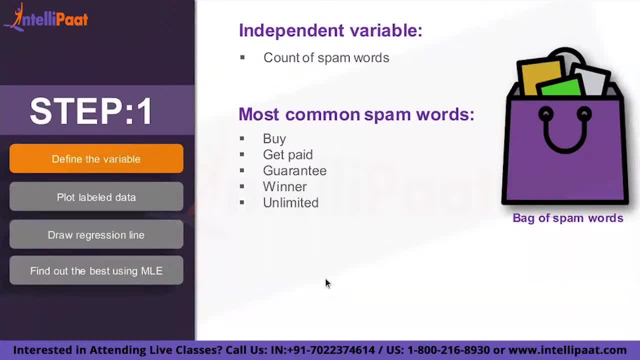 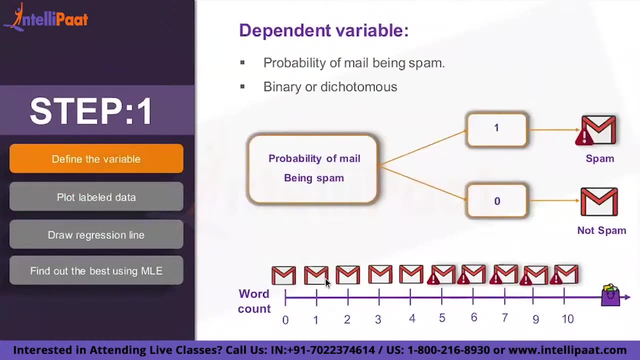 like you will have offer 50 discount by today. you have one, one lakh rupees and all that will come. no free credit card, lifetime free. so they are our spam correct now. having said this, let me take to the next example you can see here. i am just 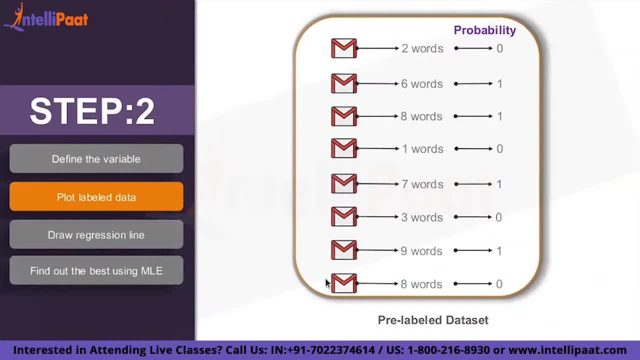 marking mail into a probability of being a spam or no spam using my historical data. so let us say, for example, at today's date you have, let us say, one lakh email ids in your gmail. one lakh email ids in your gmail, correct total in that: one lakh email ids. if you see every individual email, any email with two spam words. 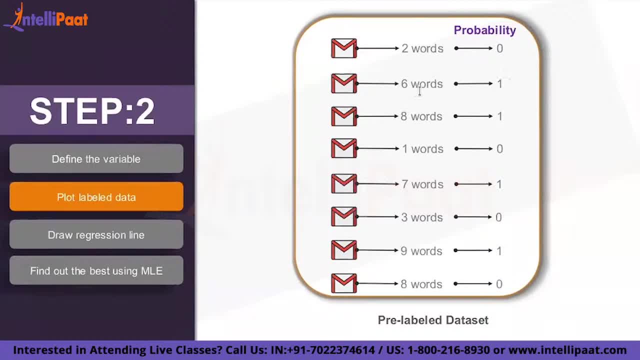 is a normal mail. any email with six spam words is a spam mail. eight spam words is a spam mail. one spam word is a normal mail. so it's like that if you count the spam words in every email and mark it as a spam mail or not spam mail, 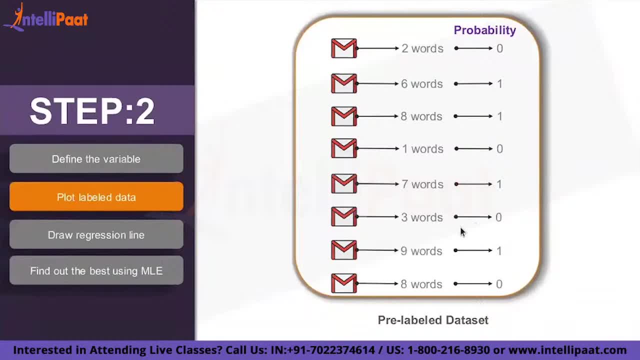 you will get a data set which is ready, so they say pre-labeled data set. but this is how your data set will become. so if you check a mail, let's say, one lakh mails are there right. so one lakh mails are there in that. one lakh mails, you count and then we mark it as spam and no spam based on what it is. 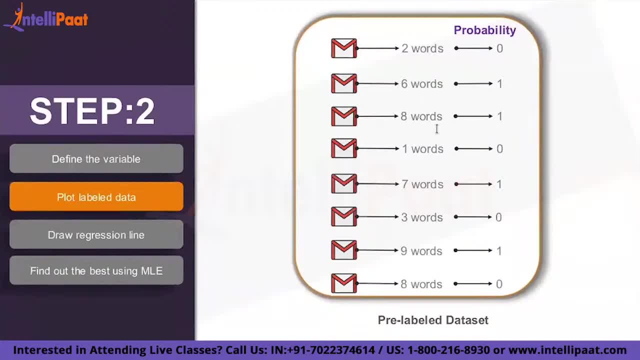 so now why this is there is because most of them will be spam, but few of them may not be spam. also, user will not scan any mails. i'm just giving you how a data set will look. so let us say you have one lakh mails in a mail mailbox. we are constructing data based on two things. we are constructing as: 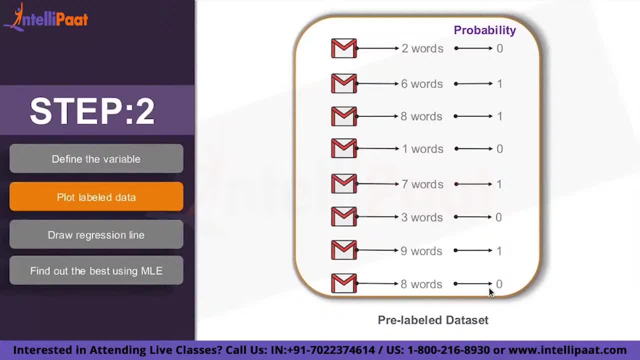 in. we are not literally constructing. data will already be available. so spam or no spam, kind of data based on our work. so what we are trying to do, so one is nothing but words. eight words in one mail, eight words is spam in one more. let us say: 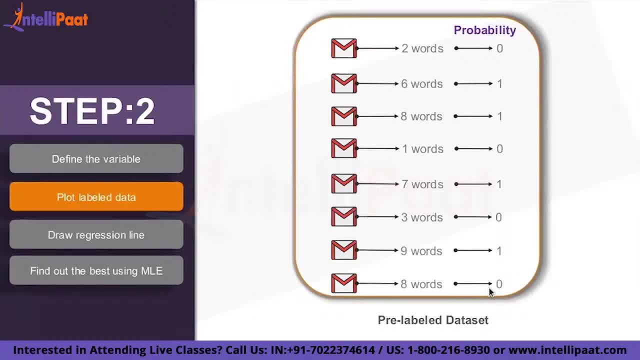 genuinely, you have won a price. so that will sound like a spam, but it is not a spam. so if you really have one, something right, right. so this is how you get to label your mails. so let us say you have one lakh rows. in that one lakh rows, you will be marking few of them as spam. you will be marking few of them. 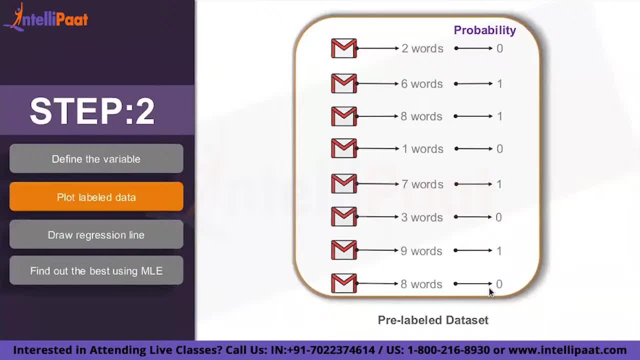 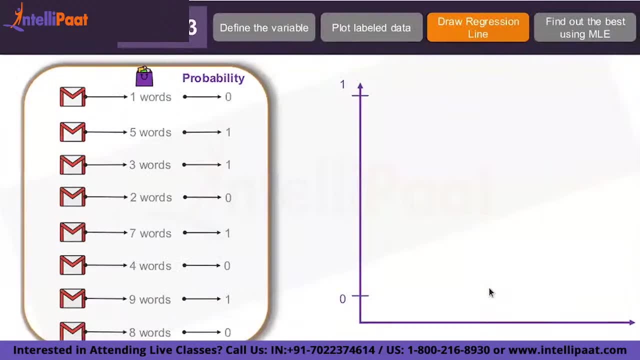 as spam, few of them as not spam. so based on the number of words, it has clear to all of you. any questions? nice, so now this is what i am telling about the graph. so whatever i told you here, this one you observe. i told now this type of graph. 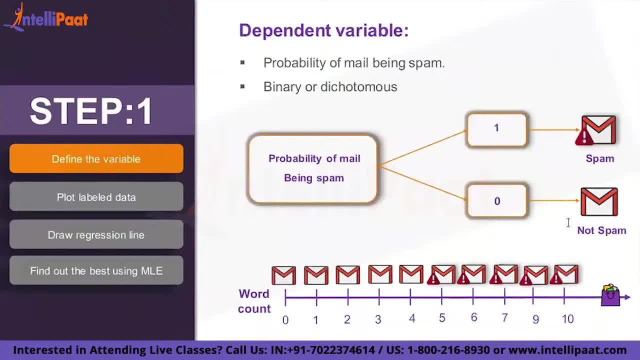 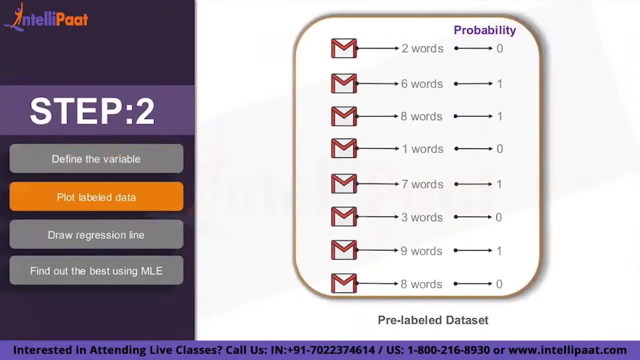 we will do it. any type of word can be a spam or no spam. it's not compulsory that you should have eight. only don't go literally. you can- you can have two words also can be a spam on the mail. so we are just trying to identify it and then we are trying to see how we can classify. 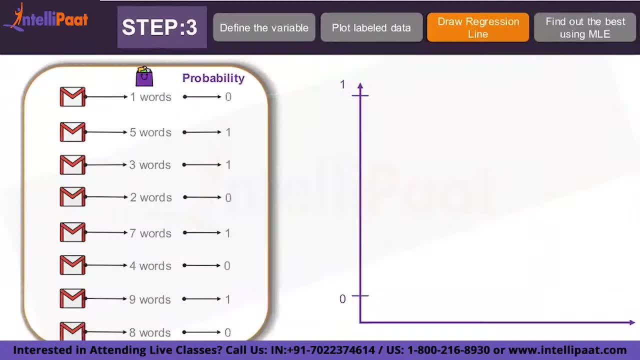 the new mails right now. having said this, you can see, i have my data. i should plot it. so how am i going to plot it? i just take a cutoff, just a assumed cutoff. there is, there are ways to identify this cutoff also, but i just take a cutoff of 0.5 and then what i do is: all the variables are. 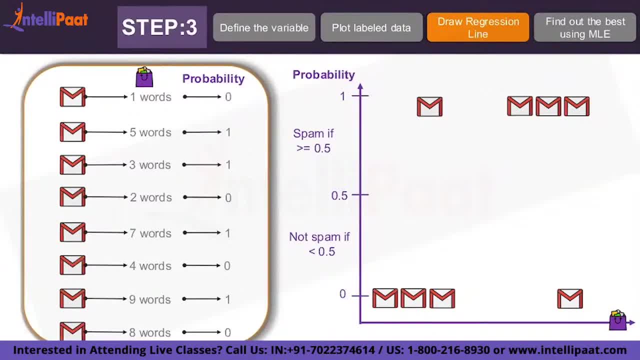 probably right. so what i'm just trying to tell you is: so we can see that when you plot these things like this, you will have some mails which are not spam and some mails which are spam, right? so any questions? how did i plot it and all that. 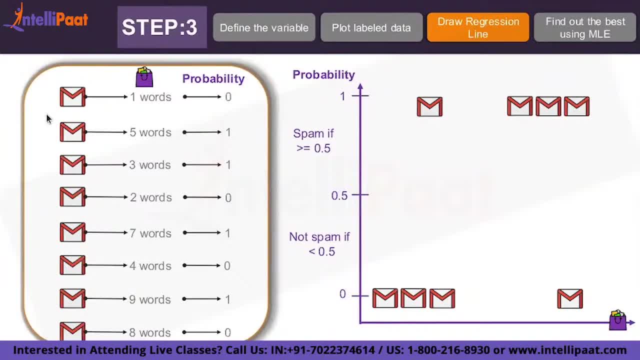 if you have one, i mean, you're just taking one mail. if it is flagged zero, you're marking here. if it is not flagged zero, you're marking based on the words. you can see bag of words. is this probability? is this okay? so let us say: if i have one word, right and then the mail is spam, right. 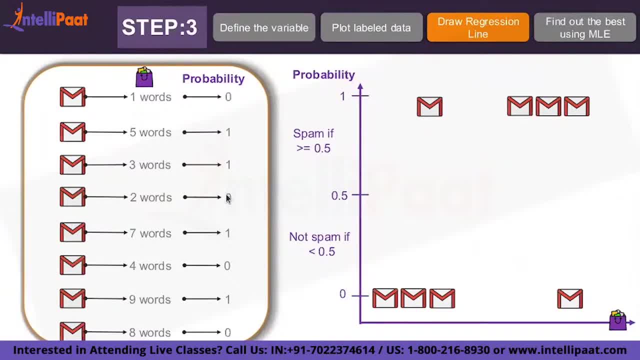 so you have one word and then the mail is spam. how it will be, why it will be, that depends on every mail, right. and then you have two words and then you can see that the name of the EMP which stands for Spoiler here. but secondly, on the real estate, the�I have been the spam for three days and we are 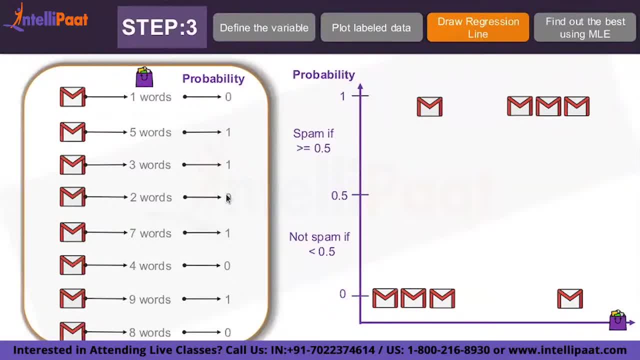 correct. so let us say that one word is: click here to enroll. that is a spam email. no, if the sender is genuine and if it's not a marketing email. even though if you have one or two spam, spam, spam words, it will be classified as no spam. so let us say you're getting a birthday wish from your friend. 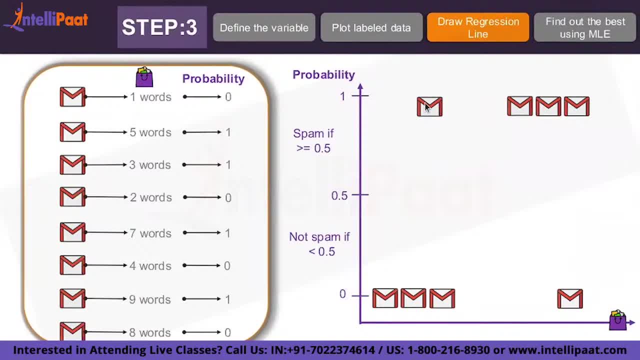 so he's telling: wish you many, many happy returns of the day. congratulations, i'm sending you reward points of amazon per thousand rupees. so that is no spam mail, even though if it has some keywords. but some things can be a spam mails without them. also, like as i told you, i am so, and so from so. 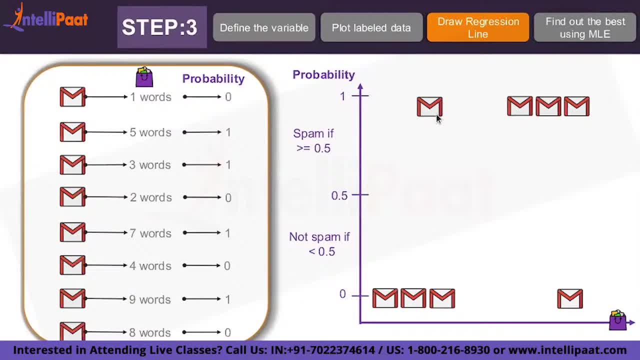 and so country, i am having this much property which i want to give it to someone. so those kind of mails right. so words doesn't define the nature of a email. they will only tell you whether you have a spam mail or not. so that is a spam mail. so let us say you're getting a birthday. 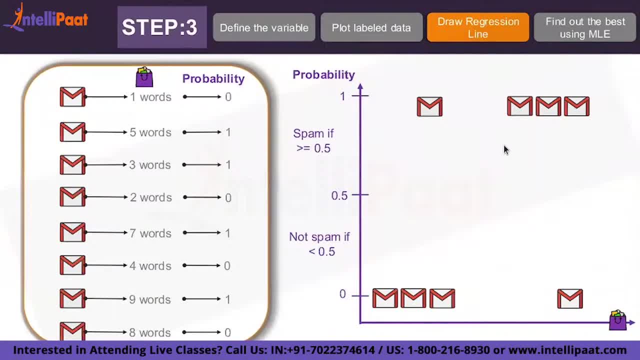 whether it can be a spam or it cannot be a spam with a probability. don't think that if i have one spam word it will be no spam. no, if i have one spam, it can be a spam based on the mail, the nature of the mail. see, the understanding is very simple. i don't know why you're complicating it. the simplest. 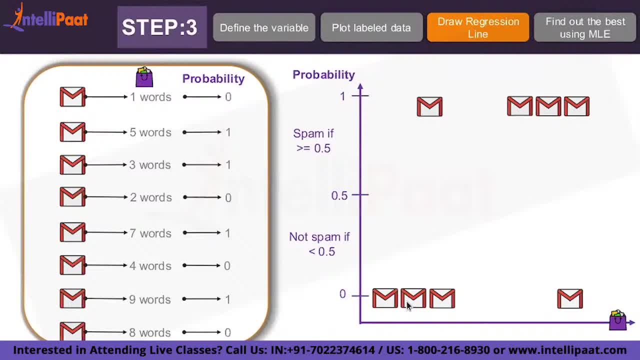 thing is, you will have some mails, out of which you will have some spam words, right so you will have some mails, you will have some spam words. those mails can be classified into spam or not, based on the nature of the mail and based on the spam words. 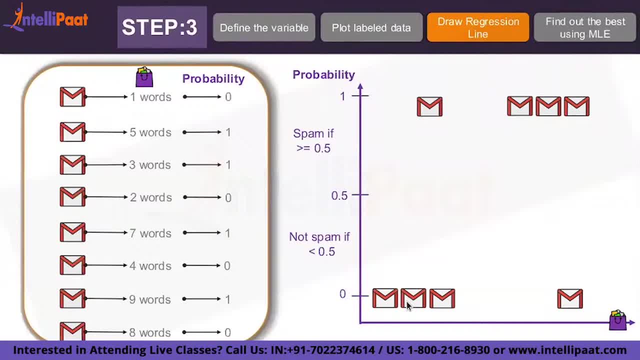 if spam words are more, then the mail is obviously a spam one. there could be some exceptions. if spam words are less, it is not spam. but here also there could be some exceptions based on nature of email. is it clear to all of you? whatever i told you now there is no way to. 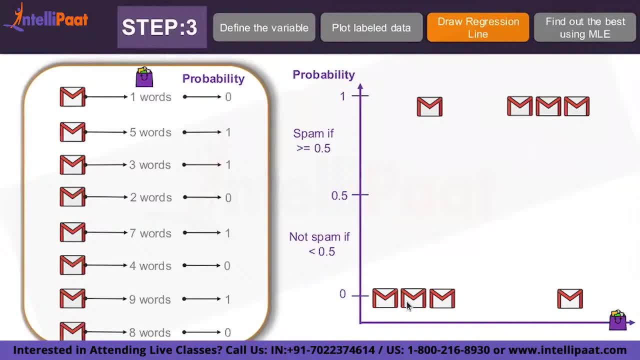 differentiate. very simple example: look at your mailbox. only you will have one lakh emails. in that one lakh emails you will have some mails which are classified into spam, some mails which are classified into normal mails. there could be one spam word, two spam word, any number of spam words. 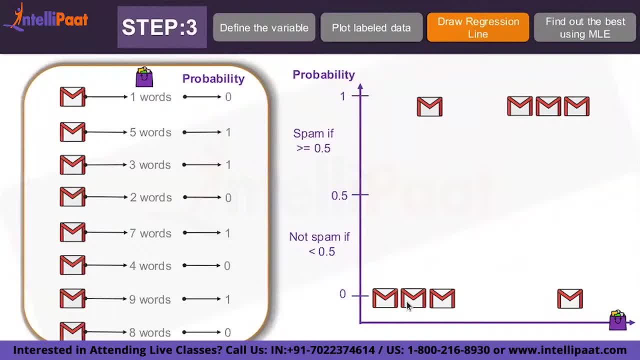 in your mails. based on the spam words and based on the spam words, you will have one lakh emails and based on the nature of the email, it can be classified into a spam or no spam. don't judge whether it is spam or no spam just by using two words, three words and all. that is not the case. 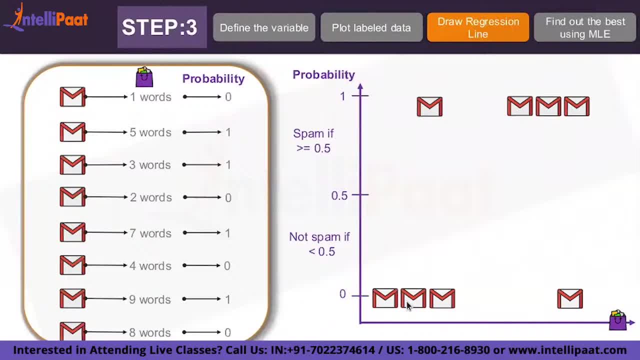 probably it can be a spam. it can be or it may not be. i can have one mail with five spam words. it can be spam or it cannot be spam. also, i have one mail with 10 spam words. likelihood of it being spam is, but sometimes genuinely, i would have won a price which means it is not a spam. understanding all of 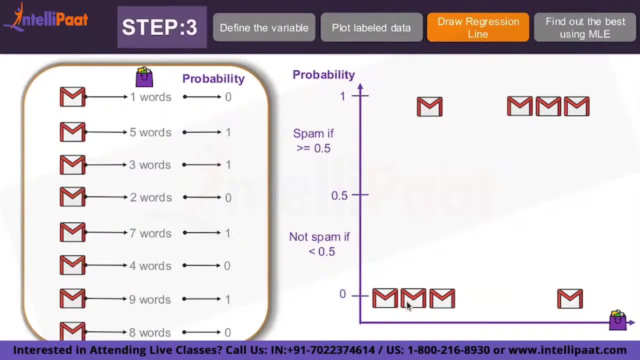 you depending on the context, correct, that is how you are plotting this. there could be one mail with lot of spam words, but it is marked under no spam. there could be one mail with less spam words, but it is a spam one. google's, forget it. google's, you can't go. google's is a very complex algorithm. 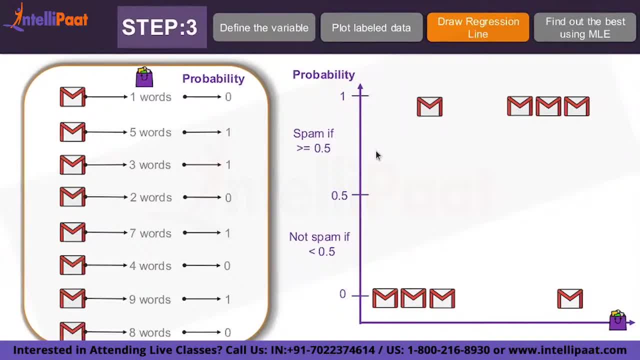 till here any questions. bag of words marking spam or no spam, with some exceptions based on the number of words and plotting them here: this probability ignore. that's what i'm telling. if it is more than five words, then no spam. less than five words, then spam, with some exceptions, obviously. clear till here all. 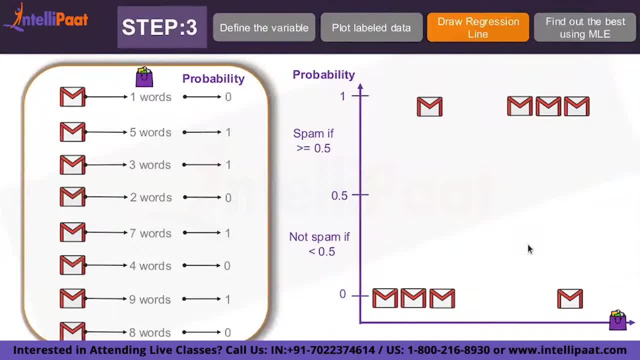 of you are clear till here. no, no one. no one has any issues. don't go to probability, don't go to uh, how do i classify? and all classification is very simple: if i have less than five words, it is no spam. there could be some exceptions. if it is having more than five words, it is a spam. there also, there could be some exceptions. 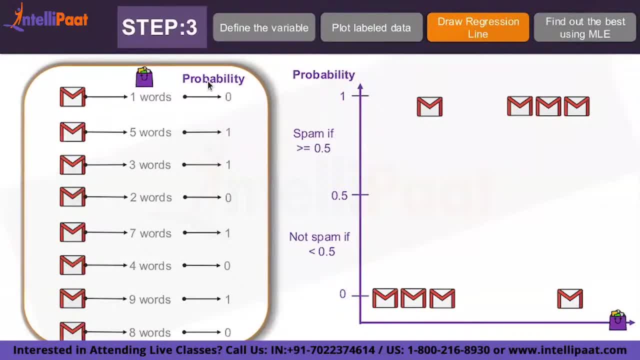 that's all. that is the criteria for my classification as of now. is it okay to everyone? clear, yes, no, clear, all of you. so this is the objective. you classified it into spam or no spam, right, so you can see here, there there could be one. this is this. 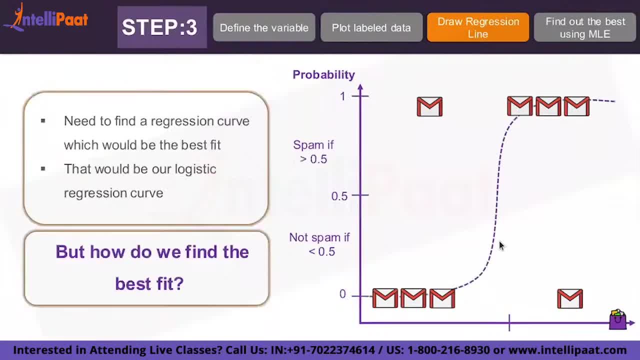 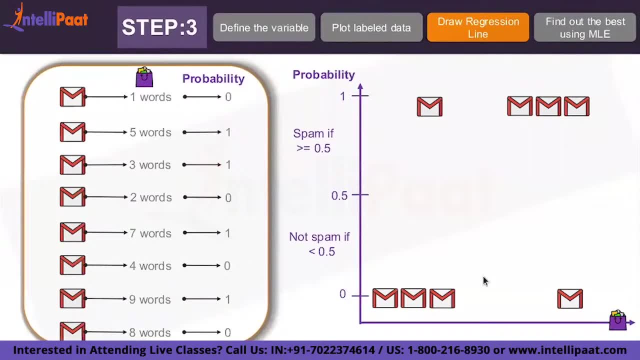 one. this one is something which will be confusing, as i told you. now. you can see this one now. what happens is when i have exactly five words that mail can either be a spam or no spam, the probability of that mail being the spam or no spam is equal- equal probability. it's just an example, for 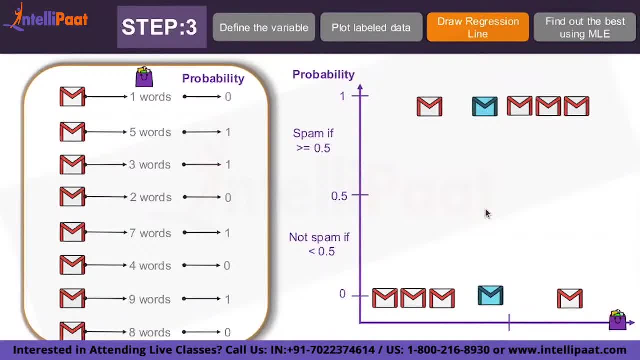 understanding correct. this is clear: less than five words. more than five words, equal to five words. five words is a confusion state. you don't know what it is. it can be spam. it can be no spam. also, exactly, just understand this idea. all of you are understanding this idea. 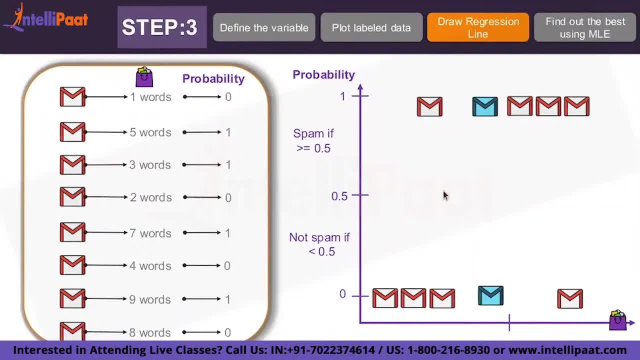 see, you can't plot it at 0.5 because you have only two outcomes: either it has to be a zero or it has to be a one, irrespective of how many words it should be a zero or one, so you don't plot anything in the middle. yeah, we are plotting five in both places because you don't know, right. 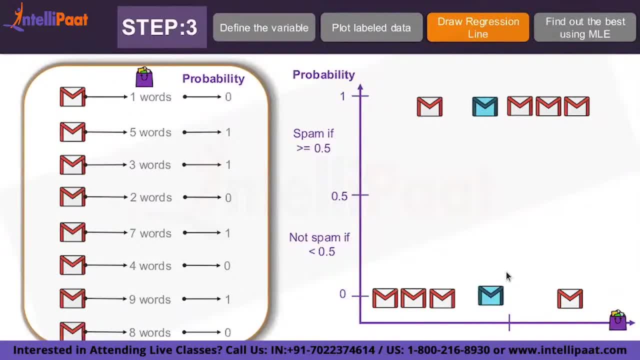 so i said five more than five is no spam. less than five is i mean less than five is no spam, more than five is spam. i have not defined a state where words is equal to five. so is equal to five is a confusion state. if you get a mail with five spam words, it can be a genuine mail or it can be a. 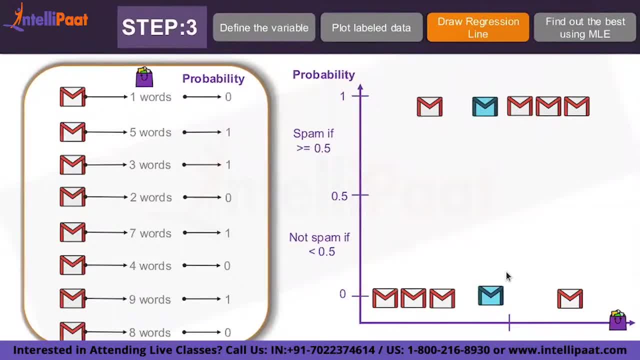 spam mail also clear all of you. so this is the concept that we are supposed to understand, right? so this concept idea is important. so if you get this idea rightly, and then we can go to probability and all that, and then it's fine. so the next step, what we are going to do, is, if you can see this: 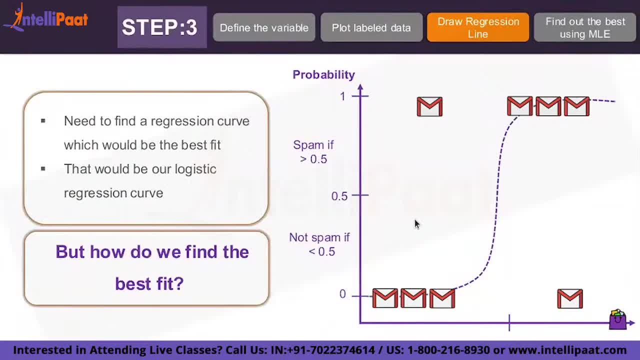 just like in linear regression- right, linear regression- we were able to go ahead and then use it for the next step. so we are going to go ahead, and then we are going to go ahead and then for our understanding, which was we were used to fit a straight line, correct in linear regression. 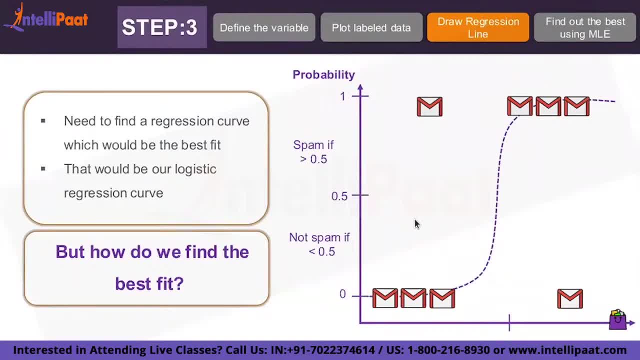 we were fitting a straight line. but here, if we can observe, we are trying to fit a curve right. so we are trying to fit a curve. we are not trying to fit a straight line, we are trying to fit a curve right. so why am i going to? 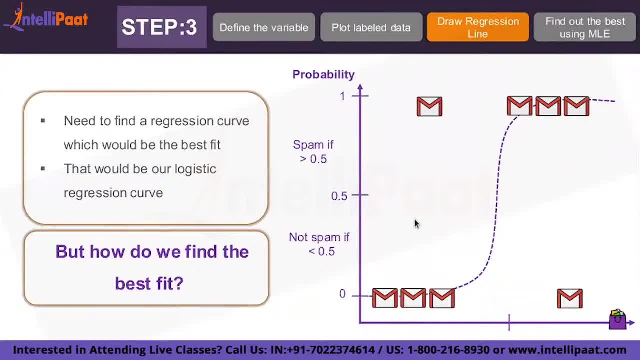 fit a curve is because if you fit a straight line, you may not be able to get a right estimation. that is point number one. and point number two is there are two categories. so, whatever you are seeing, there are two categories and then want to, if you want to like, estimate for the two categories. 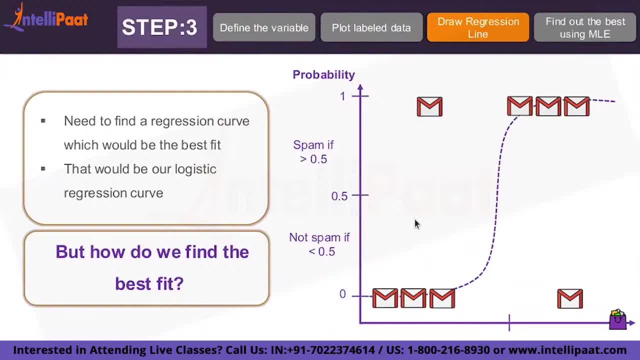 right. if you want to estimate for the two categories, you can do that right. so if you want to estimate for the two categories, you need to fit function which will address two categories. so straight line can address a continuous one. but what this thing does is it can address two categories. 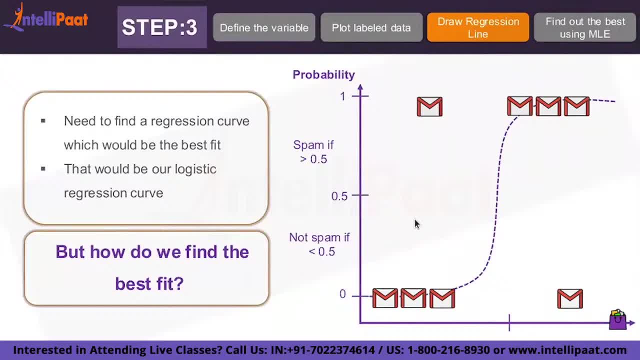 right. so yes or no? so those kind of two categories it can address. so that is something what you are trying to fit it now. is this clear? why am i using a curve with whatever i explained to? if i use a straight line, you cannot address for all of them. so if i 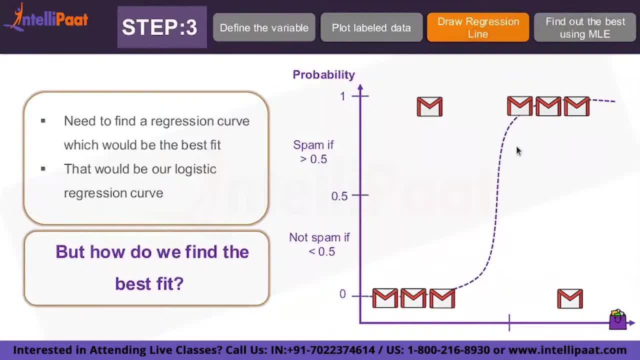 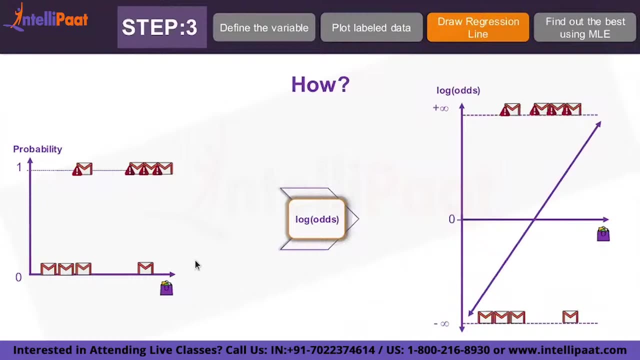 want to address for zeros and at some point in time i need to address for one, because there will be two categories. i'll be fitting a curve. good, clear, understanding it. so this is step number one. now we were seeing we have something called as logistic regression. so this logistic regression, 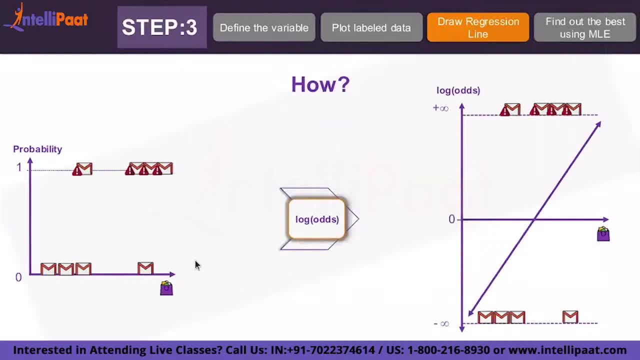 whatever we are seeing here is a logistic regression. so this logistic regression is a logistic regression we are seeing here. if you can observe, there are multiple things. one is a log of odds and the other one is see how we are going to fit this. we are taking probability. understand this. i will tell you. 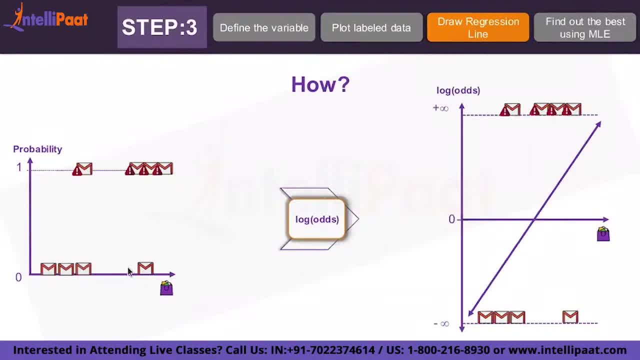 slowly, you are taking zero one. zero means not spam, one means spam. to estimate this, i'm telling you there is something called as a logistic regression. so, irrespective of what we are trying to do, it is a regression correct. irrespective of what you are trying to do, it is a regression correct. now, if you want to do a regression, we are supposed to go ahead and then. 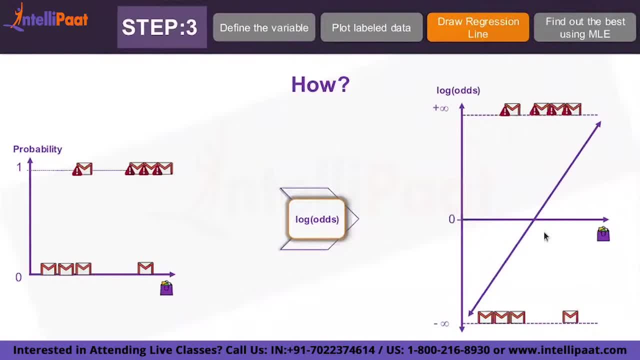 use a line. so that is what: linear regression. so regression means you are trying to find out a straight line request. now how am i going to identify this particular function? so where we were trying to get a sigmoid curve kind of a thing right. so sigmoid as in, we are trying to go ahead. 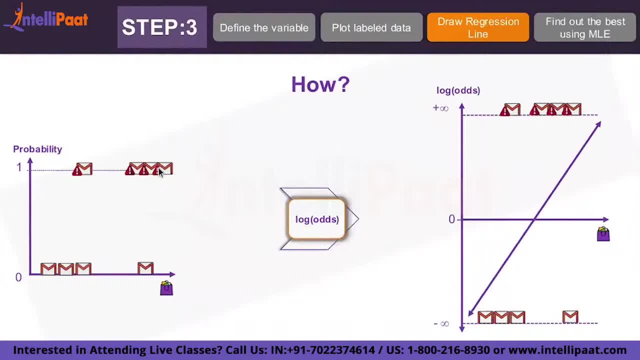 and then get a curve s curve kind of a shape. and now we are just going ahead and then finding a log of odds, right? so we have a sigmoid curve and also we are trying to buy a log of odds. so how are we going to achieve that? so we are going to achieve that by 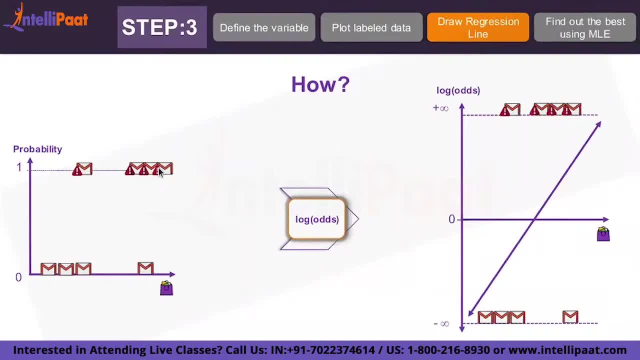 converting our sigmoid curve into a regression problem and then fitting it into our probability. so these are two things that we are able to achieve right. so this is something i wanted to tell you, and then we will try to do this. fair enough now what we will do here, if you can observe. 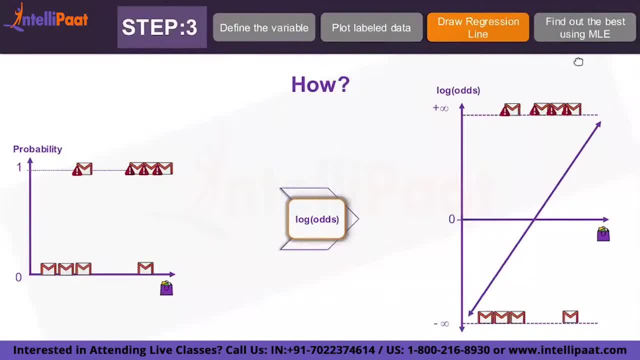 is, we'll just go ahead and then check how we are going to achieve this, so i'm not going to use much of the math because it may be a little overwhelming right now. at this point in time, however, i'll be telling you how you will be able to achieve it and then how we are going to do it. 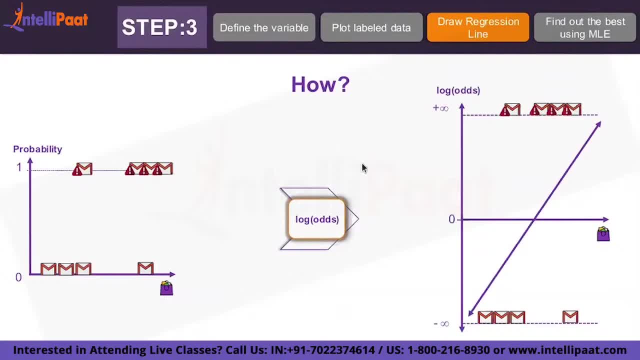 with as less math as possible. so i want you to focus and understand properly. i mean, if you are trying to read the code or write the code, that is okay, just ignore it, no problem, right? so you just need to leave it right now, and then we will be able to achieve it. first thing, 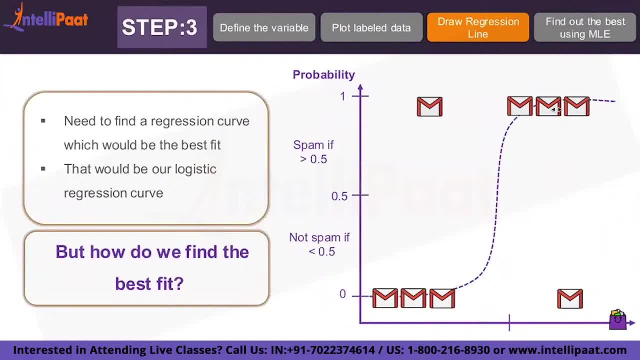 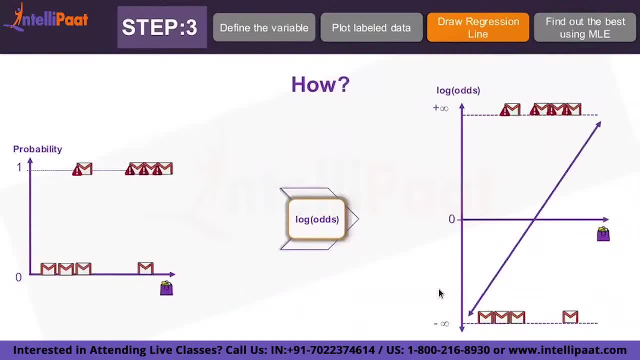 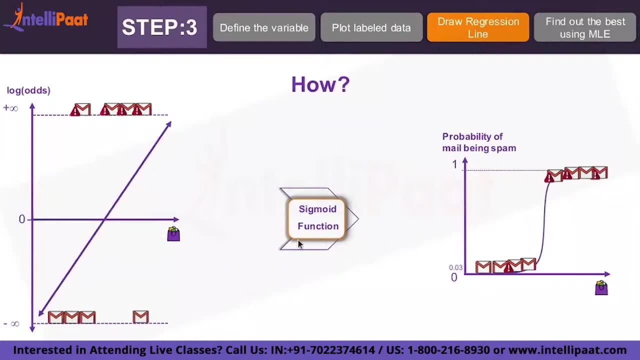 steps. i'll tell you we are planning to fit a curved line, so we may not be able to fit a curved line. so what we were trying to do is we are trying to fit a straight line first and then that straight line, convert it into a sigmoid function. so right, so this is the steps. so 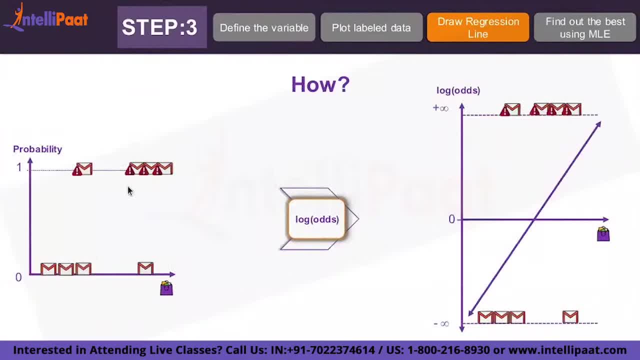 you want to get a s curve here, so that s curve is called as a sigmoid function, so that is a name of that s curve, so i can't directly put a sigmoid here. so for that what i'm going to do, step number one: i am going to convert this particular case, or probably this particular state, into one state. 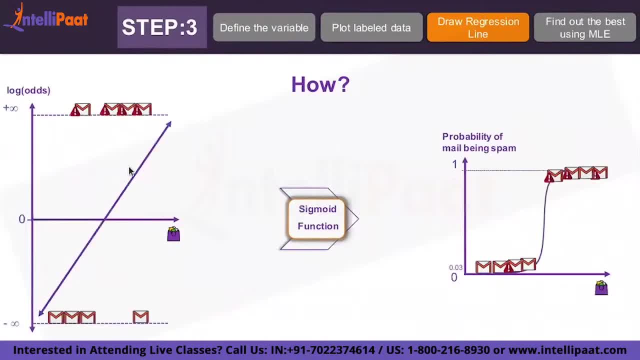 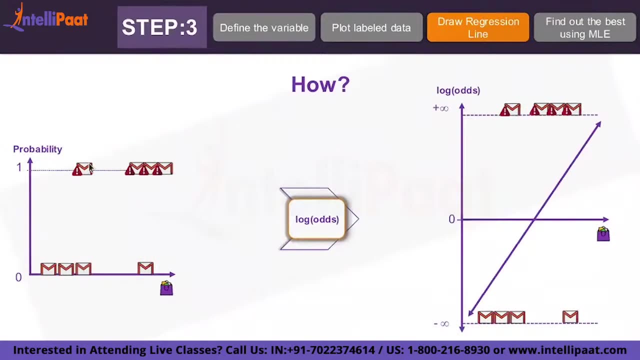 so that means i can fit a line to fit a curve, and then from there i can fit a line and then from there i will get back to sigmoid function. so this is the two-step process. fine, this is clear to all of you. you are planning to go ahead and then mark a spam and a no spam. so you're you're planning to mark. 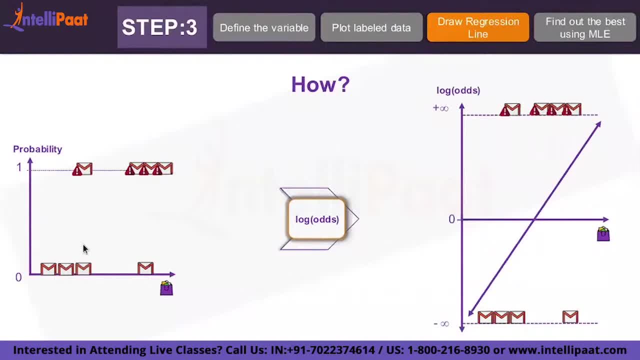 your mails into spam and more spam. in linear regression will fit it a straight line, but here in logistic regression, will not be able to fit a straight line, because because in linear regression we will not be able to fit a straight line, because because straight line cannot address this. so what we will do, we will use a s curve, so which can. 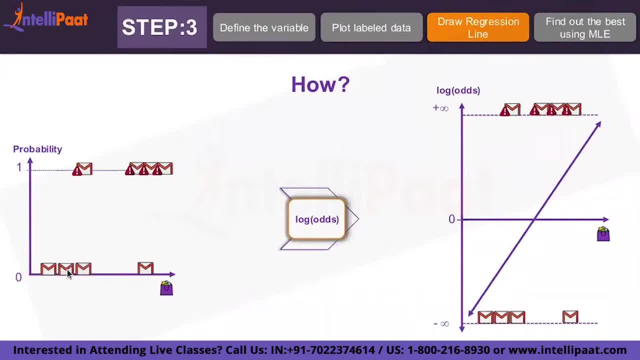 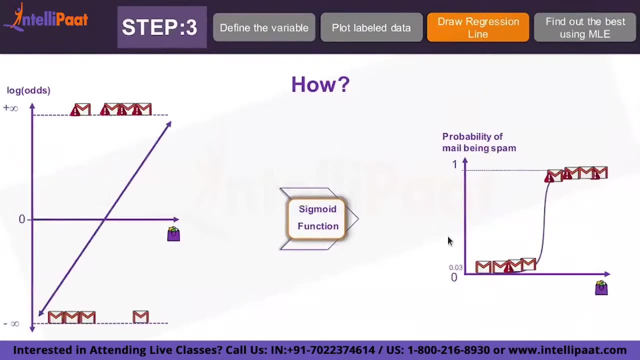 address this. so whenever my spam words are less, it will show it is no spam. when they increase, it will show it is spam. so we are going to fix that. how we are going to fix it is multiple step approach. first step is convert this into a way where you can fit a straight line and then convert. 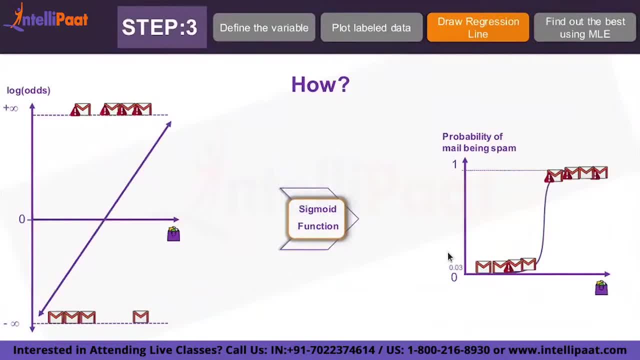 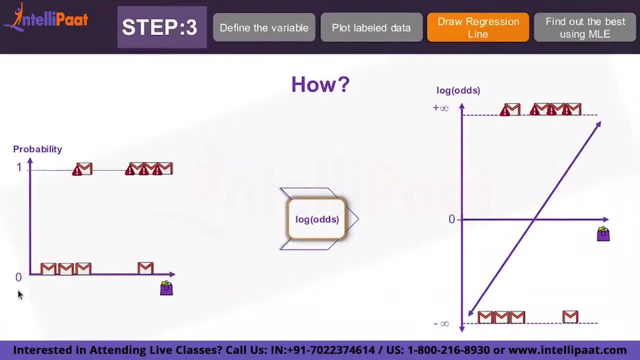 it back into a way where you can fit a sigma. so from straight line to this. so all of you know, x axis is back upwards. observe y axis carefully. here i have zero, here i have one. so here i have zero, here i have plus infinity and here i have minus infinity. so this is one transformation again from. 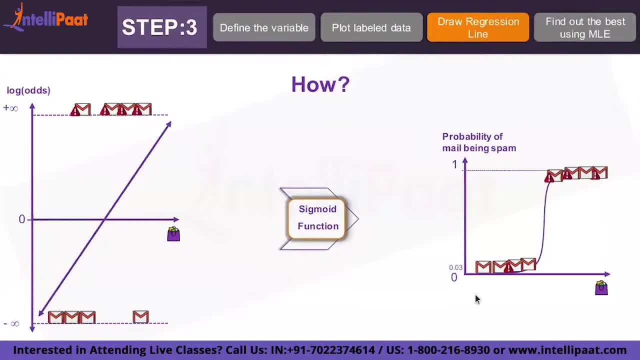 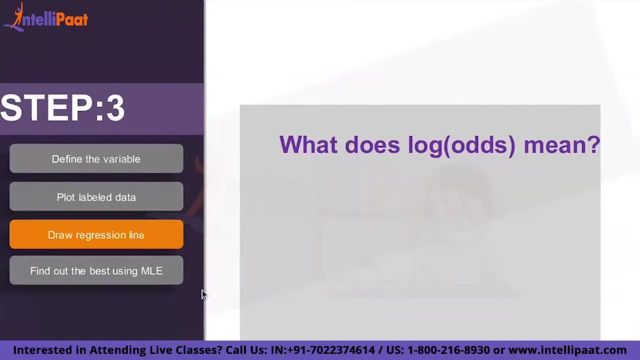 minus infinity to plus infinity. we are transforming it into one and zero. so this is a probability. so probability, probability, probability of male being spam, so using sigmoid function. so this is something that we are going to achieve right now, once you understood that two-step approach, converting into a straight line and 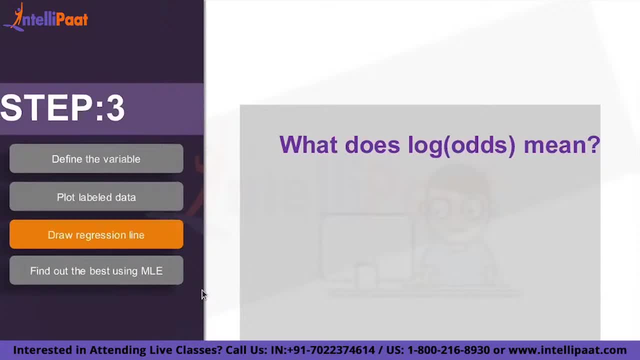 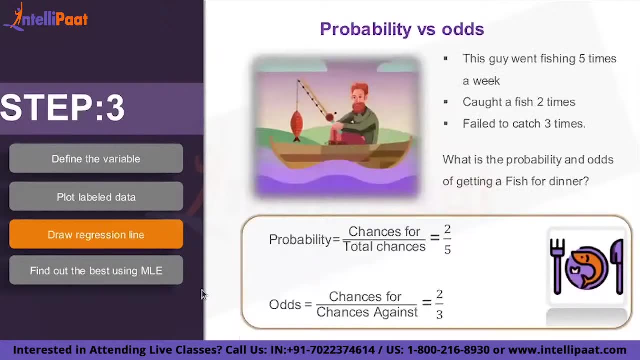 then converting back into this, we will use log of odds. so what do you mean by log of odds? so we will see that. so, basically, there is a simple example right which says a person who went fishing five times a week caught two fishers and failed to catch three times a person who went fishing. he caught two fishes and then he failed three times. 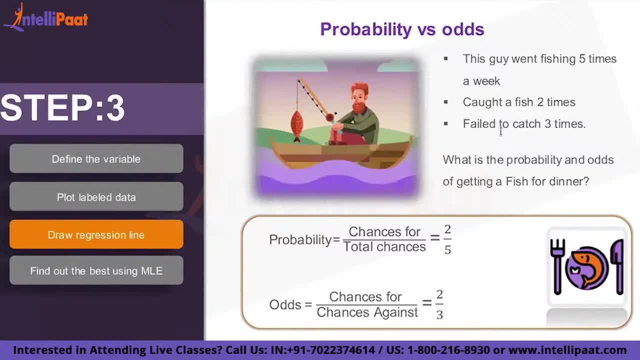 so what is the probability of odds of getting a fish right? so you can see, probability is nothing but chance by total chances, which means how many times you are succeeding in all your trials. let us say you want to go ahead and then, yeah, you are also going for fishing and you are going to catch. 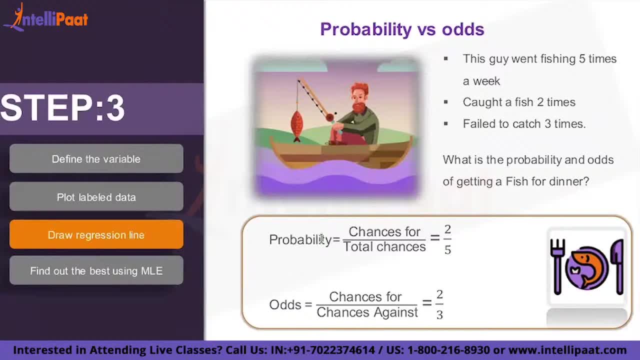 it, which is different number of times. you are going to catch fish. you are going to catch fish, so there is only one kind of probability and this is the probability of success, the live fishing assuming probability of success, the probability of failure. so, basically, probability of success is 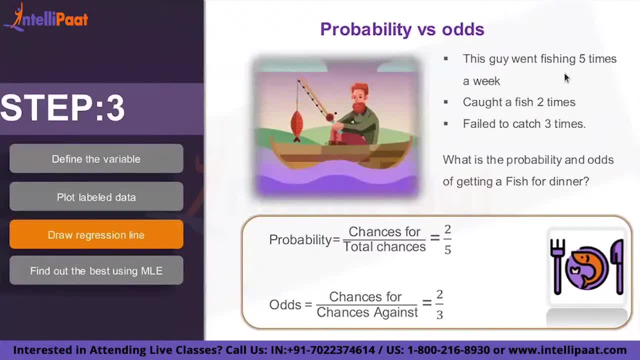 probability of failure is 3 by 5. clear till here, agree, yes or no? yes, nice. so now you understood what is probability of success and probability of failure. now, what do you mean by odds? odds means in your total, in your total attempts, in your total attempts. 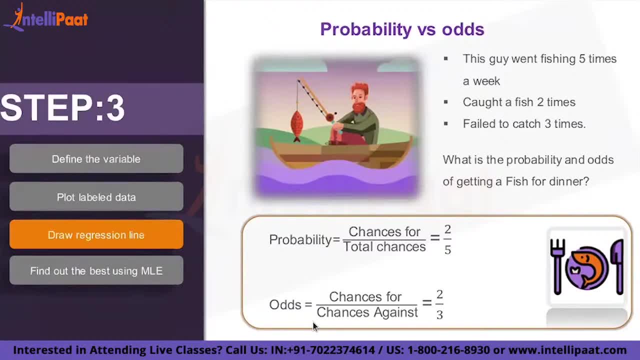 in your total attempts of fishing, how many times you are succeeding versus how many times you are failing. So that is the log of odds. Probability of success and failure is number of wins by total trials. Odds is nothing, but odds means: out of all the trials, how many are? 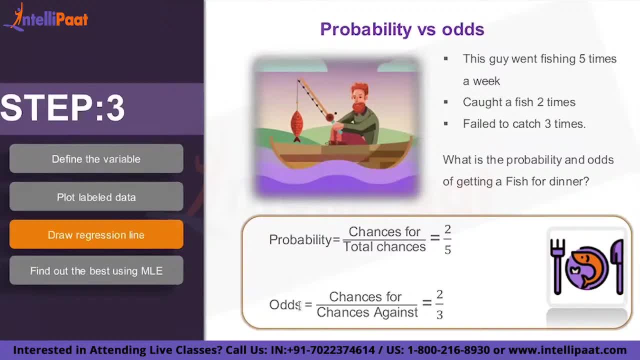 in favor of you? how many are not in favor of you? So that is your odds. This is called odds. Clear difference between probability and odds. Probability is nothing but success or failure divided by total, total number of trials that you have. So that is probability, right? So probability? 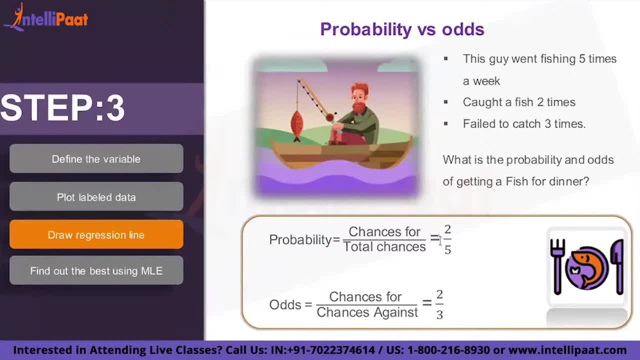 of success, probability of failure. Odds is nothing, but out of all the chances that you are taking, how many of them Are in your favor, how many of them are against you? That is odds. All of you understood this. It's simple. Now, right, Let us go ahead and then see this where it is, and then we'll explore. 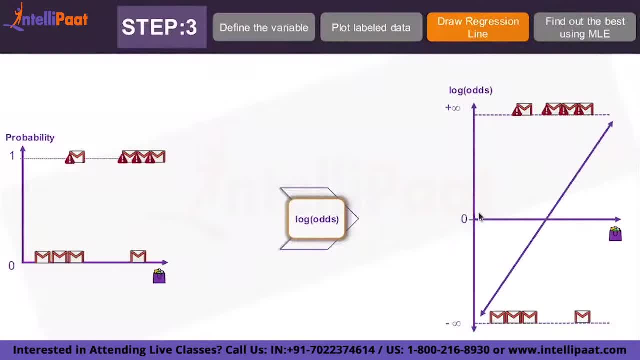 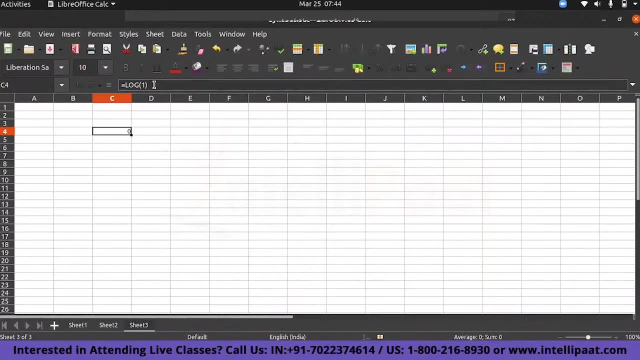 Now let us say, for example- I'm just giving you an example, okay- Log of let us say one. log of one is what? Zero? No, no, Log of one is zero. Observe this. okay, I'll tell you. 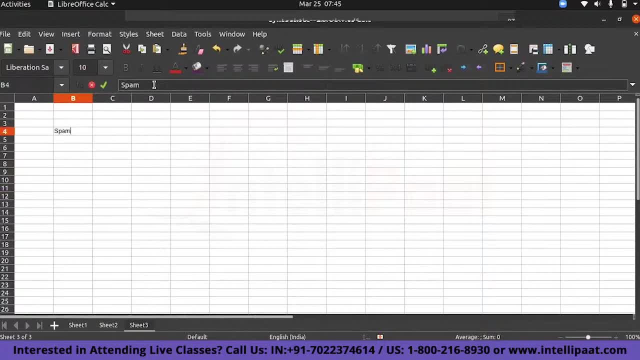 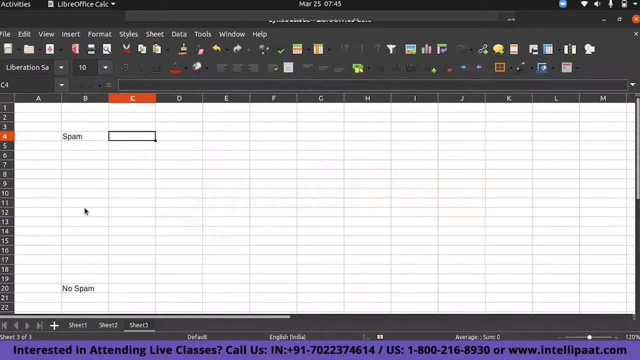 Okay, let me just go ahead and see And then mark it like this: This is spam, This is no spam. I'm just want to tell you the concept clearly Now. let us say you have this particular spam and no spam. Assume you have how many here. 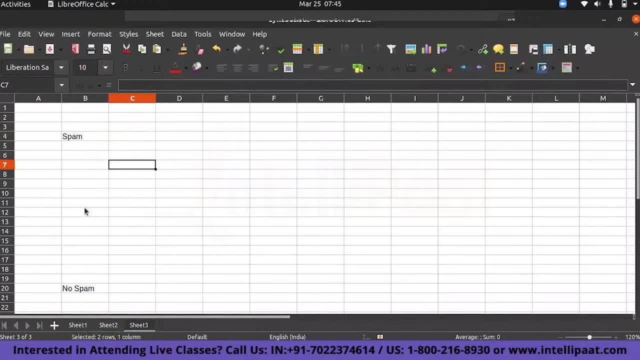 total how many it will come. Let's say I mean n number of things, Let it be like 10 or 15.. I'll take five, five by five here, okay, Sorry, Okay, I'll write it a little different. 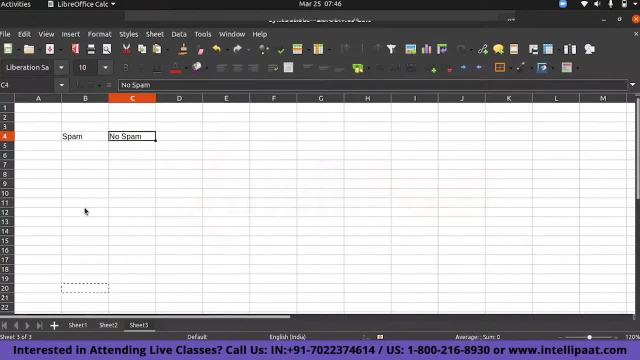 so that all of you can understand it: clear: Spam and no spam. Let us say: I have my total, I have total. assume I'll take it for 20.. 20 emails In this one is spam. two, three. 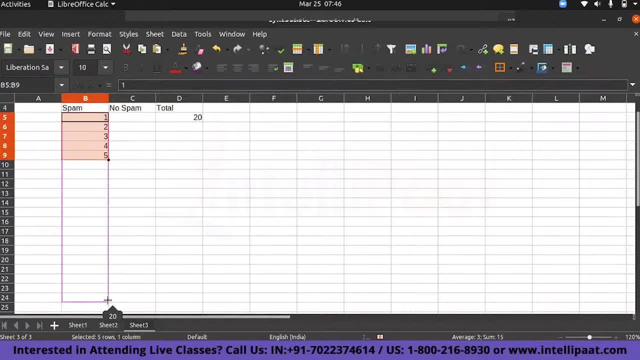 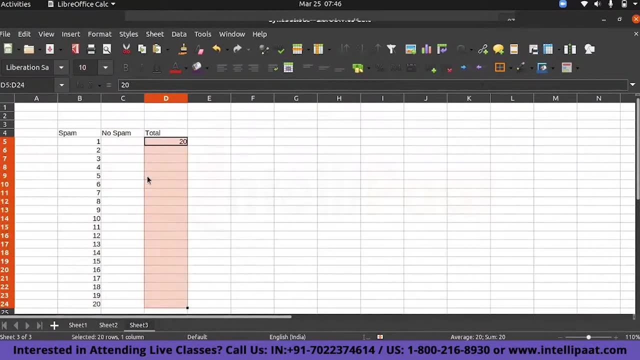 four, five is spam And I'll extend it to 20,. okay, I'll extend it till 20.. Now, if I have these many spam mails in my 20,, how many of them will be no spam? This minus this. 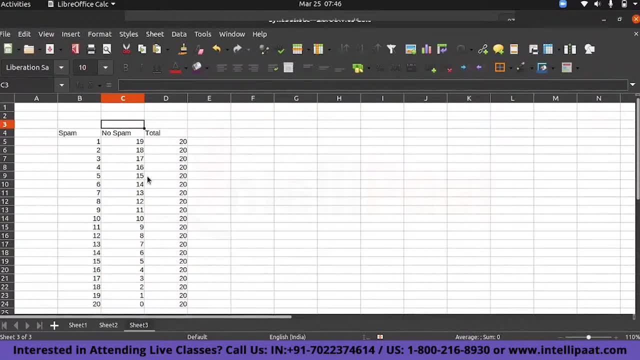 Correct, This is my no spam. Correct, Agree All of you. This is spam. This is no spam Here. what I'm trying to do. the next step is odds of spam. What is my odds of spam? Odds of spam is nothing but spam by no spam. Correct, One by 19.. This is my odds of spam. 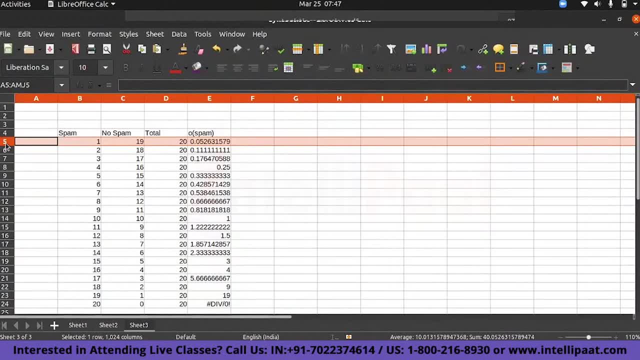 So I just need to add another line Here. this is really important. There could be no spams. also, There could be 20 spams. I mean, 20 no spams is equal to this by this Correct. Fine Till here. No, this is the number. 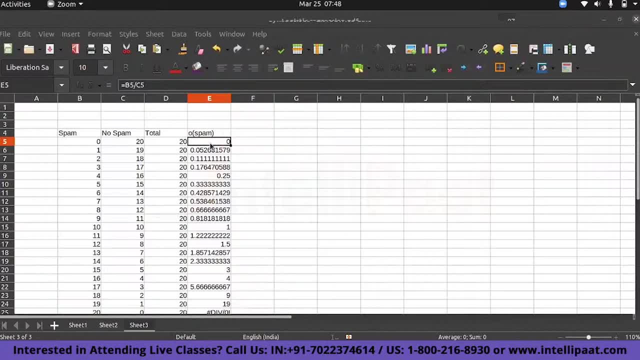 of mails, not the word count: Spam mails and no spam mails. So what I did is I took 20 mails as an example, In that I did all the combinations of spam and no spam, Zero spam, zero, no spam. And then 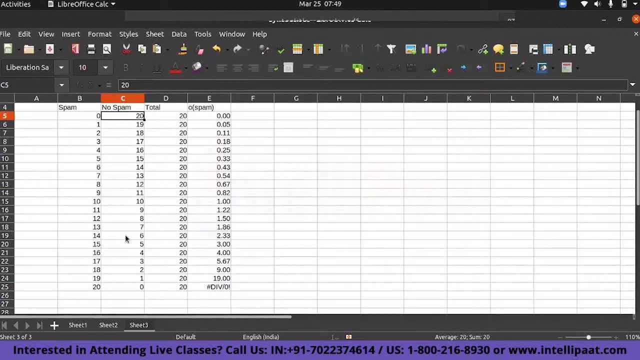 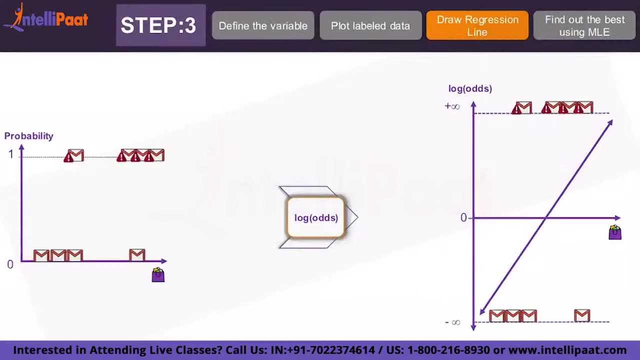 we are just writing all of them. So how many can be spam and how many can be no spam? This is odds of spam. Now if I take, I'll not take odd of no spam Not required. So if you want to do an odds ratio then you might need, But anyway, let us take that also. No issues. 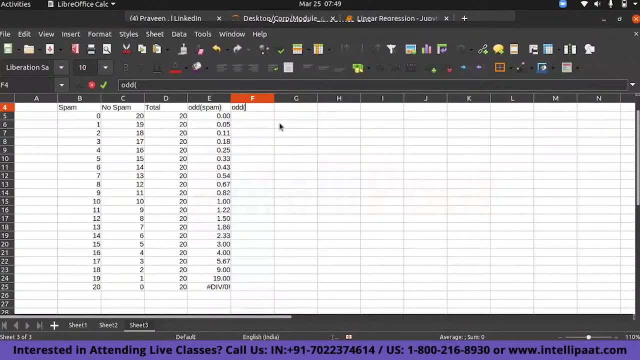 Let's try. If I were to do that, odd of no spam, So which will nothing but 19 this by this Correct. So you're getting a reverse of this. You will not get anything, You will just get a. 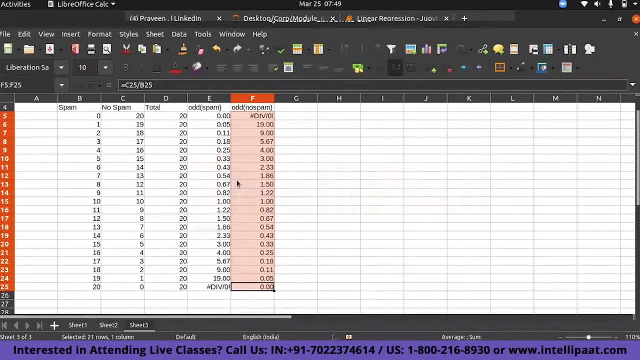 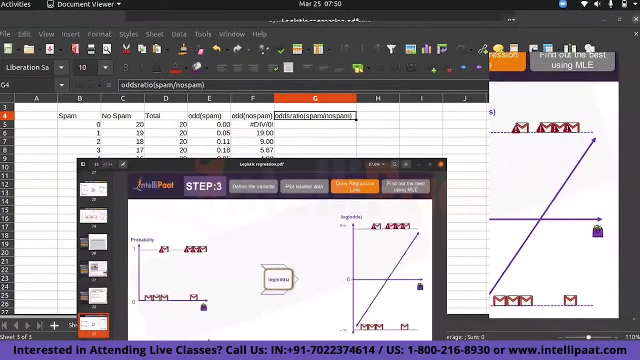 reverse of what you saw here. You'll get this here, this. here It's a reverse. Clear Odds of spam by no spam. Clear to all of you Now, odds ratio of spam by no spam You can see here. Okay. 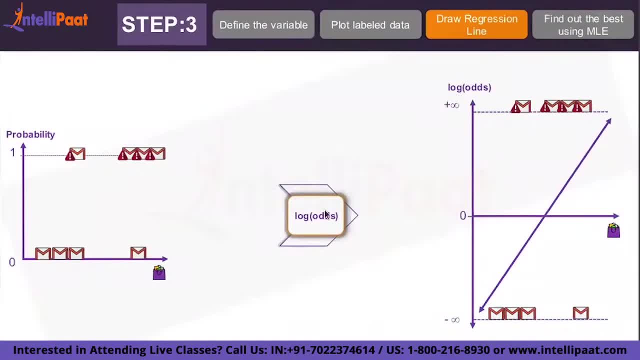 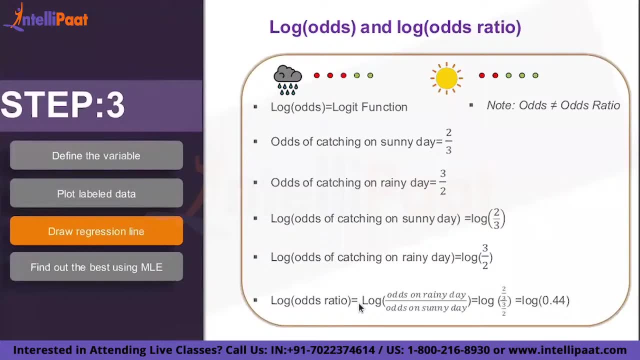 I need to take a log of odds. That is okay, I'll just do that. Now don't worry. Log of odds and log of. I can take a ratio and then take a log. That is also same, only Correct I can take. 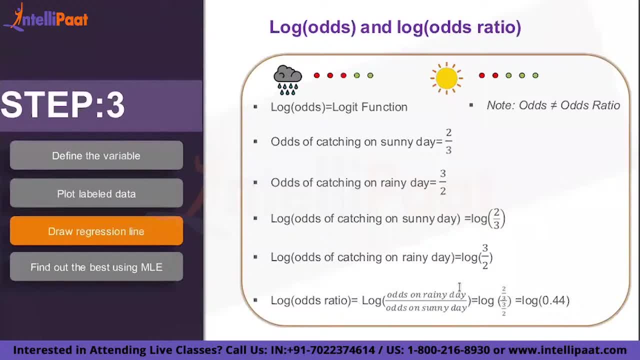 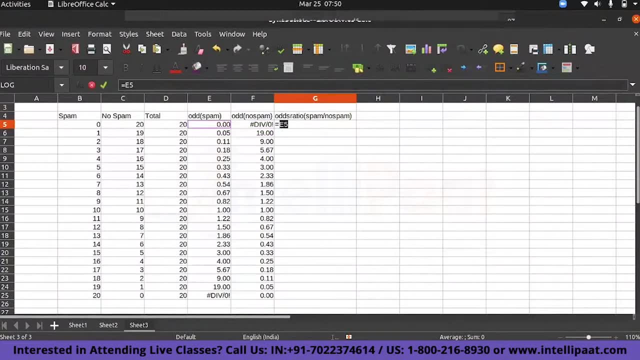 a ratio of both and take a log. Or take log, log and take ratio. I'll take ratio and take a log. So better Odds ratio of spam and no spam is spam by no spam. Correct Agree Spam and no spam. 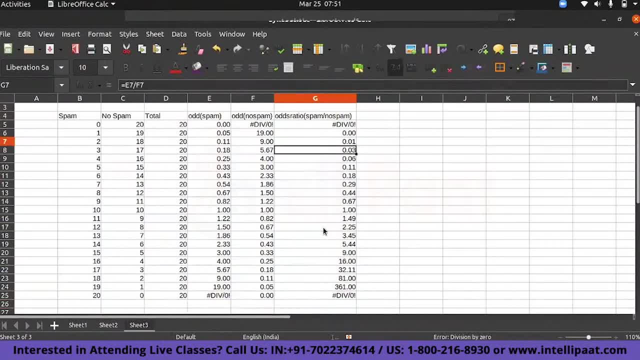 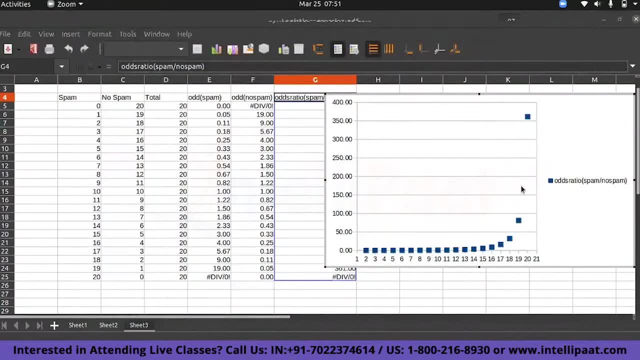 Right Now, if I check this, let me just take a simple example. You can see it is going like a exponential Correct. All of you agree. It is going like an exponential Log. of odds ratio is going to be an exponential curve. I'll remove this. I just wanted to show. 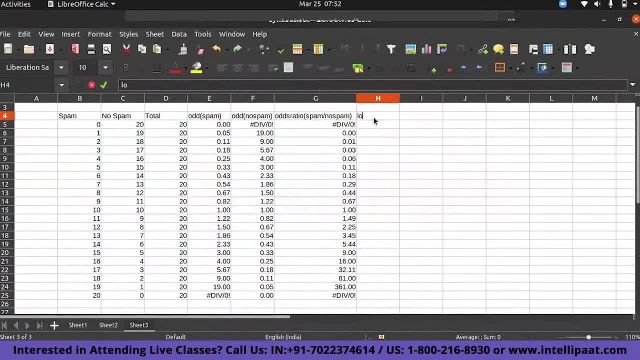 you I just deleted. Fine, Now my log of odds ratio is equal to log of this. I take a log of this and then I make it into two decimals and then I plot a rhine. So whatever was exponential when you take a log of. 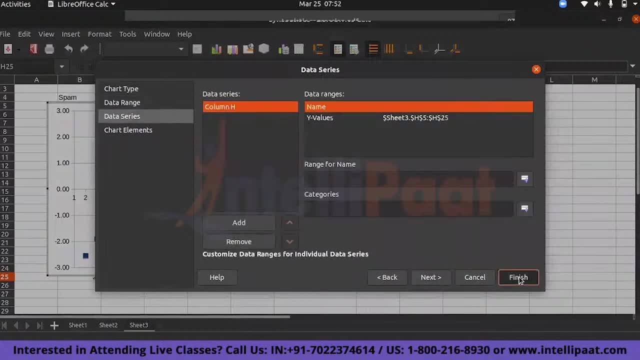 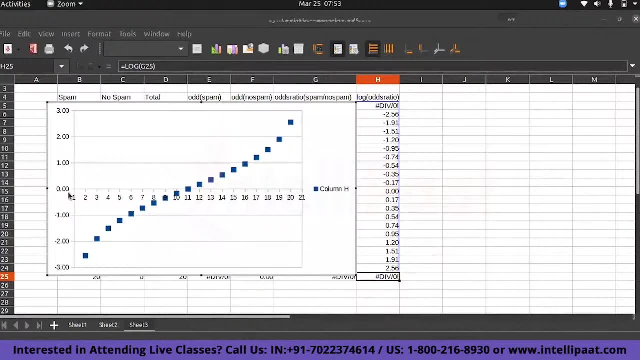 odds ratio. it will become linear. See, interesting. This is precisely what is going to. Now I am enjoying Right Zero. one, two, three, four There are. This is how it works. Okay, I'm not. 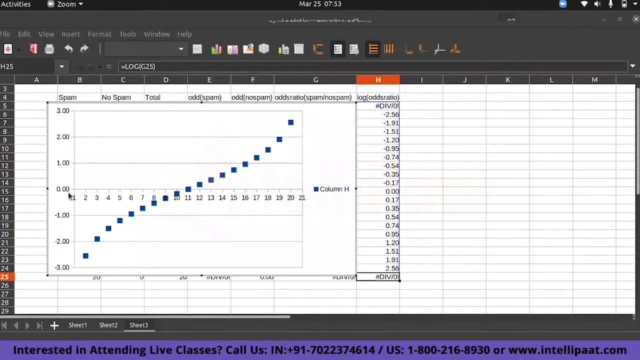 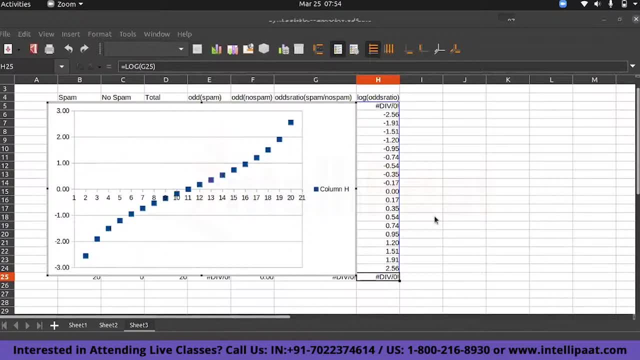 what happens in the logistic regression, the back end. Now my next question is: you saw there were like dotted, dotted, dotted dotted lines which were going up. Can you fit a straight line to these dots using linear regression? If I were to say, if I were to ask you Now, you know, 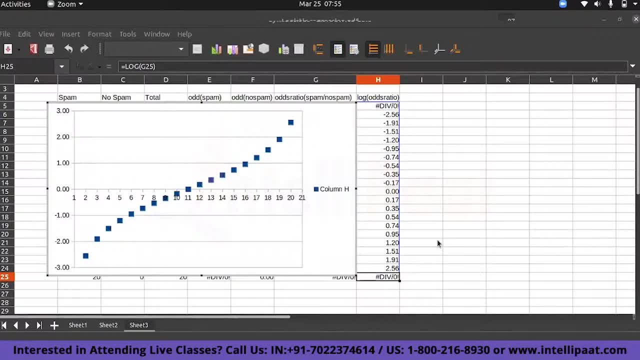 where is regression in logistic regression Understood? this concept Base is always linear Correct. That is why I converted it into a. these are spam mails. These are no spam mails. You don't need to convert. Your machine will convert. So we just need to understand the concept, That's all. 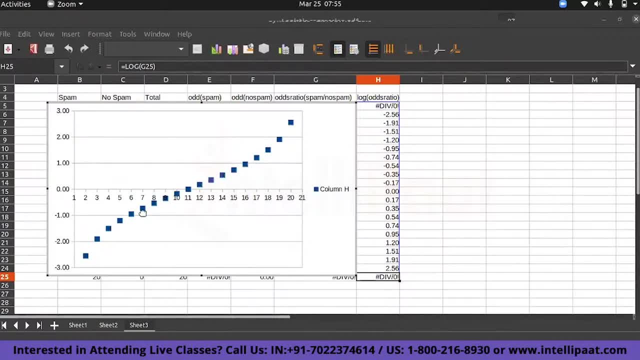 Whatever I'm doing, Python will do internally. You don't have to do, but you need to understand how it works. Right Till here. is it clear to all of you? How did I get this particular thing? Now, my question is: we took 20 emails, We got 20 data points. Okay, Correct. What if I take 1 crore? 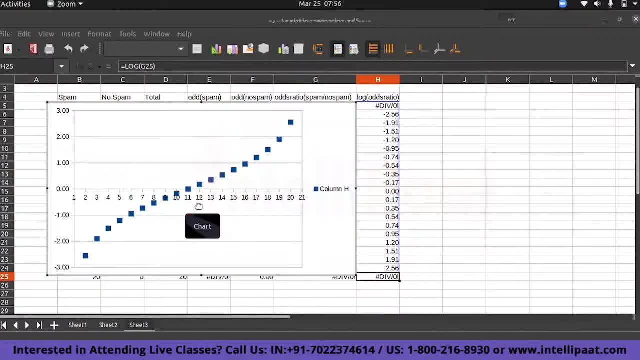 data points. If I take 1 crore data points, you will get some number on the top, some number on the bottom, Very huge numbers you will get Now. is there any limit that I should take that? Okay? No, no, I can run. 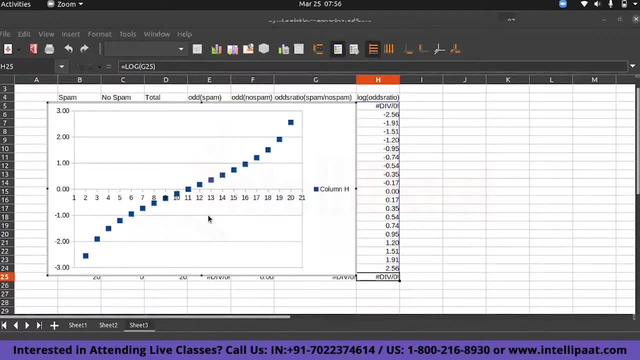 my logistic regression only for 500 data points. All right, So what is the range Infinite You can put infinite. Middle will be zero. Top limit will be plus infinity. Bottom limit will be minus infinity. Correct, Now let me just keep this aside. Okay, I'll just do an undo for this, so that 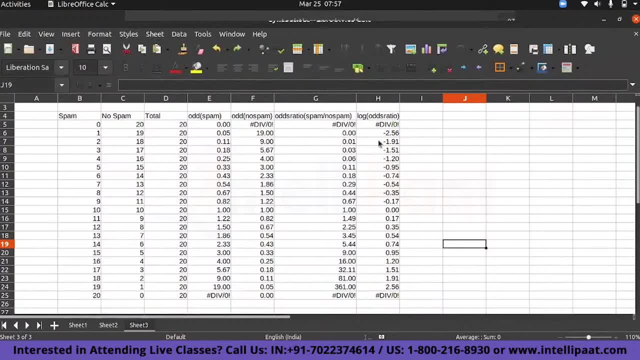 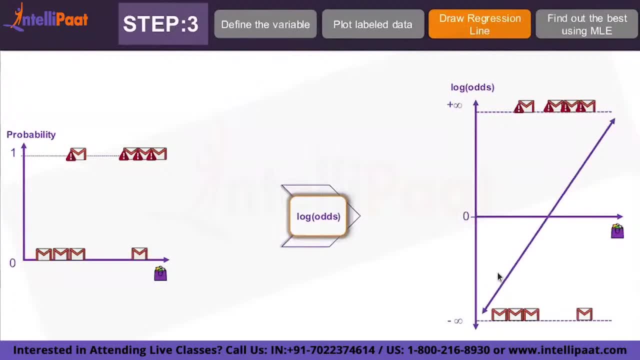 I can run my logistic regression only for 500 data points. All right, So here you get a log of odds ratio. Log of odds ratio. you get Now this is clear to you now. Whatever was this zero in the middle? Your dots will come here, here, here here. If it is below middle point, then it's a. 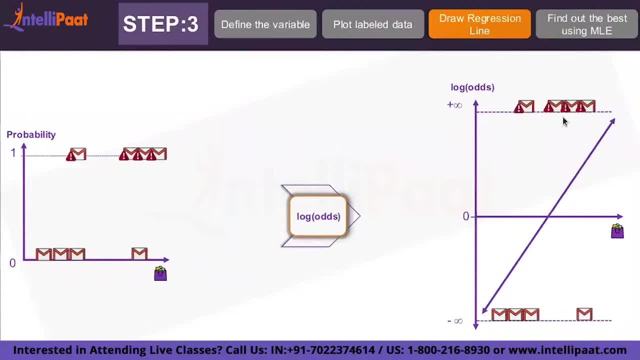 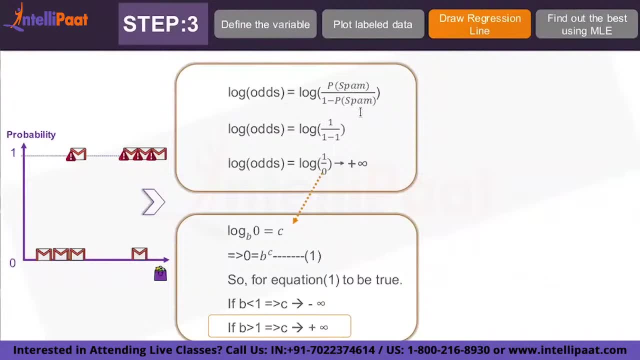 no, it's a spam. I mean, it's a no spam. If it's above, then it's a spam. So something like that Log of odds ratio. we got it Right. So this is nothing but log of odds is log of p spam by 1. 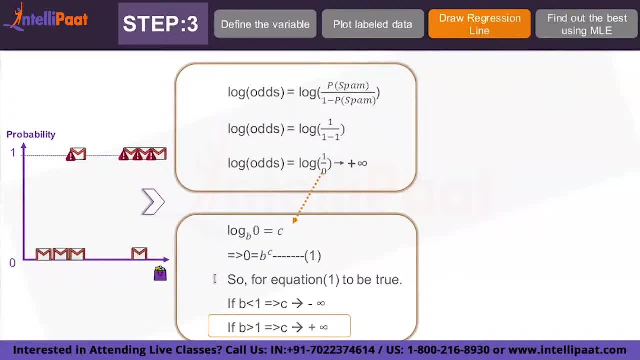 minus p spam Right. So this is basically probability. you will get Something, something, all. you will get it here. Don't worry about all the substitution and all that you will do, and then you'll get something wonderful according to this slide, But I don't know. Let us let it be. 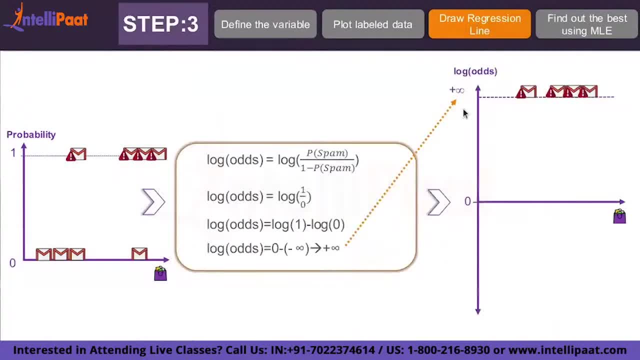 here for the time. We will understand the things better. Now. you get a plus infinity here. That is what I told. So you just take so many data points, you'll get plus infinity. If you take less data points, you'll get minus infinity. This I'm evidently showing you here. only Divide by. 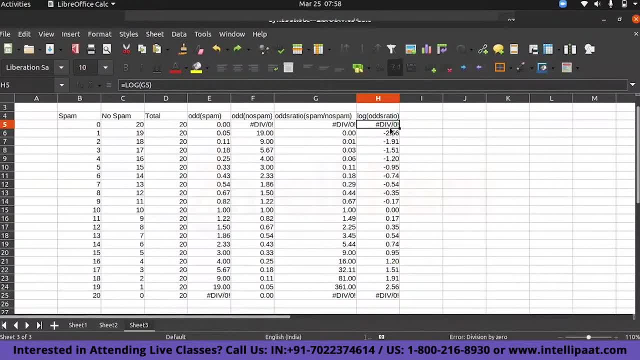 zero. Now, this is, this is infinity, This is also infinity, This is minus infinity, This is plus infinity. You can see, from zero, it is increasing, increasing, increasing, increasing, going to infinity, Increase, decreasing, decreasing, increasing, increasing, going to plus. 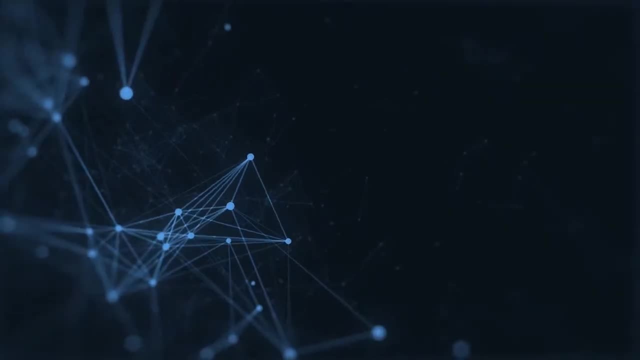 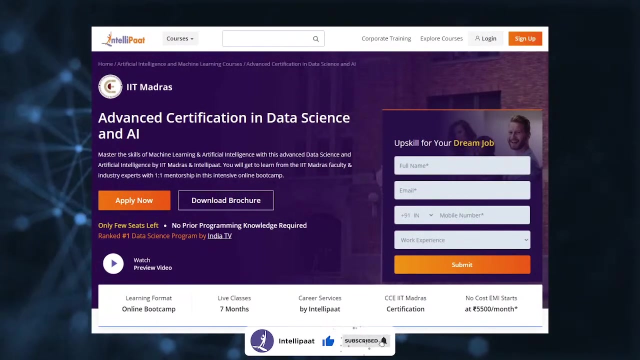 infinity. So that is what they are trying to explain here. If you want to make a career in data science, then Intellipaat has IIT Madras Advanced Data Science and AI Certification Program. This course is of very high quality and cost effective, as it is taught by IIT. 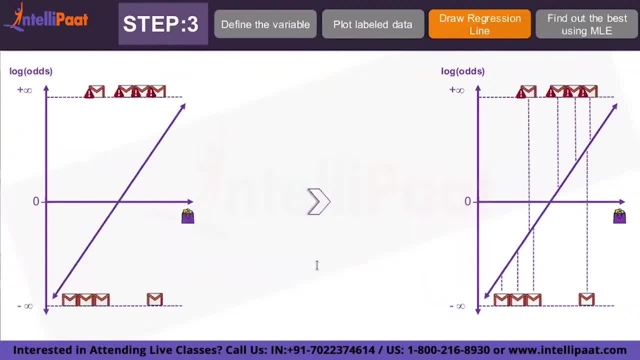 professors and industry experts. Now you're plotting Log of odds ratio. Whatever you plotted- no, your spam, no spam that will come- is nothing but a log of odds ratio. correct. Once you have that log of odds ratio, what we will do is we will spend some. 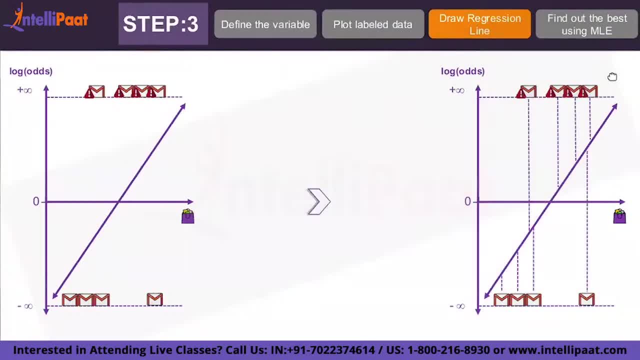 time with the Excel sheet again. Just hold on for a few minutes. You have plus infinity. you have minus infinity. You plotted your log of odds ratio. correct Your mail. whatever your spam mail that you're checking. no, it can be anywhere between zero to infinity. 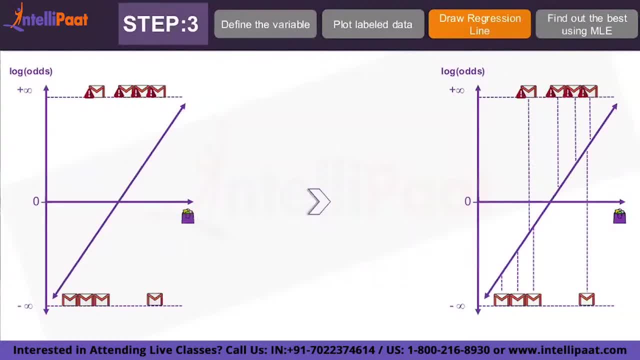 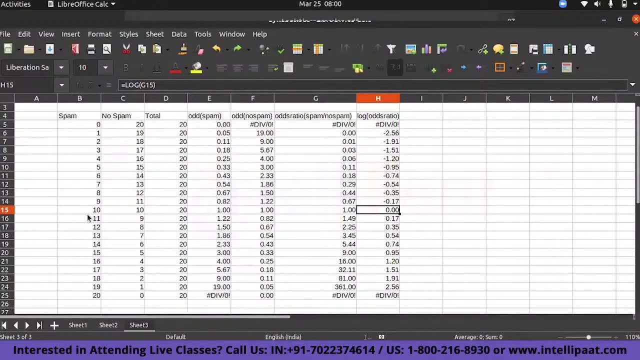 It can be at this point, this point, this point You can see in this one, you can see based on the probability. These are equal means. I told right, These are equal, equal kind of scenario, Same same words, So confusion. state So zero, and classify Here it can be anywhere between zero to plus. 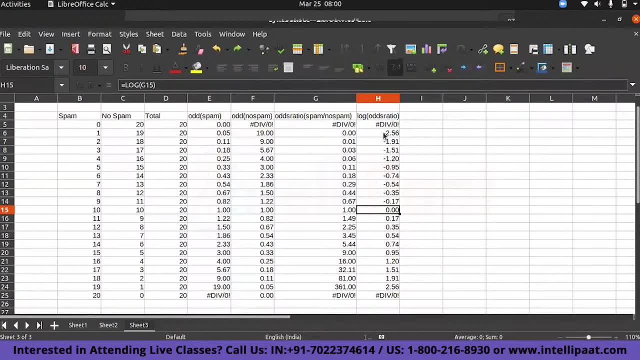 minus infinity, zero to plus infinity. The range I'm talking about, You can see: zero to plus infinity, zero to minus infinity. It's the range. Now, what will I do? I'm going to pop that in here. I'm going to pop that in here And I'm going to. 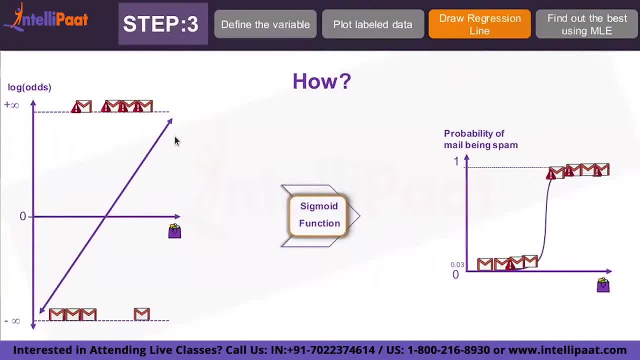 I'm going to pop that in here And I'm going to pop that in here And I'm going to pop that in here And I'm going to. we will do is, if you want to give you converted it into a linear function. okay, you converted into. 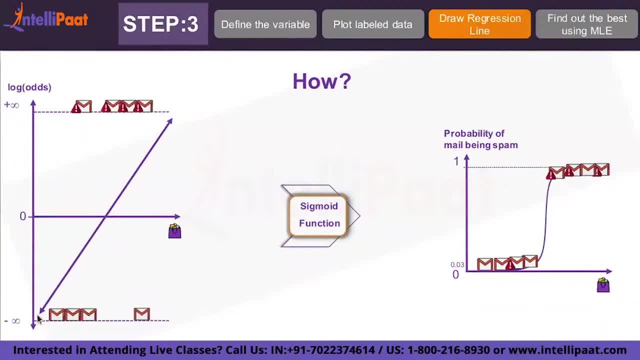 a linear function, log of odds. now you have to fit something. it can be a straight line, curved line, whatever it is. you converted your data into a linear kind of a data, which means you can do a regression on that. linear regression means you will fit a linear straight line. now you want to. 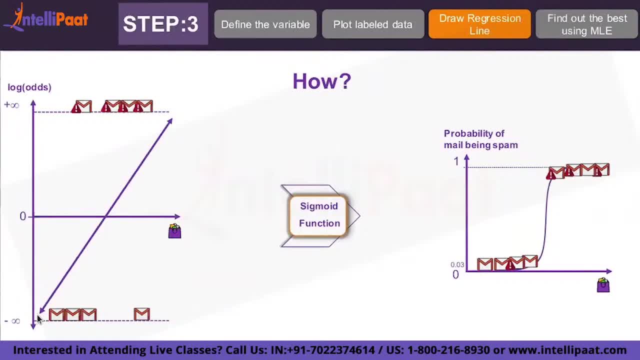 fit one line which can help you right. so that function which can fit this is a sigmoid function. it's not a straight line function, it's a sigmoid function, correct? so now you are changing the axis from infinity to one, from minus infinity to zero. axis would change, right. so we'll see. we'll see. 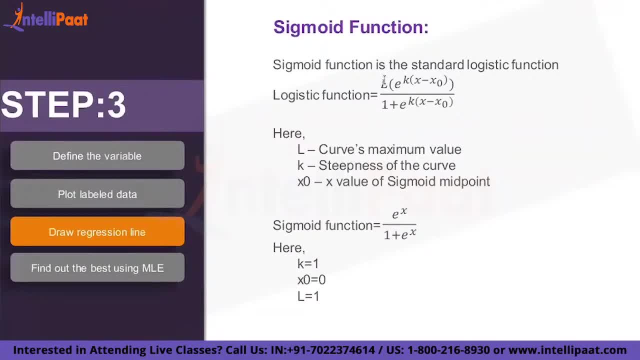 how it works. what does sigmoid function means? so sigmoid function is a standard logistic function. logistic function: e power, something. e power, something. what i'm trying to tell you here is to convert something into a log. you will take what you will take- a log. to convert a log back, what you will do. you will take e power, exponential anti-log- you can take. 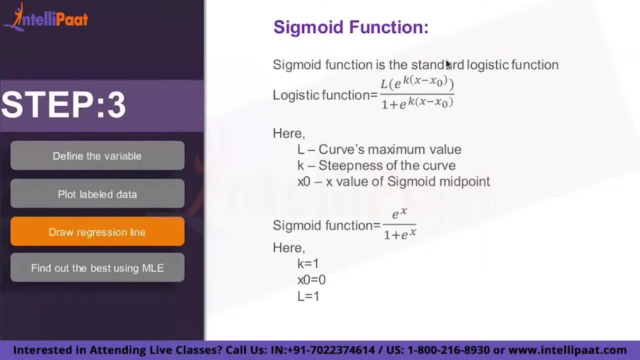 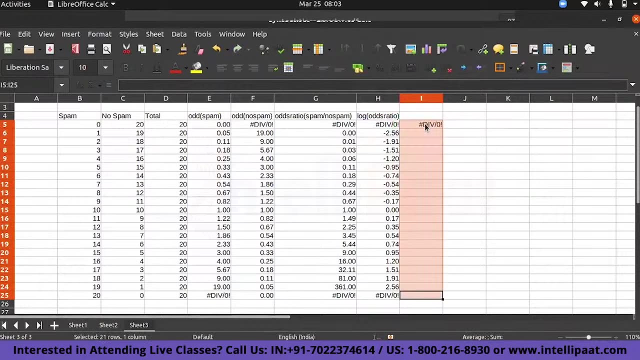 e to the power, right. so exponential e power, you will take correct natural log log to the base 2. so there are two types. anti-log is e power. so i'll just put here: i don't know if e power works on this. let me see if this works. if not, we will check and then we will see later. no issues, so if this works, 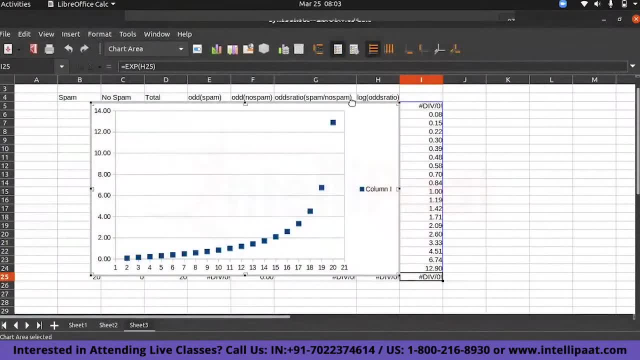 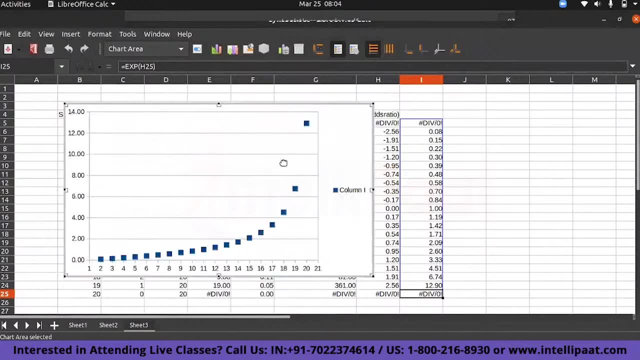 fine, if not, then i will see how it works. you can see same thing. no, i reduce the decimal point, so that's why we are getting little different. it's. it's an exponential. yeah, it's an anti-log. whatever the data previously was in exponential, we converted it into linear and now we are converting it back. 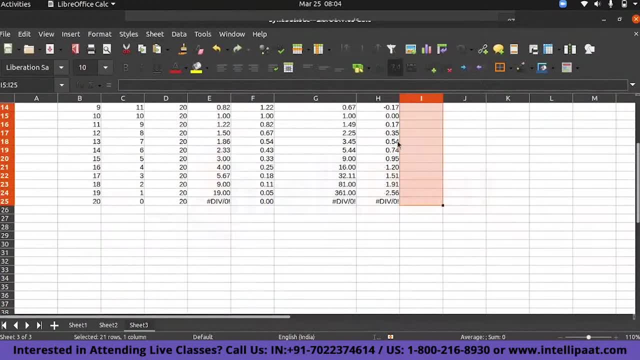 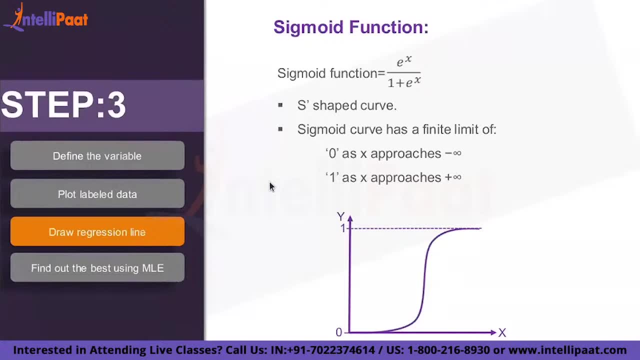 into exponential. so this i don't need. i just wanted to show you e power will convert it back into a linear clear till here. all of you any questions? nice, now, this slide is a little important. so the equation of sigmoid function is e power x by 1 plus e power x. sigmoid function is e power x by 1 plus e power x. so this is my sigmoid function. 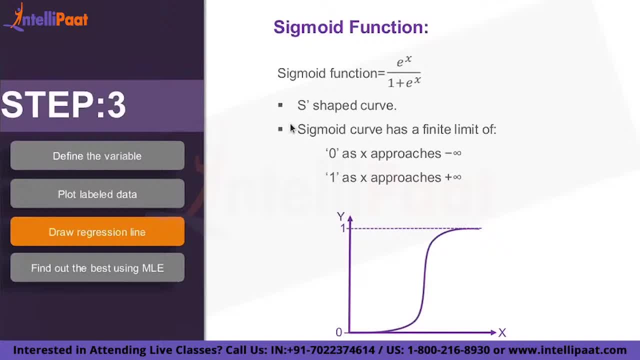 or the s-shaped curve that we talk about. whatever we were seeing has an infinite limit, which means your range can go from zero to infinity, but the functionality of sigmoid is it will become zero if your value approaches minus infinity. it becomes one if the value approaches plus infinity, irrespective of how big or how. 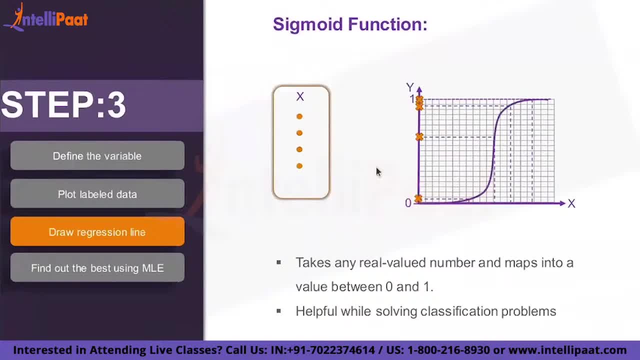 small it is. this is how it will work now. you can see here any number- you take real values- it can be mapped between zero and one using sigma information. any number between zero to infinity can be mapped. anything between zero to minus infinity can be mapped between zero to infinity. 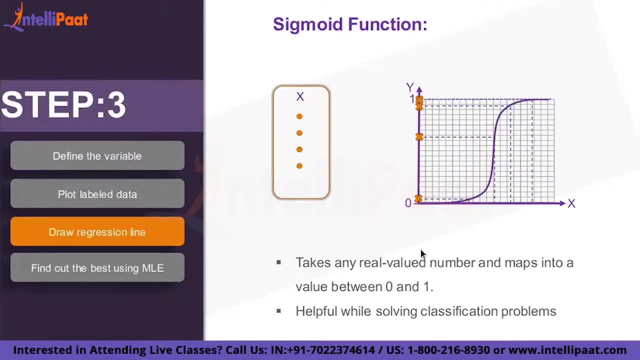 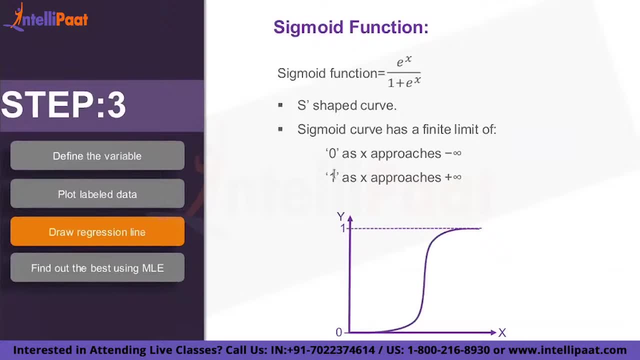 can be mapped, which means you're taking your complete range from minus infinity to plus infinity and then you're mapping it into zero and one. this function is your logistic regression function. agree, now clear conceptually, you're getting it following nice. so now what we'll do is like we'll 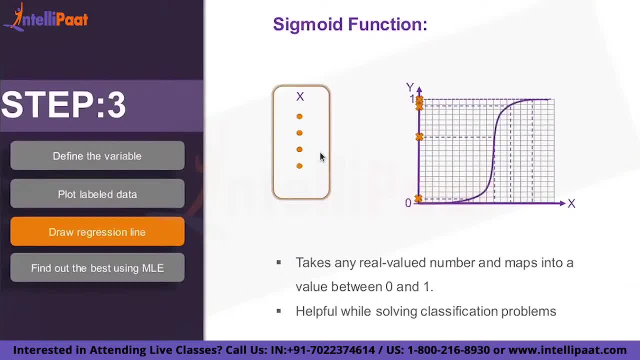 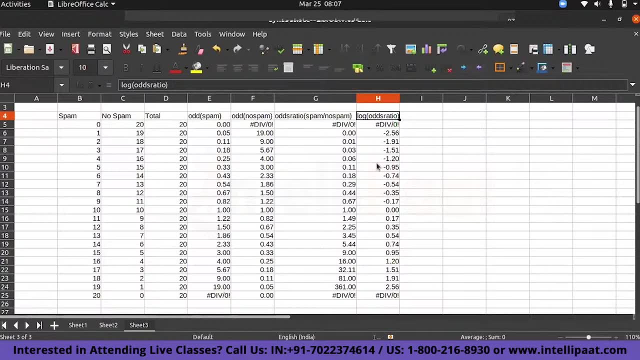 go ahead. yeah, so what i was saying is: whatever distribution that you created here, its range is between minus infinity to plus infinity. if you want to do fit a line, fit a curve, do whatever. you'll not be able to do it within minus infinity to plus infinity. now, if you want to get it inside, 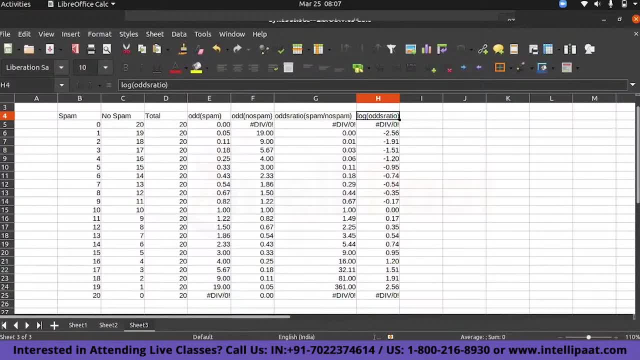 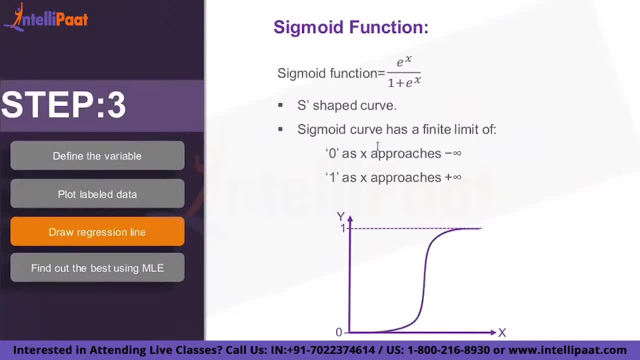 a range where you can fit a curve. that range is zero to one. there is a math function called sigmoid function. its range comes. if it is minus infinity, then sigmoid function approaches zero. plus infinity, then sigmoid function approaches one and everything in between can be fitted. so that is why we select sigmoid function to do our logistic regression clear. fine, all of you? it won't. 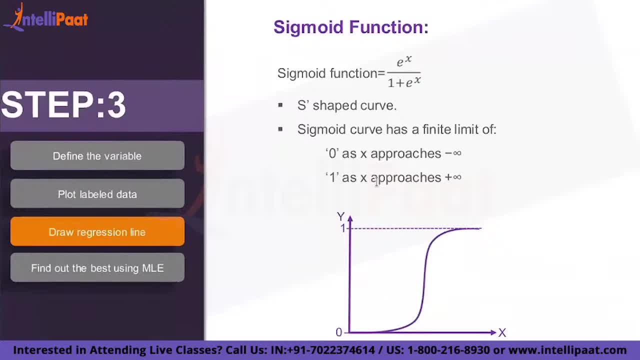 go in negative or also in positive. it will not go to minus infinity. no, it will not go into negative. it will not go into minus one. correct, it is only zero or one, because we should identify zero and one only, no binomial. that is why use this sigmoid function. so now how we are going to use it. okay, 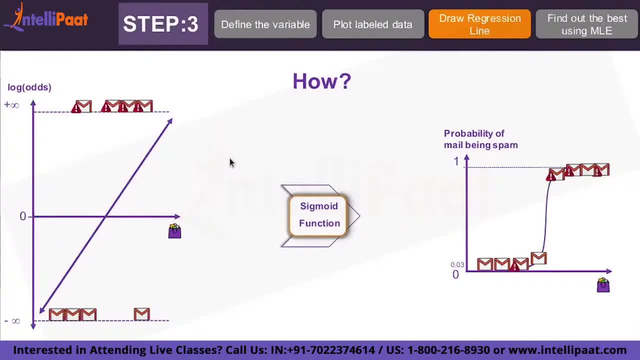 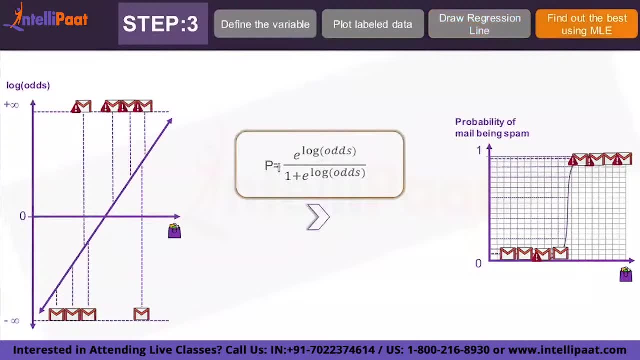 right. so let us go ahead and see next what is going to happen. so we saw minus infinity, plus infinity, and then you are getting a sigma. how is probability is nothing but e power log of odds ratio by one plus e power log of odds ratio. just see this probability of something happening. 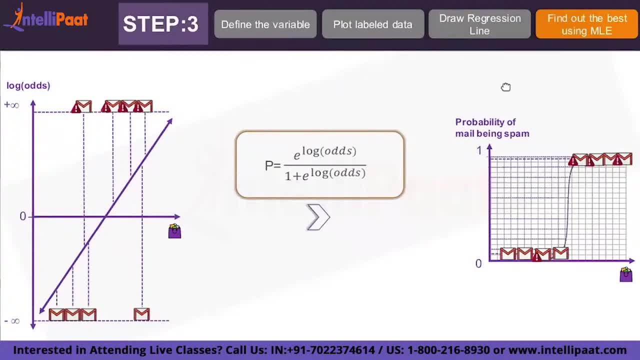 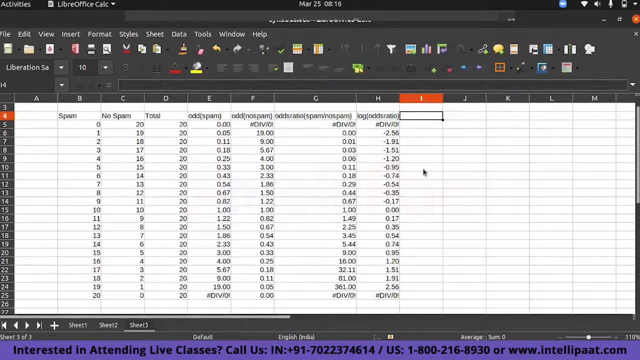 to something not happening. e power: one plus e power log of odds ratio by one plus e power log of odds ratio. Now, what I will do is I will take this and I will take the probability of e power log of odds. will do is i will do something called as probability. probability is nothing but e power. 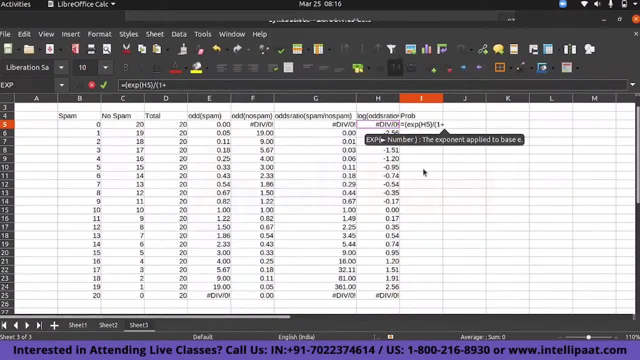 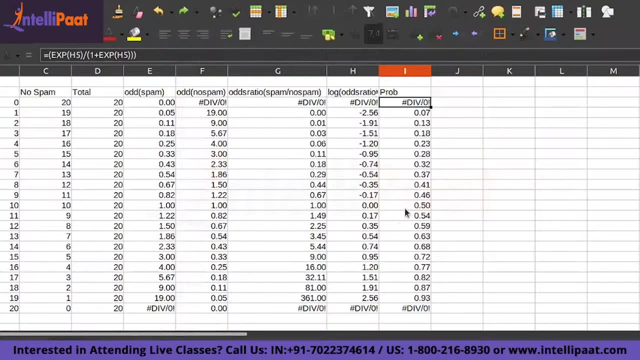 this divided by one plus e power. this. is there any mistake that i did? it's not one plus no, it's one plus only. correct e power log of odds ratio by one plus e power log of odds ratio. that's what i did not here. it's natural law anyway, this is supposed to be. do i say zero and this is supposed. 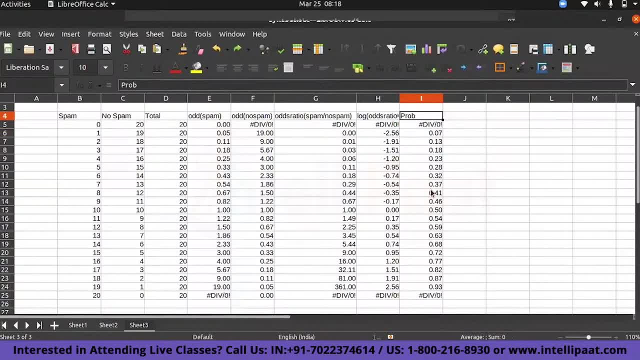 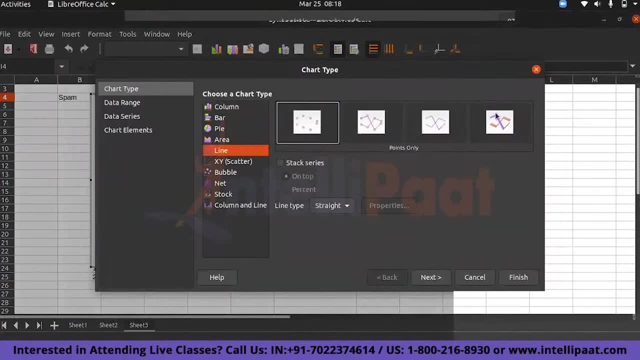 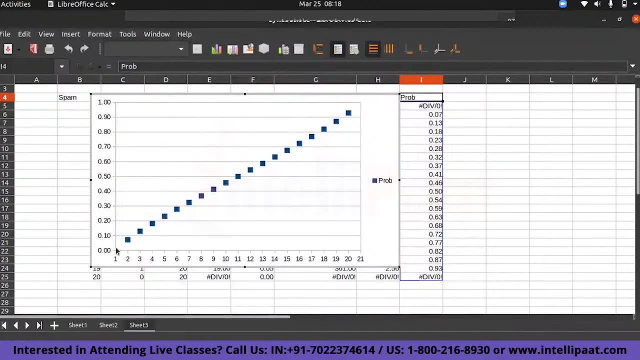 to be one, but anyway, let us plot this and see you will get a sigmoid curve or not. it's like base one, base two, such stuff, but anyway, let us plot this and then see whether we'll get a sigmoid curve or not. next, next finish, you can see you're getting curve which is straight like this: 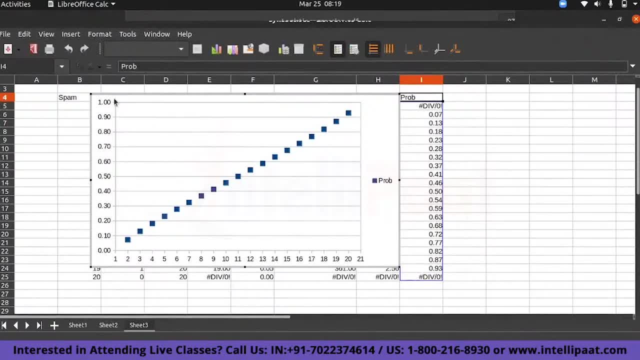 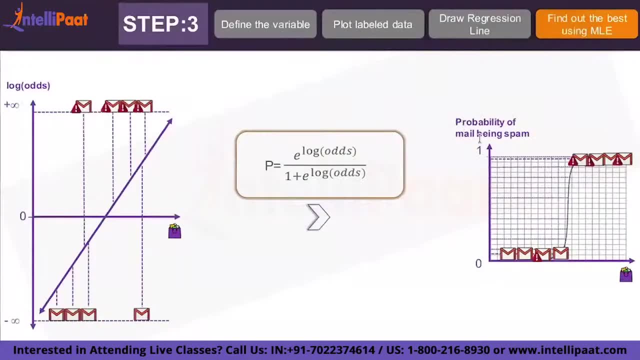 probably from zero. i'm bringing it between one, correct? you can see now probability. i got it from zero to one right now. that is what is here. also, probability is between zero to one, correct. agree with me. now, if you can see this, i'll just put it like this: this one we tried. now what i'm trying to do is i'm 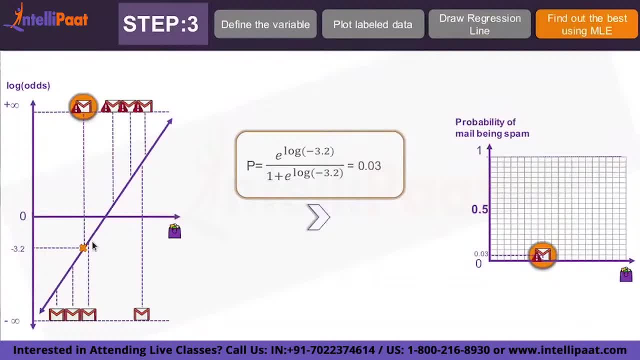 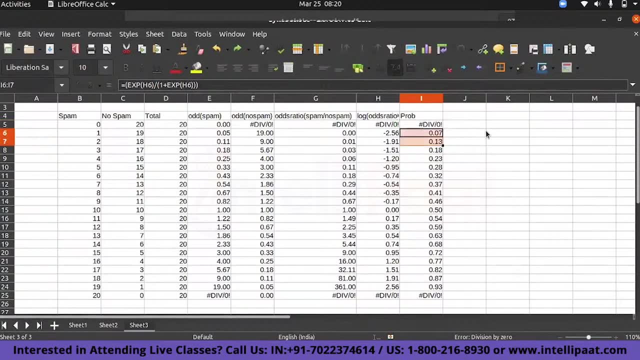 just checking negative and positive, all negative numbers, whatever you have, are spams, positive or no spams? same thing, i think, with us also. you can see you, negatives are less than 0.5, positives are more than 0.5. now, what we are trying to do, 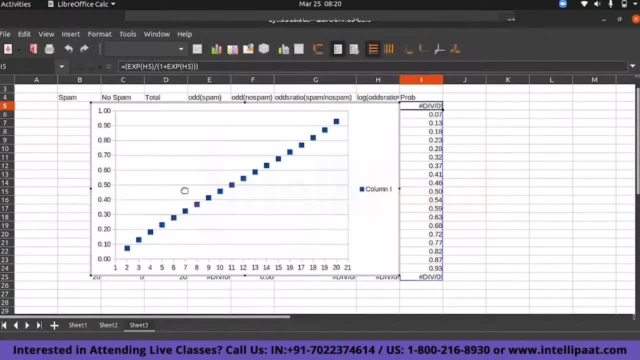 you. i'll just put it again and then i will show it to you. all the points which are below this become zero. why the probability of them being a spam or no spam is less, which means probability of them being a spam is less, so i can mark this also as zero. this also zero. this also zero, all. 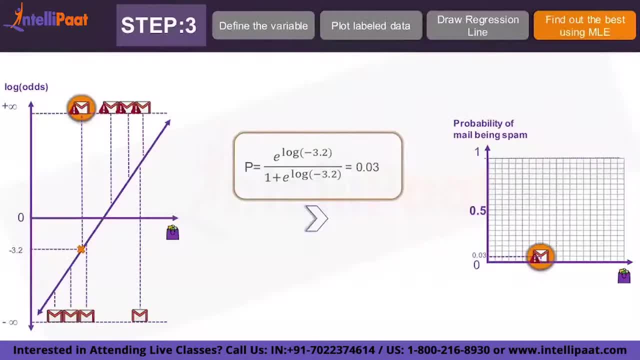 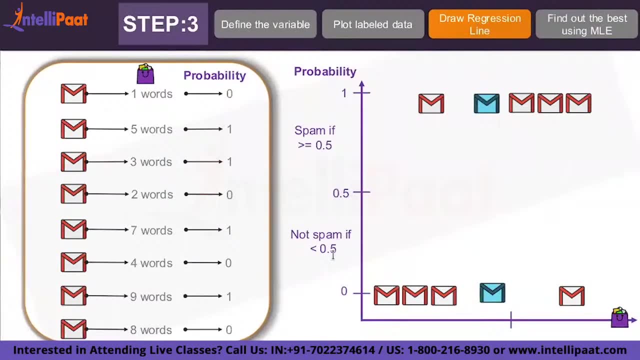 of them, i can mark it as zero till 0.5. agree what we saw here on the top. i'll show you where we saw that here: probability: if it is less than 0.5, then you mark them as zeros. if it is more than 0.5. 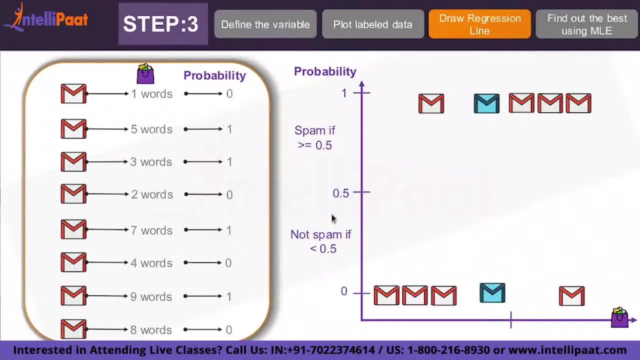 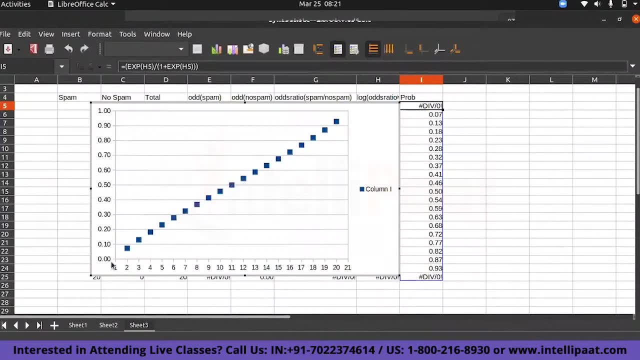 mark them as ones. now, whatever image you are seeing here, the same graph i plotted here: 0.50, 0.51. whatever is less than 0.5, mark them as zero, which is not spam. whatever is more than 0.5, mark them as zero, which is not spam. whatever is less than 0.5, mark them as zero, which is not spam. 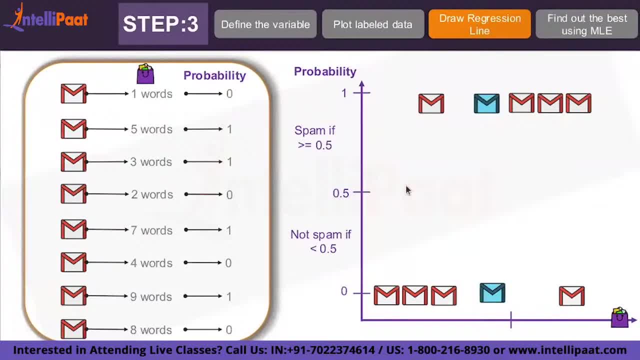 as one which is spam. correct this one: agree till here, agreeing all of you concept. you are getting no. this video you have to see multiple times. only you will understand or else it will be difficult. okay, so now, once you do that, so till here, you got it. this also is done. so this is spam. this is no. 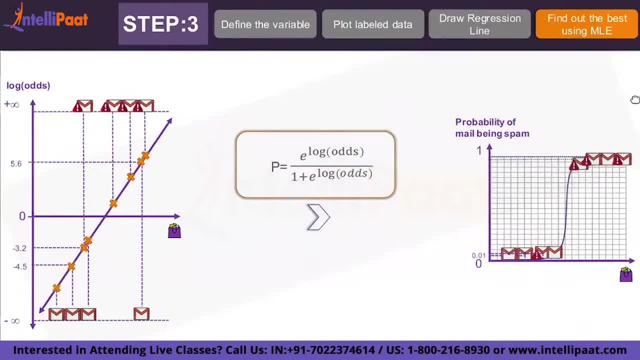 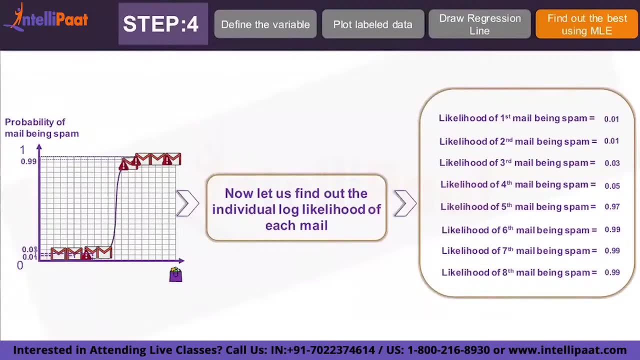 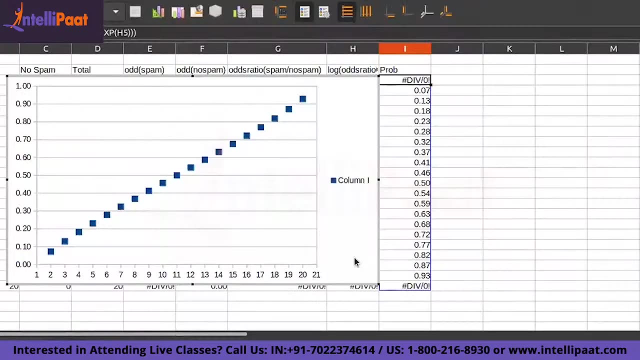 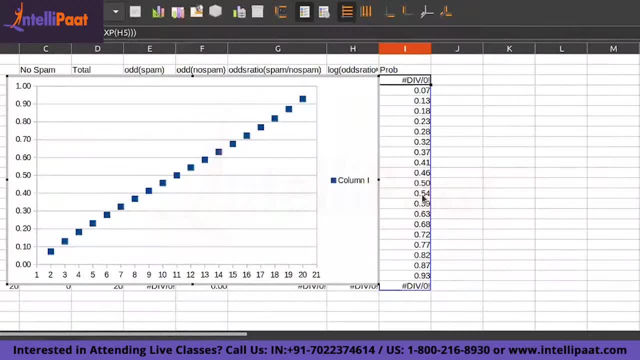 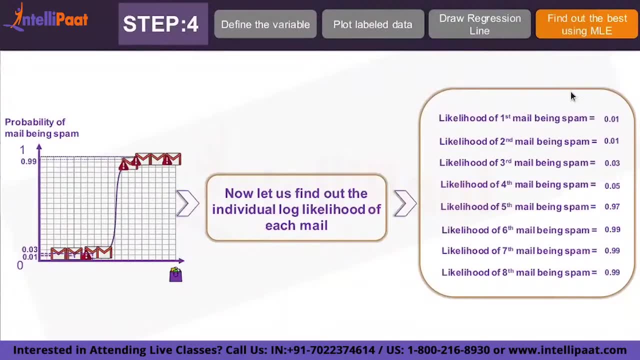 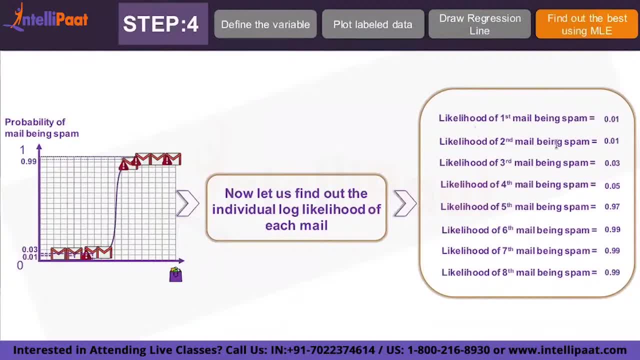 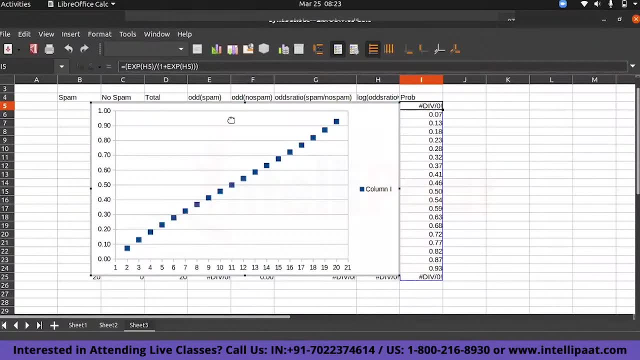 spam is called likelihood. this is likely, how likely it is a spam. so i told you this is a probability, right? so there is a chance of fifty percent that this being a spam or no spam. there is a chance of thirty percent this being no spam. i mean seventy percent that this being no spam. and 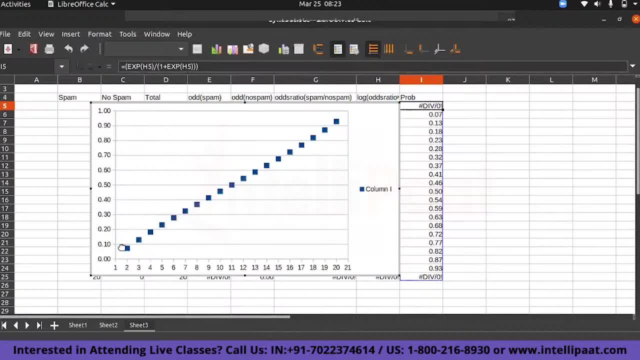 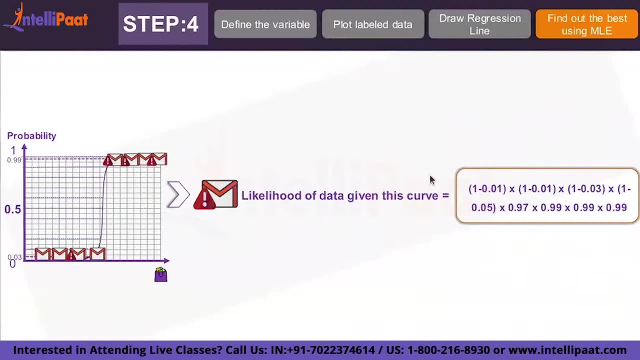 thirty percent between the spam, so like that. so all these things are not spam. all these things are spam. there is an associated probability which is called as likelihood. now, what we are trying to understand is: you get all these data points here. now you can see. you are supposed to do it like this: likelihood of a given data. what is the likelihood of given data? 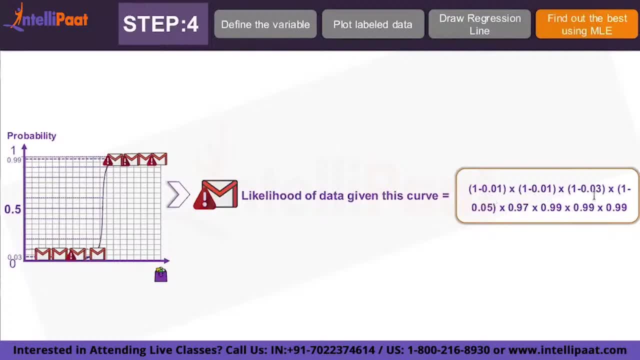 one minus zero point zero. one one minus zero point zero. one one minus zero point zero. one one minus zero point zero. five zero point nine, nine, nine, nine, all these things. this is nothing. but if it is less than 0.5, you are doing one minus, because it is no spam this formula. see this formula, not this. 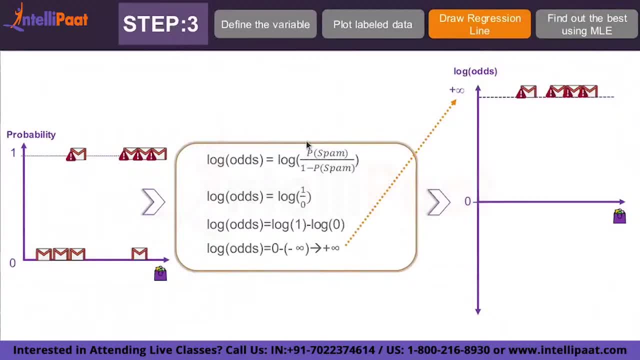 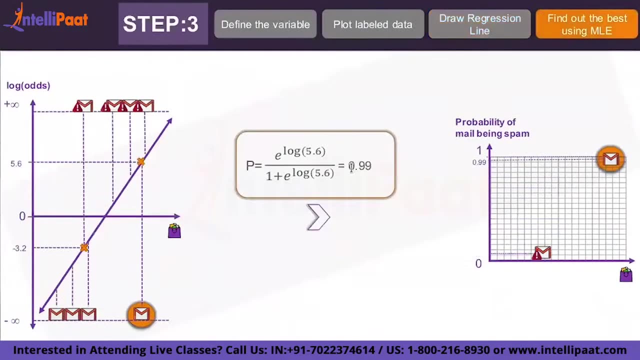 is a log, likelihood, log of likelihood, log of odds. this is likelihood function. log of odds is nothing but your log of likely logic. you can see same thing now what you are trying to do: p of spam by one minus p spam. this is the ratio. but now what you are trying to do, the complete likelihood. you 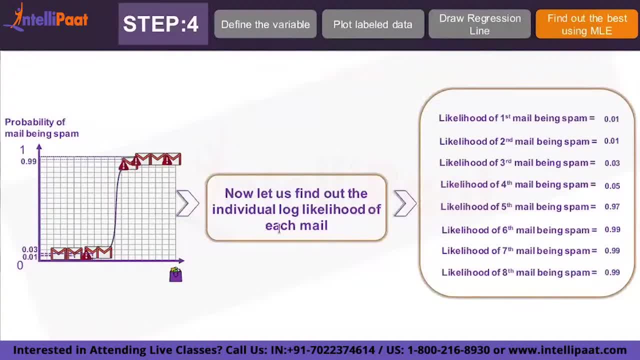 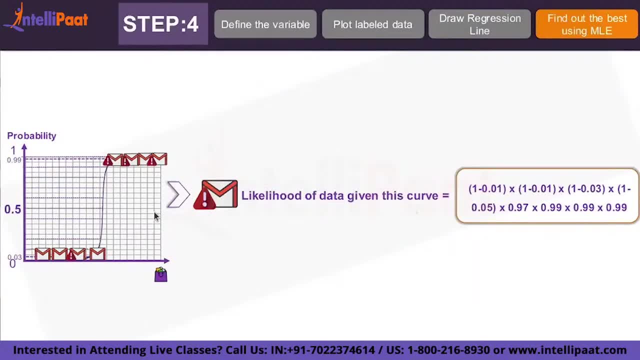 are trying to identify individual log likelihood of each email. is this now likelihood of the complete data, given this curve? so if this is the curve, what we will get one minus 0.5 till here into this one. so you just supposed to multiply all of them if you do this and then take a log of it. right, take a log of this likelihood then. 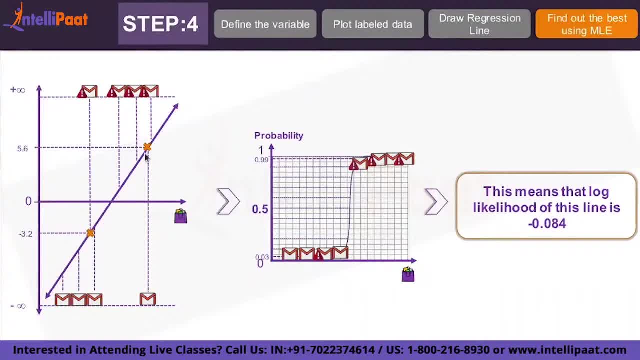 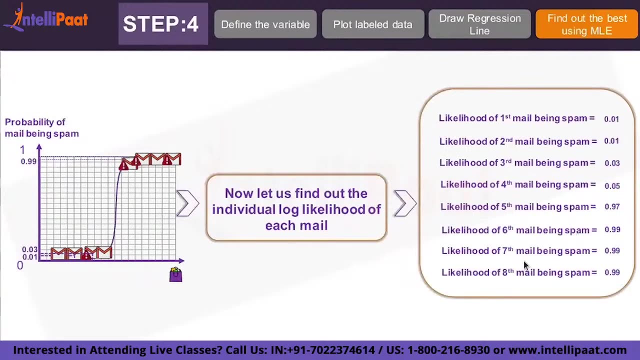 you will get the log likelihood of this particular line that you are fitting is 0.85 or minus 0.85. so log likelihood of that, this concept- i'm not doing it in excel because it will. it will take time but just understand till here. is it clear to all of you? how do i find the likelihood clear? 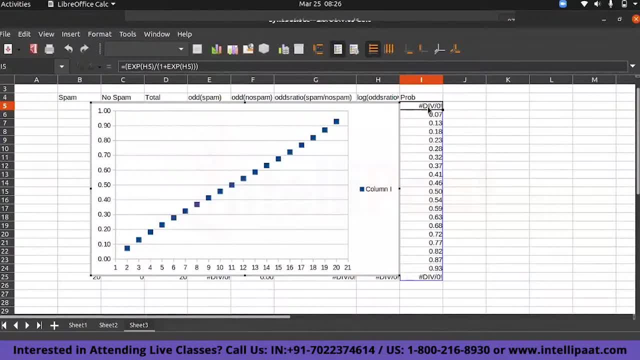 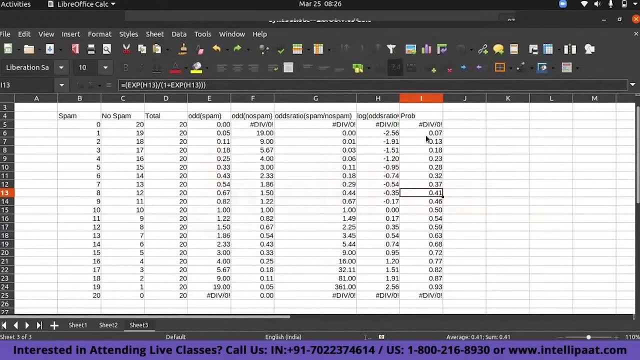 likelihood is nothing but the probability that we calculated here. so this is the likelihood. what is the likelihood of some male being a spam or no spam? that's a probability is likely. if you see this. let's say this in here: there is 0.07 percent one male. some male is a spam here in this set 93. 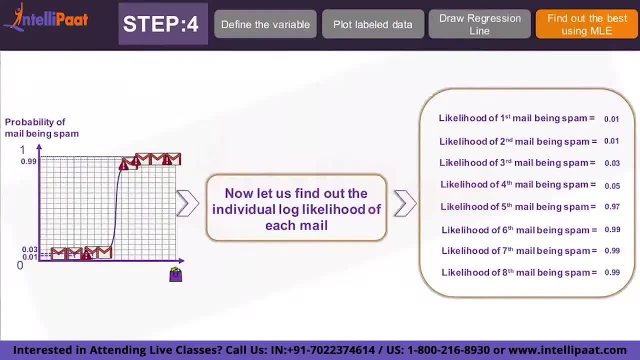 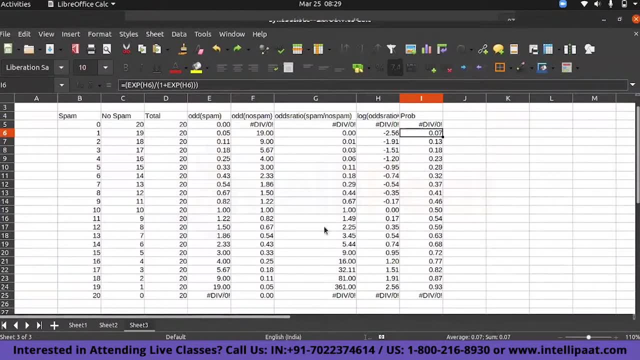 probability spam. that is the one right. so likelihood is nothing but the probability. so what we calculated here, so you can see likelihood or probability, is e power 1 plus e power logs order ratio. so e power logs of order ratio by 1 plus e power logs of order ratio. 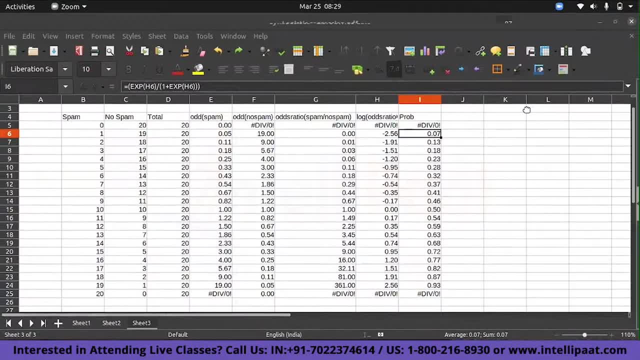 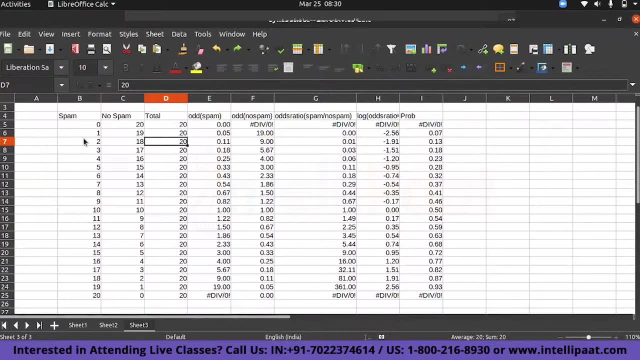 yes, are you understanding till here? basic calculation. i'm not doing any complex stuff. let me be very clear. i took my set of 20 mains. i took set of 20 mails. i took all possibilities of being spam and no spam. i found out the odd of spam. you know how to found out odd of spam. i found out odd of no spam odds. 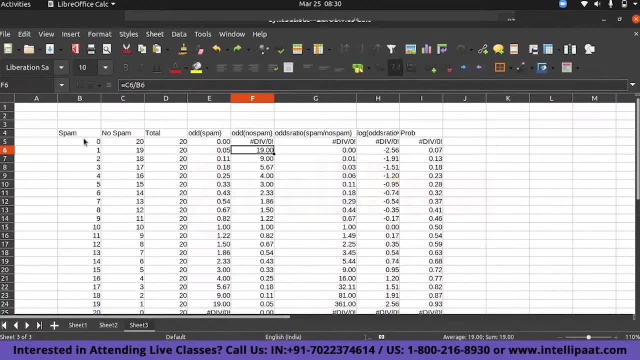 of log. you did i mean odd of spam, odd of no spam, odd of ratio, spam by no spam. then you took log of odds ratio. then you took probability. so how do i find probability? i have to take e power x by 1 plus. now i'll tell you one very simple concept. till here is it fine flow, if you see the video once. 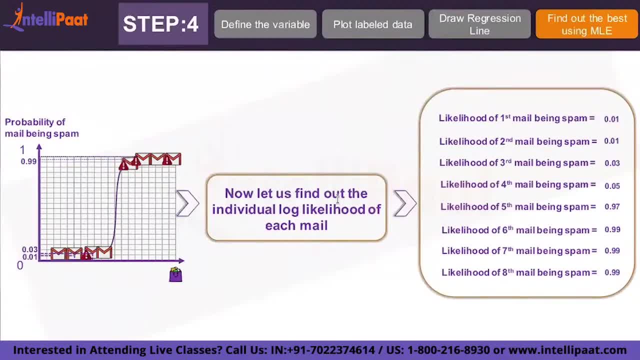 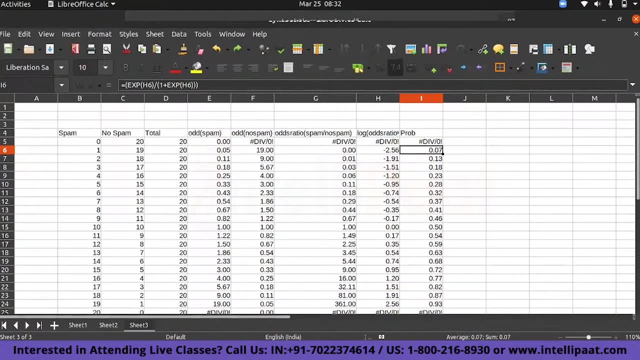 again, you will understand how the calculations are done. also, that's it. it is binary as of now, 0 and 1.. i'll tell you what does that signify? i'll tell you. whatever you are seeing here, this probability, is this column, probability i column in excel, true? so now what i'm going to do is: 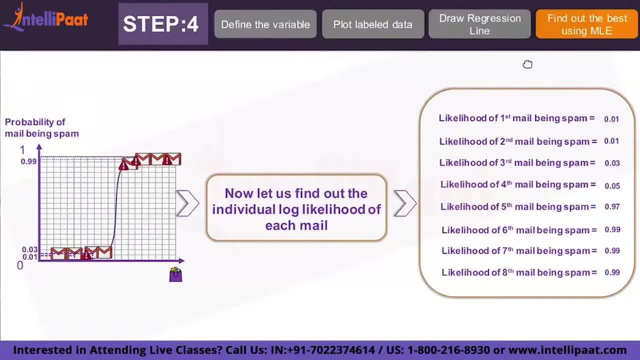 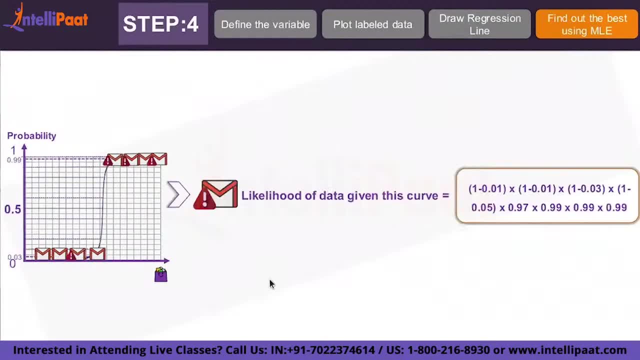 i'm going to tell you we are just doing a simple calculation. okay, for all these ones, you have 0.1, 0.1, 0.99, all these things. now we are going to take likelihood of data, likelihood of data, p, whatever is less than 0.5, you are subtracting it and then, whatever is, 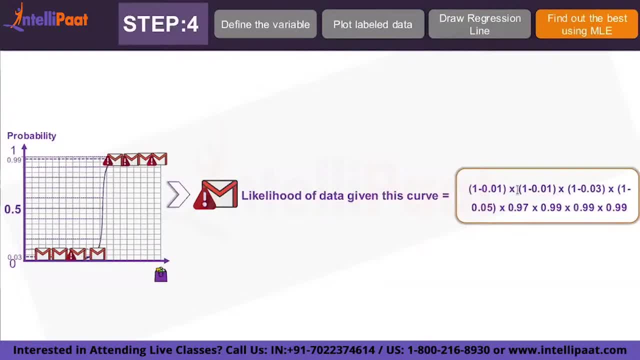 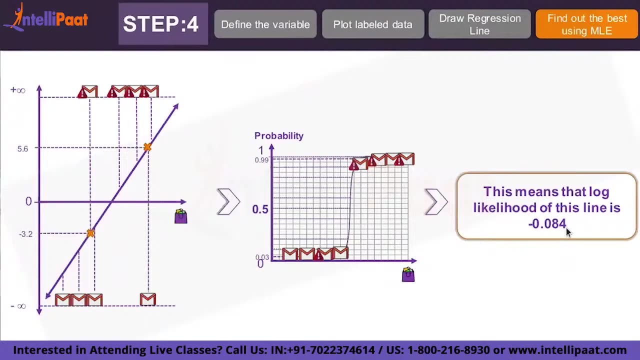 greater than 0.5. you are just having it like that: 1 minus and 1 plus. so something like this you are trying to do: once you do this particular calculation like this clearly, and then take a sum log likelihood, you will get a value which is 0.08. so this calculation will try to do it. this is the 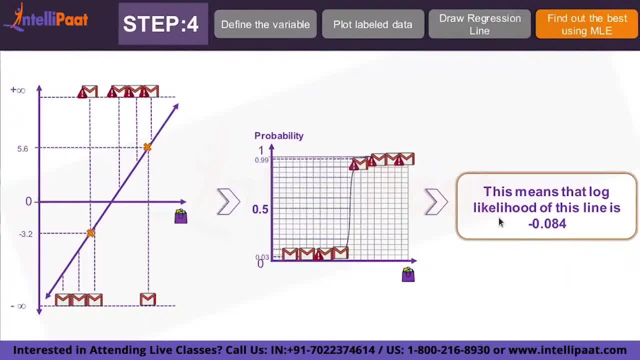 likelihood line that you will get. like this: the log likelihood of this particular line is this: there we were in linear regression. we were having a line where we were trying to minimize the error correct. agree with me, all of you, we were trying to minimize the error here. here also, we'll try to do. 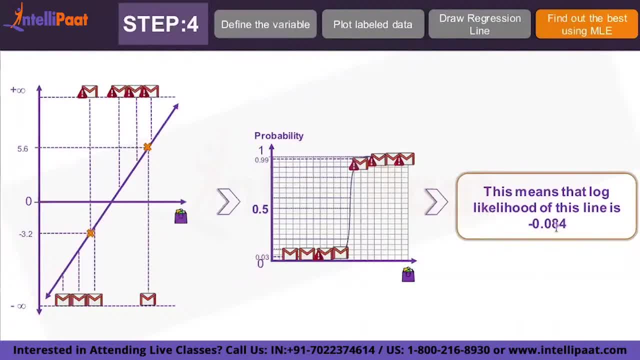 something. so this is one line for which the log likelihood is 0 point minus 0.084, correct? so in linear regression we were trying to minimize the error- actual versus predicted- and then find the best fit. here there is a likelihood, which means the log likelihood of this line is 0.084. so this is something that is coming. this is the line. 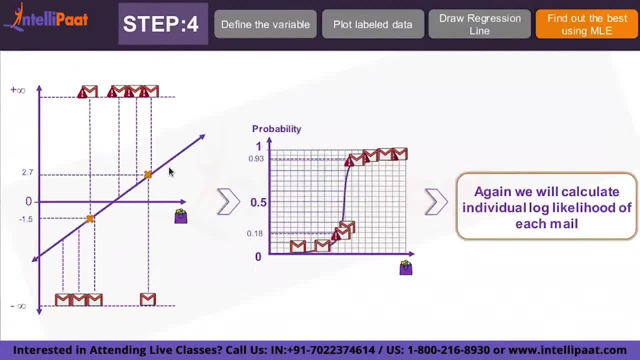 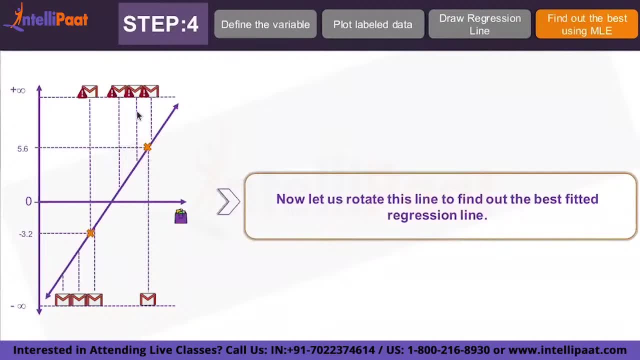 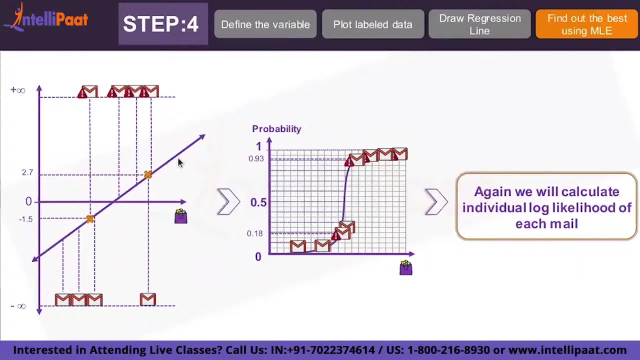 that you are trying to fit. now, if you take another line like this first line was like this: you are going to fit the first line. you can draw infinite lines. now, here also, it is not fixed to a single line. you can draw infinite lines and check if you change your line like this, and then again find out. 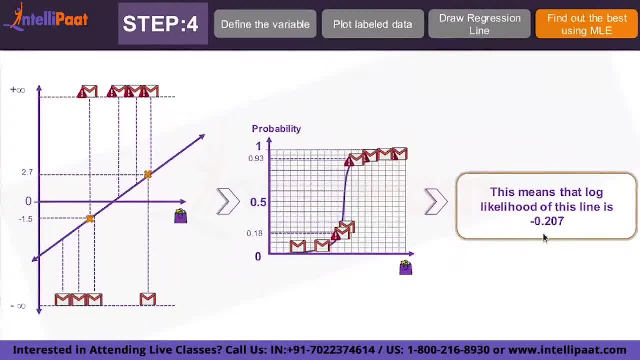 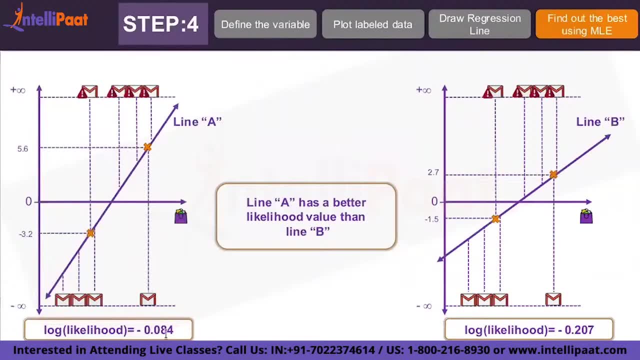 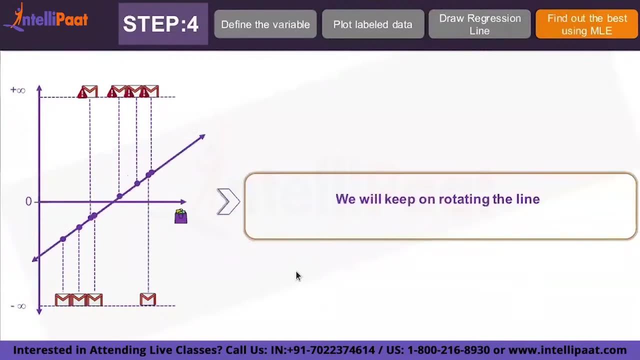 log of odds ratio, you will get some value minus 0.27 if you change this again. let us say one more line here: line a is 0.085, line b is 0.024. similarly, you can have multiple lines like this. you can just keep on taking multiple lines, fitting multiple lines and then finding the likelihood. 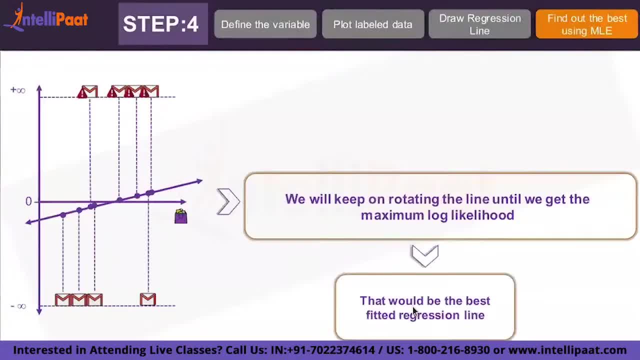 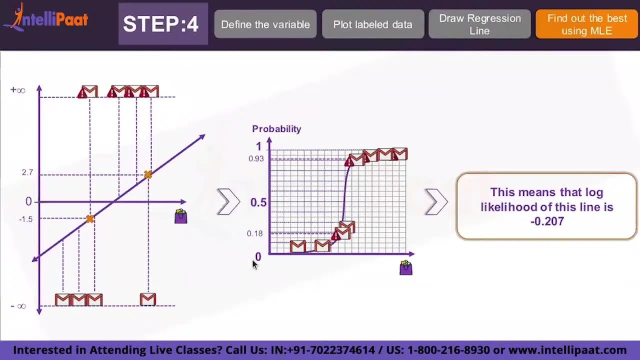 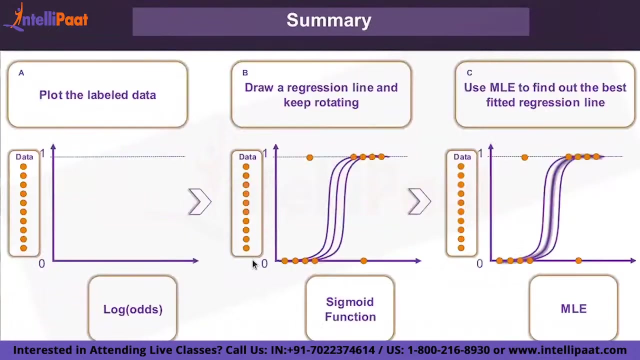 where you get the maximum likelihood. this is called as m l e, maximum likelihood estimate. whichever line will give you a maximum likelihood estimate, the sigmoid curve corresponding to that line is your best fit curve for logistic regression. is it correct, correct, correct, correct, correct, clear to all of you. conceptually you got it will. logistic regression will not give mle logistic. 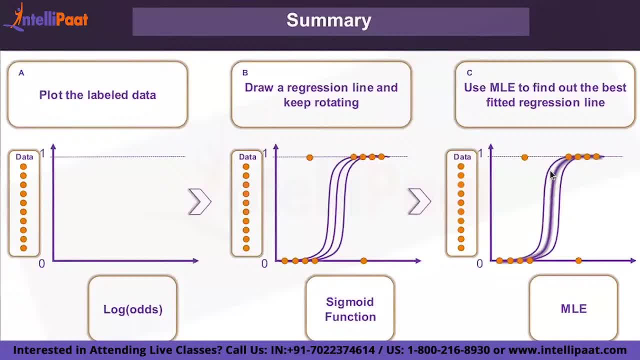 regression will is nothing but us. it will not give mle. you need to find. you need to find the maximum likelihood estimate using your straight line. so for every straight line you will have an associated sigmoid function. when you have log of odds ratio, it is a line. when you take e power, x by 1 plus e. 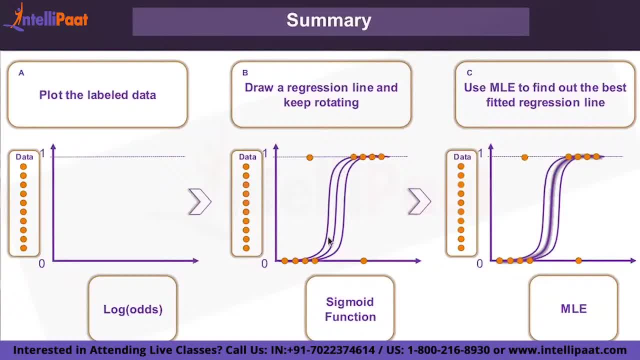 so every straight line will have an associated sigmoid curve. so when you plot all of them, everything, every curve also will have a mle maximum likelihood estimate. whichever line gives you a maximum likelihood estimate, that curve is your correct fit for logistic regression. so this this takes some time to understand. see the video multiple times, you will get it. 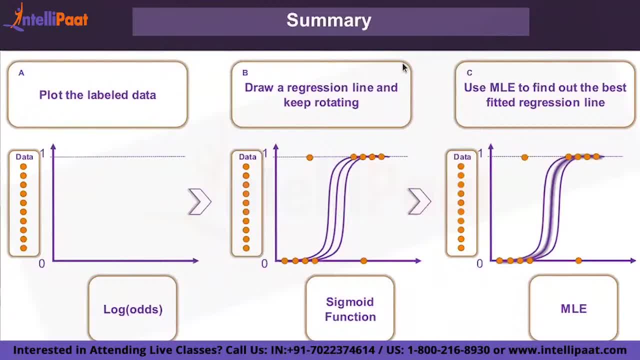 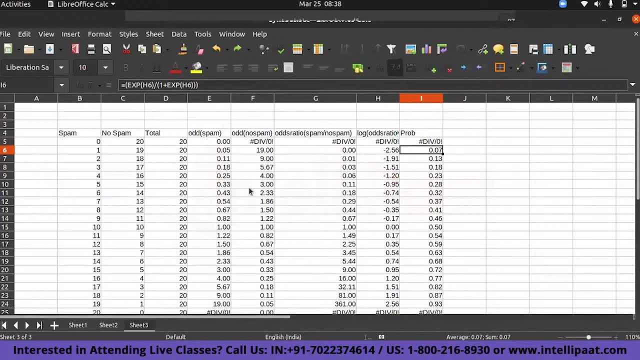 are we clear here? we will get the same line. see when we? what i told you is for the spam and no spam mail. so whatever data that you are getting is for spam and no spam. these are the data points that we plotted for this. data points. you can fit multiple lines. no, i'll give. 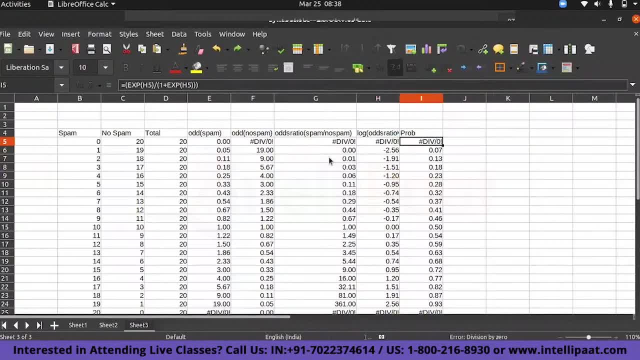 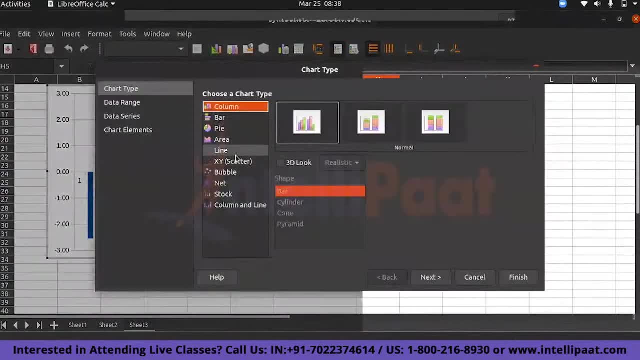 you an example? i mean, just in case you are confused, i'll give you an example. okay, let me just give an example. fine, no issues, i'll just plot a graph. you tell me how many lines i can fit to this particular curve, i mean to this particular data. 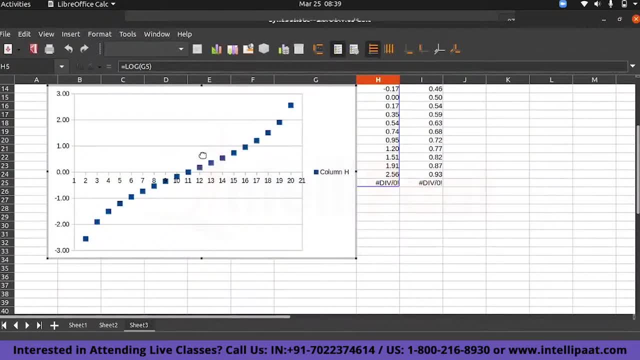 how many lines i can fit. you tell how to fit line means you can just take estimates like you, just assume that this line, this line, this line like that, so you can have infinite lines but one will be the best fit correct. just like linear regression. same linear regression concept is here you can have. 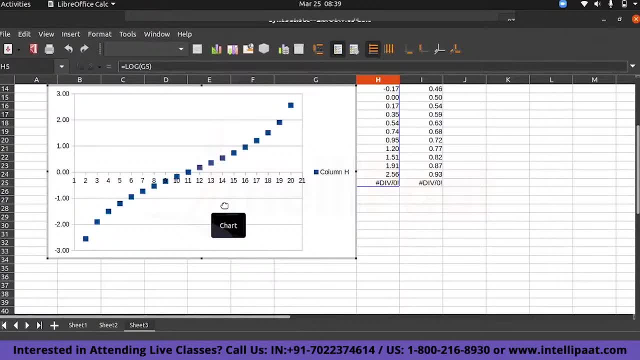 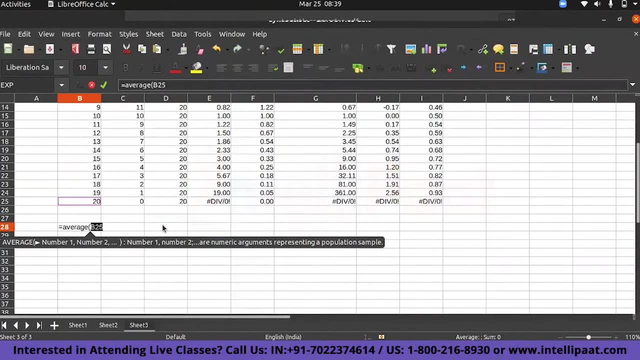 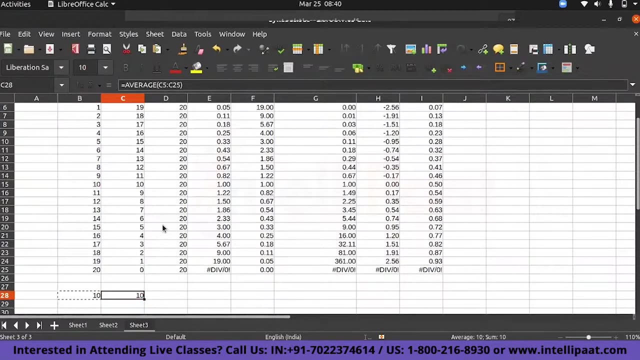 you can fit infinite lines correct and again see the same concept. if you want to fit line to this, you can see what is the average of this same average of this particular table 10. same thing: if you just do it here, this will also be 10.. so your first point in linear regression is: 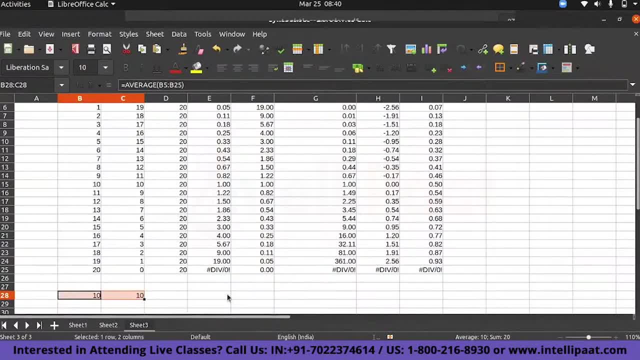 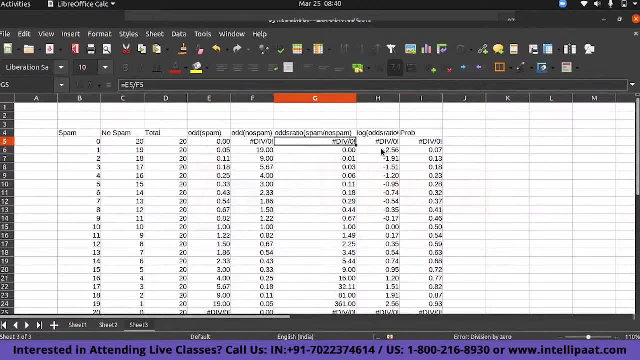 what 10 by 10.. so your line should pass through 10.. if you put a graph here, whatever i showed you, y is equal to mx plus c line. you get one one, one value here. already. you already have a 10 by 10. 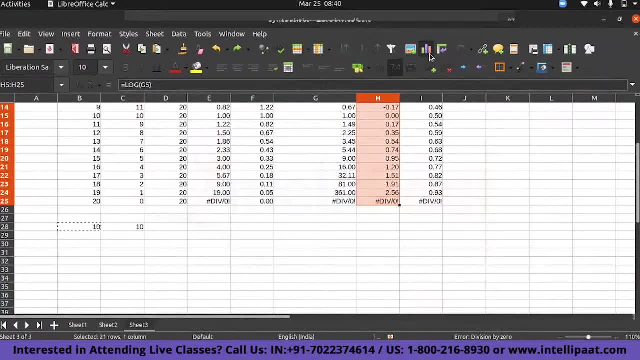 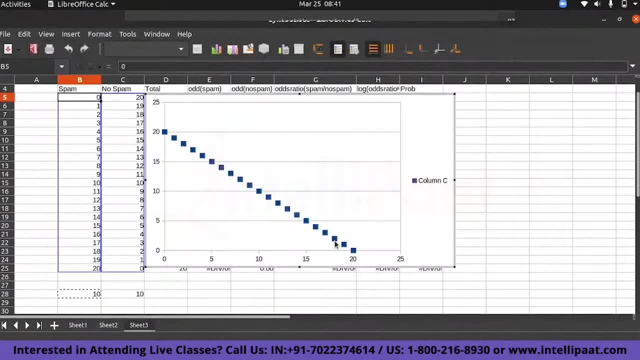 10 comma 10. you will have already one line. you have to have one line. you can see 10 comma 10. this is the middle one. you're not supposed to take this also spam and no spam. so it is actually: uh, no spam and spam. so you will get a positive one. 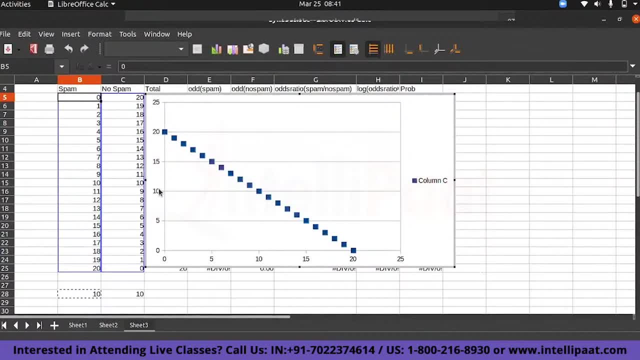 since you have taken spam, no spam, you're getting negative. so your one line will always pass through. this 10 by 10 mean point, you can have so many lines for this. i've just taken a proper example. so that's why i'm getting a line. but if you take random, random numbers here, then your dots will be. 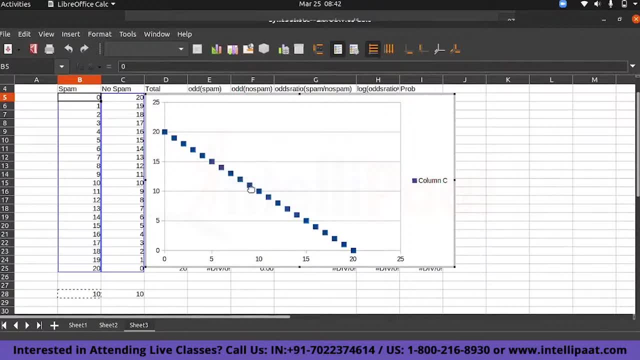 here, here, here, scattered around right, one point will pass through 10 by 10.. where the next point will pass, it will pass. it will pass through the next point. where the next point will pass, it will pass at the intercept. so make your y value zero, make your x value zero. see how many spams will. 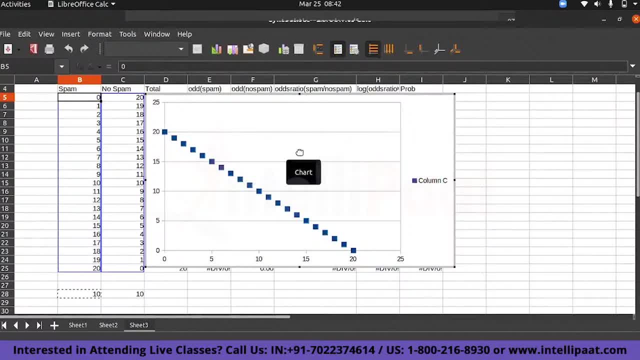 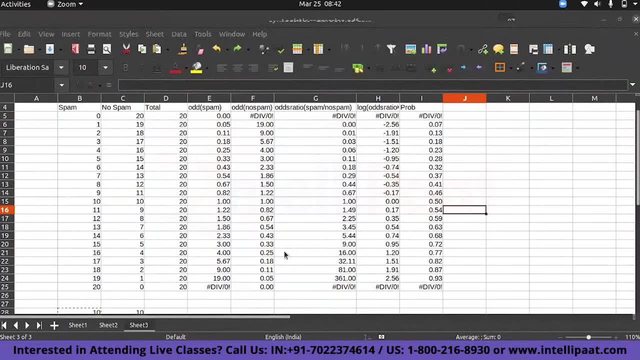 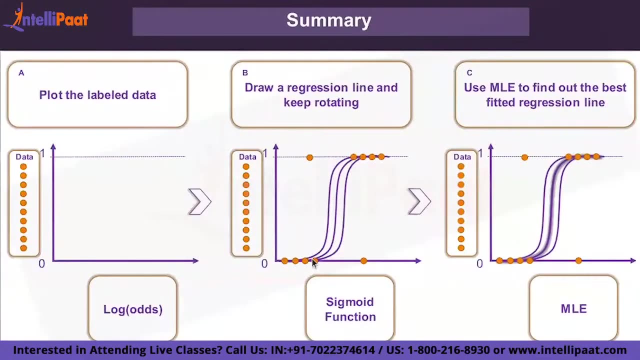 come. so if if it is zero, then it will pass through zero. like this, so like that, you can have multiple lines. so whichever line gives you maximum mle for this line, it will not change for this line, it will be same, only in reality. you know, when you take multiple data, multiple random scatter plots, no. 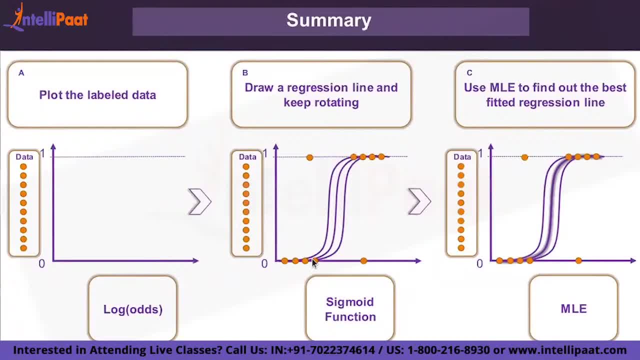 it will not be overfitting. it will not be overfitting here. maximum likelihood estimate is what supposed to consider, right? so whichever line gives you a maximum likelihood estimate, that one will be. it's not different columns, different rows in that column will be different. so when you have those multiple things, whichever line gives you highest likelihood by calculation. 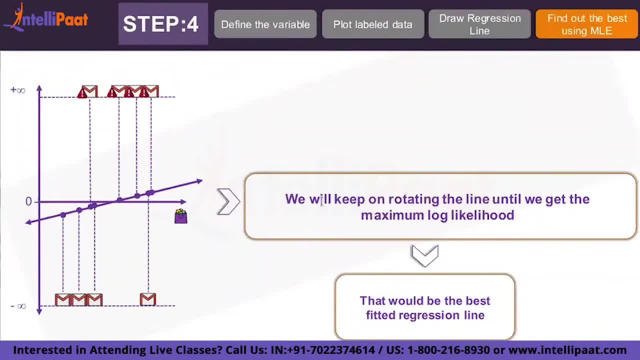 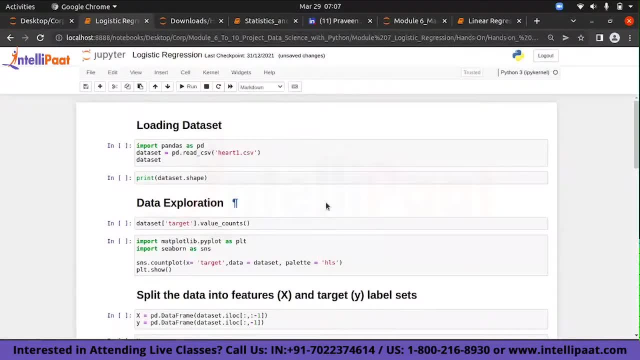 so like this: if we do that one, we will consider it as a best fit sigma and function correct. fine, all of you nice. so what we are going to do now is we are going to take a data set and then, by using that particular data set, we will continue and then we will use our logistic regression in that. so i'm 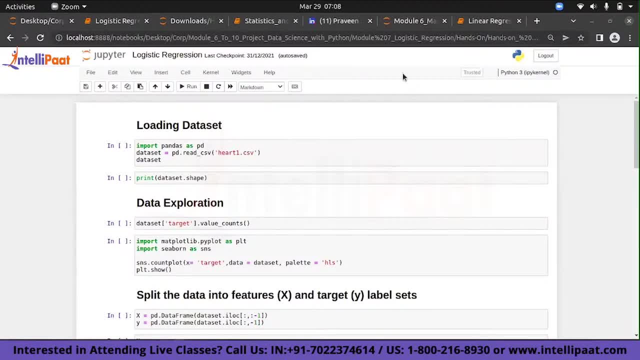 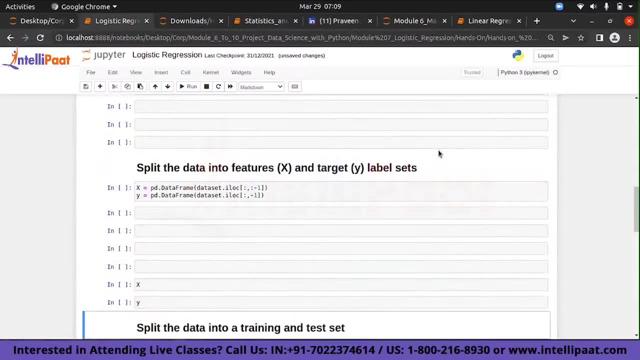 just giving you the data set. so, step by step, we will see how we can achieve things in logistic regression. there are few things which i would want you to do, and then there are few things that we will do together. you: 70,8,7,9,10,11,12,13,14,15,16,17,18,19,20,20,21,23,24,25,26,26,28,29,21,25,26,29,23,29,29,30,24.. 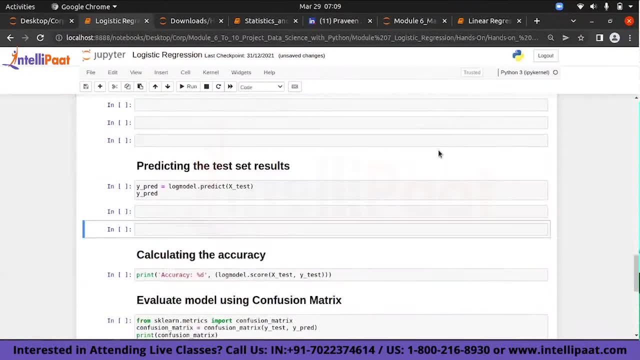 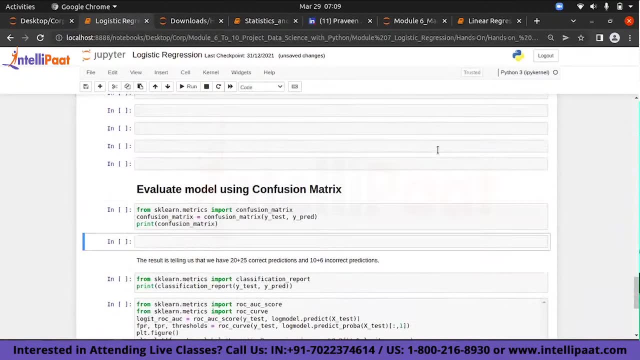 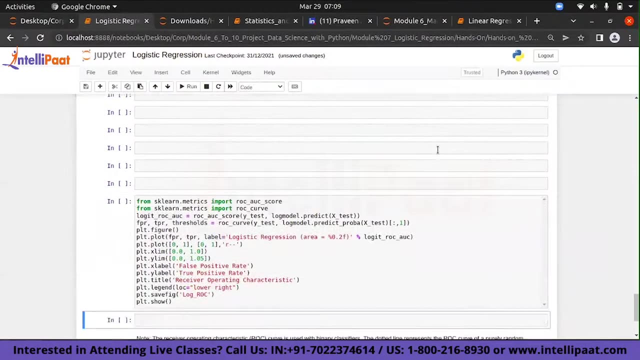 then we will go ahead and then build it. one thing that you need to understand in today's session is you will learn something very important which is called as a confusion matrix. so i will teach you what is confusion matrix and also i will teach you what is a ROC curve. so ROC curve also I will teach. 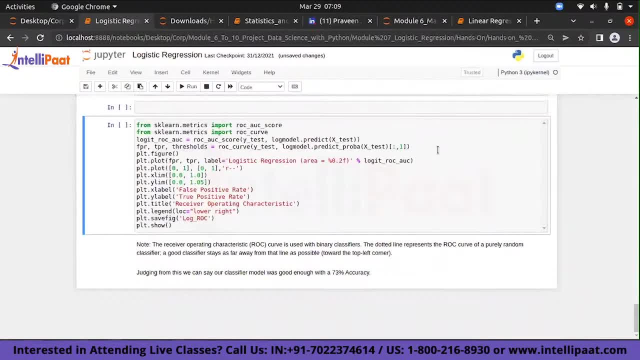 you and then we will see all that. right so, these things and all we will consider in today's session, and then we will start. right so, confusion matrix. right so confusion matrix is totally different. this is where we will get into the important concepts, so 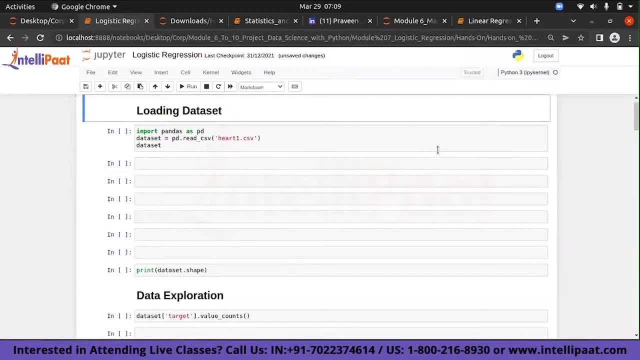 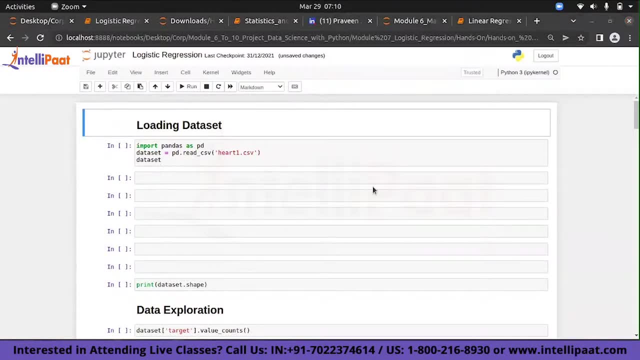 matrix and all of that are important, very important, so let us go ahead and then do it so before going to that. so today we are going to implement the logistic regression using the code. so today is the coding part right, so hope all of you are okay with the linear regression one. 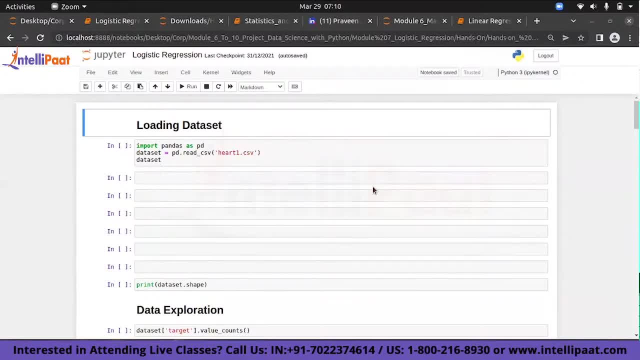 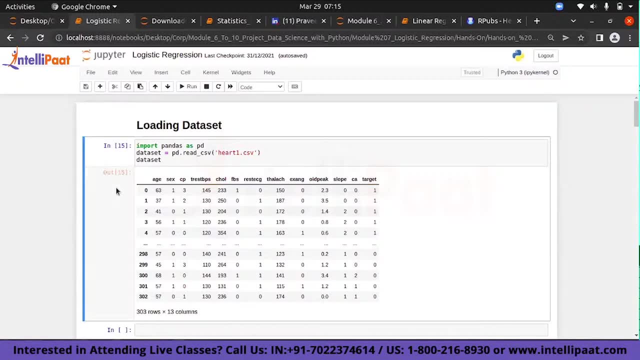 so we are going to do the logistic regression in the form of code. cool, so now what we are trying to do is we will understand this data set first. so what is this data? right? so if you can see, you have some variables which there are some variables which you are seeing, so you can see, age is in. 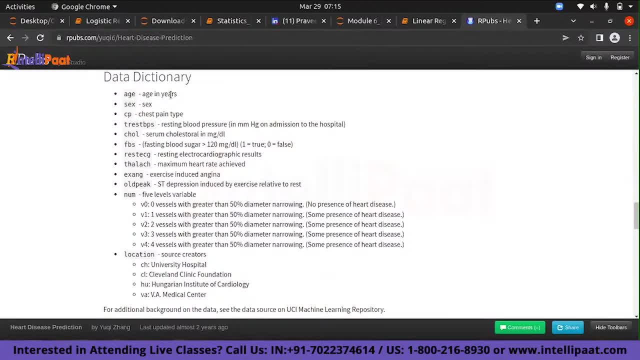 years. gender. cp means chest pain type test, bps, which means resting blood pressure. so t rest bps means resting blood pressure. cold means serum cholesterol. fbs means fasting blood sugar. rest ecg means resting cardiographic result, which means what is the heartbeat cardiography that you get when you are resting. so resting cardiography, then uh, thalac means maximum heart. 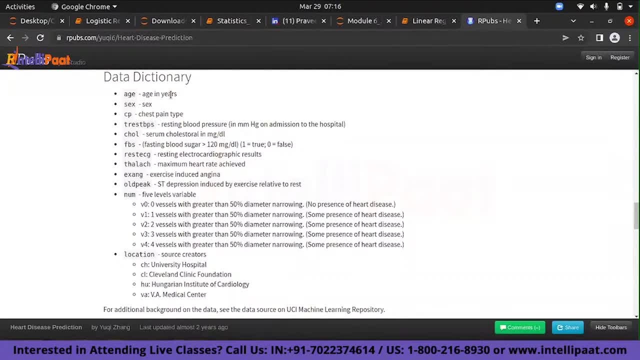 right, so that is a term. uh, then you have something called as x, x, x and x and means exercised, inducing, agnia, some kind of- uh, what can i say? disease or something, so that they are having it. um, i don't know the exact meaning of that because they are medical terms, but 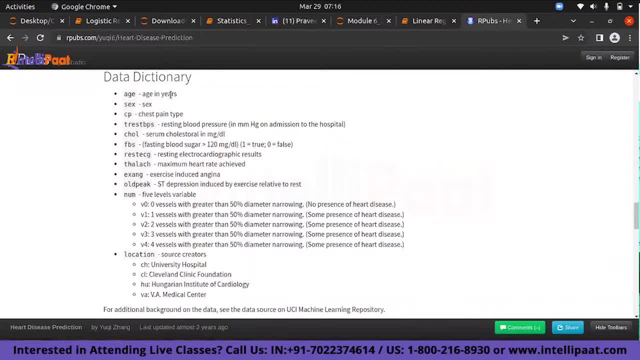 they're all our x variables. old peak means depression induced by exercise relative to rest. that is one num, five levels of variable, um, so five levels of variable, which is v0, v1, v2, v3, v4. so all these things, a location. you can see which hospital they are from, where it is captured. so these are some of the main. 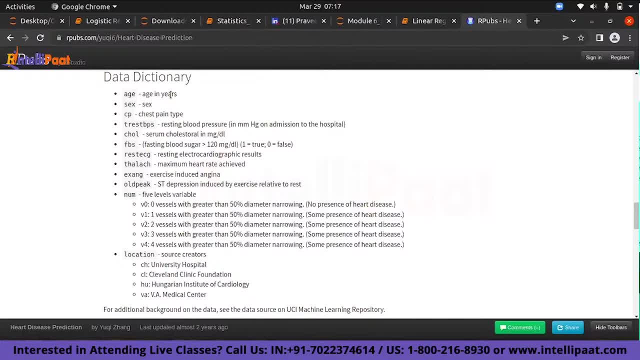 attributes that we have for the data. so here what we are trying to do is we are just going ahead and then checking out our x variable and y variable. now you understood the data, you need to understand what is my x variable and what is my variable, y variable. so to do that, 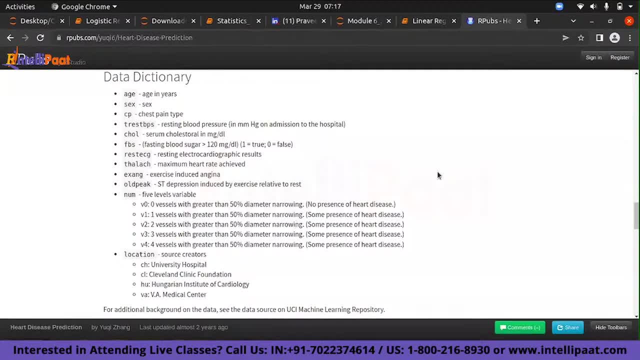 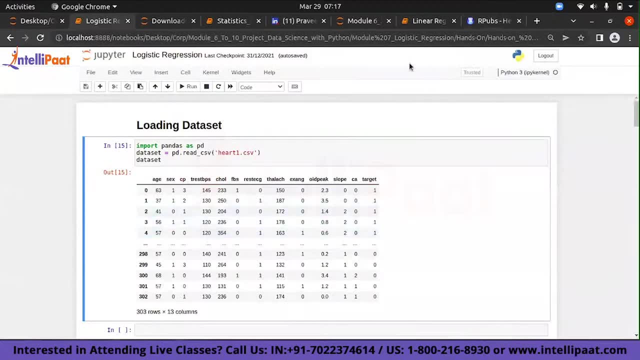 what we are trying to do is we will just go back to our. that's okay. i just took a data dictionary. it may not be the same in case. if you don't have it, that is fine. so this is a little limited one. they have given you the target, so there's a small change. so other terms are there, right, just to. 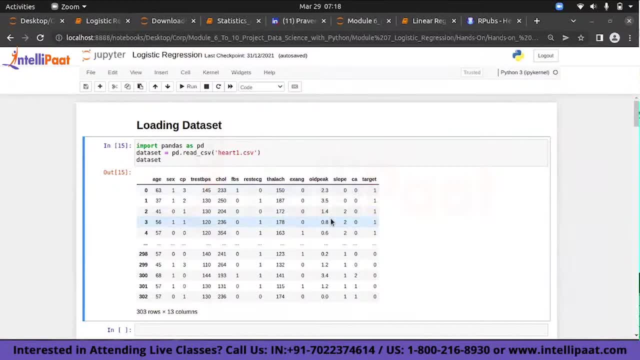 understand the other terms. i took that right. so data data set. you don't worry that it should be the same. it is like a little different. that's okay. now what we are going to do is there are two major things that we are checking here so you can see clearly. you have something called as a target. 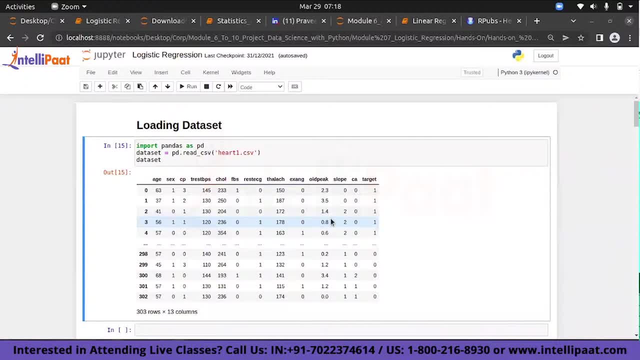 so what does the target mean? target means the person who is having one is highly likely to get a heart related issue. a person who's having zero, he will not get any heart related issue. so these things are something that we are getting it right now. so now, once you have these, import, 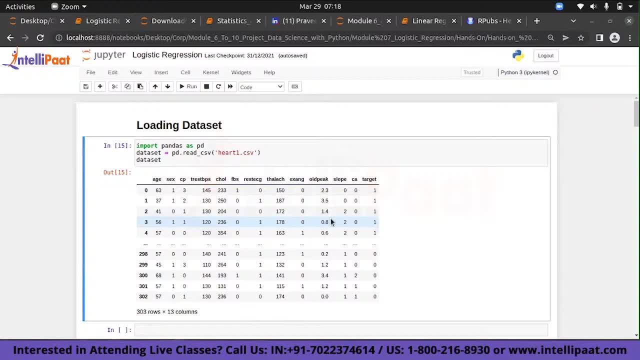 pandas, spd. read it and then do it. all of you are able to read it. can i get a yes or no using the same code, keep the file in the same location and then read it, fine, cool. so if all of you read it and now you understood. now what we are going to do is just like how we built a linear model for a. 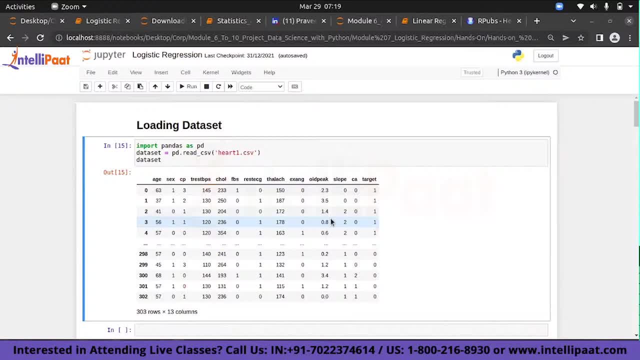 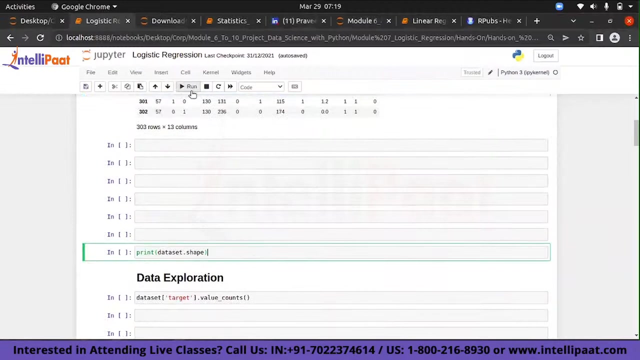 price. we are going to build logistic regression model for our heart related data. a basic classification model is what we are going to build right now. our going to achieve that is something that we will be seeing now. right, so you have pandas, pd, heart, csv. now the first step in this is we will just go ahead and then explore the data so you can just 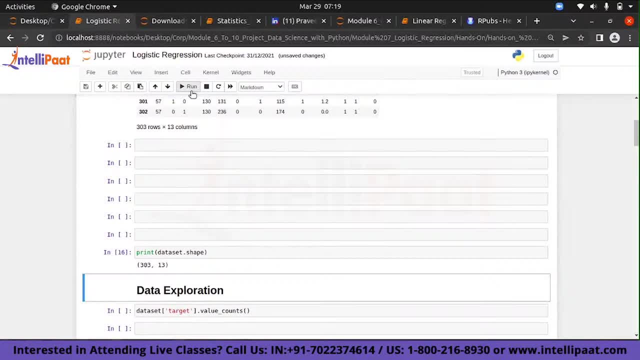 go ahead and then do all the describe functions and all that and then see. but what i'm trying to do is i'm just trying to explore my data. so there are 303 rows, 303 patients and 13 columns. out of that 13, the last one is my target. 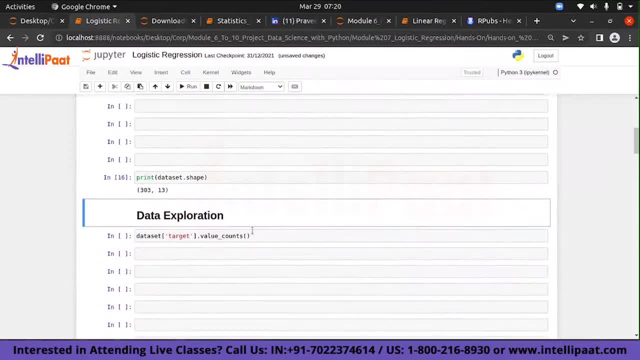 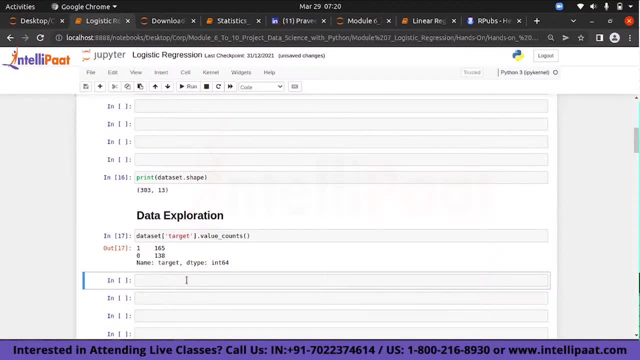 so the first thing that i'm going to do is i'm just going to just do a value. dot counts, if you can see, this will give you differentiation between your ones and zeros, right? so can you do this? i'll tell you what are the significance of this. can you just do it? once you're done, you can type: completed. 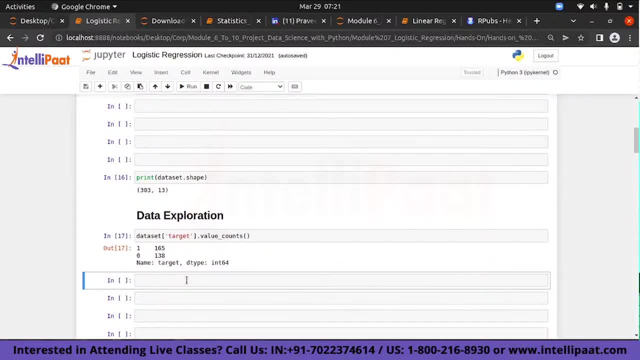 so the main thing that we are looking at here is: we are checking what is the proportion of my positive and negative data. so when i say what is the proportion of my positive and negative data, i am just seeing whether the data that i am checking is imbalanced or not. so what do you mean? 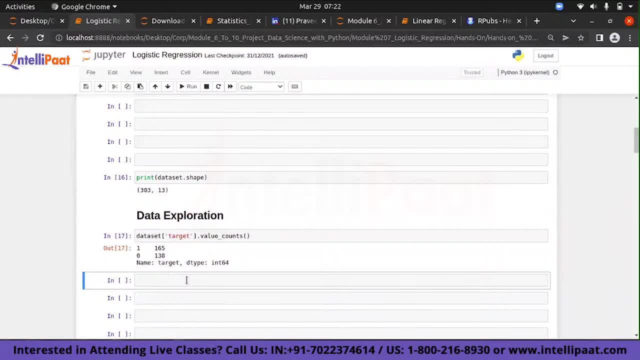 by an imbalanced data is whenever you have your ones very less compared to zeros. understand this: whenever you have ones very, very less compared to zeros, that is called as a imbalanced data. right, so means your value of ones will be very, very less. so usually those kind of things would occur in. 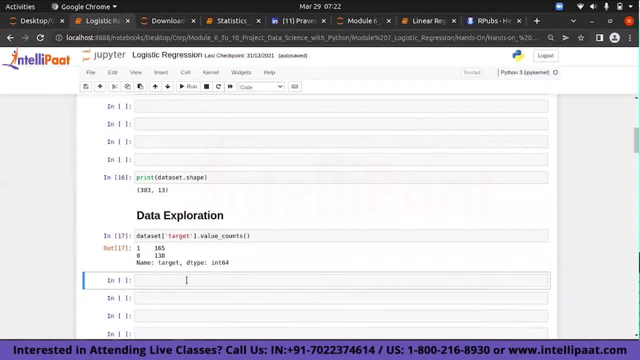 these places right, so you will get them very often. so that is something i wanted to tell you. it is imbalanced. now, whatever data that we are using is not imbalanced because you have almost a 50- 50 percentage, are we okay? the bracket you should use is a round bracket. you have used a. 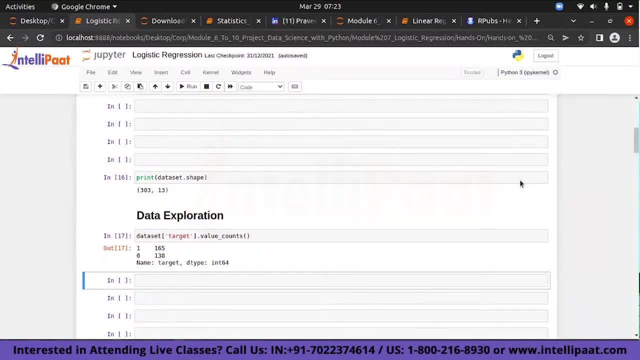 flower bracket. so that is why you are getting a error right. so all of you got the importance why we are checking this particular thing. if you have very less- let's say maybe one percent, two percent, like that- then it is called as a imbalanced data. right value counts will give the number of value counts correct. so if it is, 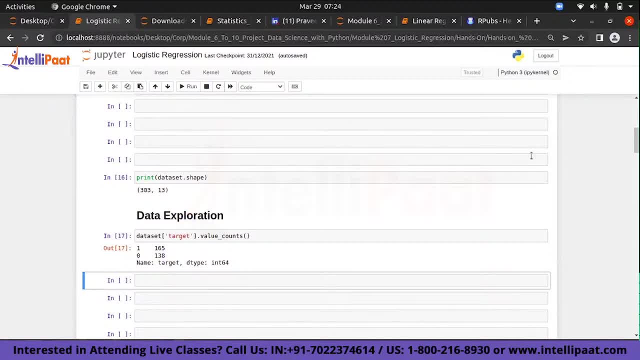 imbalanced, then we have multiple ways to deal with it. so we can go ahead and then do a sampling under sampling, over sampling. so that is again a completely different thing altogether. i'm just telling you for your understanding, these things, you can go ahead and then do so. i'm just 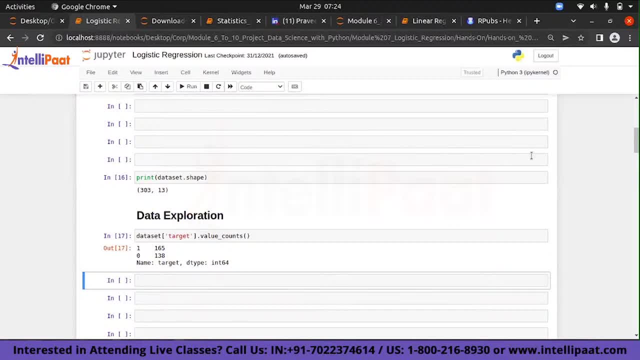 giving you an estimation of the imbalanced data. so if the data is imbalanced, you can go ahead and then do multiple ways of arriving at it, and then you will be able to achieve it. so that is something i wanted to tell you, right? so, under sampling, over sampling, multiple techniques. 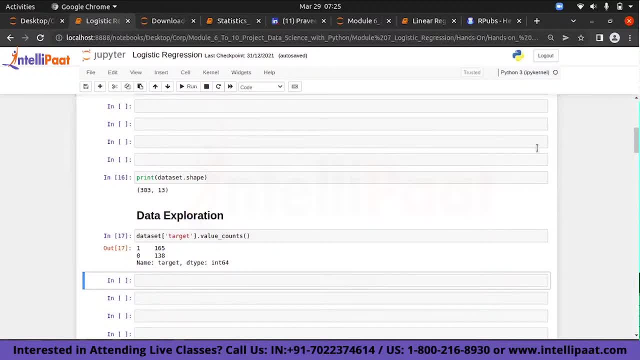 are there to handle it. this is not imbalanced, because you are having an equal, equal kind of a data, so this is not an imbalanced data. so let us go ahead and then see how exactly we are going to achieve this. so now what we are going to do is: we are understanding it that the data that we are 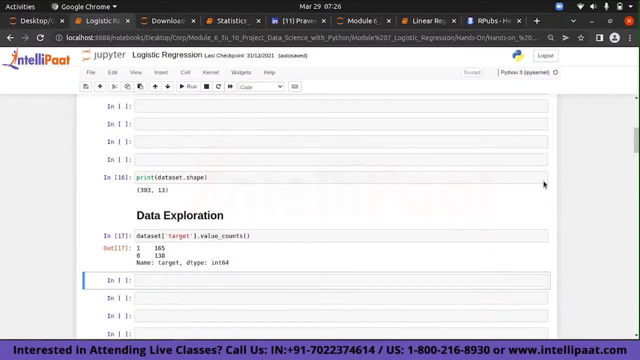 using now is not an imbalanced one. we can proceed further and then we will be able to use it for our analysis without any issues. so we understood that and then now currently what we will do is we will just go ahead and then see how this can be used further for our analysis. so we'll just go ahead and then check that and later. 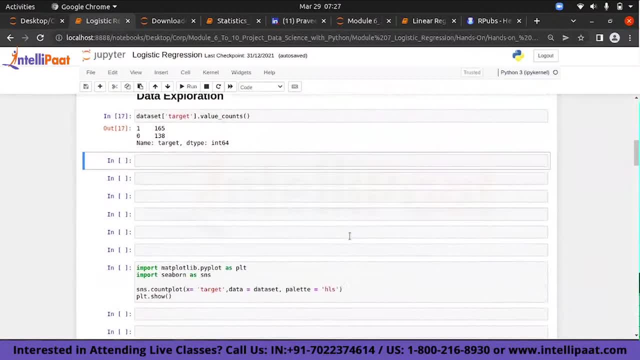 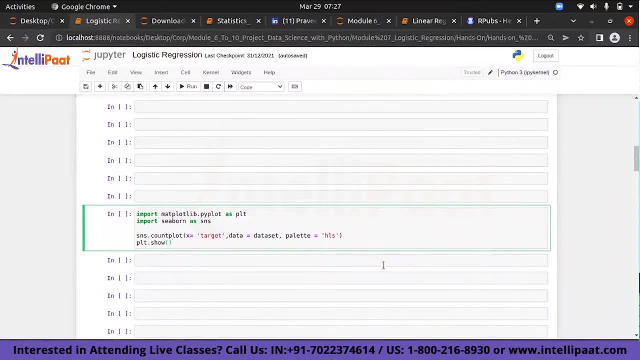 we will see how it can be done. we will go ahead and then check, plot how our target looks. this is also a continuation of the same thing: how we are going to use it for our analysis. so, basically, whether we are going to take it and then check whether we are going to use it for our analysis. 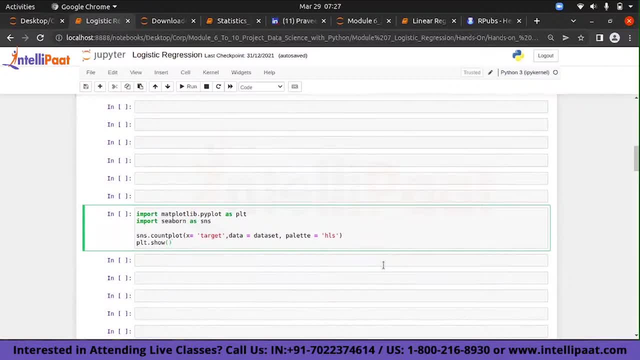 whether it is balanced or imbalanced, that one. so we are just checking this out. so i request all of you to please do this as well. just plot it using this one. it's not compulsory if you have done the above, but for the sake of completion, please do it so that all of us are in the same page, right? so? 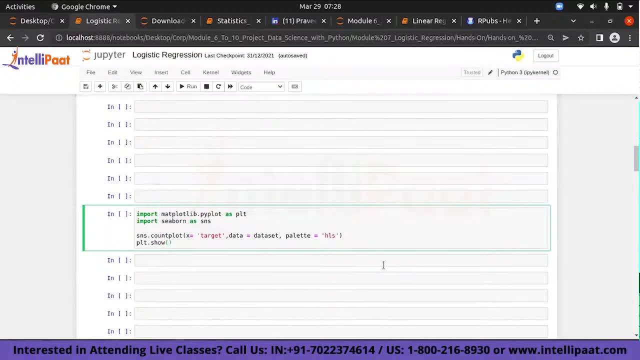 we can just go ahead and then do it. once you are done, please give completed. yes. so it is just giving you a visual representation of what we saw, so nothing much. but let me run this and then we will see. right, so you can see. you're just looking at it at a visual level, so you're not. 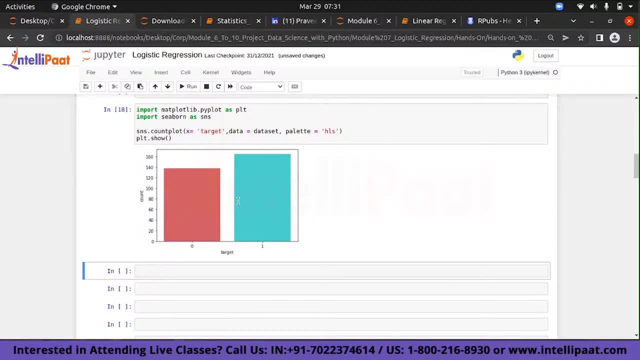 looking at it anything else. so it is just a visual representation of whatever we have seen. so that's it. so what we are trying to do here is we are trying to generate a bar graph. the bar graph- what you are seeing here- is mainly used to visualize the target variables if you want to make a career. 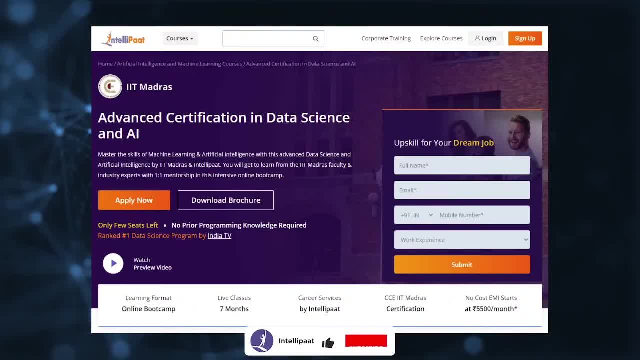 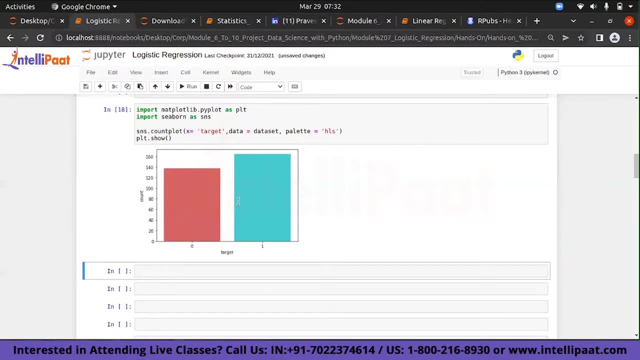 in data science, then intellipaat has iid address, advanced data science and ai certification program. this course is of very high quality and cost effective, as it is taught by iit professors and industry experts. how many target variables are there? so this is as good as the previous one that you did. the value dot counts, it will just. 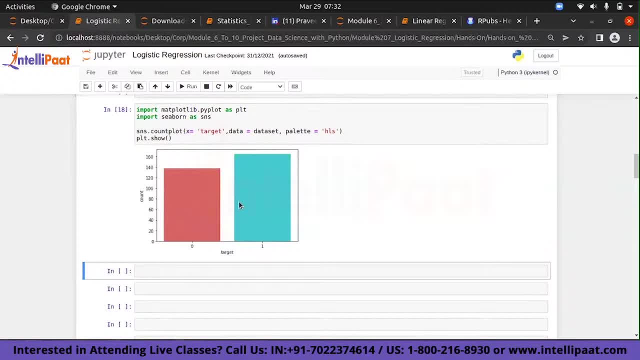 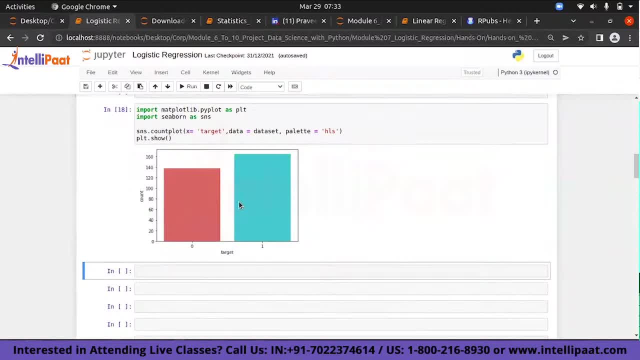 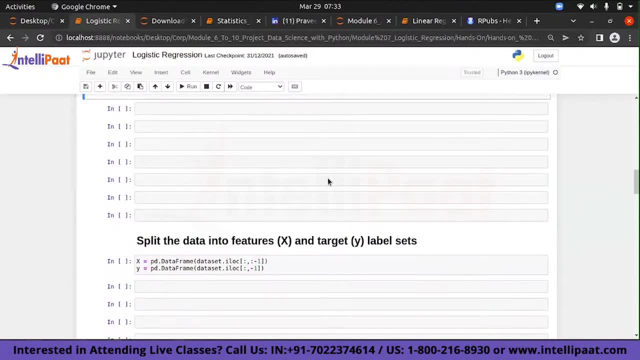 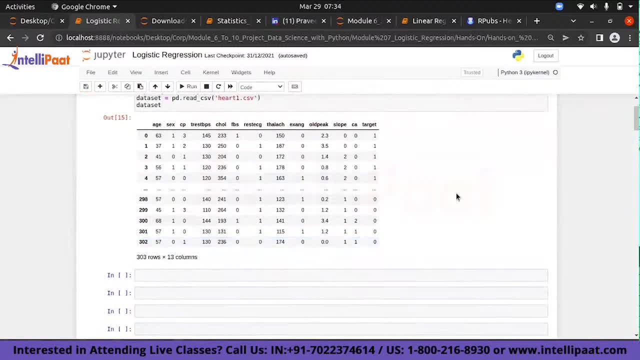 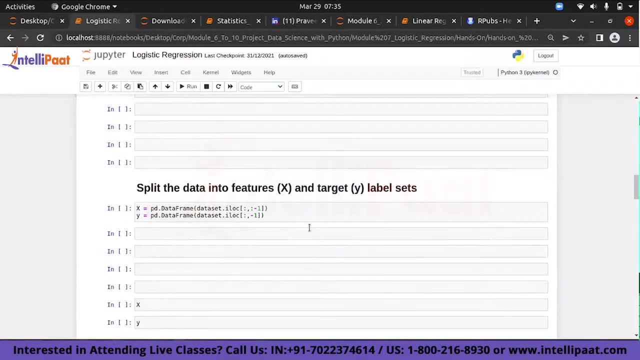 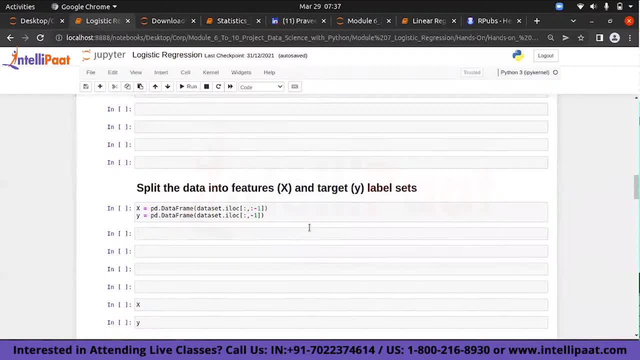 just a standard. so you don't. you don't say like this is how it should be and this is how it is, just to maintain a standard. we are having it. so it's a markdown cell. so you have to make it into a markdown so you can see cell. is there no cell type? if you convert it into markdown, it will come. 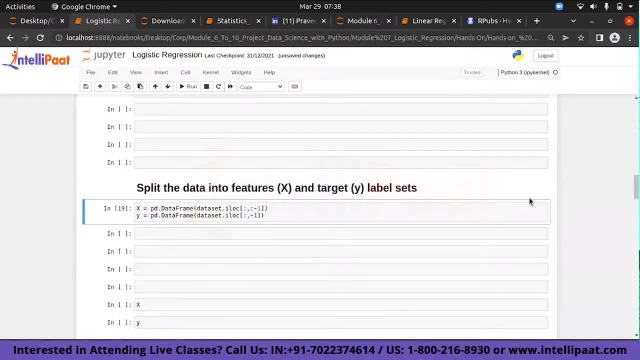 like this: so once you split this, you're having basically a x and a y, which is already created. now, what we are going to do? we have to do something next. so what is it that we are going to do? it? can someone tell me any guess based on what we have learned till now? you want to take? 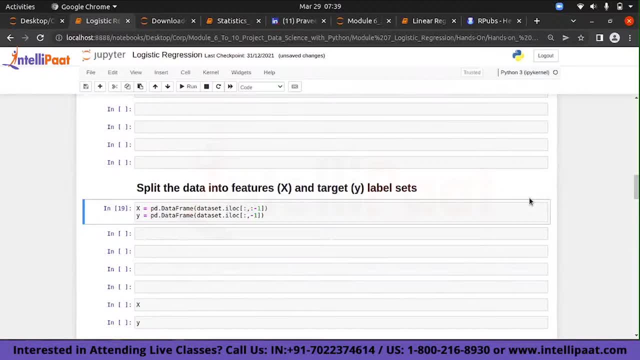 any guess? yes, so basically we want to do something called as a train test split. so why do i need this train and test split? all of you are aware train and test split. we need it because we want to train our model on some data and later we have to test the same model. so once we train it and once we 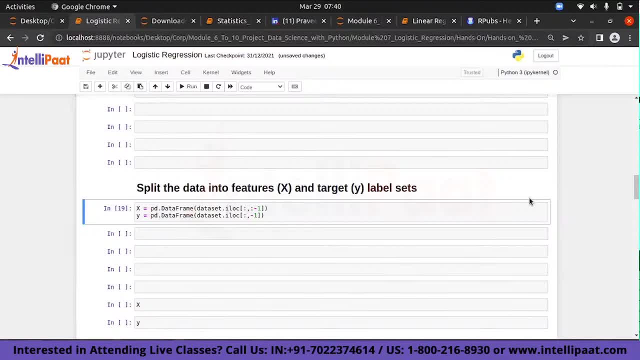 test it. we will be using those things for building our model. so, basically, training and testing is the process that we usually use, so that's why we will use that. so we'll just go ahead and then see how we are going to make this thing happen. right? so we see what is our x and then we see what is our y. 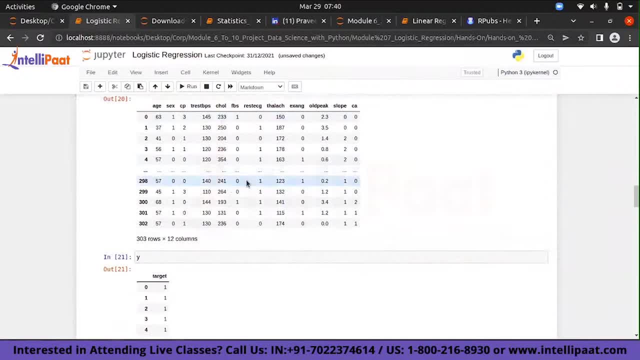 so, basically, you get all the variables into this and then you will be getting just one extra thing, which is your target, into this. so these are two things that we will get, and later we will just check how things are working at this point in time. so now, having said all these things, we will just go ahead and then see how our analysis and how our 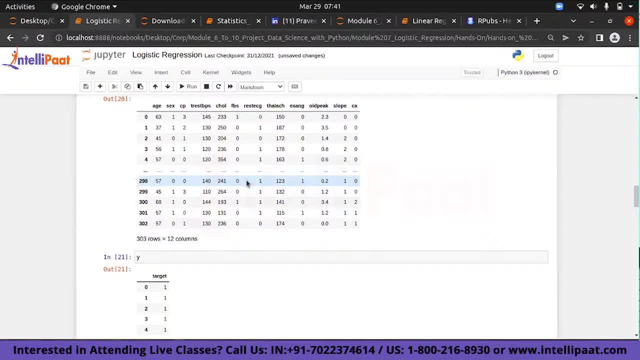 functions are working. so let us just go ahead and then do a small deep dive into this one, and then we will just go ahead and then see how it works right. so we can just go ahead, do a very small deep down and then see. so see, there are multiple things that you can do so you can check correlation. 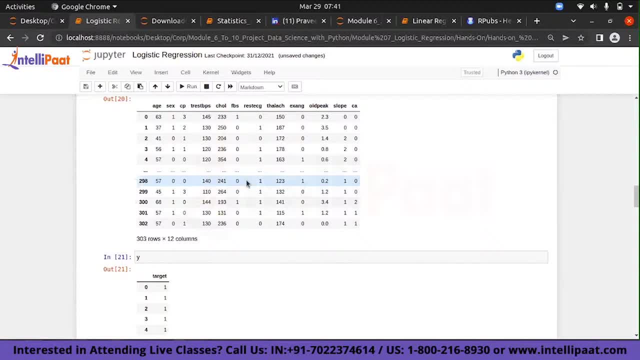 you can remove them. you can do all of that. what you said is right, but our concept today is to build a logistic regression, so that is why we are entering into directly building a model. so when you build a proper model in reality, so what you're supposed to do is you have to do a full 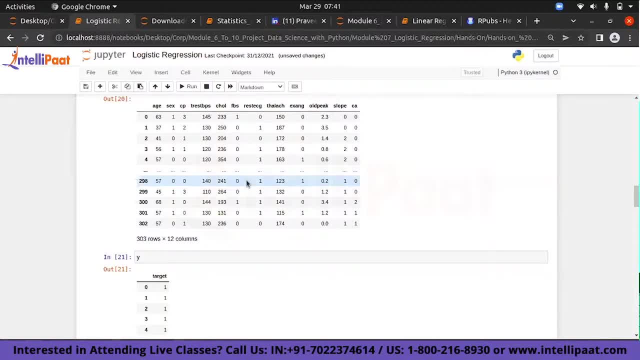 fledged eda. so, if you remember, we did a eda in the previous sessions where we were checking the every variable: what is skewness, what is kurtosis, something similar to that. we have to check every aspect of the data and then build a model, right so? but now, since we are our, we are 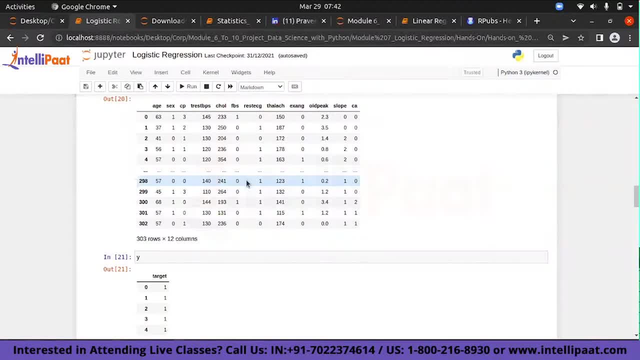 understanding logistic regression. so our objective is a little different, right? so that is something that we are trying to do. so it is like learning a small, small snippets or small, small modules and then, in reality, putting them all together. right, so the first step is to start out and find out where the model is. so that means we are going to 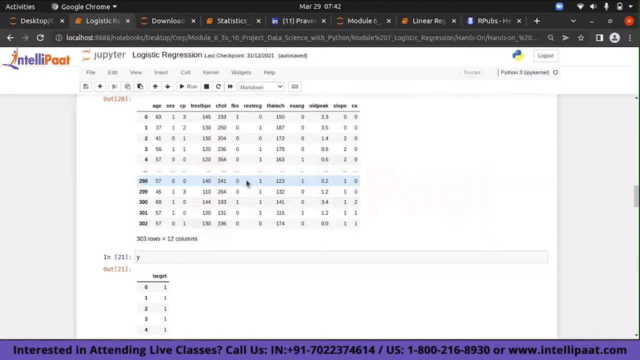 show you the model, design these models and then in practise them. we are going to do a little bit of a fledged regression and then we are going to show you a normal regression. so we have to do that and then, when we are all ready, we are going to see what the model looks like and when 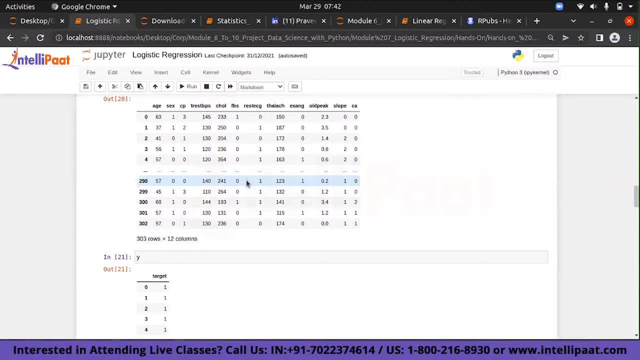 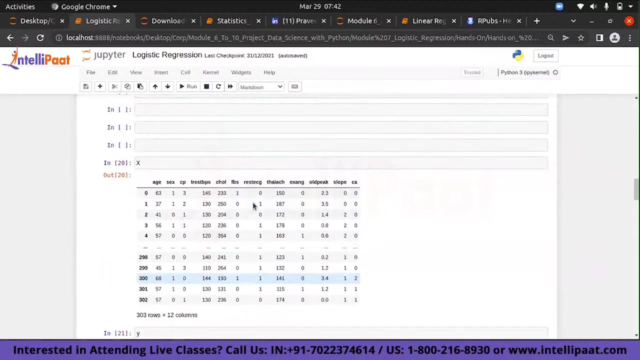 we are finished, we are going to go ahead and we take a look and we are going to go ahead and start to build this model, right? so this is our logistic regression. so the model that we are you, that is something that you do, it now we understood. 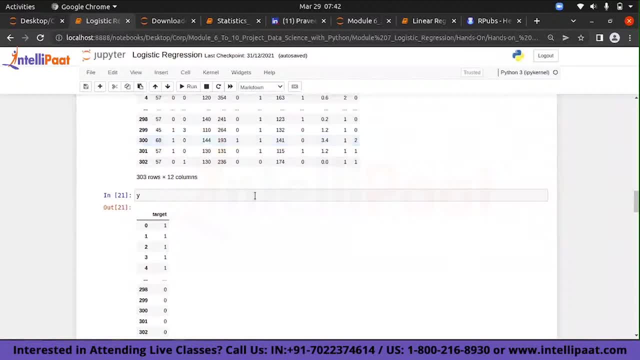 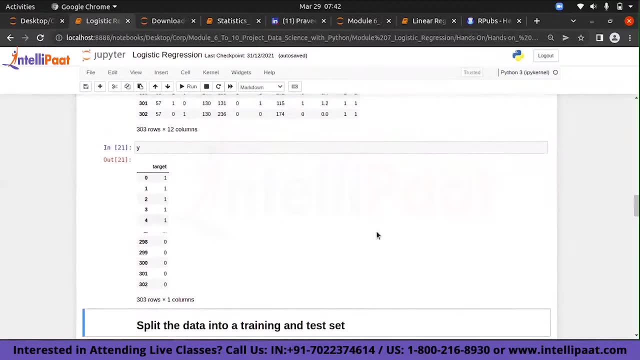 the x and y. so now we are splitting it into the training and testing data, right? so can someone probably take a guess? what did we use to split our data into training and testing data in our linear regression? this is something that we would like to learn. can. 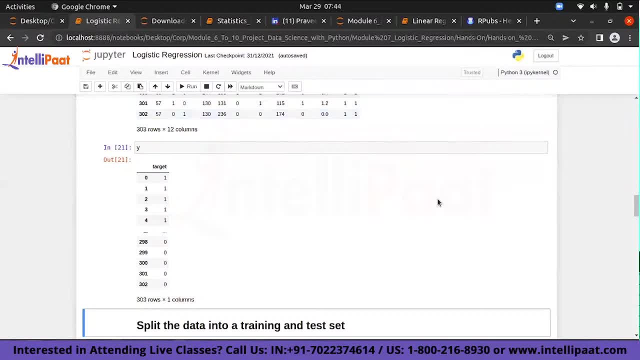 you just try that out once. i'll give you one minute. try how to split it into x training, i'll give you one minute. yes, so most of you, whatever you need to, So whatever you have done, I think you are able to get it. so whoever is the next can express what I explain and what I say. so that is good. 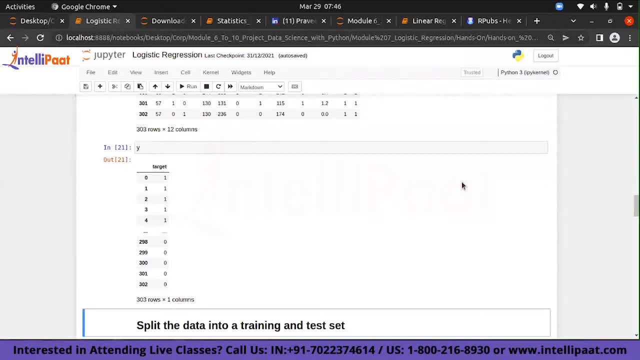 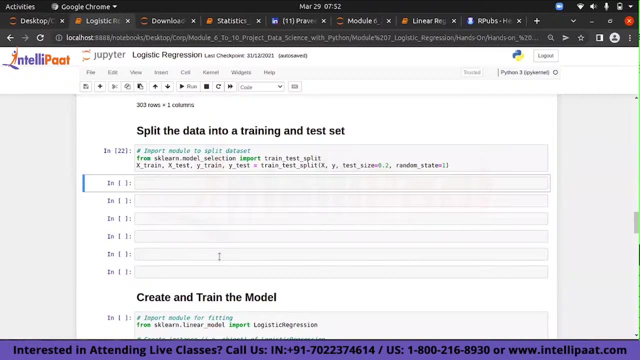 Now what we will do is I will just show you how exactly we are trying to achieve it and then we will see. So now the next step, once you have train and test data set, is building a model. So you have to just build one model xy, where we feel the data to split correct. 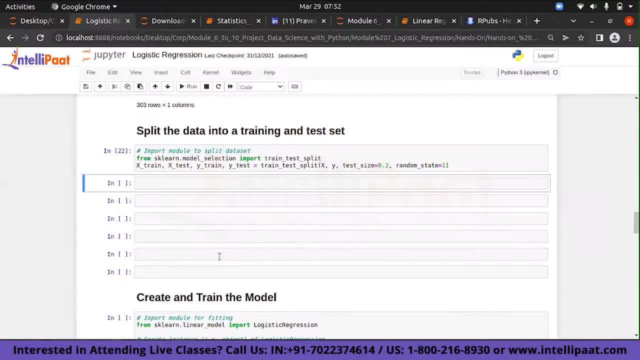 So into x and y, you are splitting your data, you are right. So what we are going to do is: once you have this, you are going to build a model, right. So how we are going to do that, how we are going to use it, that is one thing that I will show you. 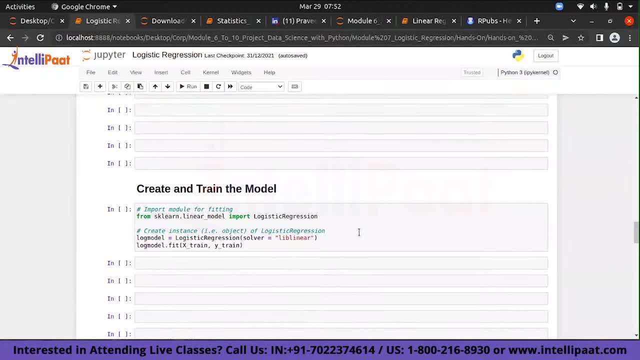 So these lines I will show it to you. this would be a little challenging. I will explain you few things, So you can just start with this. I will explain you couple of things. let us see Right, so you can just see this. 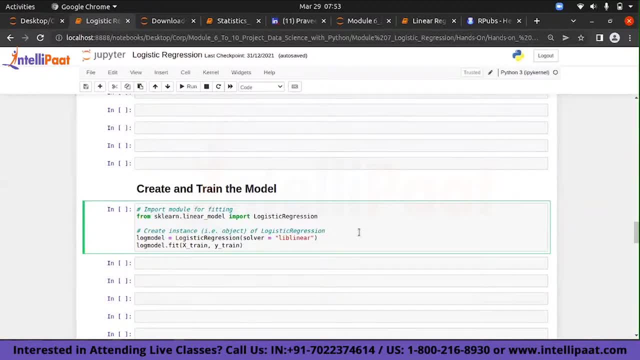 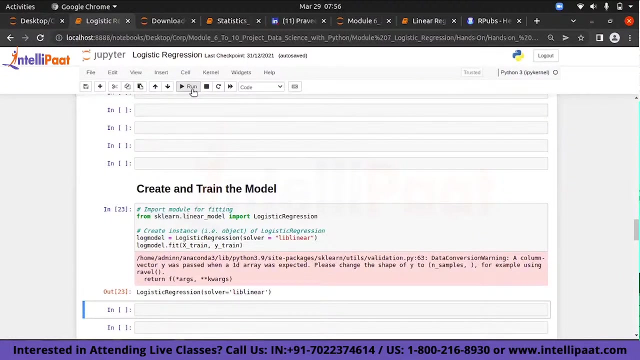 Just try to use this code. There are some things which I want to clarify to you in this one. I will do it Once you type all these things. completely Ok, that is cool. So you will understand this in a little detail now. 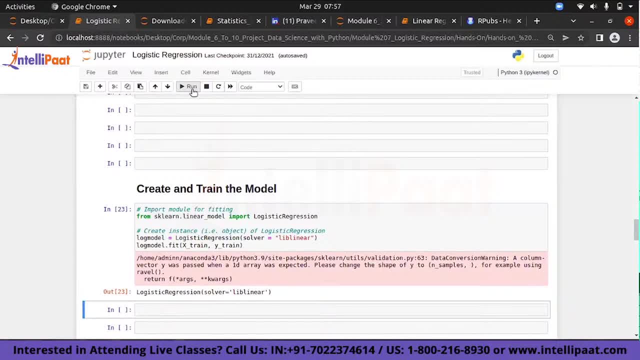 So that all of us are aware. So I will tell you slowly. It is just so simple. Just try to use it or speed up your writing or change the style, And then you can do it yourself. Again, as I have said, the distance that you are going to need is 5, which is 3.. 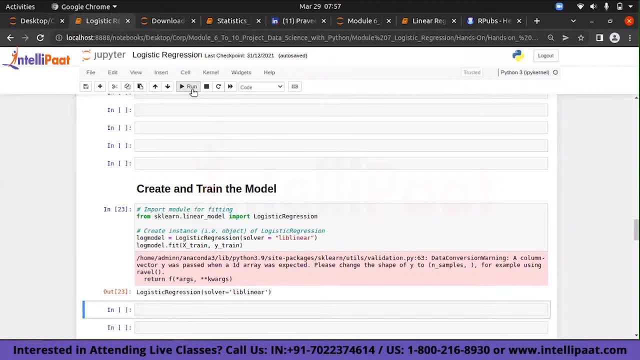 So what we are doing is 5. You want to copy the distance here, So you will need to copy the distance here, And then you are going to copy the distance of the distance here. Ok, and now we are going to do this. 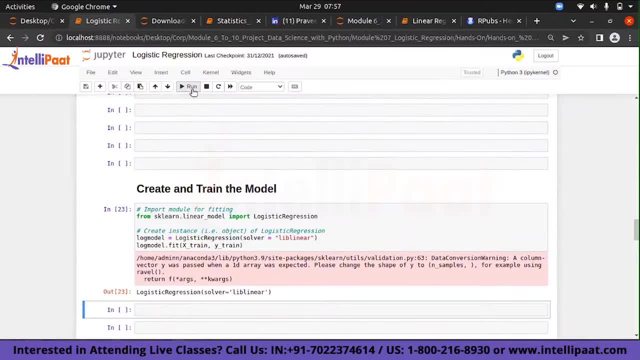 our sk learn dot linear model import logistic regression. so what exactly that does? can someone tell me? take a guess, first line, so that one all of you might should know right? so basically, your sk learn has a function which is called as logistic regression. correct, that sk learn function will give you all the things that documentation. so i have multiple 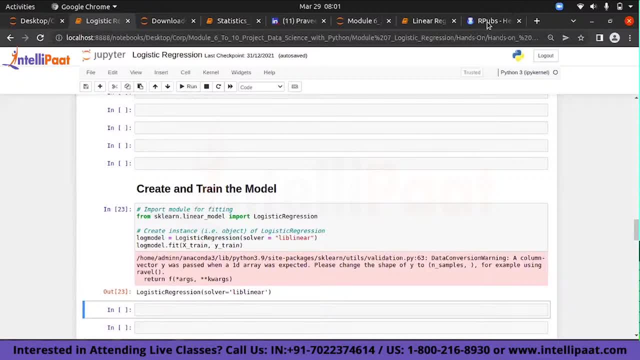 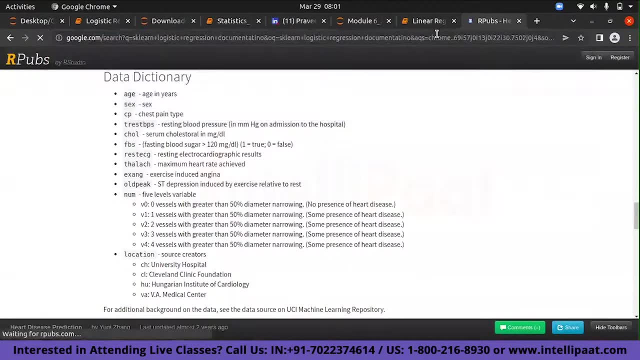 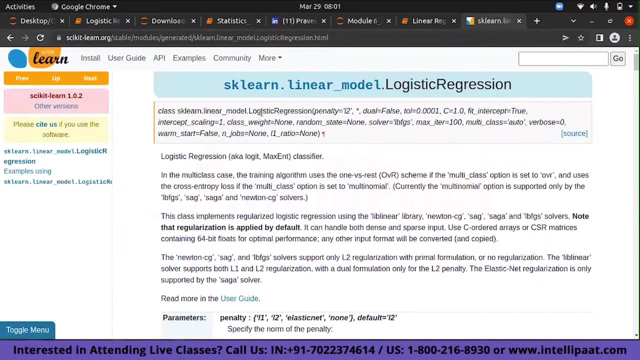 types of solvers. so what those solvers do something. we will go ahead and then understand sk, learn logistic regression, right? so i'll just go here so you can see. there are so many things that come in default. these are all the parameters. for me, solver is something which is important, right? so solver what it does. 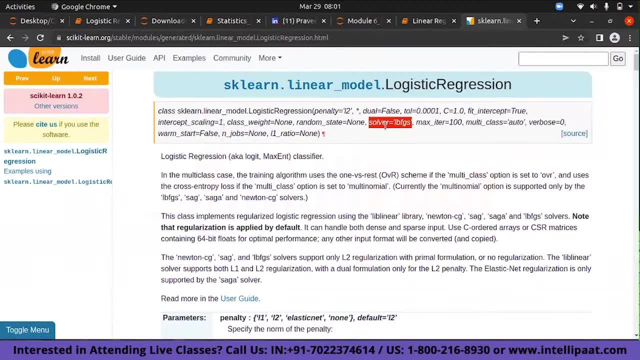 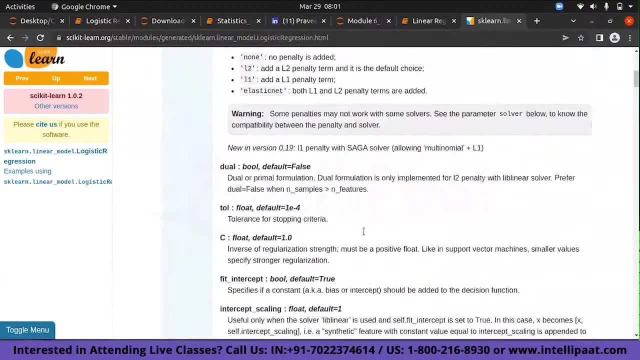 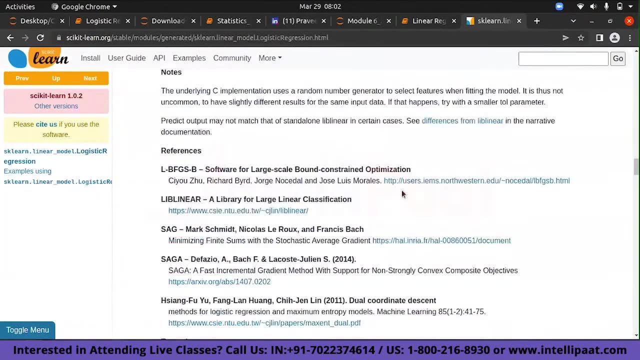 is it? it is a mechanism to find the best fit curve. solver solves the problem to find the best fit curve. so i'll show you here so that it is detailedly explained why i'm showing you all this is because i would have just told you like that few things i don't remember. point number one and second thing is, if you want, 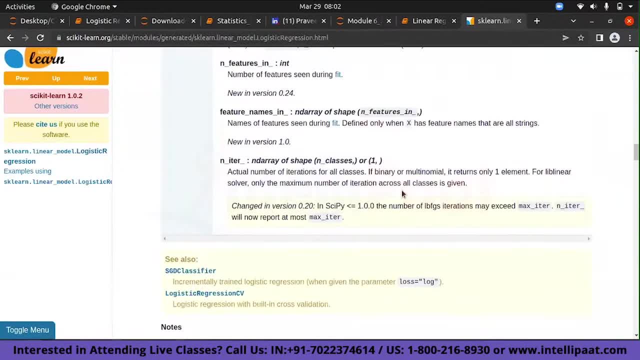 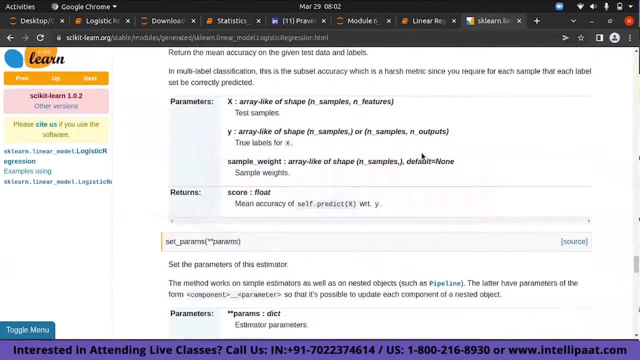 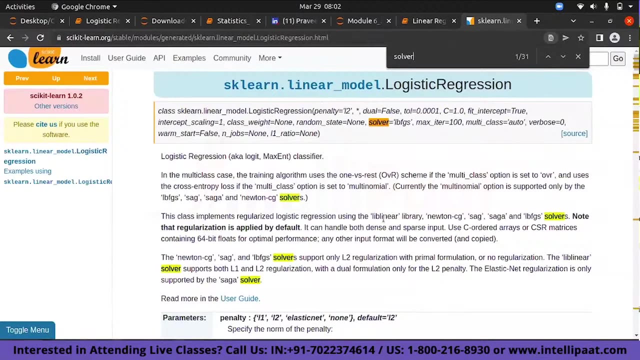 to find out on your own. next time you should be able to see it, you should be able to understand from where this thing is coming from, right. so with that objective, i'm just trying to tell you. so, right, yeah, you can see there are multiple things that are there in solvers. so, basically, 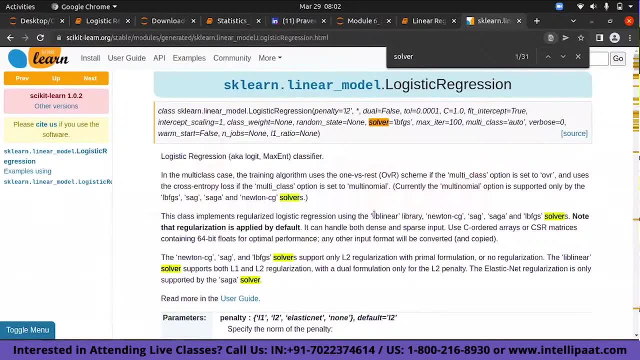 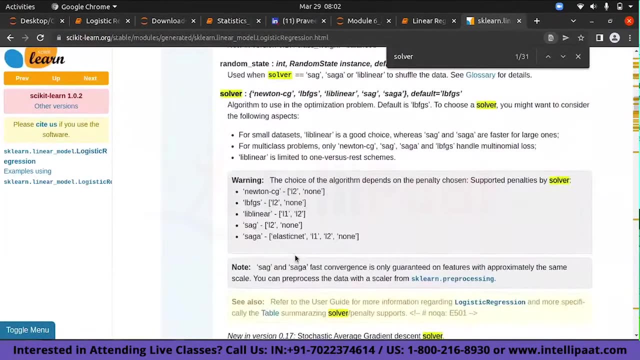 there are four or five types of solvers. you can see lib, linear, newton, cg, sag, saga and lbfgs solvers. so what are these? liolnir and all of that we will see in the down. so i'm not going into the detail of every solver. 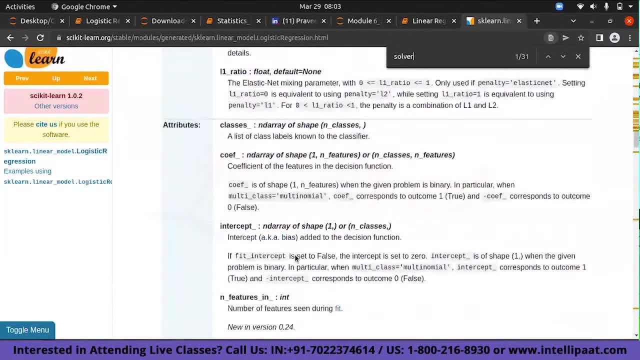 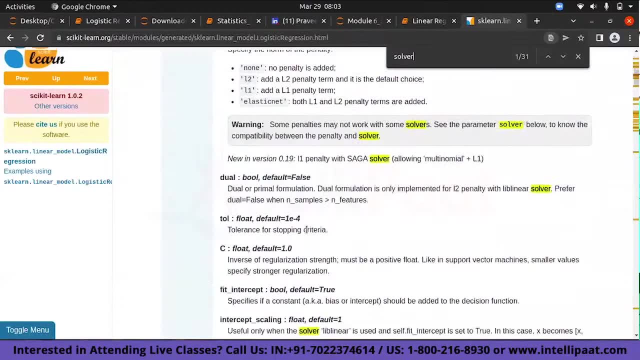 but just understand how exactly these things would work right. one one solver is used for one of purpose, so which is listed here? i'll show you. there is a place where they have listed all the solvers so that i can just show it to you. you can see here. so these are some of the solvers that are 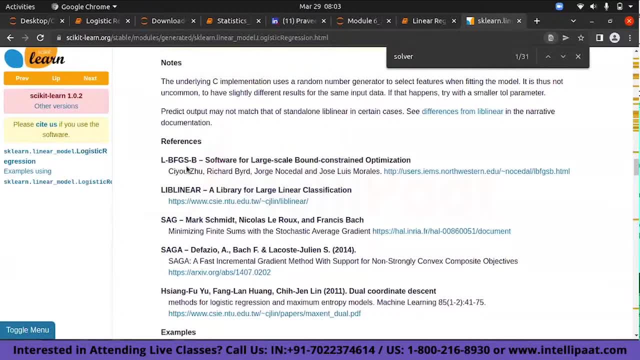 of the solvers. So what does LBFGS stands for? It stands for large scale bound, constrained optimization, which means it will find out your best fit curve based on certain criteria, using large scale bound, constrained optimization. Now LibLinear, a library for large linear classification. 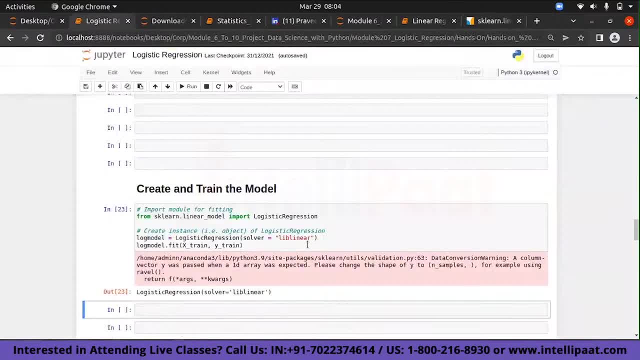 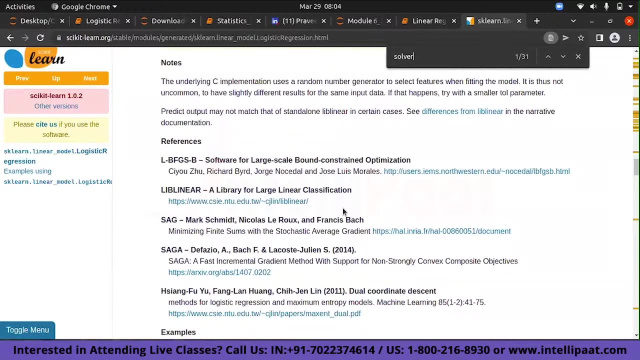 So, if you can see, we have used something called as LibLinear. LibLinear is a linear classification solver. So, which means the method that we learned right, using linear regression, we are fitting a curve, right sigmoid curve. we are fitting using a straight line. So that is your LibLinear. 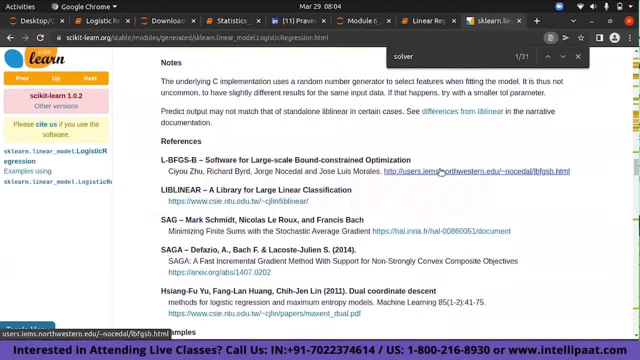 The reference is there. all of them are some international universities where people are given right. So SAG is based on a gradient descent kind of approach. So this is stochastic average gradient SAG stands for. So this is based on gradient descent approach. and then SAGA is again strong convex optimization. So this is fast. So there are. there are various. 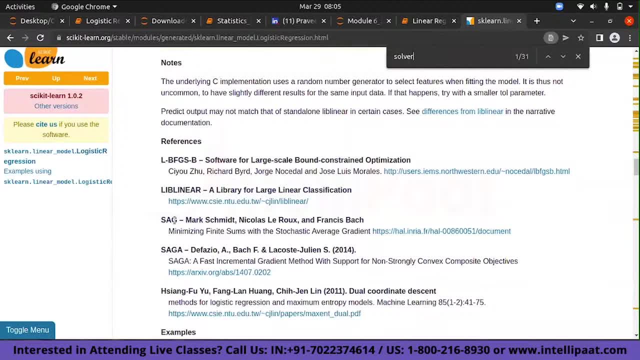 ways of finding a same sigmoid curve, So optimizing different, different types, right? So these are. this is what a solver means. What we have used is a linear solver, which means the method that we used. right, We found out log of odds and then we did all that. 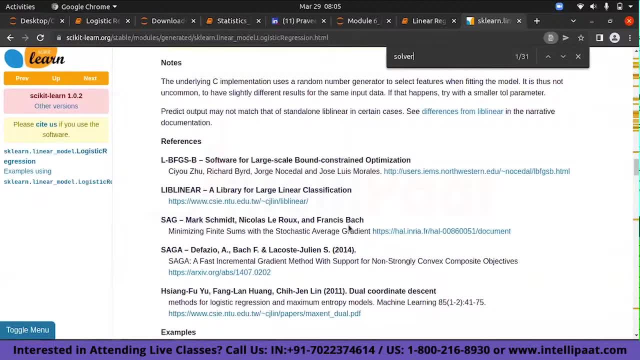 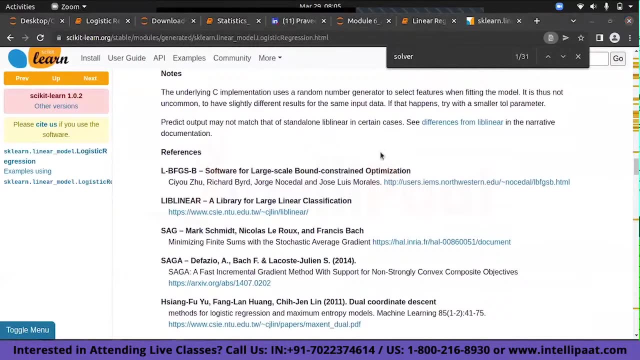 That's a LibLinear. Similarly, there are different methods by which you can find the same solution of sigmoid curve. So that is your solver. I'm not going into everything in detail, So I've just shown you how you can just get it right. So does this answer your question? What is solver? So some 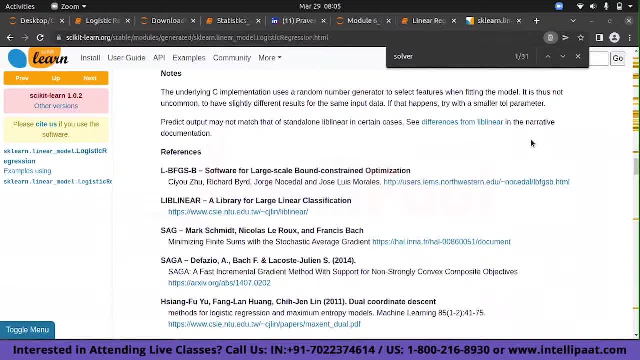 solvers would help you to. some solvers would help you to get better results. Some solvers have some constraints. So, just Like I'll tell you, based on your problem, you can use some solvers, You cannot use some solvers. So 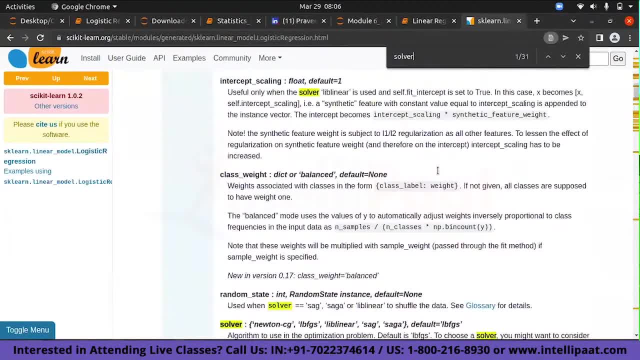 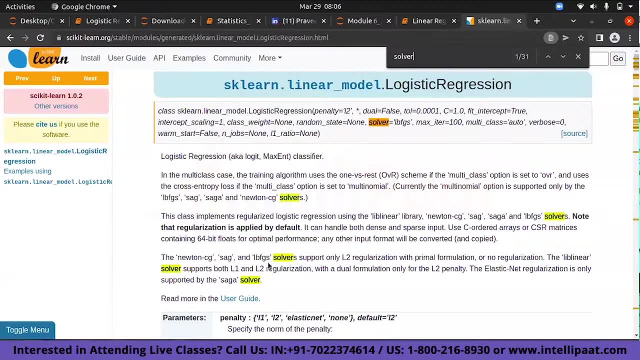 I'll tell you. what is it. So if you can just go to logistic regression here on the top, they have mentioned what to use, what not to use. You can see. the Newton, CG, SAG and LPFG solvers only support L2 regularization with primal function. The LibLinear supports both L1 and L2 with duality. 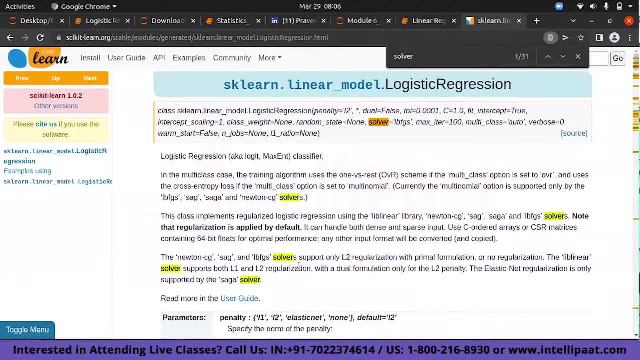 formulation. So this is something which you this, this you will get it When you go into depth. So this you will not get at this point in time, Right? So there are some constraints. So what is L1 regularization? What is L2 regularization? So those things and all you. 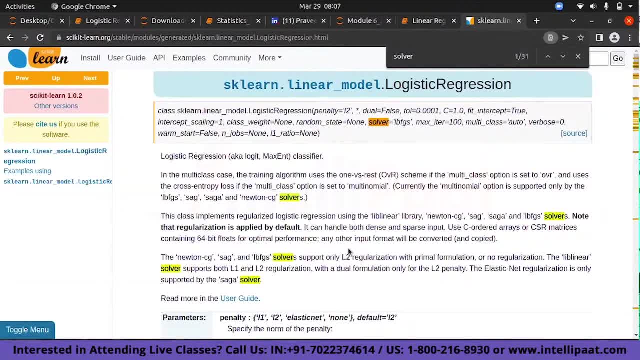 have to go ahead. So everything is mentioned here itself. So you can use, and then you may do that here, If you can see in multiclass training algorithms, multiclass that uses cross entropy multinomial, currently multinomial supported by- only by LBFG. 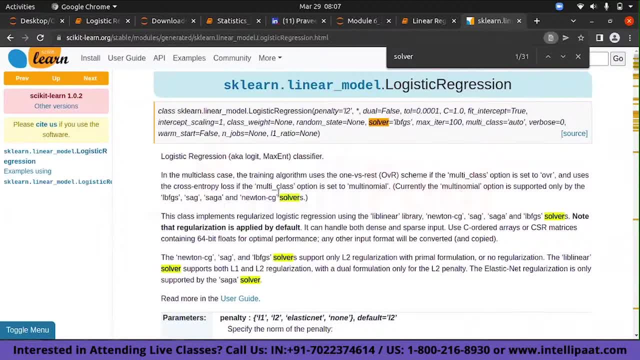 SAG, SAG, Newton, CG solvers. multinomial is supported by these Right. So if you want to use binomial, let us say linear, Right. So client regularizing using these things, Right. So these these some things you need to read and then, based on your problem statement, you can use it. So you can't. 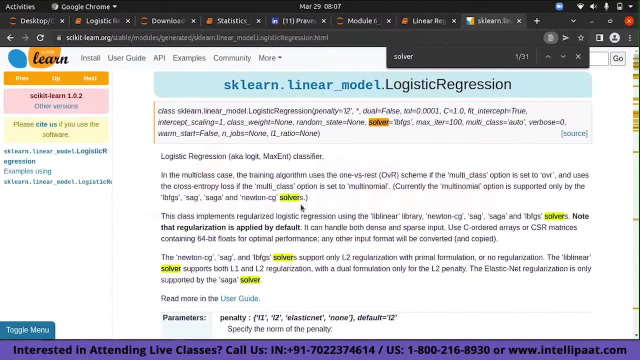 use any other solver. I mean you can use it, but you cannot use LibLinear for multinomial because it is not supported. So something similar to these things. you have to go through and then you can use it. So if you want to use binomial, let us say linear. So 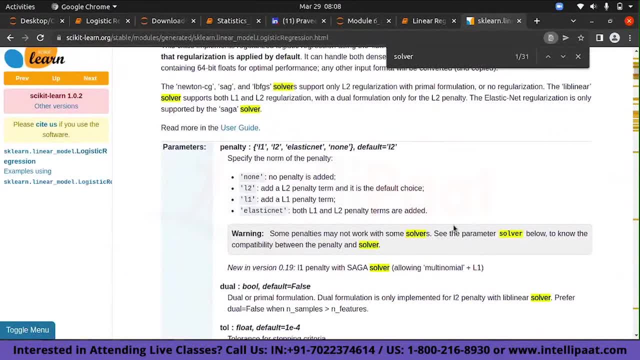 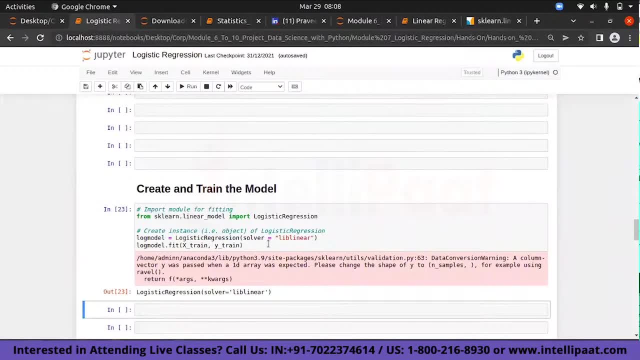 if you want to use binomial, let us say linear, So something similar to these things- you have to go through all these things in detail, Right? So you'll get all the resources. I'm just showing you how this works, Correct? So we're not going into the complete detail of it. But as of now, since we 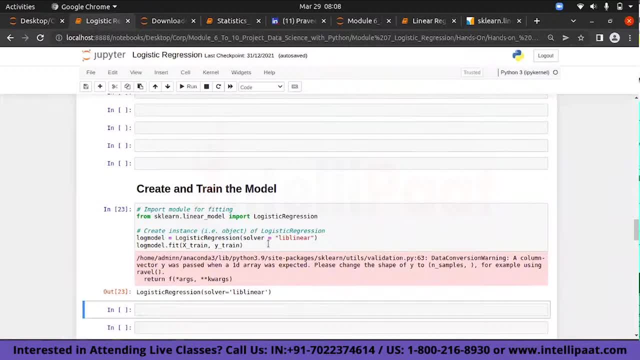 used a linear approach. so we are using the LibLinear solver and we are solving it. Is this fine to all of you? Anyone has any questions at this point in time? Are you following it? It will almost be similar, only not be like different, but the performance will vary for each solver- LibLinear- 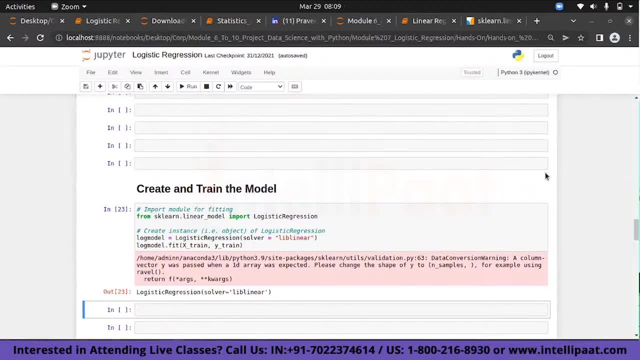 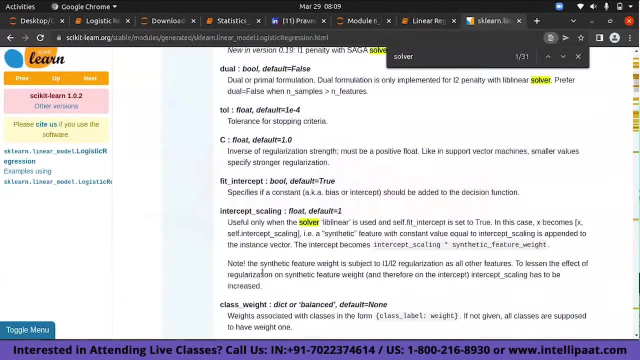 only most of them will use. If you don't use solver default, it will take. So there is no, there's no issue. So you can see, LBFGS is some kind of optimized way, So it stands for large scale bound, constraint optimization. 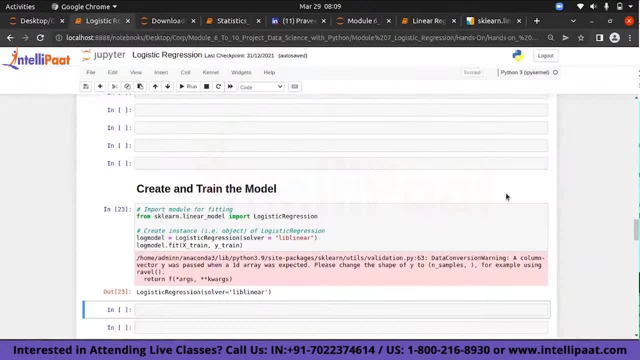 That is a different way of doing it. Default is the LibLinear one. All of you getting it. Are you following the steps, following the flow? So now, if we were to go ahead and then check Things that we were seeing, We'll just go ahead and then Right. So this is how you create your. 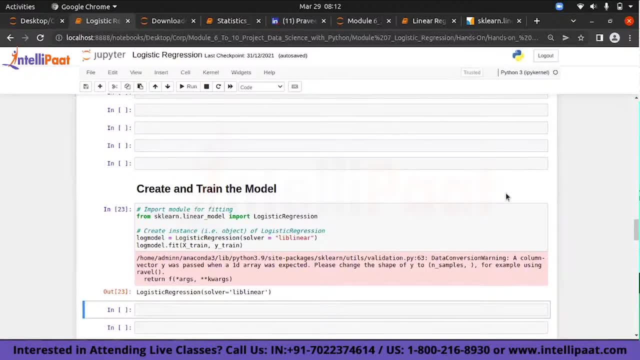 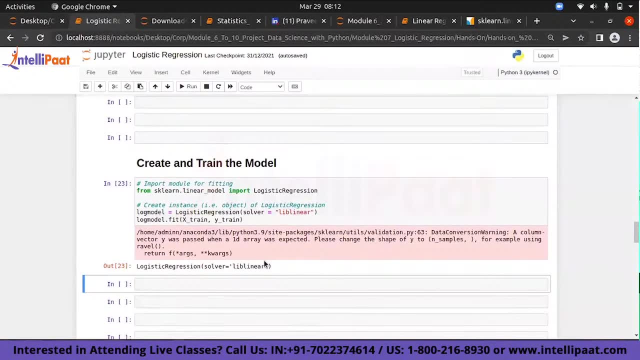 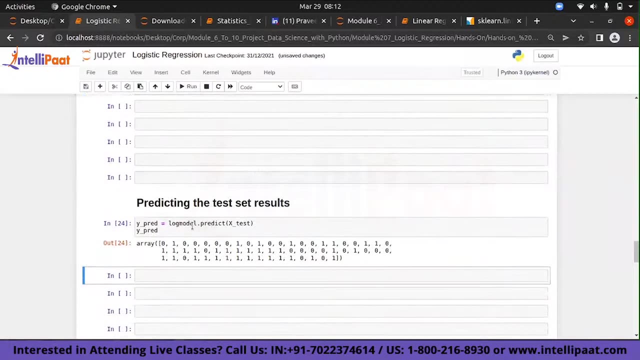 logistic regression model. You created your logistic regression model and then you have done it. So nothing to worry, because everything your data takes care of the back end. So your model is done. Now you are just doing a prediction, So predicting the results, So you can see predicted. 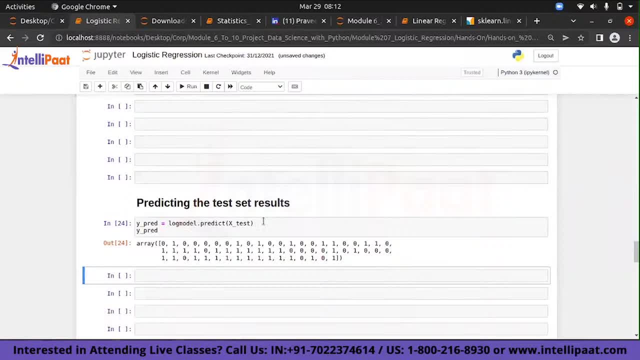 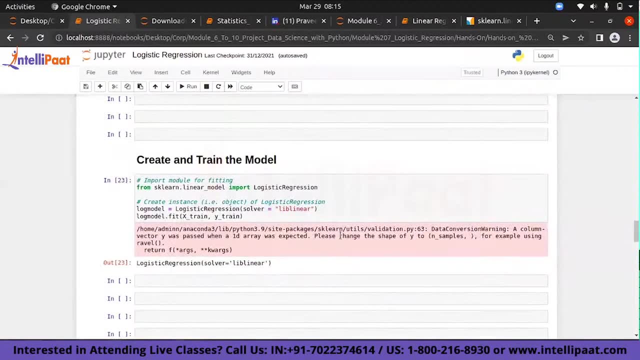 log model: dot predict of X test. So you're predicting it based on your X test. Can you run this? Take few minutes. So you're just trying to predict. So how many values are there in the test? Those many you'll get. So I have taken 20 percent, So that much I will get. 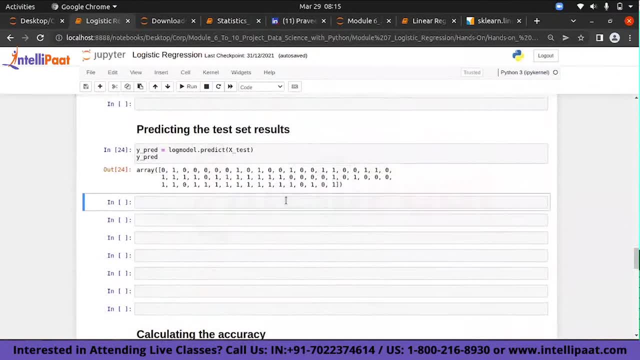 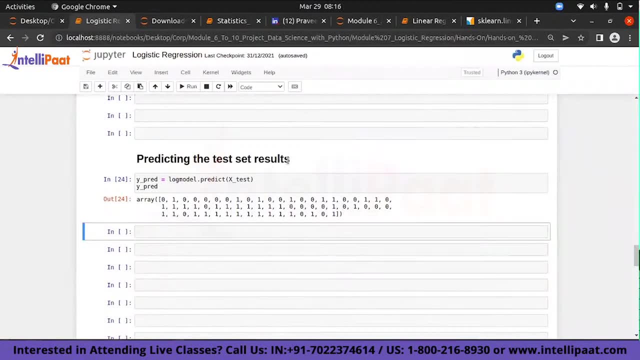 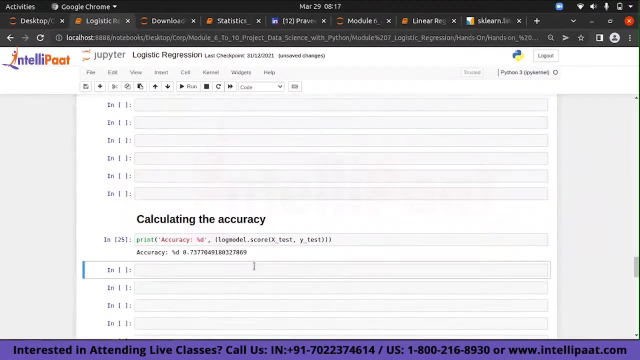 Yes, So what I will do is once you have done this. that is one important thing that we will understand today. Before that, all of you are able to achieve this, Cool, No problem. So now next thing is we need to find out the accuracy So you can see you're getting a model with 73 percent. 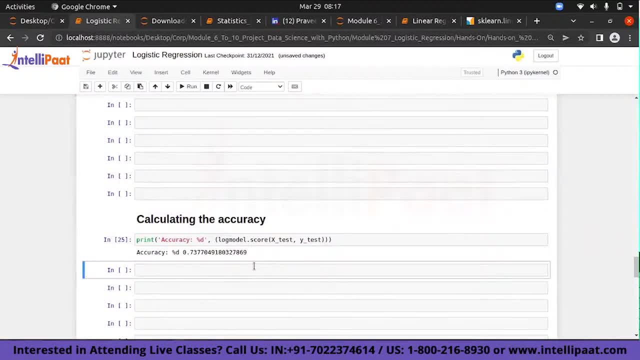 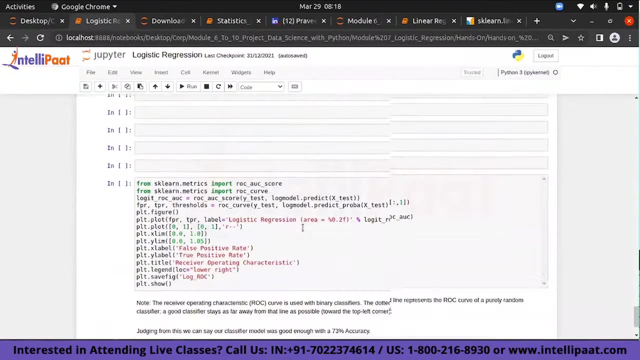 Accuracy. can you try this out? accuracy may vary, who worries? but you got it right. nice, very good. all of you others, are you getting this cool now? you have done till accuracy. so now, if you can observe, there is something called as a evaluation criteria. okay, so there's something called as a. 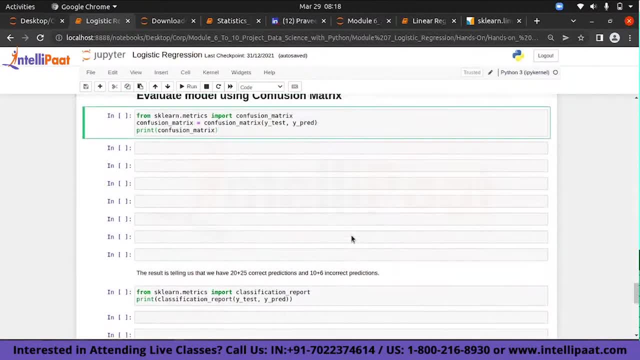 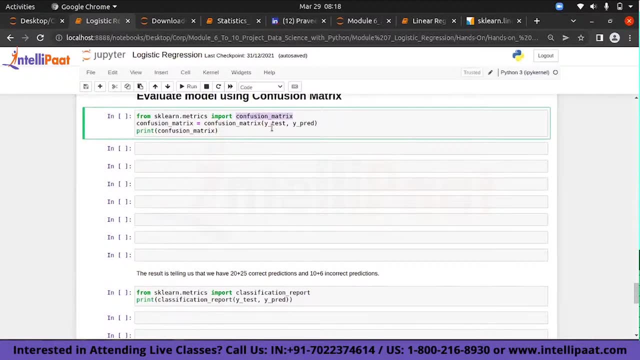 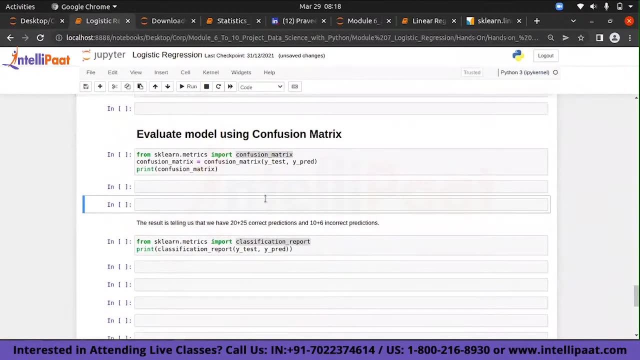 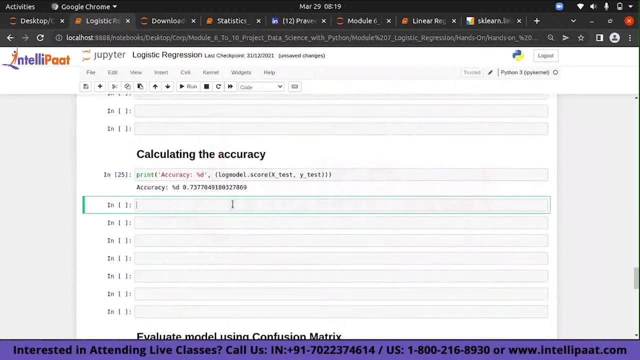 evaluation criteria. there are two things which we are taking- you can see here, understand this carefully- from sklearn matrix import confusion matrix. from sklearn matrix import classification report. so basically so these two things we will use to find out how accurately my model is performing correct. i'll also show you how this number can be got. i'll ask you to do a small math. 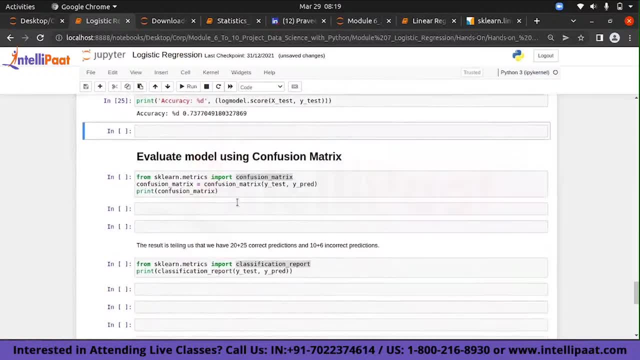 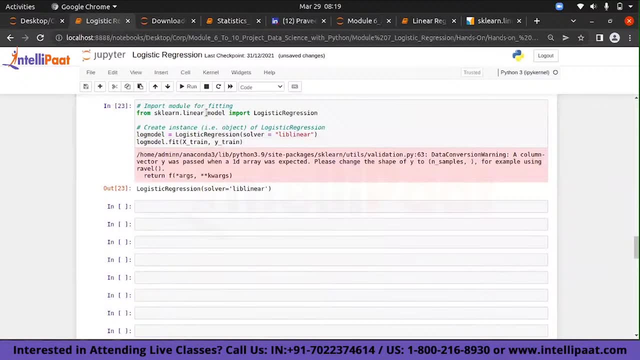 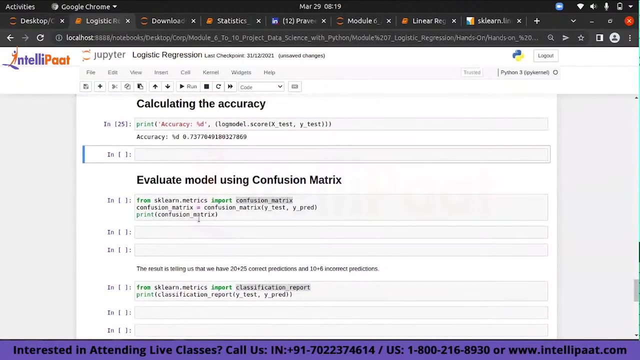 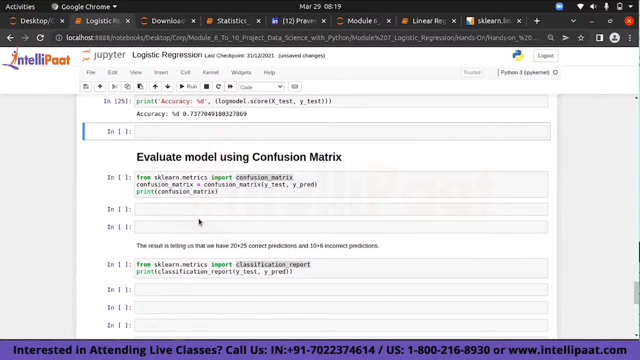 now just a small calculation. just observe this carefully. so, just like how you had sklearn dot linearization model, sklearn dot linear model is a folder where you will get logistic regression function. similarly, sklearn has multiple metrics. so when i say metrics, metrics are nothing but the functions for measuring model accuracy. so sklearn matrix, you import confusion. matrix, sklearn matrix- import. 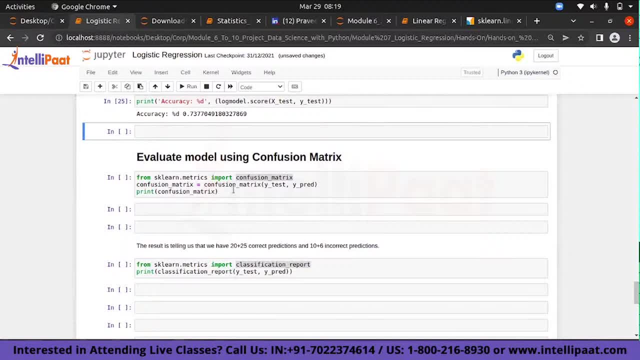 classification report: right, confusion matrix. you have to compare between y test and ypred. so if you compare y test and y pred, you will get a confusion matrix using which you will be able to do that. cool these two things. i have not gone into detail, but just letting you know. are you, are you getting these? 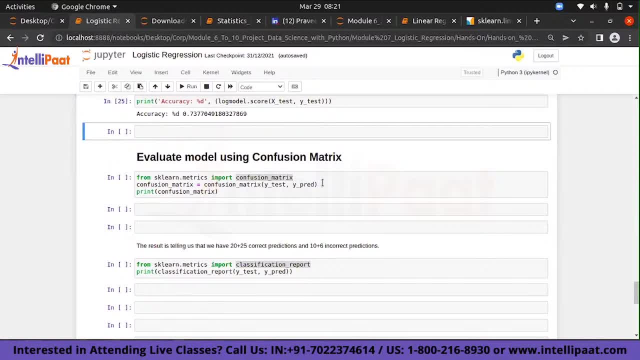 two lines correct. so basically doing it, yes, but now what we are trying to do here is, if you can observe, one thing that i want you to understand is you're comparing and then getting our test and predicted values. now, if you run this, just run this, you will get a small matrix kind of a structure. 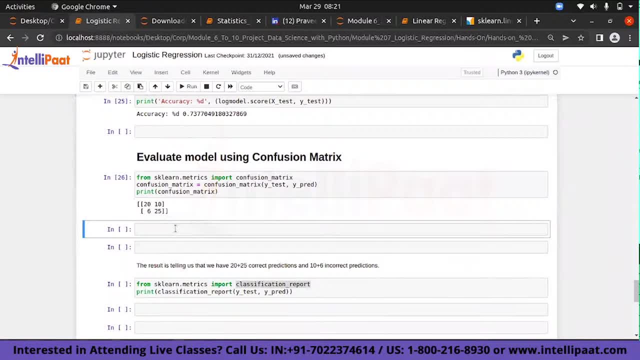 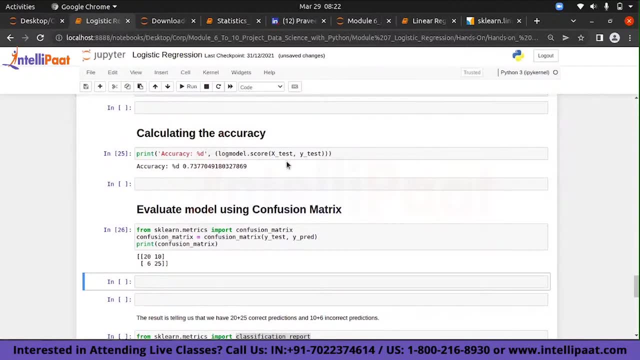 all of you got this slowly. do it, no problem, slowly do it. just observe, i'll show you one thing: how exactly this works, your accuracy. you got it by using log model score 73 here the see this you cannot remember always, because this is not a standard form. okay, so this is not standard form. 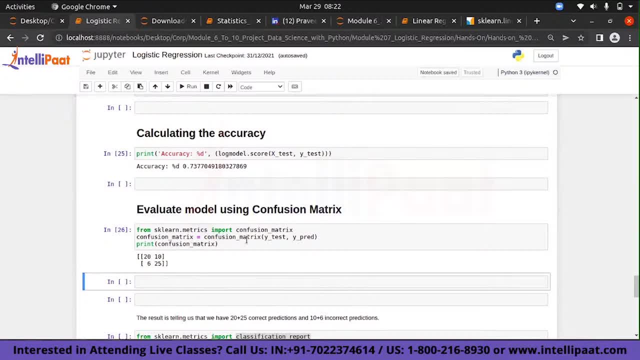 this one is a standard form, any, any model. so this is a standard form of identifying. so the first thing what i want you to do whenever you get a confusion matrix. so what is the total here of all the four numbers? 61, correct? you're getting 61. right now take the diagonal elements 20 and 25, which is 45. 45 by 61 is how much, just. 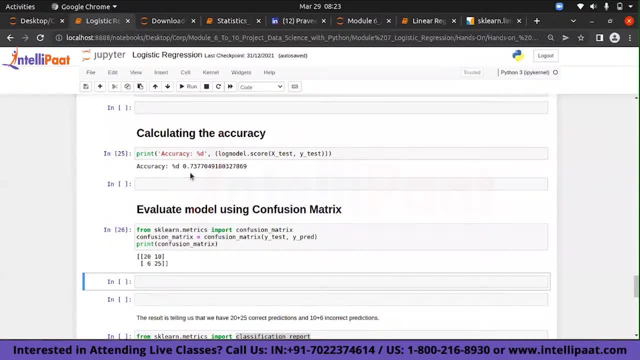 divide 45 by 61, are you getting your accuracy score here. so this is the standard way of identifying accuracy. so confusion matrix will give you all the things that you want. so one link i will give you to understand confusion matrix better. so that link is wikipedia. so this, this. 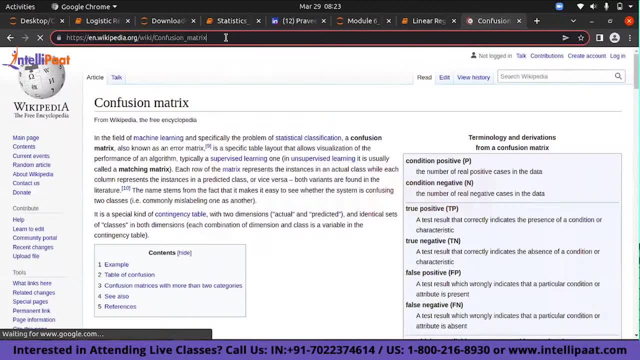 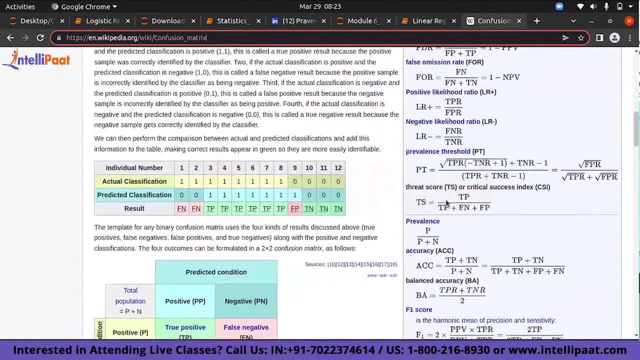 gives you a full understanding of your logistic regression confusion matrix. so you can see there are true positive, true negative, false positive, false negative. all these things will come for us. what is the confusion matrix that we did is? you can see it's a very simple way of identifying. 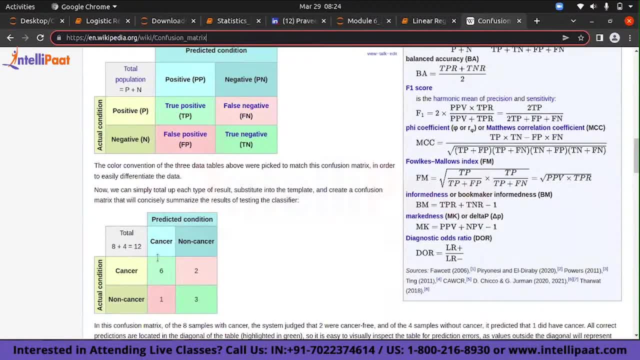 you can see three things if you want to know what happened in this situation, if you want to know how many times this situation happened, and so from your prediction, you can accurately identify these two things. so if you are looking at the index of the left hand side, you can. 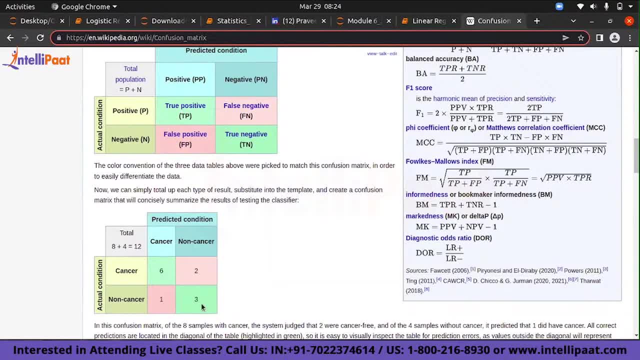 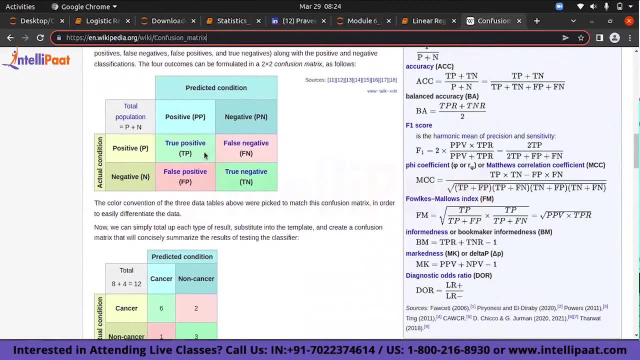 see the blue line in the middle right now. you can see the blue line in the middle of the two plus one and you can see that the blue line. if we were looking at the right hand side, if you were looking at the left and right side, it would be negative because 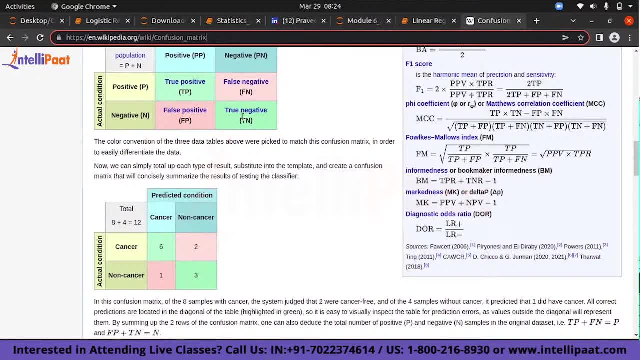 of the relation between the left and right. so it's very simple. right now, you, if you think true, negative, this is called as false positive, which means when a person doesn't have it, you are telling he has it. that is false positive. when a person has it, you are telling he is not having. 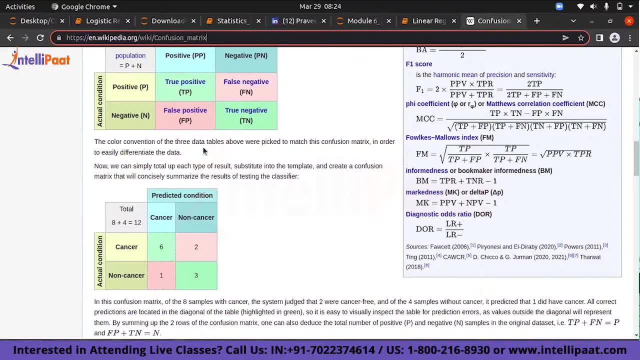 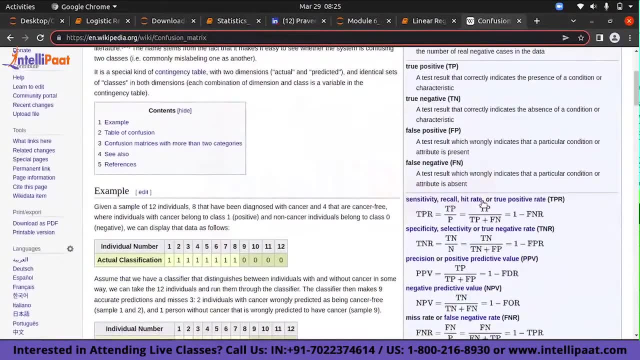 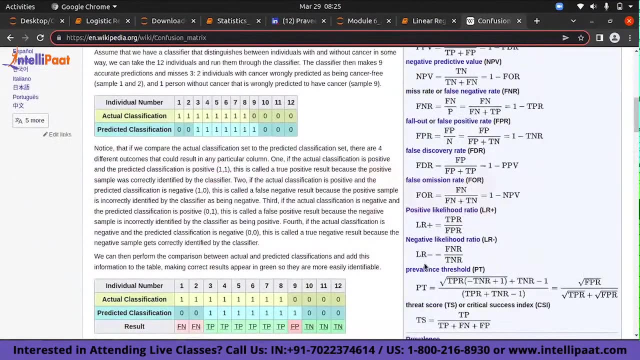 it. so that is false, negative, so both of them are errors. so this is one basic level understanding of confusion matrix. apart from that, you have multiple things, which is called as sensitivity, specificity, precision. all these things you will have, so you can just go through this and whenever you want you can use these things are nothing but a combination of these only. 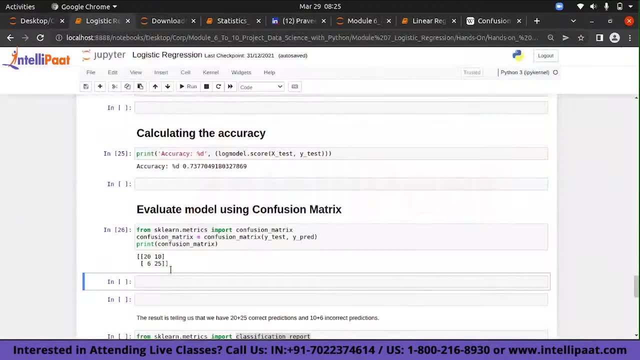 mix and match of this. i just told you about this small table. got it exactly: confusion matrix is something that is required, true, cool. so basically, if you can see, 20 and 25 are correct predictions, 10 and 6 are false. so 20 when it's yes and yes, you are getting 20. no and no, you are getting 25. 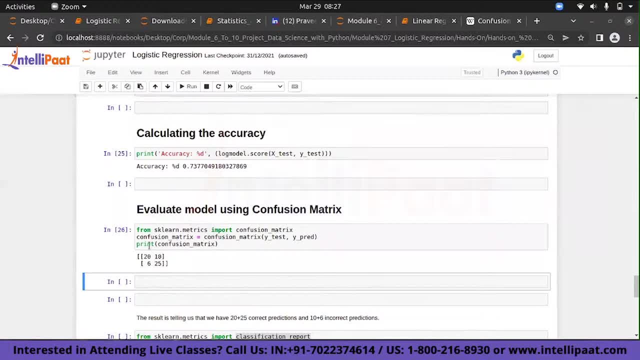 when it is no and yes, which is a false, you are getting 10. when it is a yes and no, you are getting 6, which is also a false. so basically, 20, 25 are the correct prediction. exactly true, david. what you said is correct, so you are. 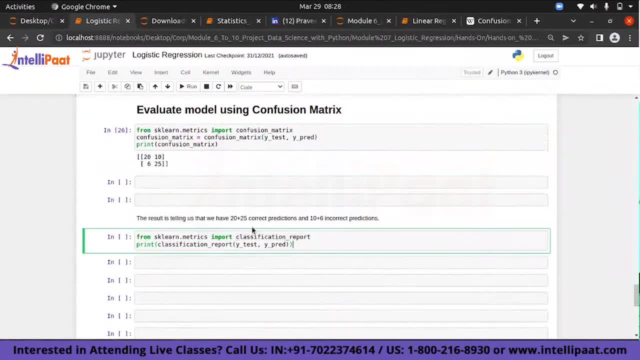 marking them as negative, correct, which is not correct. so the result telling us what you have: 20, 25 is correct prediction. 10 plus 6 is incorrect prediction. so here, when you have 10 plus 6 incorrect prediction, so you take 20, 25 by total. that will give you the accuracy. cool getting all. 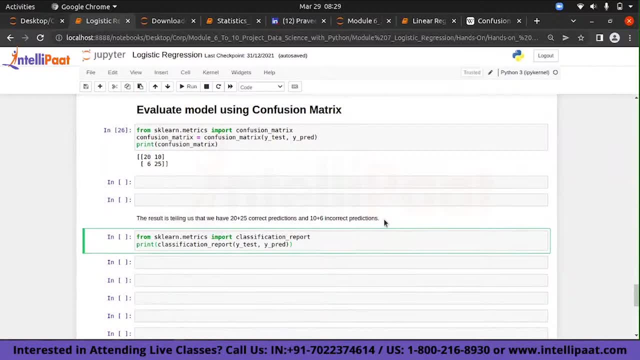 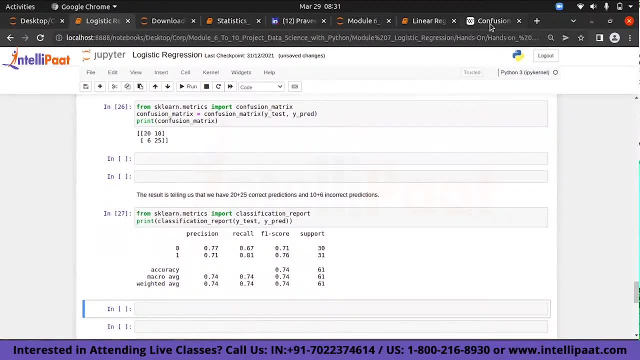 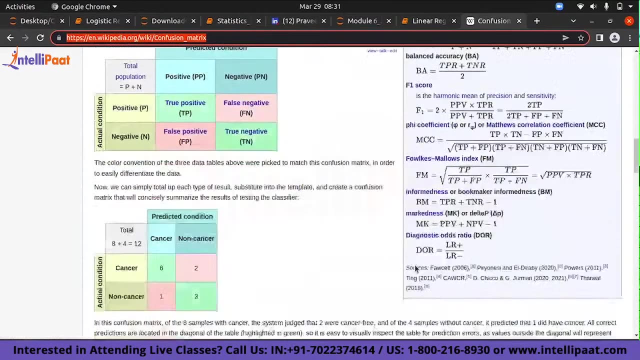 of it. so now do the same prediction report. try to type this right. so if you generate this one, you can see in confusion matrix. if you can see, you saw you had some values right so you can see here accuracy f1 score, all these things. so these are some of the important things that are required whenever you are building a model to check. 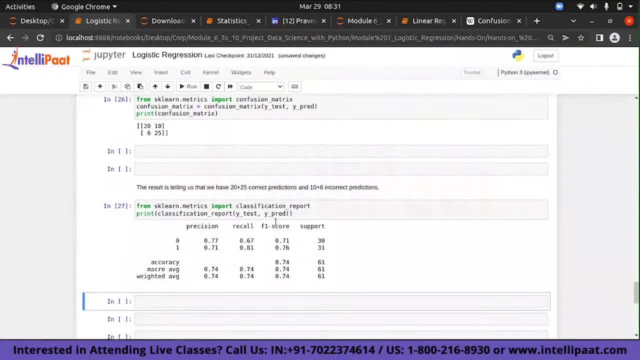 the performance of your model. so, basically, a classification report will give you all this so you can see precision, recall, f1 score, all these things. accuracy, all of you know it is like 74. so this complete report, it will generate weight right. so this is something which i wanted all of you to understand is this: 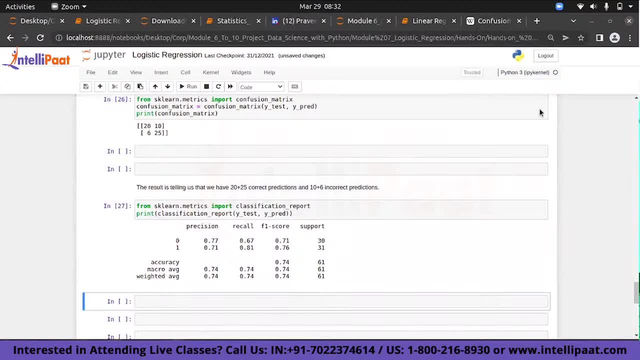 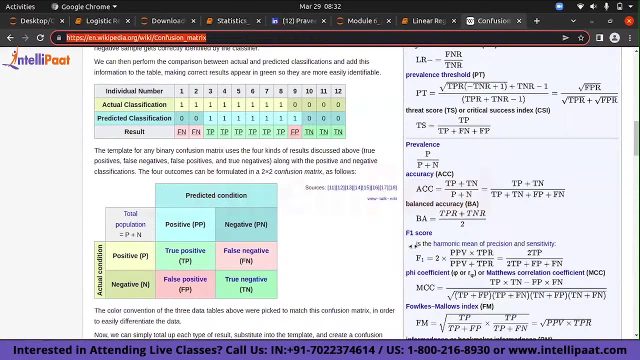 fine getting it. all of you is it. is it good? some people getting different accuracy because sampling might have become a little different, so that's okay. so this report will give you the f1 score confusion matrix, all these things i showed you in this particular link. i told you these things can be calculated right so you can see f1 score accuracy, precision. 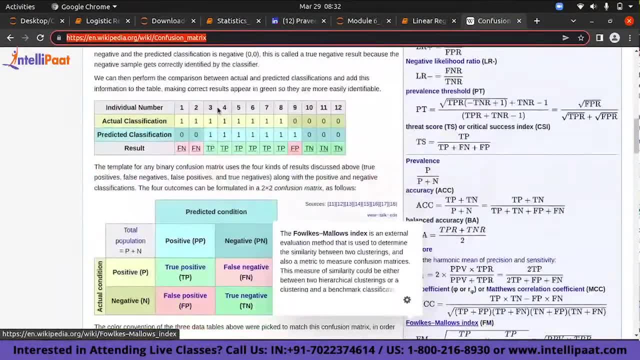 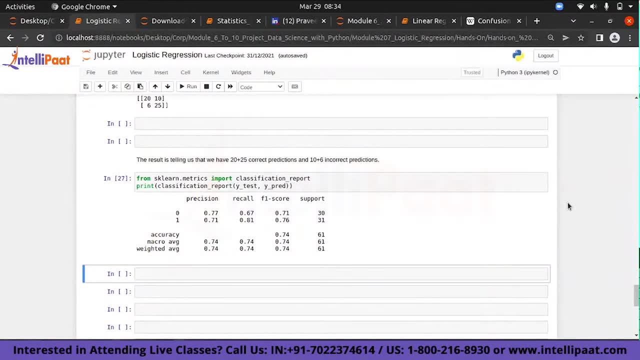 all these things. so there's no need for us to calculate all of them. so there is a function that will give you that, which is your classification report. cool, fine, let us say, for example, how do i explain? okay, so what? basically, macro average is a problem that comes in when you have multiple sets. 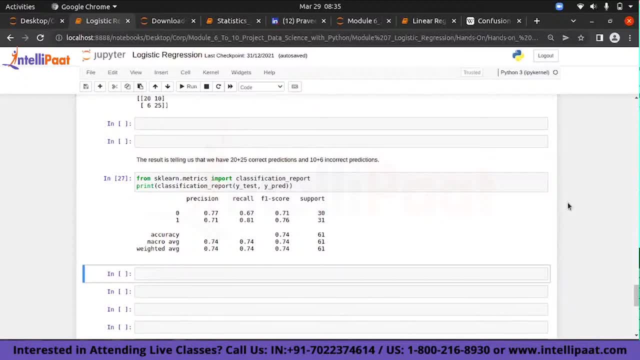 of binary predictions. so i mean it. it has a whenever you have a multi multi-class prediction, right? so you have multi-class predictions, whether i mean here you have zero and one, but let's say you have zero, one, two, three, four, which is a multi-class prediction. now, macro average. what it does is it will bring down your 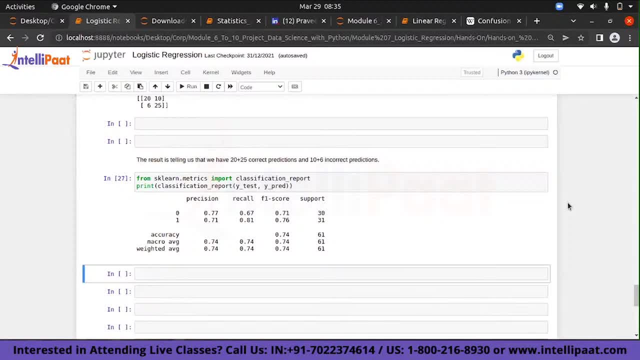 multi-set of binary- i mean multi multiple predictions- into a multiple set of binary predictions, calculates the corresponding matrix for that binary cases and then averages it. let us say, for example, you have zero one, two, three, four, five, six. it will take zero one, two, four, five, six, like that binary it will take and then it will. 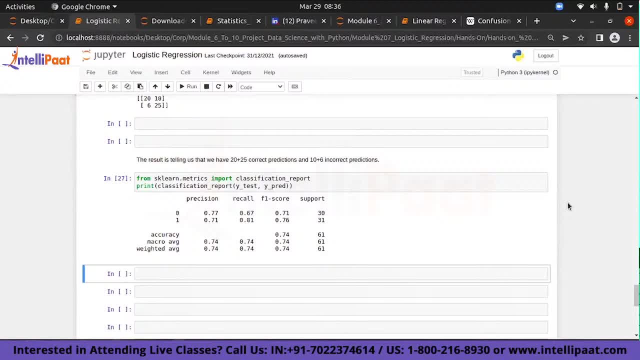 take an average and it will give you. so that is your macro average. so weighted average is nothing but few variables will get more weight, few variables will get less. so that is something. so all these things are here. support confidence. f1 score: yeah, since it's a multi-class prediction. 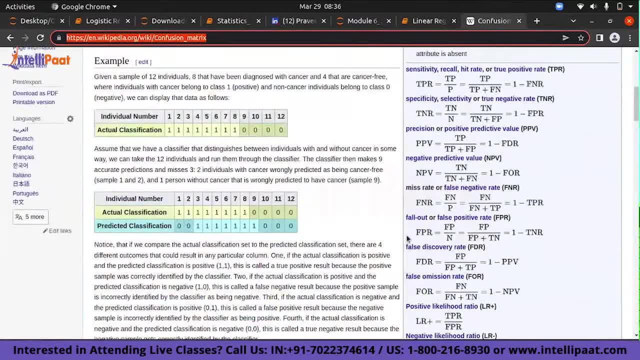 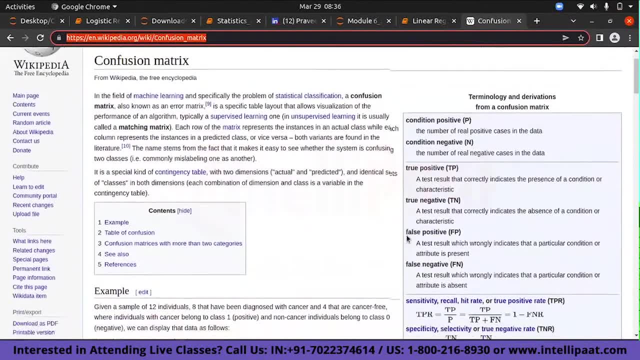 it is binary, we are getting the same thing. you can see all the things that are mentioned are here, so that depends on what business value that you want. so f1 score is a harmonic mean between your precision and recall. so what is precision? what is recall? true, positive, rate, false positive. 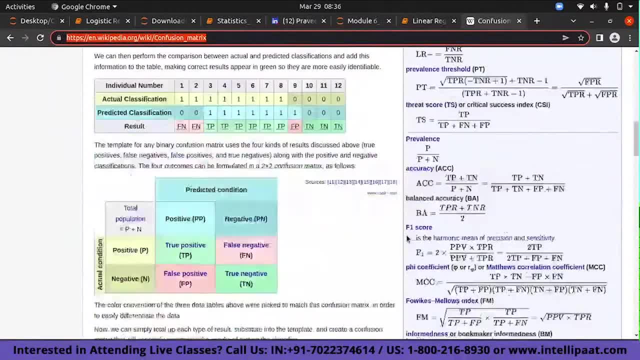 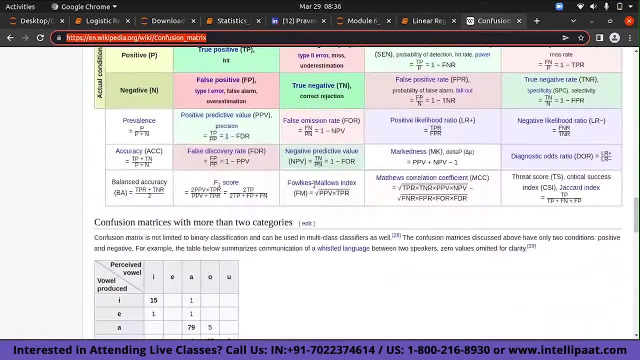 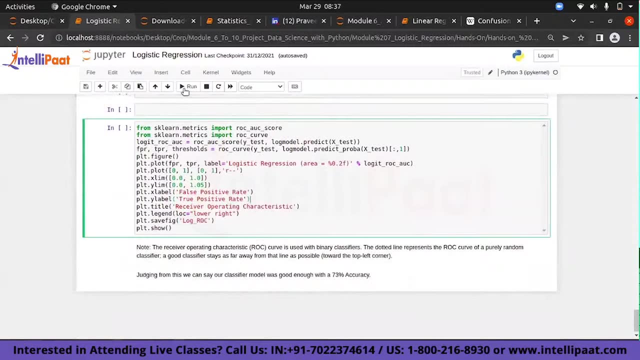 rate out of them, how many true, how many- falls? so all these things are here, so that's why i gave you this link. this will give you a complete understanding of the conclusion matrix which is required, so this is something that you can explore right now. last but not the least, i don't want you to type this, i just want only to. 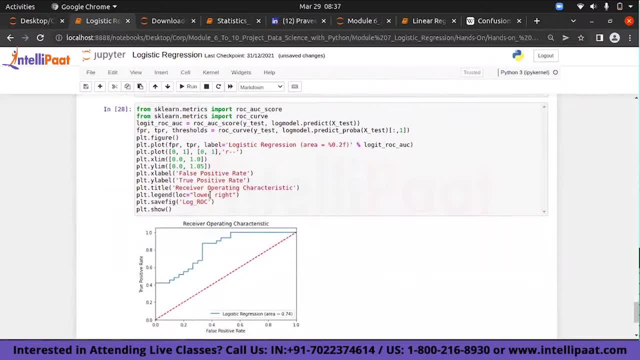 understand it, i have something called as a roc curve. so roc curve stands for a receiver operator characteristic curve. so roc means receiver operator characteristic curve, right, so now how am i going to use this particular receiver operator characteristic curve for my analysis is what we are going to see cool. so we are just going ahead and then we are just 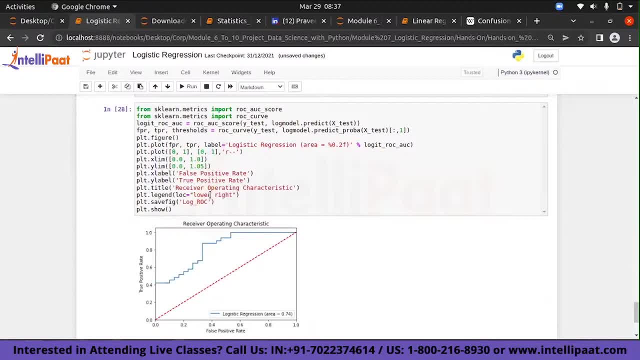 trying to do it for our analysis and then we will understand how we are exactly doing it right. slowly, we will see how exactly an roc curve is constructed. so if we can observe this roc curve, how exactly it comes, is just hold on. so, basically, whenever you have this particular roc curve, how we 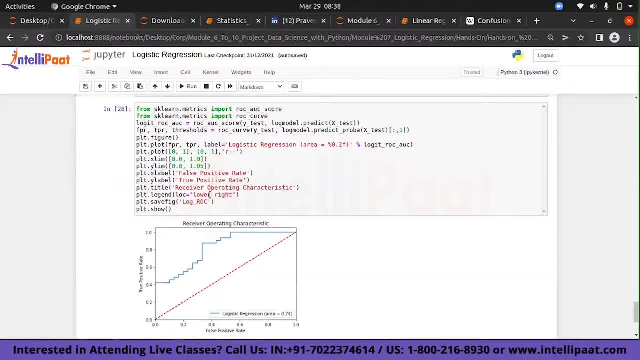 are going to use it, how we are going to use this particular roc curve, how we are going to use it or probably how we are going to construct it is something we will see now. right? so, whenever you have your data, you will have two things. right so, you have positives, you have negatives now, whenever, 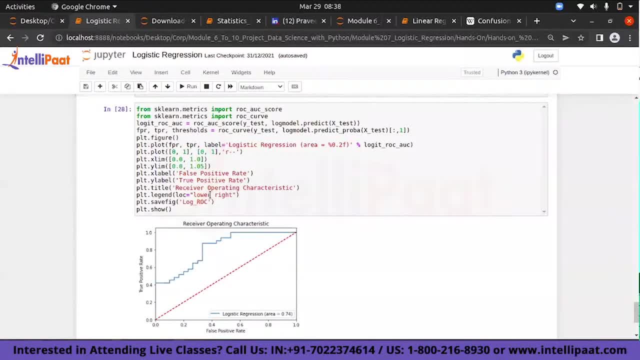 you have a positive or a negative, for that matter. so there are two things that you can do. so what are those two things? you can find out: a false positive rate and a true positive rate. right, so there are two things that happen here. the first one is that what are the positive? and the positive rate is a 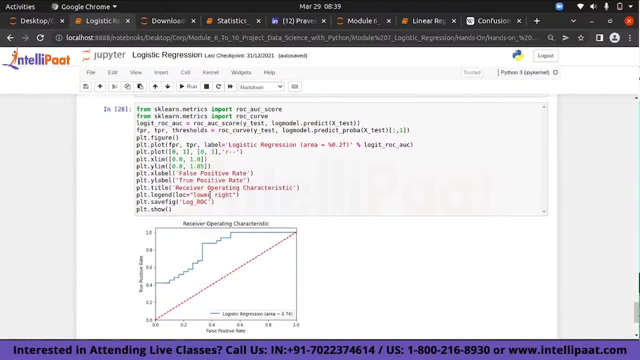 false positive rate and true positive rate. now, having said that, so with the false positive rate and true positive rate, you are plotting a graph. so, based on the understanding of this, you are plotting a false positive rate and a true positive rate. so, when you construct a graph like that, the 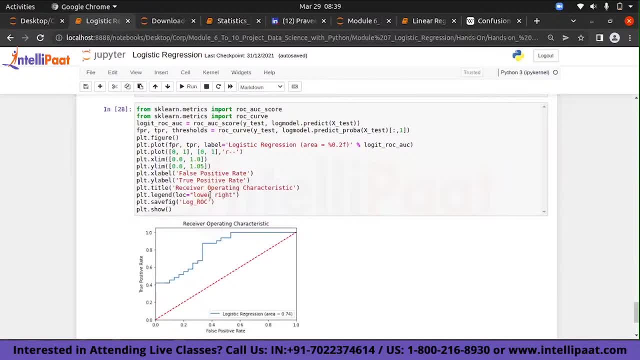 red line. what you're giving is like a baseline, which means the blue line. what you're checking there on the top should not go below that. so that is something that is there now. having said that, whenever you get to see a roc curve like this, you will be able to identify how my model is. 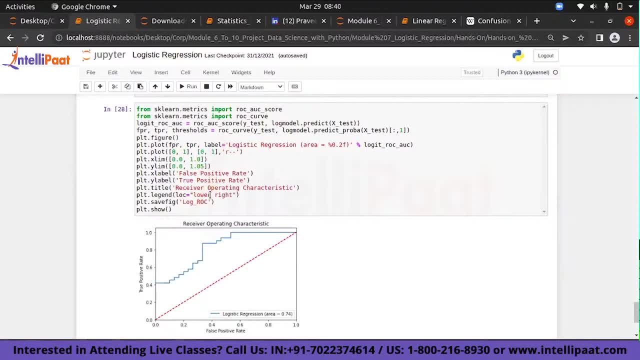 performed. so if your blue line and red line, blue line is almost near to the lead line, which means my model is not so good model, the far away the blue line is, the better the model is. so that is something which you can probably conclude by this. so this is roc curve, which will help you. 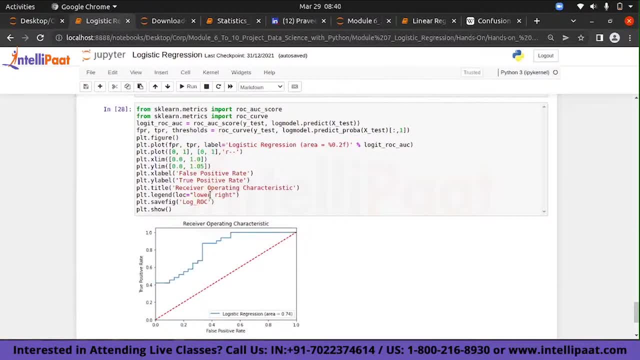 to analyze your model better. so the far the roc curve, the better the model is right. so this is something i wanted to tell you. this is fine. are you understanding it? this is like basic, basic things i'm telling you. i'm not complicating it much, sure. so, basically what we are trying to: 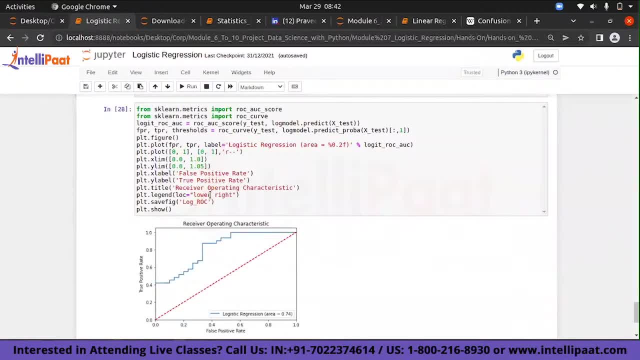 achieve in. this is very simple, so you can see. so i'll explain you this and then we will see my scale and matrix again. we're taking and roc curve, so these are also in between. which is your zero to one right, so which is zero to one, which means 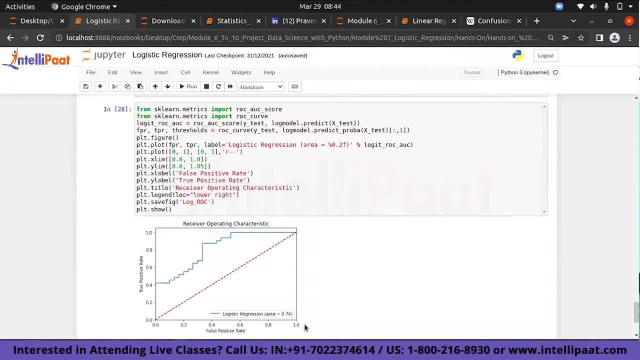 this is your. so what we are trying to do here is: this is like a template, you can use it. so, from here to here, what you're trying to do is just plotting this one, so your plot dot figure. you're plotting your values, right? so zero, one, one, two, all these things is your x limit, y limit, which? 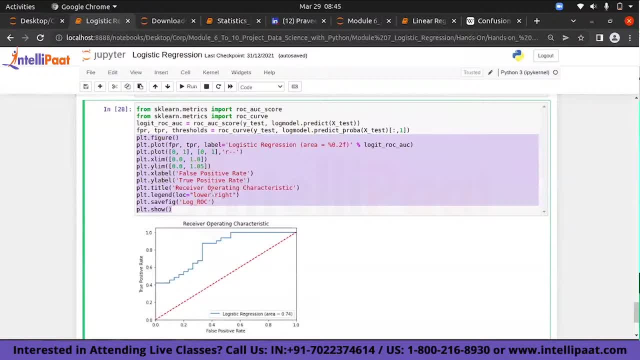 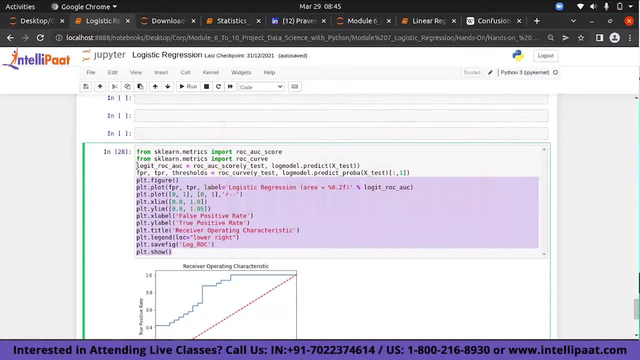 means the axis from where to where you want your x axis to be. title legend: all these things you are giving. now, the main thing that you're supposed to do is only two lines. so these are the two lines, what you're getting here. so roc auc. this is for the blue line. logit roc auc. so this one you will. 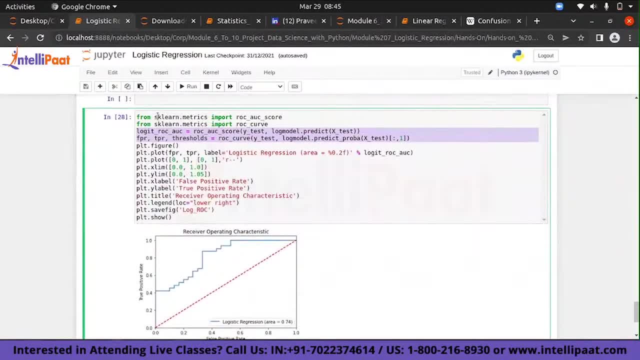 find out by using the roc auc score function from your sqln matrix. then you have fpr, tpr, threshold. all these three things you will again get from the roc curve function. so these lines you need to just remember. no need for you to buy heart or 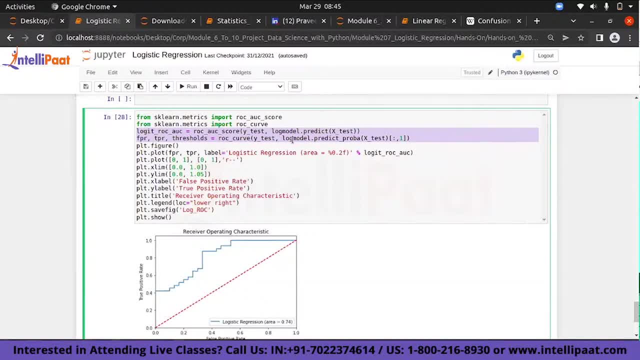 maybe remember exactly this. you can use it as a template whenever you're trying to learn the, whenever you're trying to implement a logistic regression model. you can use this template and then you will be able to get the same kind of graph. so these are not required to understand. 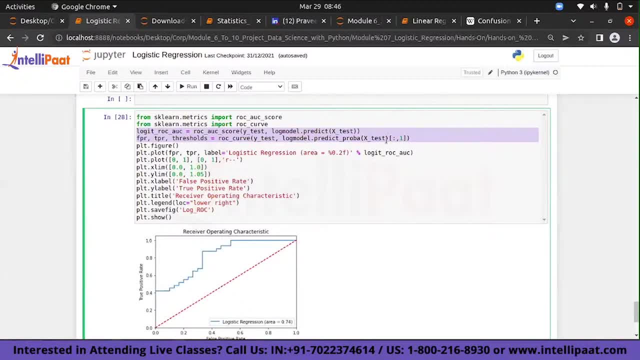 so you're predicting probabilities of x test. so whenever you use x test, no, in the last one is your target. so you're you're taking that one and you're going to get the same kind of graph. so you're taking that one, only nothing else. cool, all of you're getting an idea about all these things. 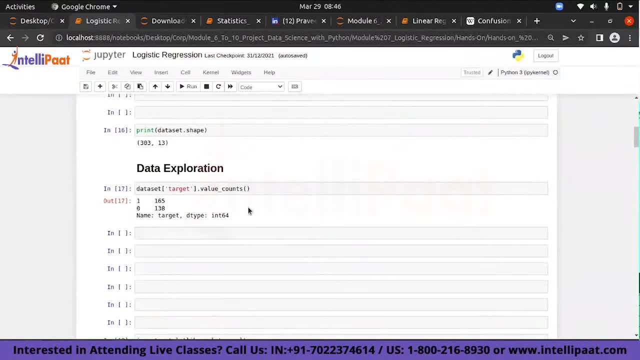 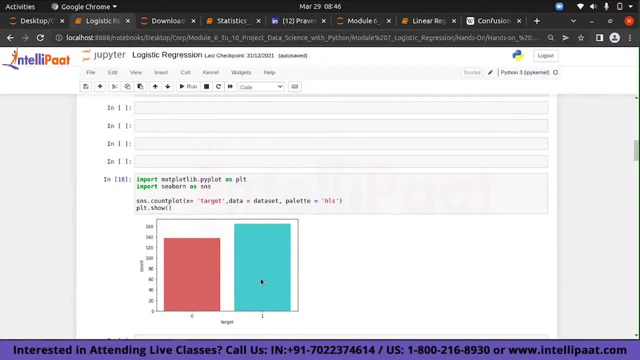 whatever we discussed now. so you read the data, you explored it, you understood whether it is imbalanced or not, right, and then you understood the difference between this. you saw whether it is imbalanced or not visually, and later what we did is like we split the data into training and 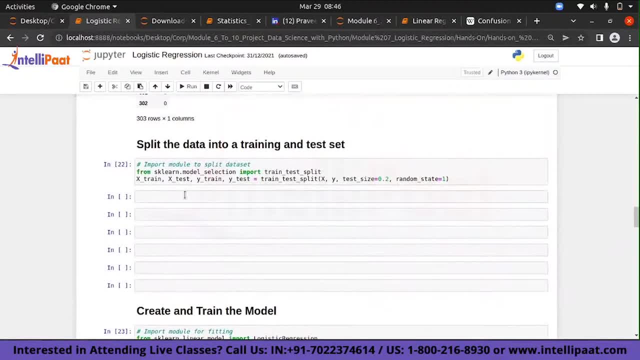 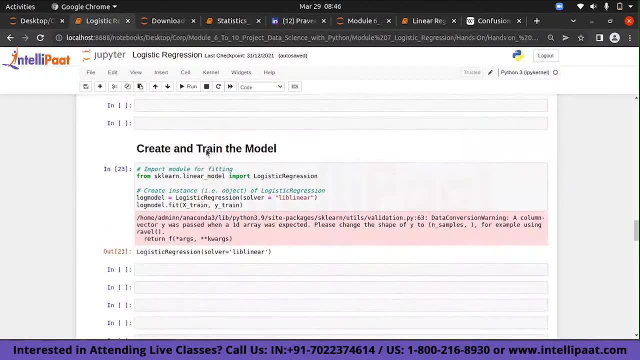 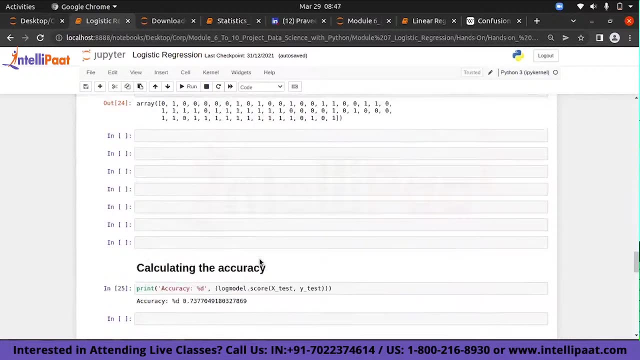 testing data set and then training and testing data set. then you made a x train, y train, y train, x train, right. so these things we understood. then you under we, you built a basic- uh train model, so basic train model. you trained it and later you predicted it training and production. once you do that, you found out accuracy. so one 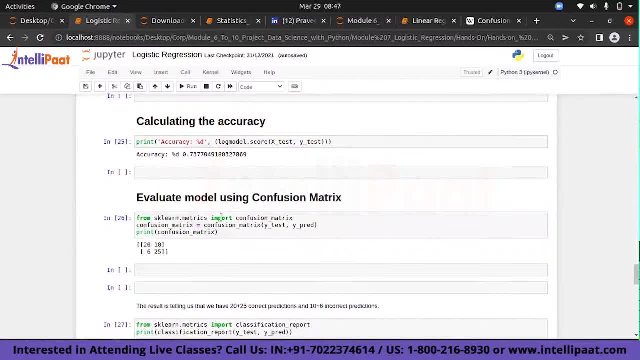 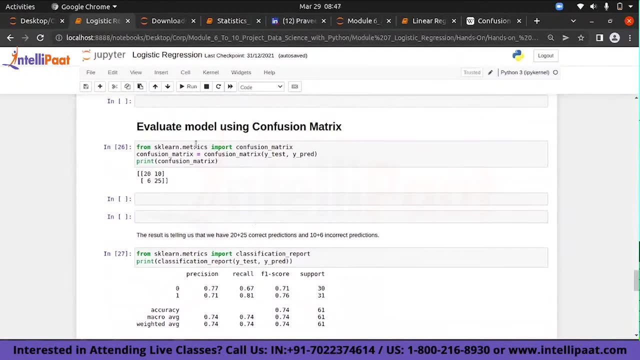 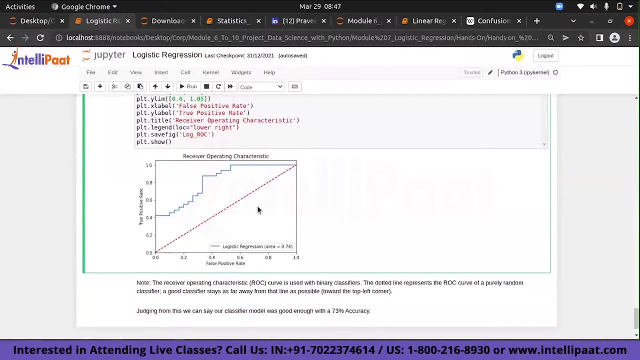 is the log model accuracy. this you can use, or we need to use, confusion matrix. so we understood how a confusion matrix works and also classification report. so confusion matrix is important, so this one you are going to use for our plotting the roc curve. so i told you what is a basic roc curve. 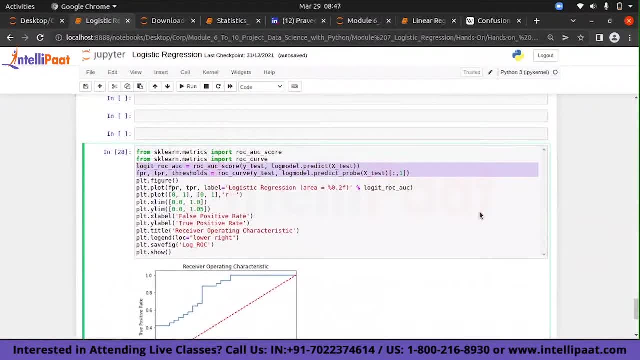 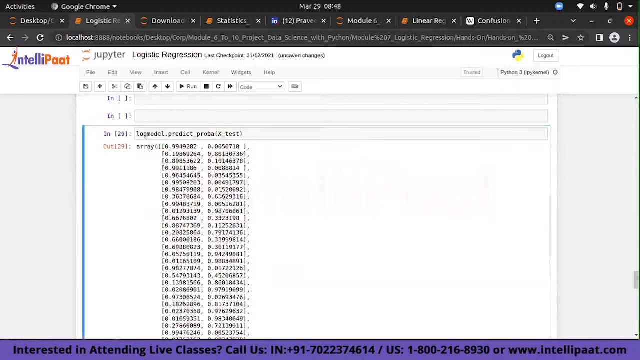 you will be able to understand, it should not be minus one because you're just taking the log model predicted probability. so whenever you just take this log model predicted probabilities, it will give you a term. i don't know whether it will print or not, but i will show you. you can see there. 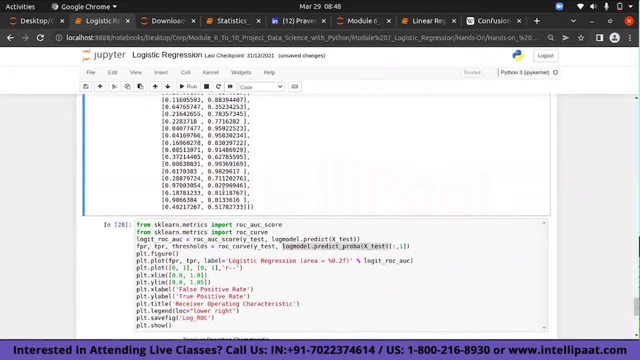 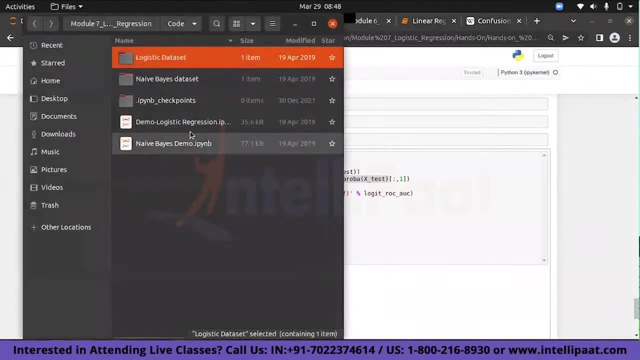 are two things in this, so that is the reason why you are taking the second one through nice. so this is internal, so you can use it as a template save fig. what it will do is it will save your roc curve. so inside the hidden mass output, if you look inside this, i have theoh. thats the method um and the